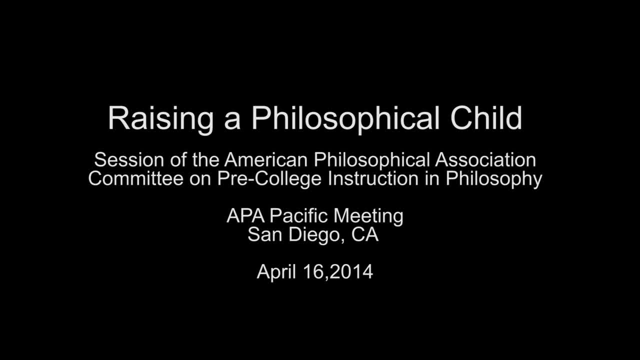 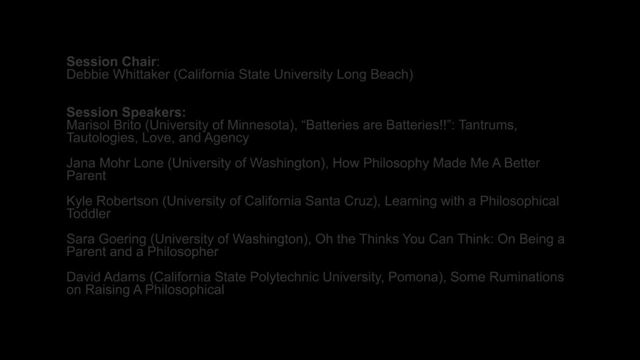 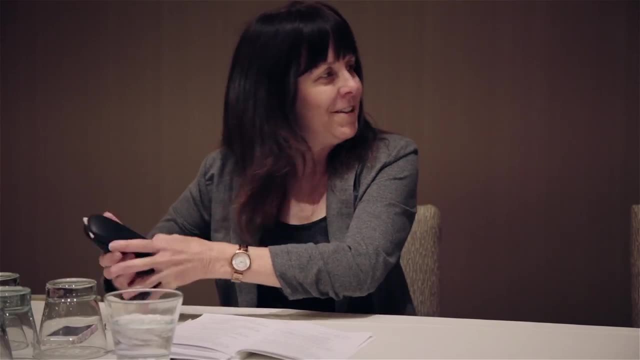 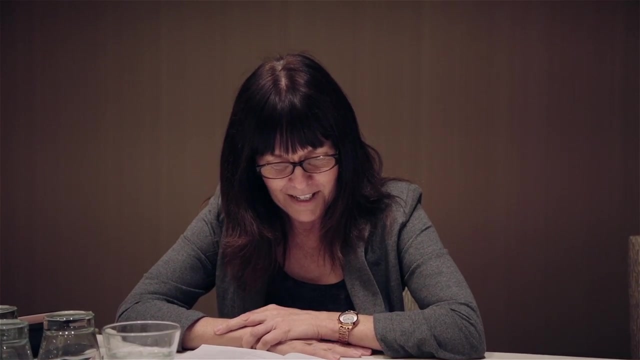 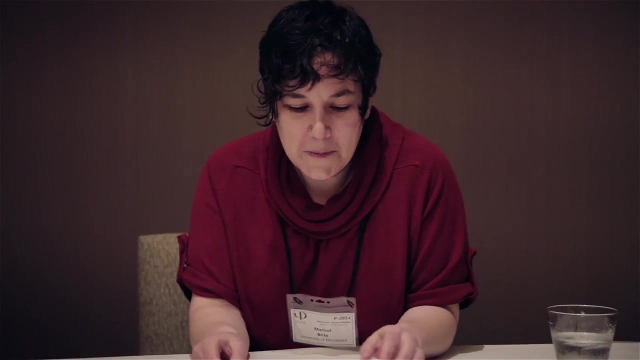 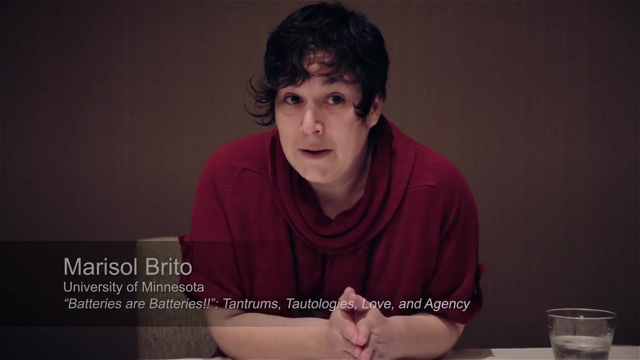 So our first speaker is Marisol Brito, from the University of Minnesota, And the name of her session. I'm not sure I get this right. batteries are batteries, tantrums, tautologies, love and agency. So let's welcome Marisol, Thank you. So it might be the stage of parenting. 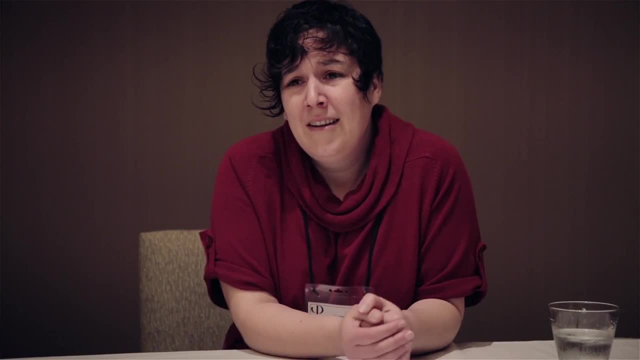 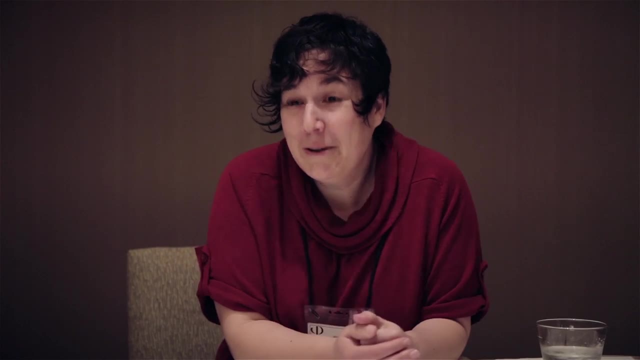 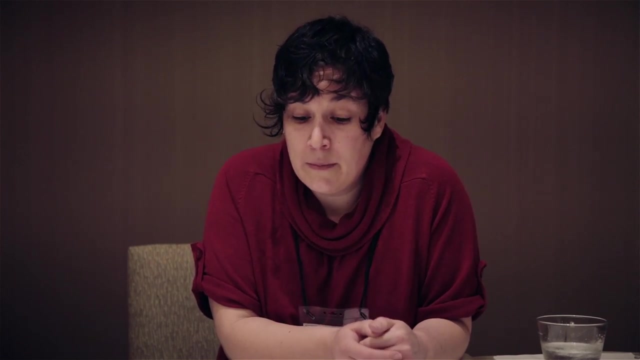 that I'm in, but currently I often feel that, rather than raising a philosophical child, I am being raised by a philosophical child. I experience parenting as key to my own growth and my own learning, And in this talk I wanted to share a bit about how I've come. 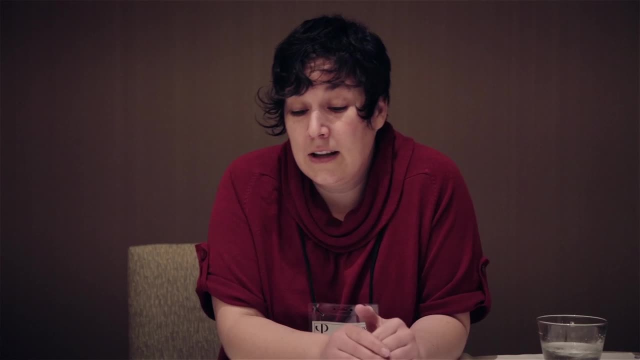 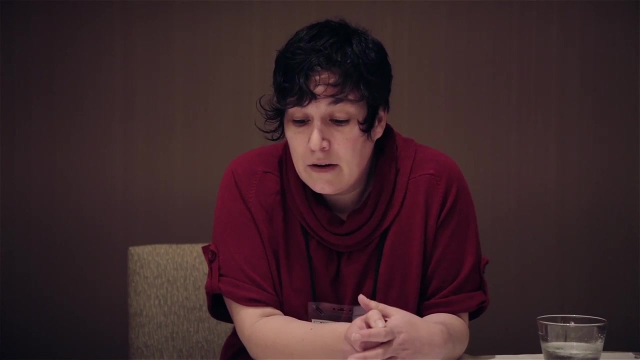 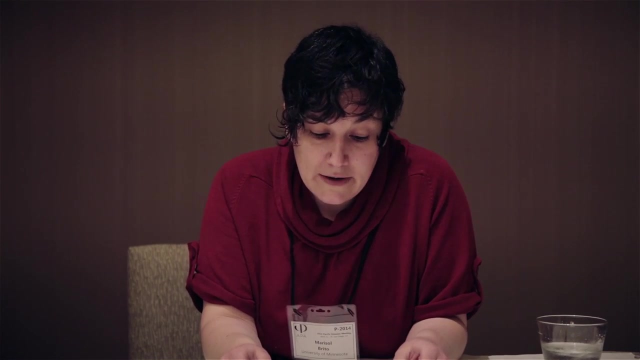 to view parenting as an opportunity to have an epistemologically privileged position, one that influences not only my relationships with young people, but also my teaching, my work in philosophy and my worldview. So the title of the talk- batteries- are batteries. 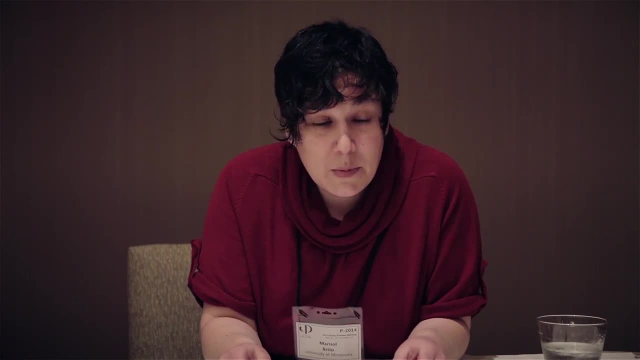 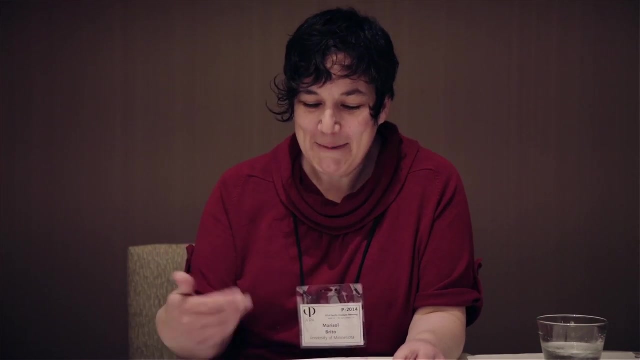 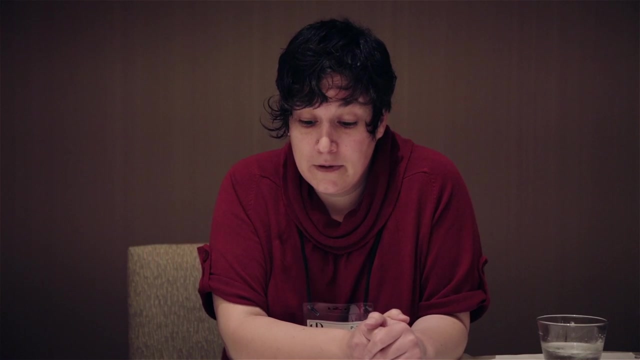 tantrums, tautologies, love and agency is in part, taken from one of my son's first jokes, Or at least one of the jokes that I actually understood was intended to be a joke. At around two years old, my son, Emilio- he goes by Leo- said he had a joke for me and proclaimed: 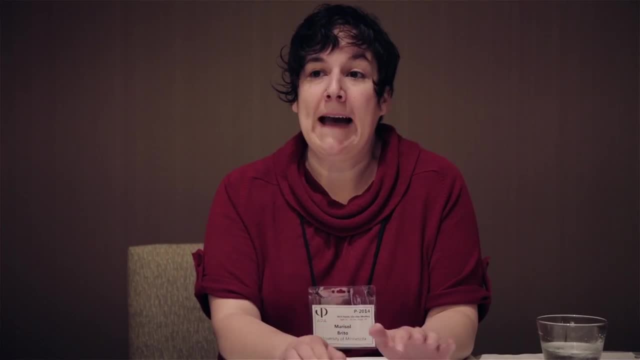 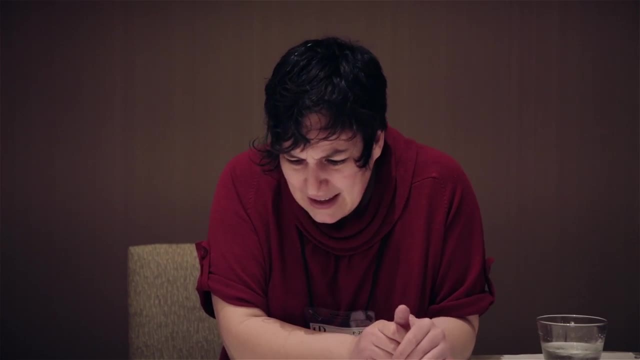 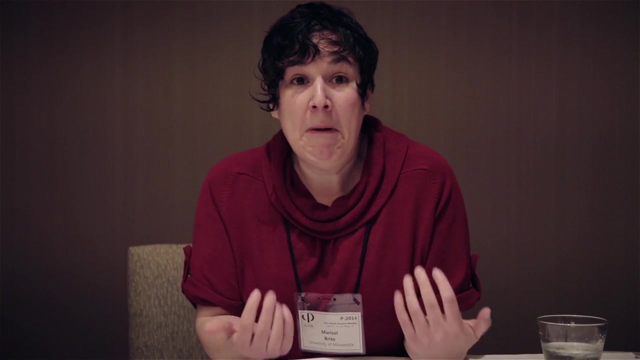 batteries are batteries and proceeded to laugh hysterically. It turned out it wasn't just batteries. Any tautology could be hilarious: Elephants are batteries, Elephants are batteries. Elephants, Books are books. Your mom is your mom. Tautologies are tautologies. It's all funny. 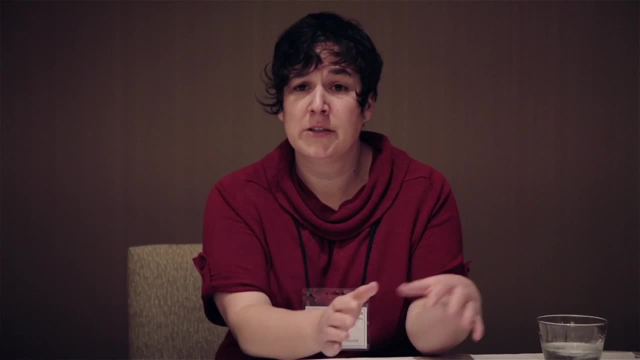 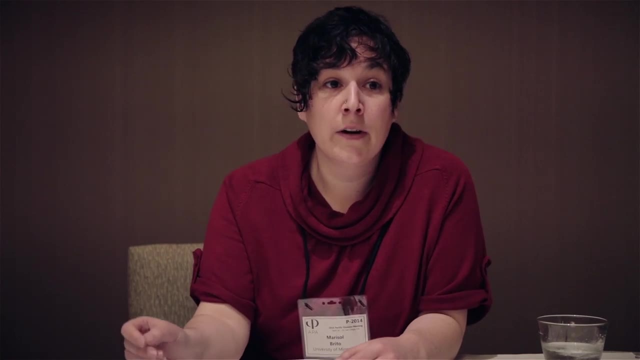 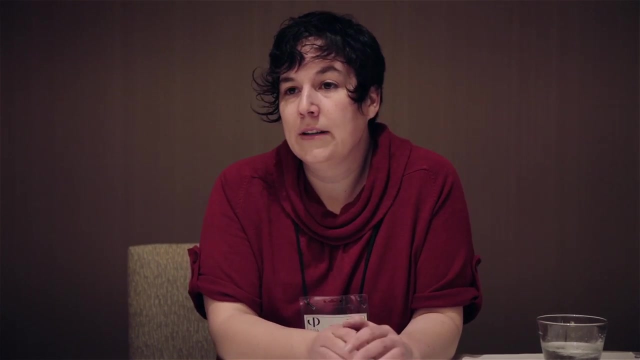 And then one morning, while getting ready, respectively, for small people school and big people school, I set down a bowl of blueberries in front of Leo. And it was winter and we're in Minnesota and blueberries are expensive, right, And I knew Leo loved blueberries, so I'd gotten. them as a special treat. And he looked at me and I said: I'm going to get you some blueberries. And he looked at me and I said: I'm going to get you some blueberries. And he looked at me and I said: 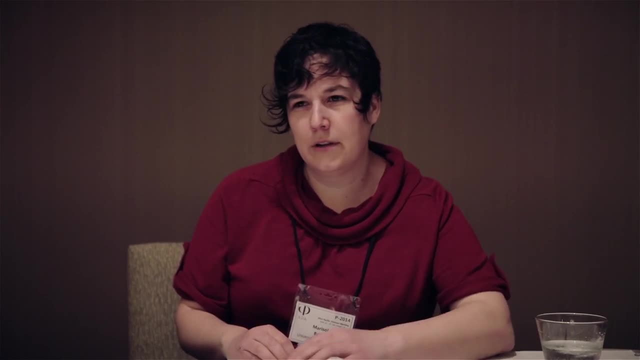 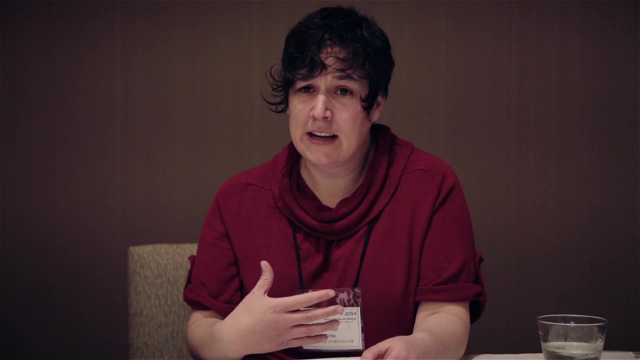 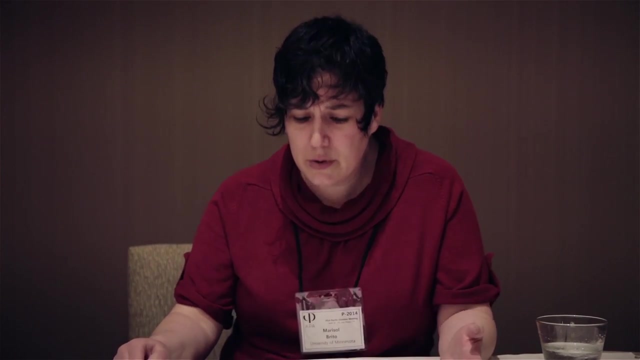 put the blueberries for a minute and then disdainfully pushed the bowl away without saying a word. In retrospect, this was probably not the best reaction that I could have had, But I said: you don't want blueberries, but you love blueberries. At this point things escalated And 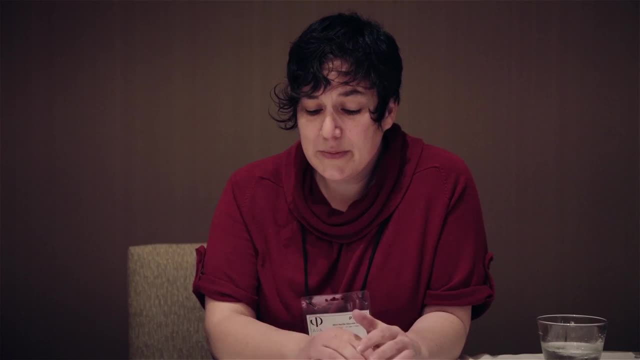 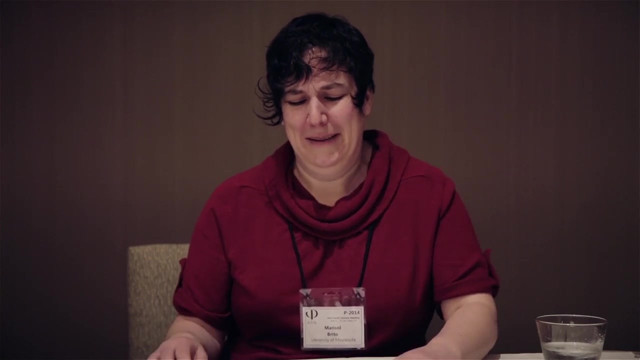 soon. Leo, who wasn't prone to tantrums, was so upset he'd fallen out of his chair and was on the floor screaming: my blueberries are blue, Blueberries are blue. So he's screaming and he's on the floor. 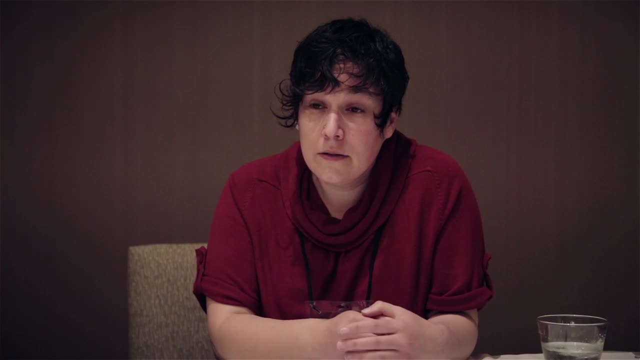 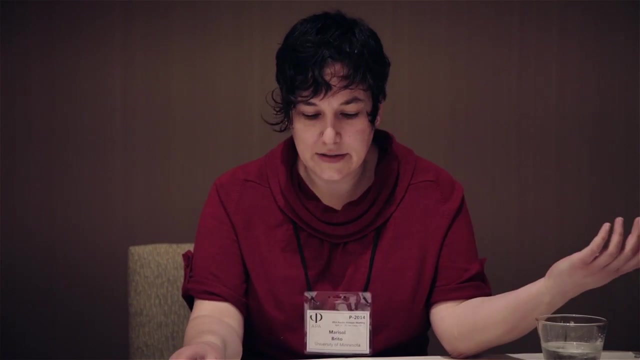 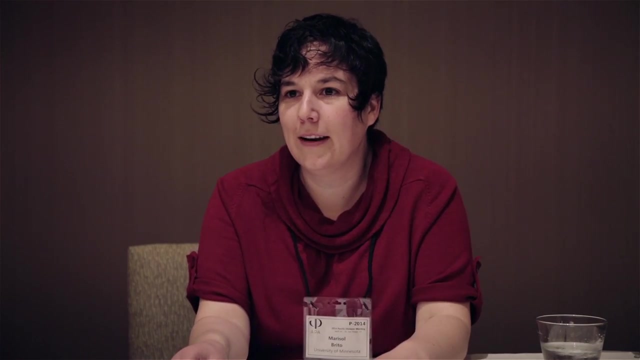 And we're going to be late for what? in my view, standing there looking down at him amounts to little more than a tautology, Which remember was hilarious just last week. So and I'm frustrated and I'm thinking, what if I tell him they're purple? I mean, I don't even know what to do here. 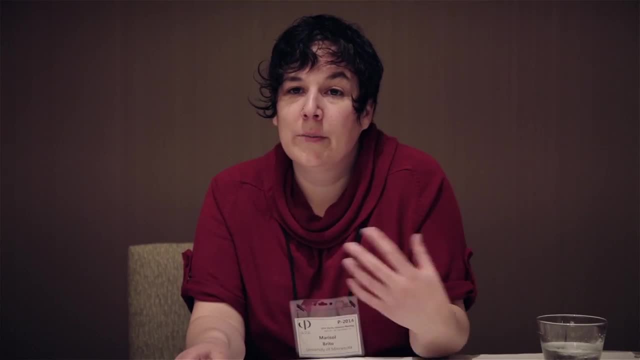 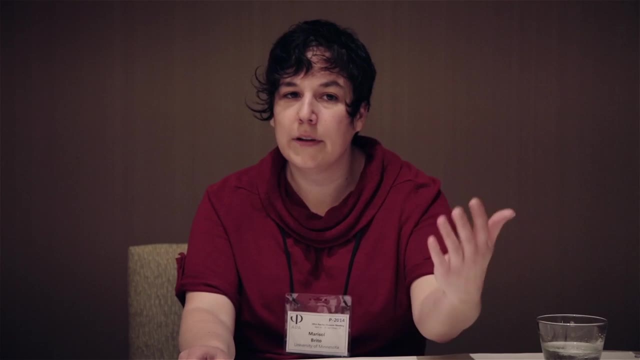 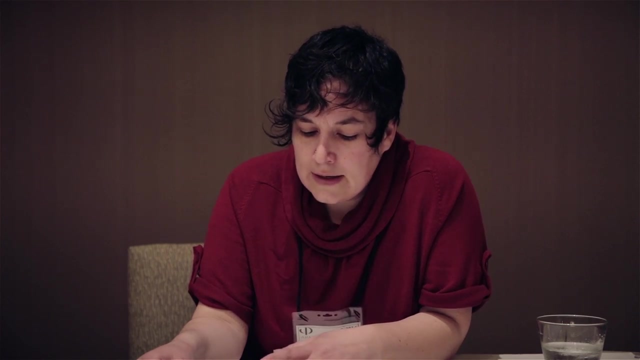 So I want to transition away from that story, but if you can keep it in your mind. And I wanted to move to a quote from Charles Payne. All of the things I'll quote are on the handout. If that's useful to you, feel free to look. He's writing in this passage about the organizing tradition. 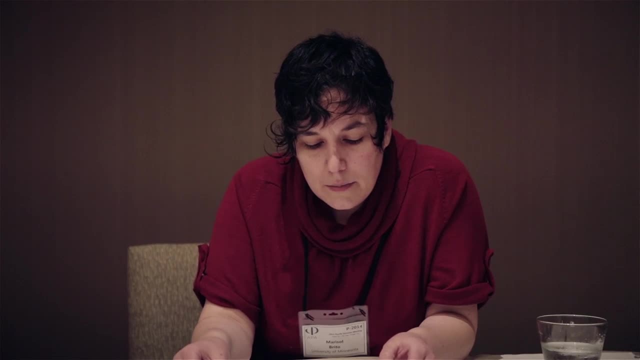 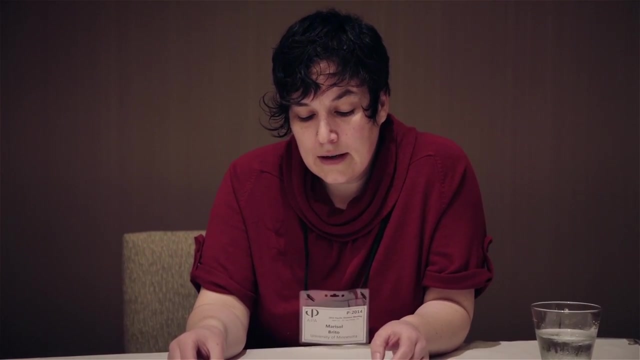 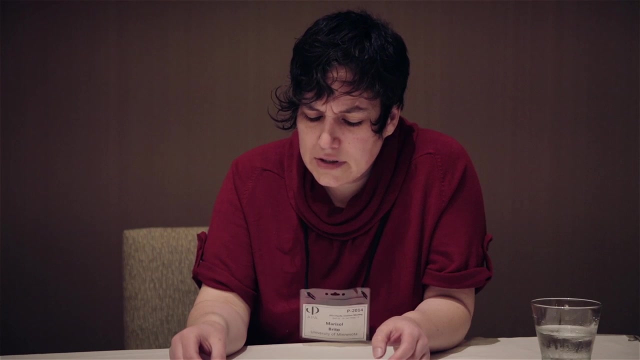 and the Mississippi freedom struggle. Part of the legacy of people like Ella Baker and Septima Clark is a faith that ordinary people who learn to believe in themselves are capable of extraordinary acts, Or better, of acts that seem extraordinary to us. precisely because we have such an impoverished sense of the capabilities of ordinary people, If we're surprised. 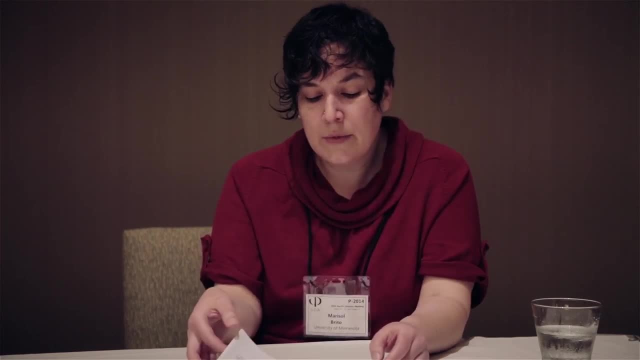 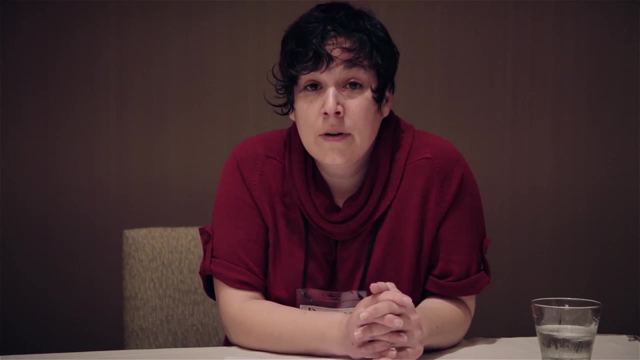 at what these people accomplished. our surprise may be a commentary on the angle of vision from which we view them. So I bring up Payne's work because I want to borrow two major points: First, that we have an ability to have an impoverished sense of the world, And that we have an ability to 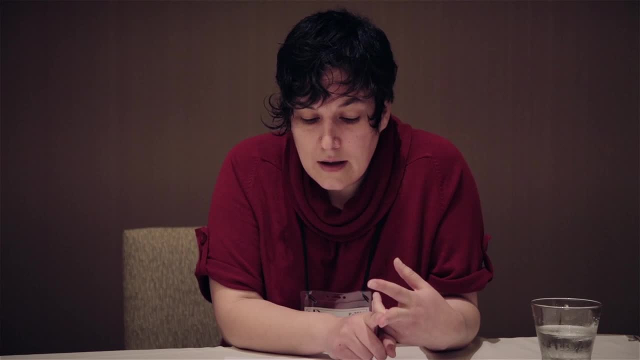 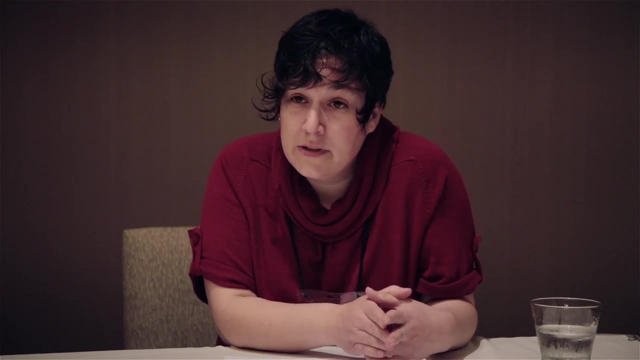 have anicy sense of the capabilities of others And second how the angle from which we view a person can impair our ability to see them. I believe these points are particularly salient in our relationships with children. We can recall the things I just reported. 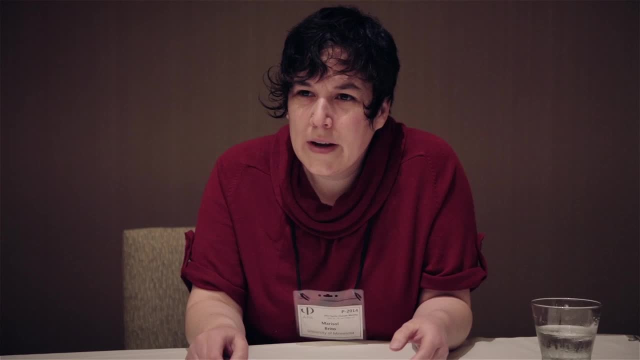 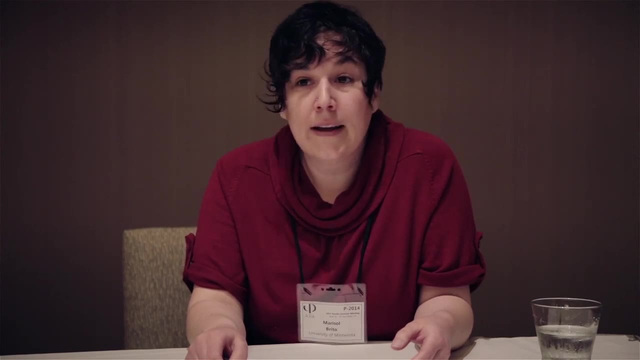 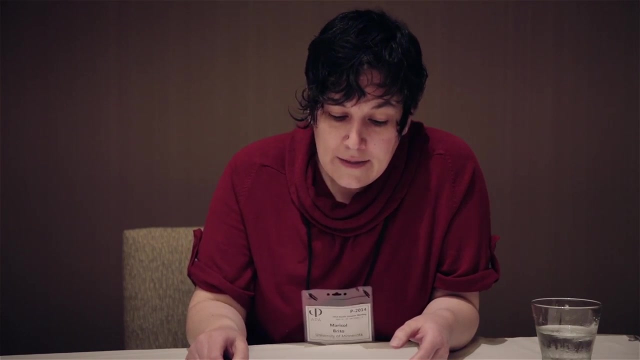 saying to my own son: You don't want blueberries, but you love blueberries. I know what you want. I know what you like better than you do. You are not as capable as I am of knowing things, And there I was literally looking down on him. you know thinking. 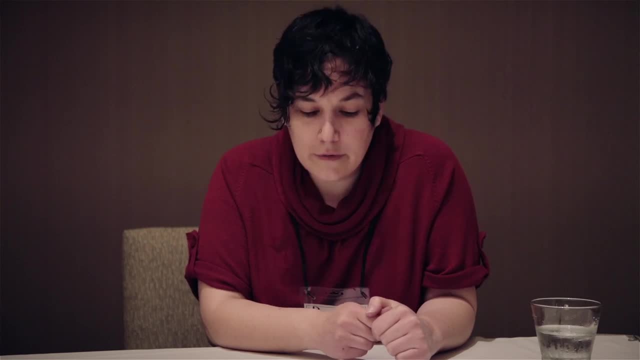 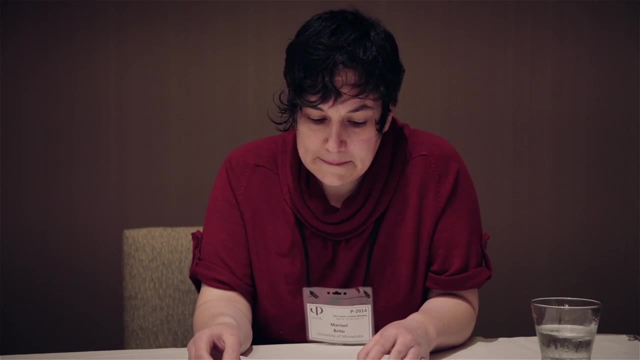 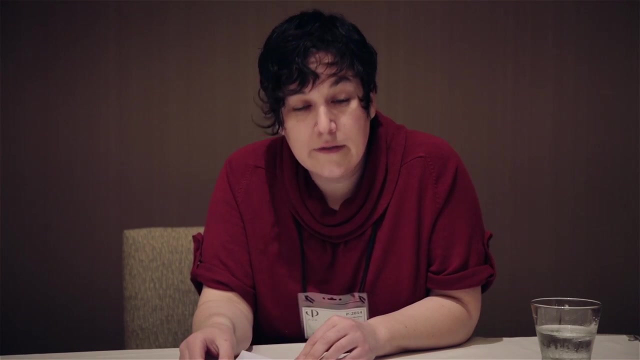 this is ridiculous. He's being ridiculous. He's upset over nothing. We discount children. We don't believe in their capabilities, We don't see them clearly In their article. Have We Got a Theory for You? Lugones and Spellman talk about the challenge of exchange. 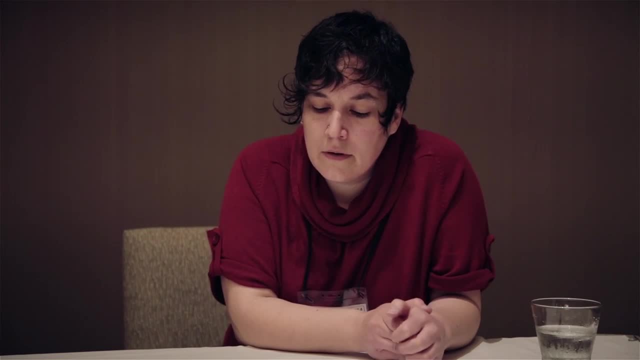 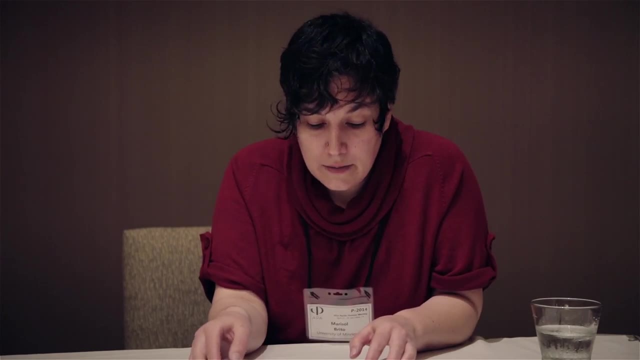 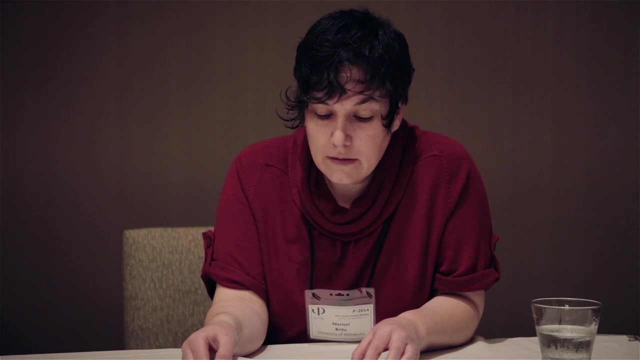 engaging with the language and culture of power. when your own language and culture are marginalized and excluded from the culture of power, We, the minorities, and you, the dominant, do not talk the same language. When we talk to you, we use your language, the. 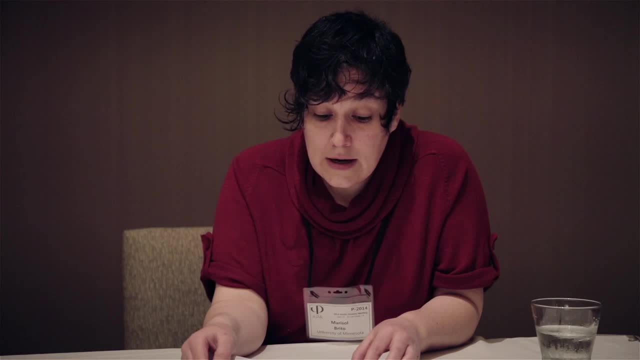 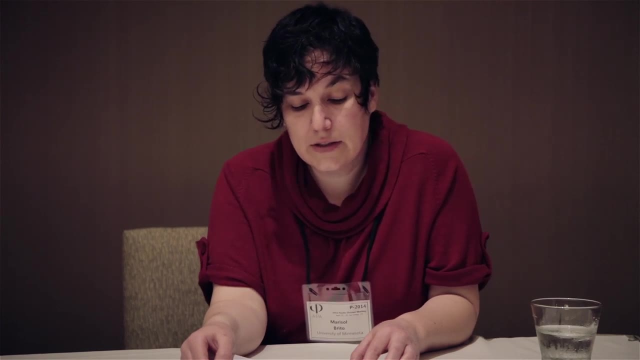 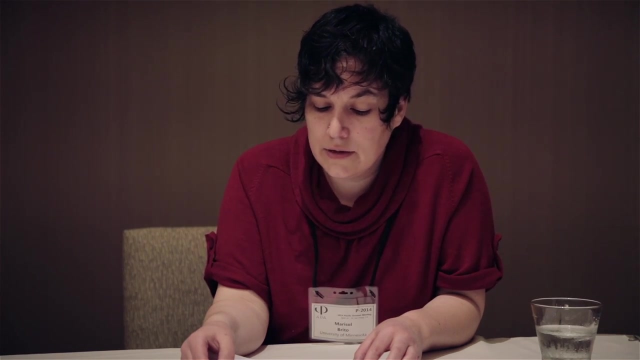 language, of your experience and of your theories. We try to use it to communicate our world of experience. But since your language and your theories are inadequate in expressing our experiences, we try to use it to communicate our world of experience. We only succeed in communicating our experience of exclusion. We cannot talk to you in our 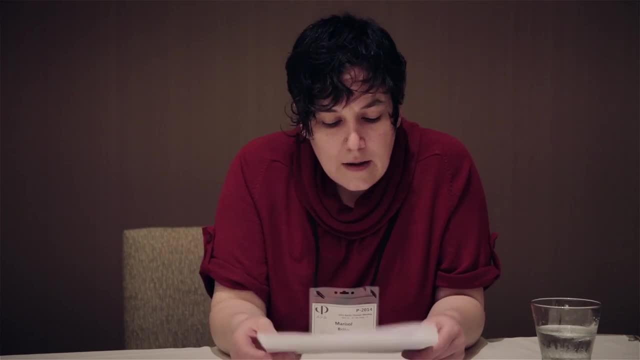 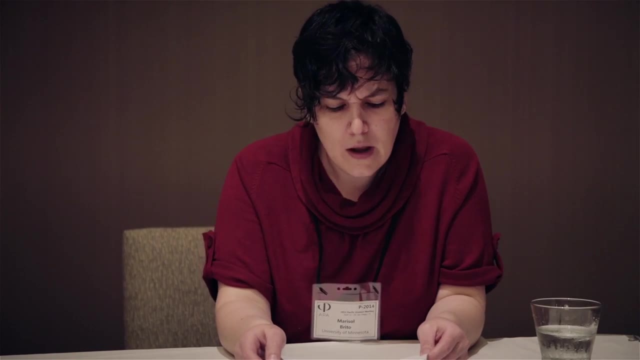 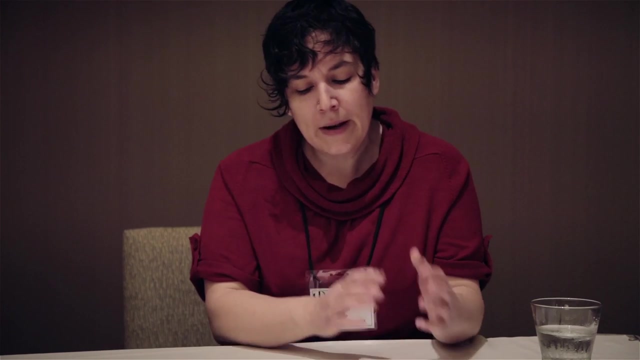 language because you do not understand it. If my son had taken up the language and culture of power and said something like you know, mom, I do often appreciate blueberries and I know it's a privilege to have them and thank you so much for getting them, but I'm 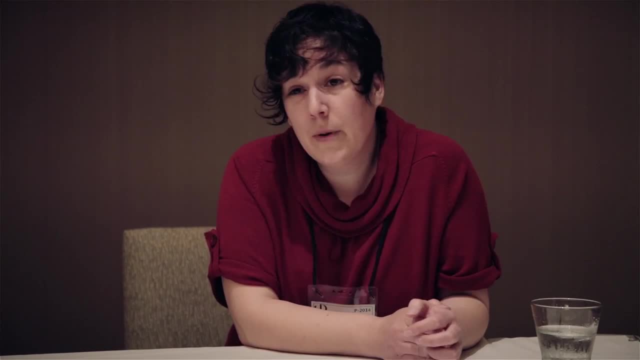 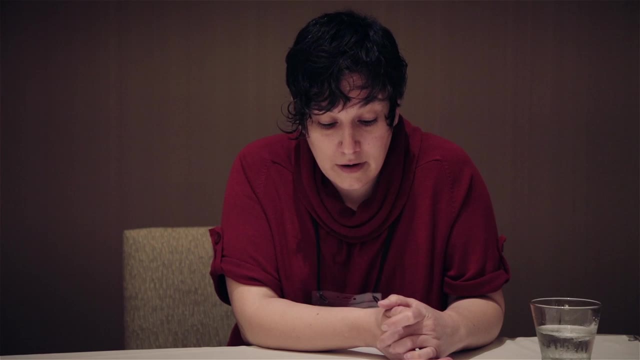 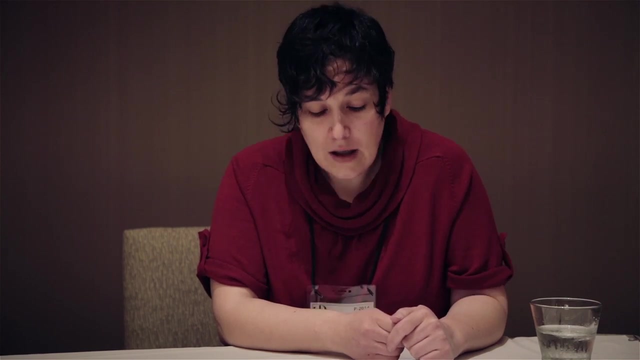 really not feeling like eating blueberries this morning, I probably would have had a different reaction. Or if an adult friend, someone I wasn't already looking down on, had said, blueberries, oh thanks, but not right now, I wouldn't have demanded an explanation. I certainly wouldn't. 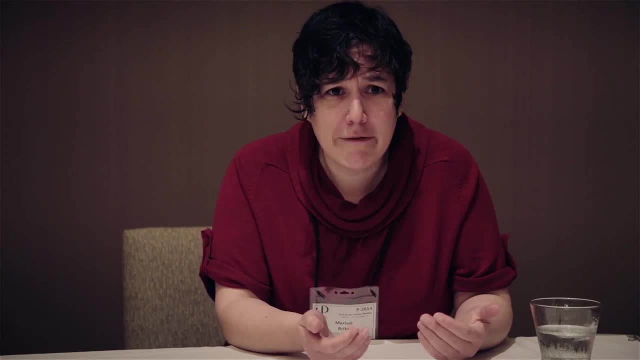 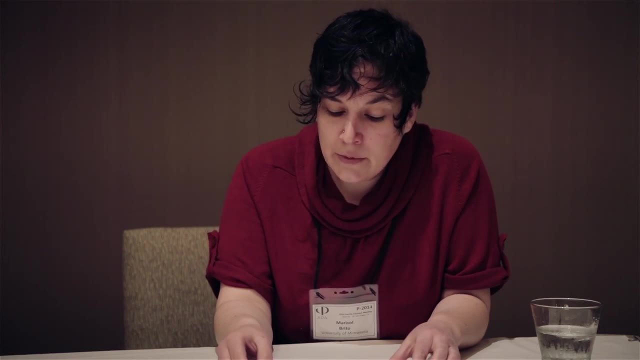 have said: but, adult friend, you love blueberries. And the truth of the matter is it didn't even occur to me that Leo genuinely could not want blueberries because they are blue. That doesn't fit into my understanding of the world. 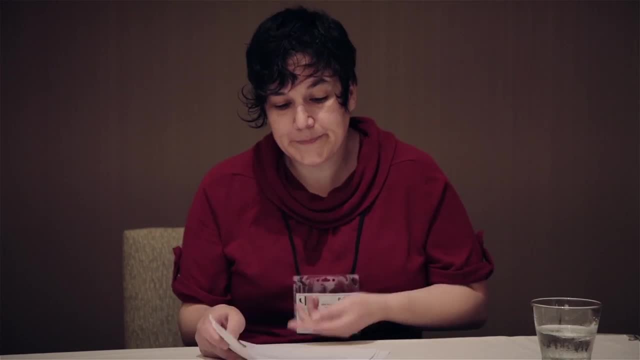 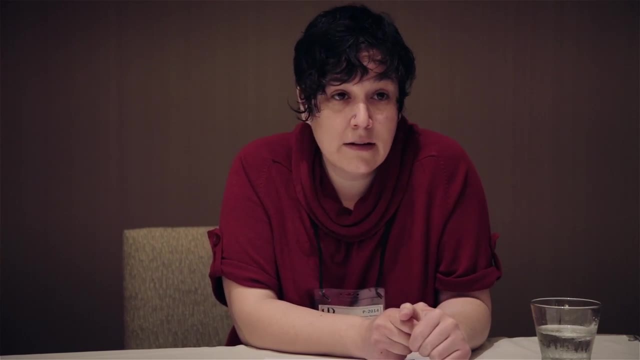 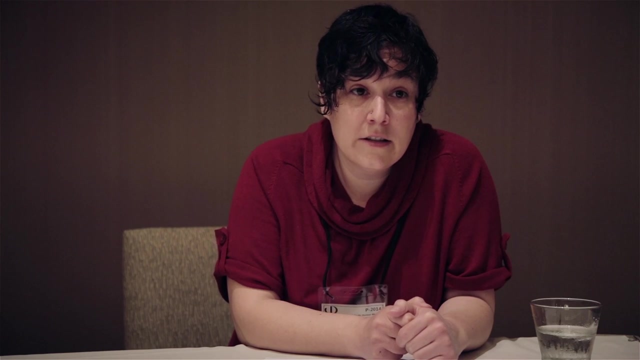 Tautologies are not things to get upset about. He was not speaking my language and he was not speaking to my experiences and my theories, so I discounted him. I have an understanding, a narrow understanding, of what it means to make sense in the world, to be intelligent. 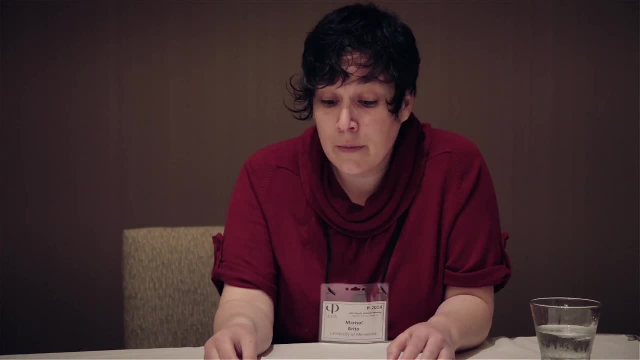 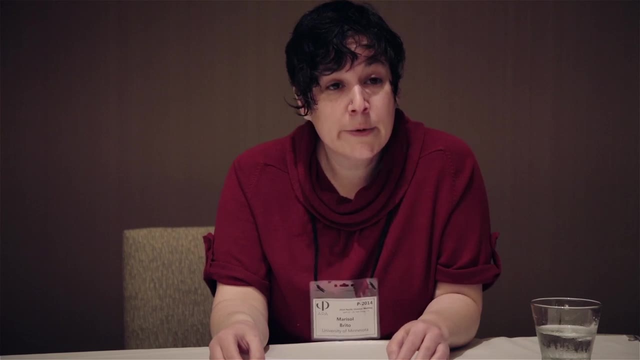 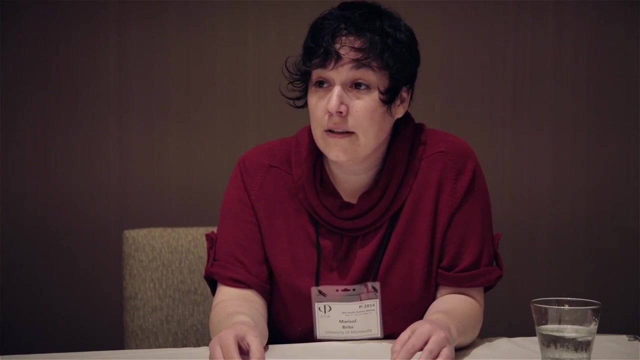 to contribute and in that moment at least, I wrote him off. But, as pain warned us, we don't only write people off when they don't fit our mold. Sometimes we write them off when they do. We can see their actions as extraordinary, at least in part because we expect so little. 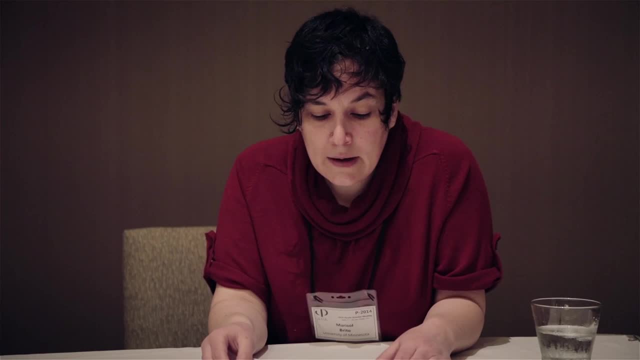 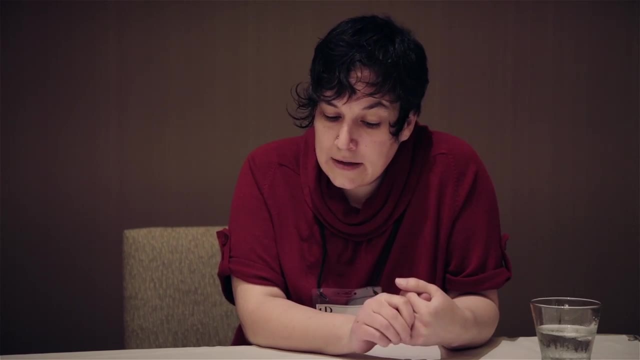 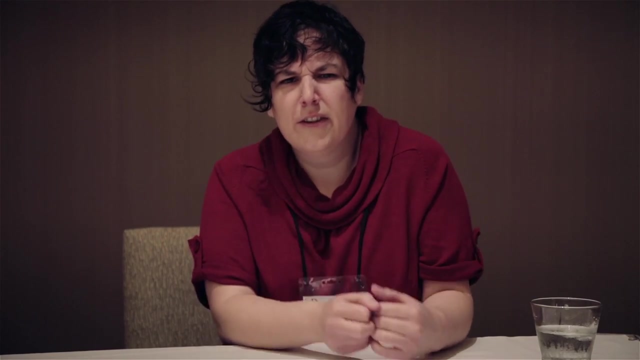 of them, Leo and I, were riding in the car when he was not quite two and the song Pumped Up Kicks was popular at the time and he was playing on the radio as we pulled up to a stop sign. He had been quiet, you know, during the drive, but suddenly he leaned as far forward as he. 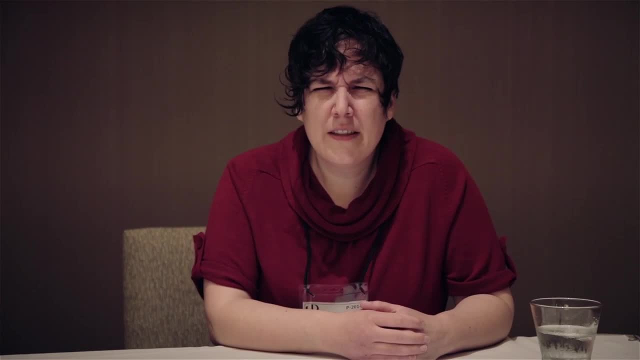 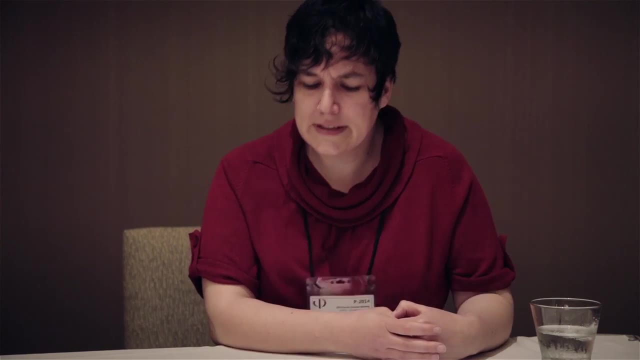 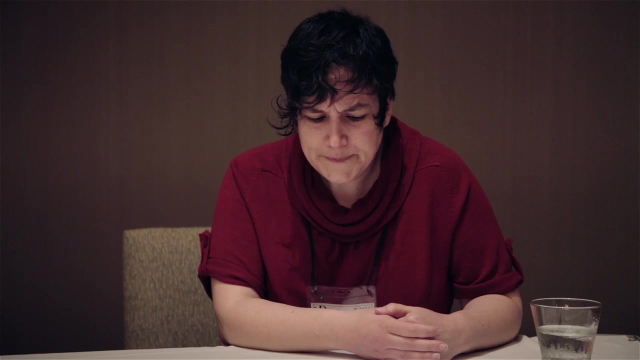 could, in his car seat and said: Mama, I think I prefer the acoustic version. A few days later we're sitting on the floor coloring and stamping and he looks up and says: what is art? And these things make us pause and we're amazed and amused. but they also reveal what 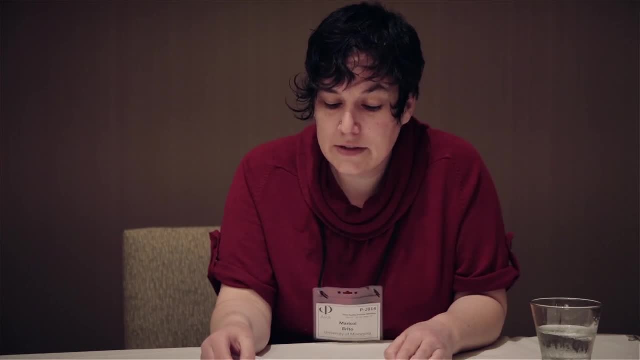 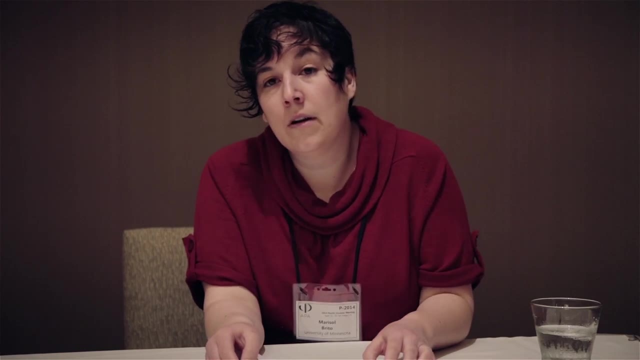 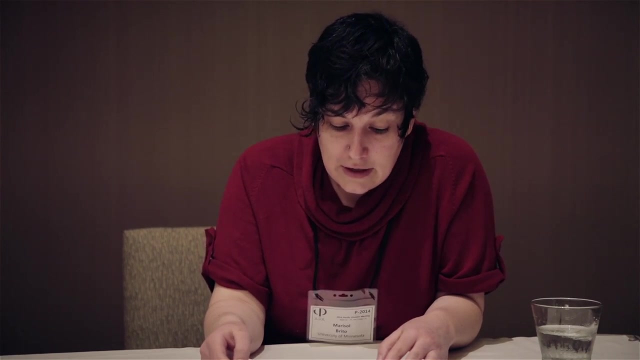 we expect and what we value. We don't expect children to engage in ways that we find meaningful, and we value them when they engage in ways that seem to map onto our ways of making meaning. Morelone makes a similar point in a section on respect in her work The Philosophical Child. 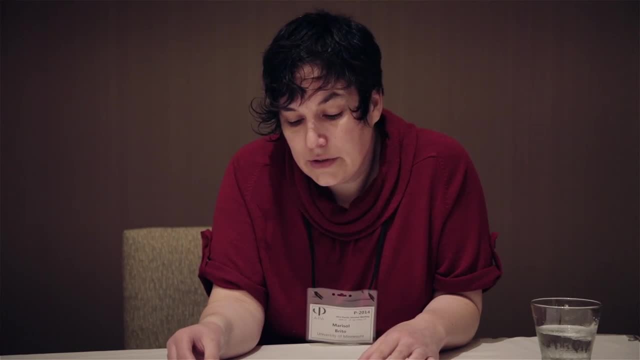 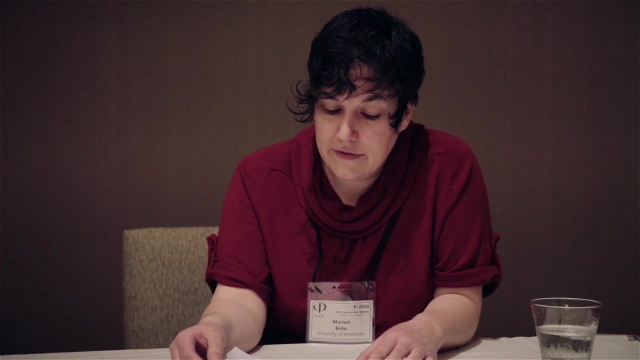 She writes. Too often we approach serious issues with children with too much assurance that we know what's best for them and too little confidence that they possess the potential for figuring things out for themselves. Advancing respect for children's ideas is not a priority in our society, or in most. 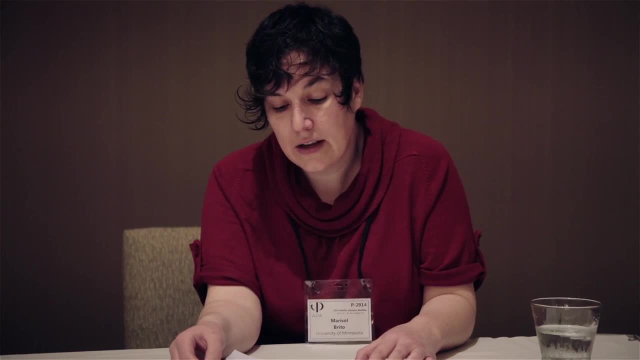 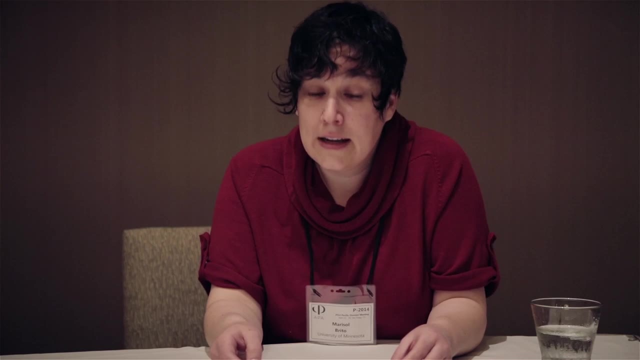 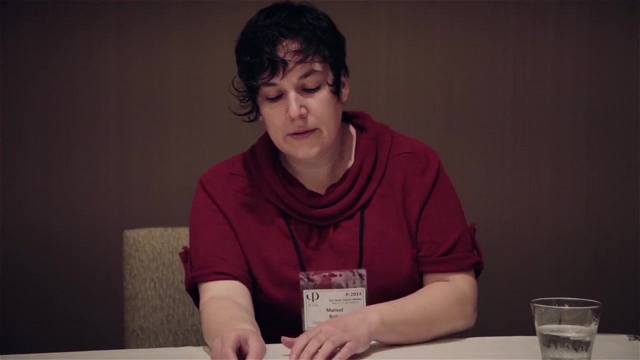 families. Children are typically patronized at best when they propose serious ideas about difficult subjects. What these dismissive and patronizing attitudes call out is a prevalent and insidious ageism in our society. At this point I want to take a minute to examine a graphic on recapitulation theory. 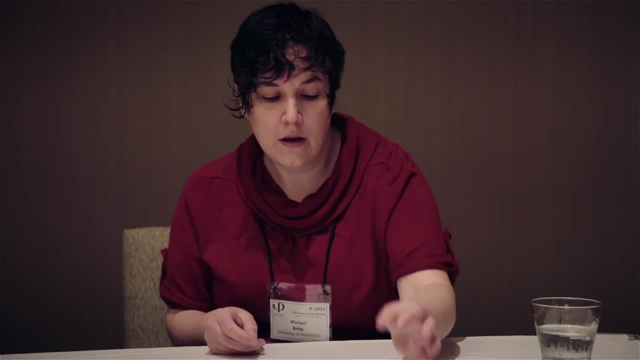 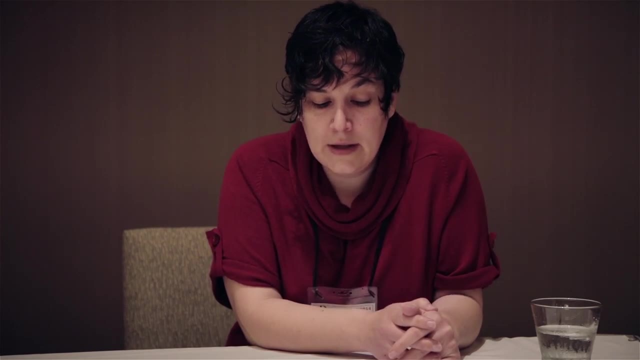 and this is in your handout. In brief, recapitulation theory sets up parallels between stages of individual human development and stages of societal development. We now hope- I certainly hope- that we may be able to achieve the same goals that we have achieved in our society. 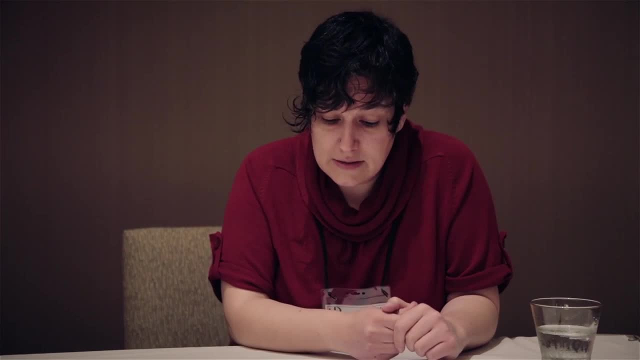 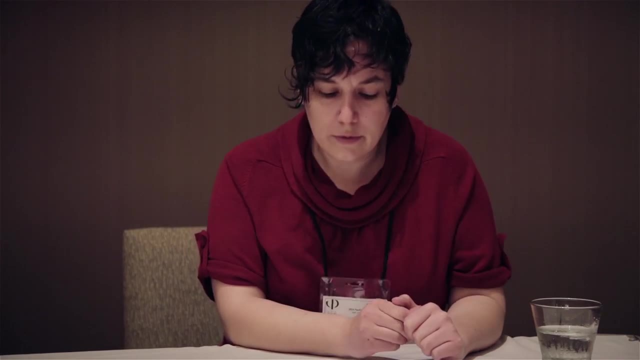 When we look at the right side of the diagram, it gives us pause. We have a sense that we are not at our best when we think of, as is quoted on the diagram, tribal groups as lesser than or less developed than, say, the Western medieval period. 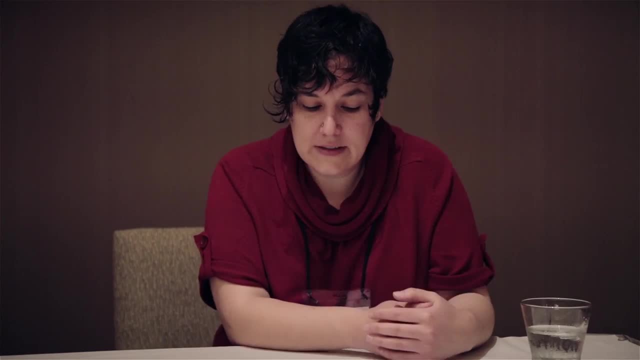 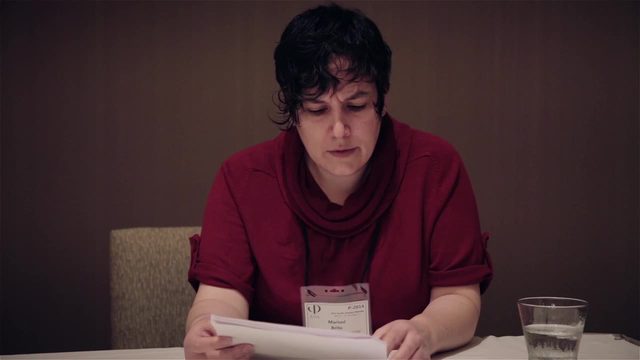 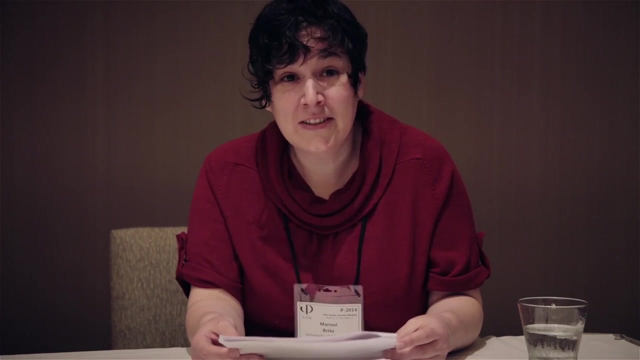 Or anything really. But what about the left side of the pyramid? Shouldn't that also give us pause? Is a 40- to 50-year-old white man on his way to work, the pinnacle of individual humanism. He is almost certainly a representative of the dominant language and culture of power. 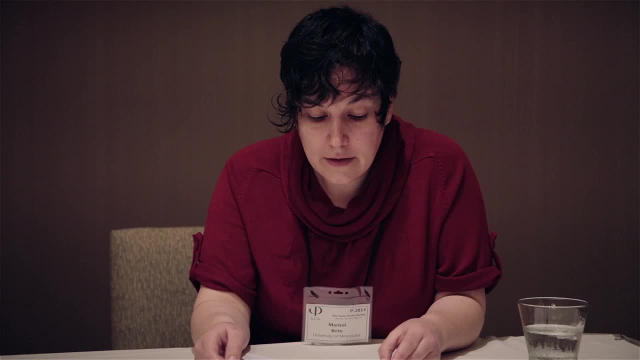 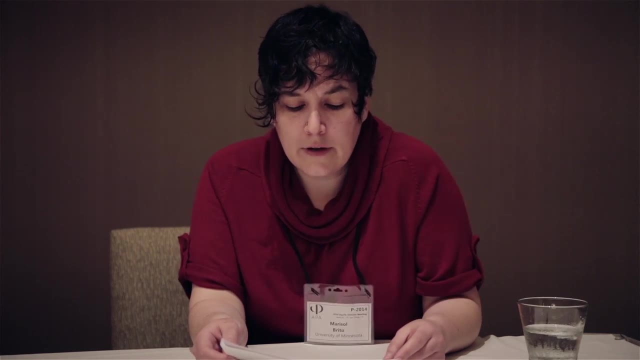 But do we really want to hold him as more than better than the others on the chart and those who are completely absent from the chart? Who can we learn from? Who do we want to learn from And who do we most need to learn from? 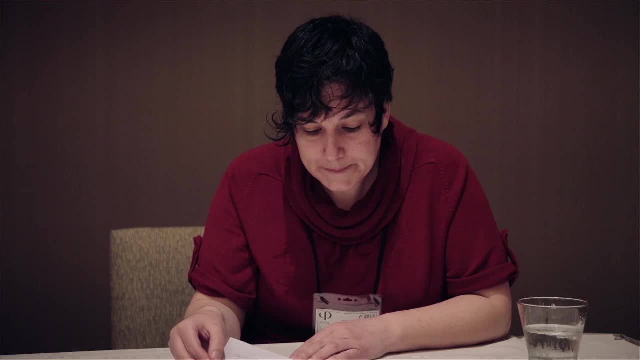 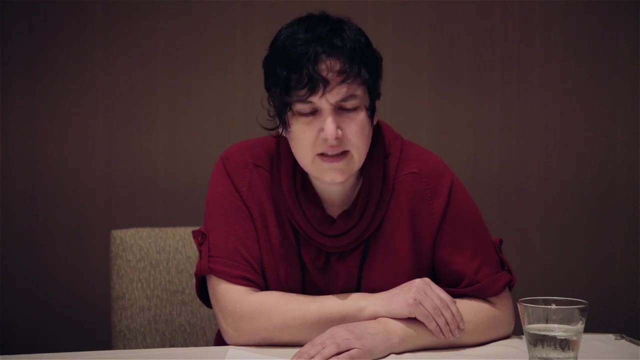 Here I have a story from a friend and her daughter, Zella. Early on with Zella, we started noticing that she would, like most kids, often, seek out triggers, things to get her crying, And she'd get angry if we tried to comfort her too much. 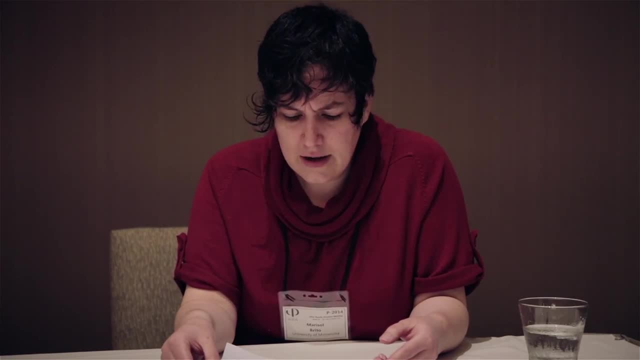 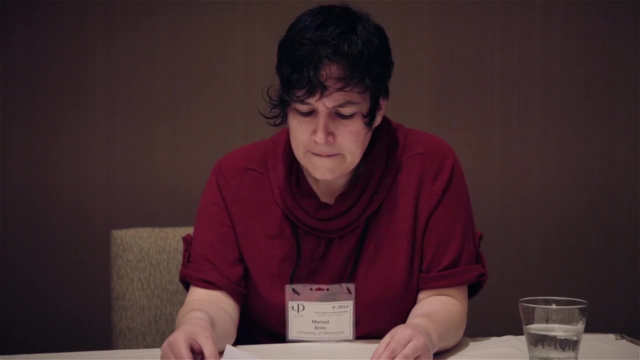 We started asking her: Do you want to just cry? And a lot of times she'd say yes. Now she articulates herself: I just want to cry, Which is great, but it seems that my three-year-old has a much healthier emotional state than me. 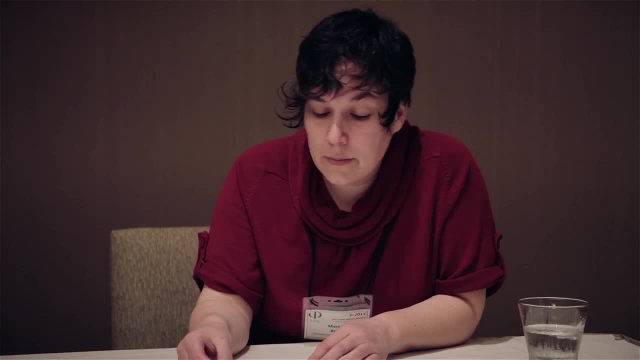 This story states. I'm not sure if it's true, but I think it stands out to me because I see it as one example among many examples of a way in which children seem to have a great deal to offer adults. As adults, we've learned and been molded by languages and cultures of power. 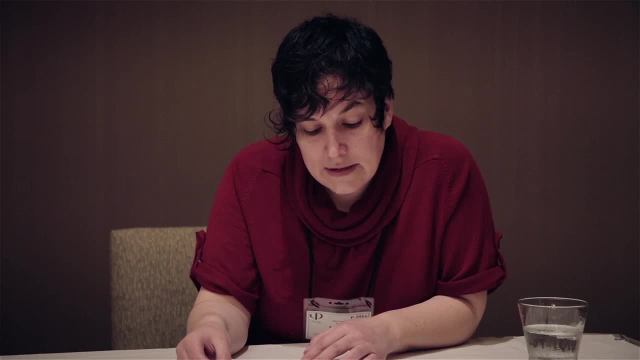 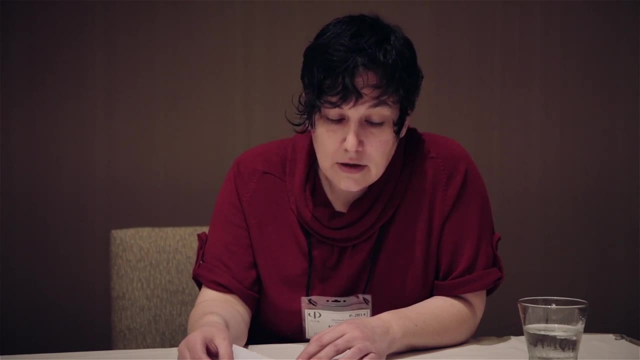 We have a particular set of strengths and scope of being. Children can offer not a lesser, but a different, many different ways of being in the world. Interactions with children are in many ways cross-cultural interactions. At least they have the possibility to be. 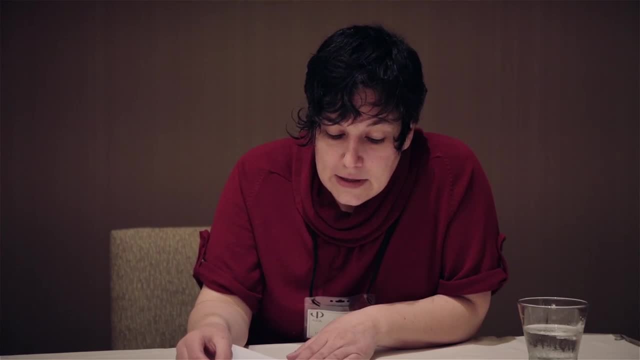 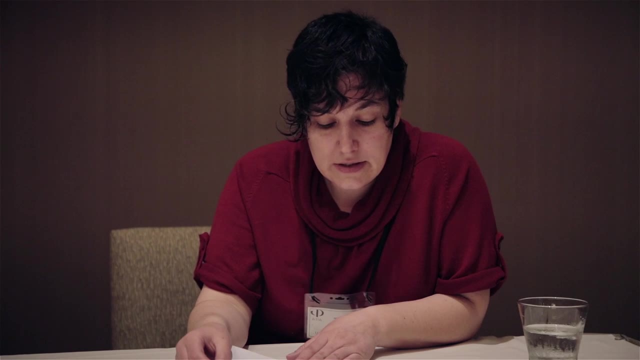 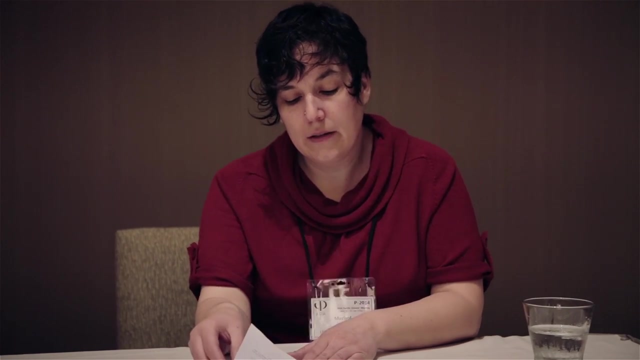 If not, then why? If we are open to them? The Reggio Emilia approach to early childhood education holds that children are citizens now, not future citizens. One of the pedagogues behind the approach, Malaguzzi, wrote a poem that speaks to the many ways of being that children may be able to engage with that are often lost to adults. 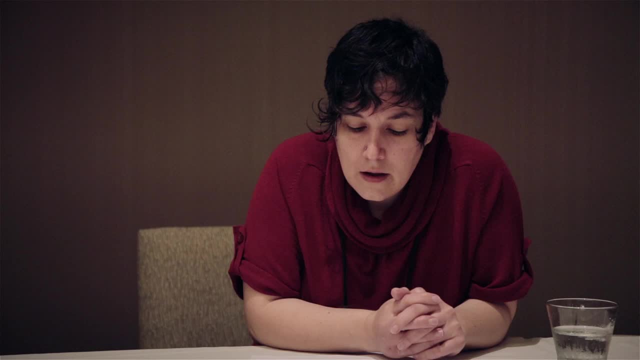 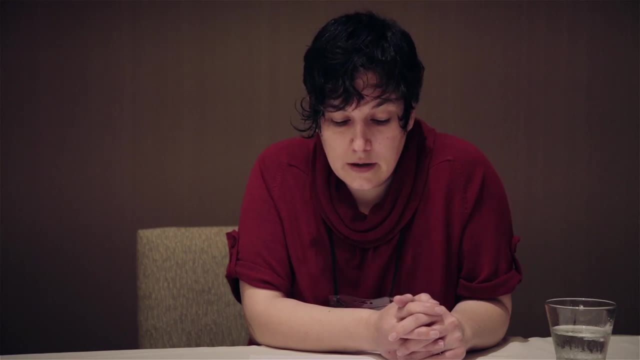 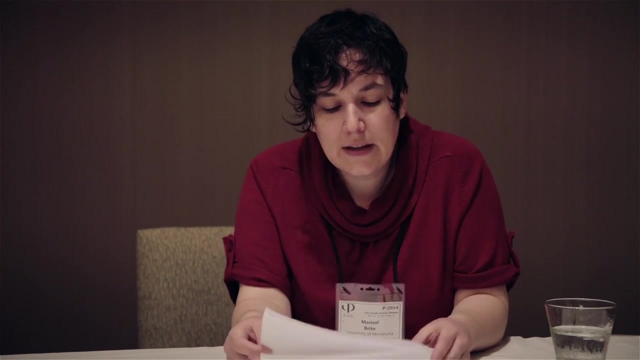 This is from the Hundred Languages of Children. It's called No Way. the Hundred is There. The child is made of one hundred. The child has a hundred languages, a hundred hands, a hundred thoughts, a hundred ways of thinking, of playing, of speaking. 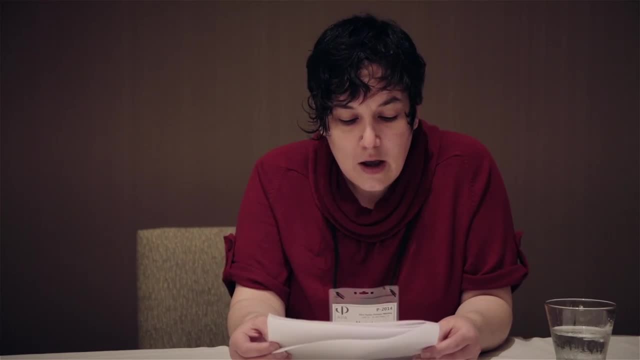 A hundred, always a hundred ways of listening, of marveling, of loving. a hundred joys For singing and understanding. a hundred worlds to discover a hundred worlds, to invent a hundred worlds to dream. The child has a hundred languages. 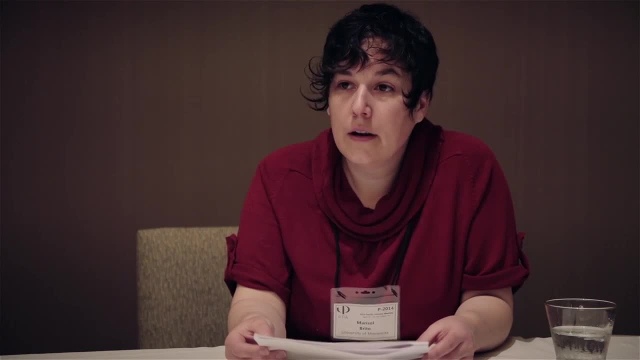 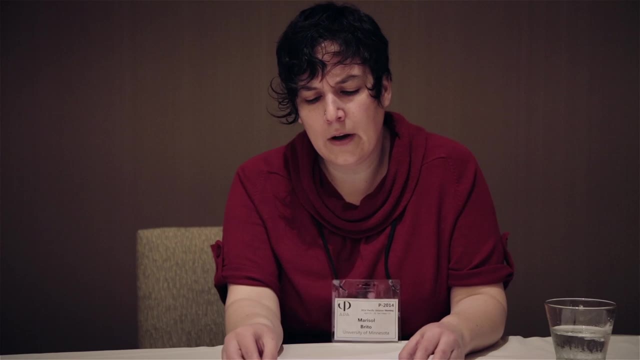 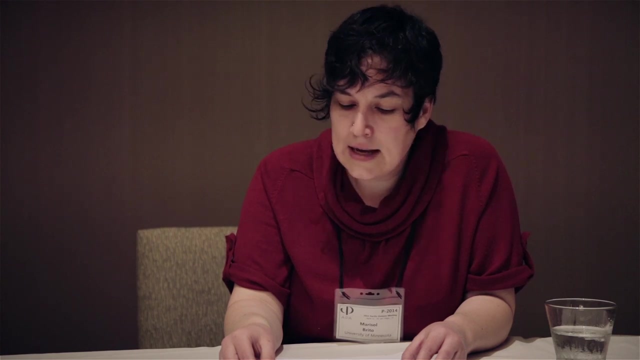 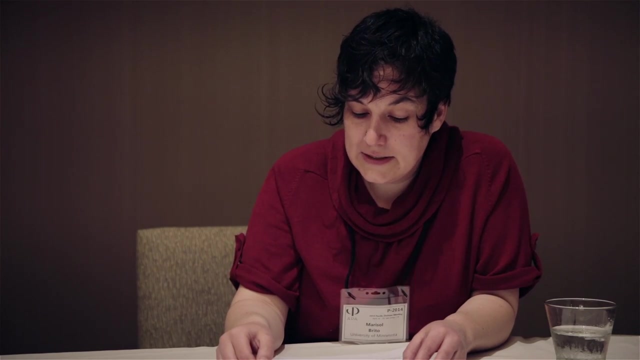 And a hundred hundred, hundred more, But they steal ninety-nine. The school and the culture separate the head from the body. They tell the child to think without hands, to do without head, to listen and not speak, to understand without joy, to love and to marvel only at Easter and at Christmas. 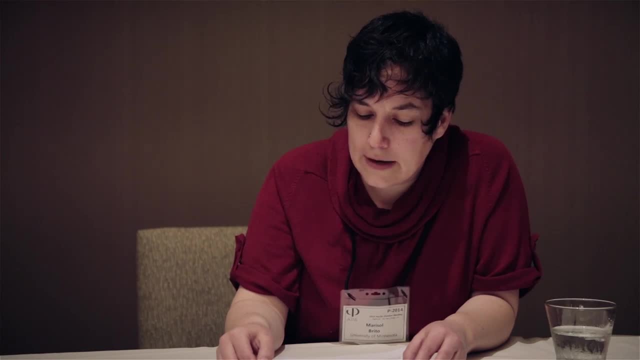 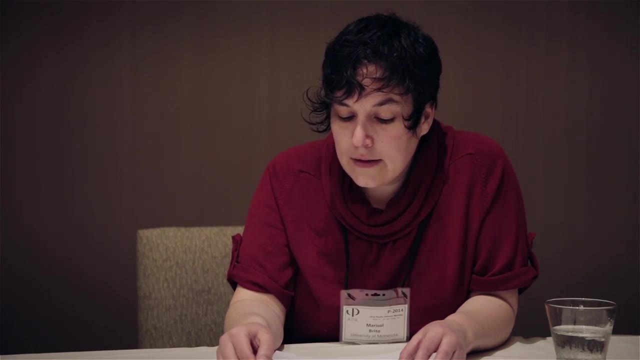 They tell the child to discover the world already there And of the hundred they steal ninety-nine. They tell the child that work and play, reality and fantasy, science and imagination, sky and earth, reason and dream are things that do not belong together. 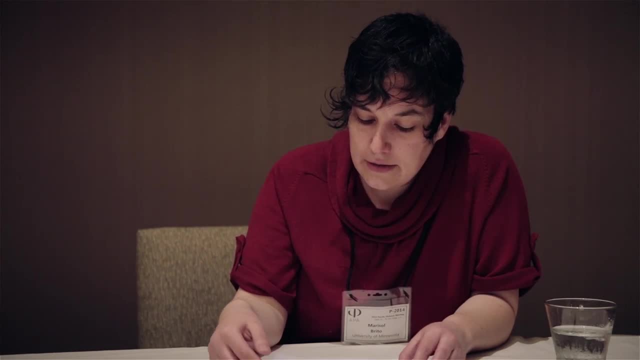 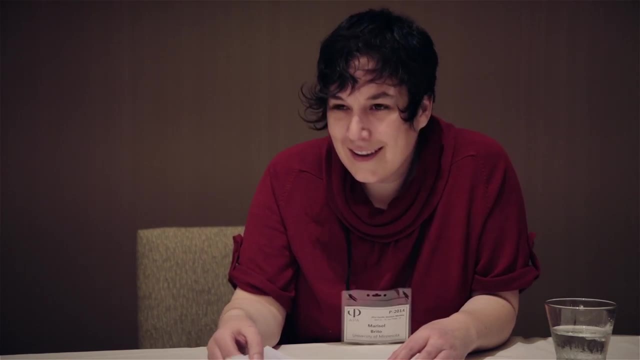 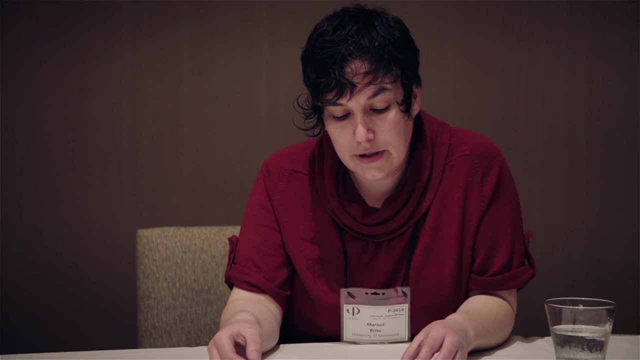 And thus they tell the child that the hundred is not there. The child says: no way, the hundred is there. If ageism is a force that denies the hundred languages of children, favoring a narrowed language of culture and power, what is it that can combat ageism? 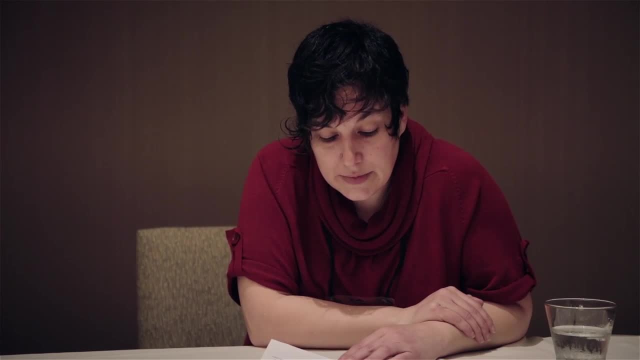 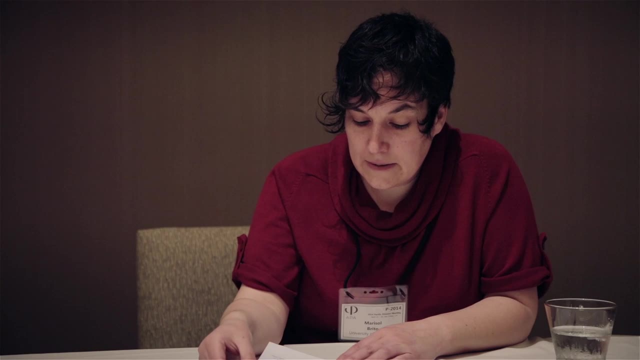 Pulling from my broader work on interpersonal relationships as a way that we grow, I believe that fostering friendships between adults and children is one way to challenge ageism. This is similar to the claim Lugones and Spellman mentioned earlier, make in their article. 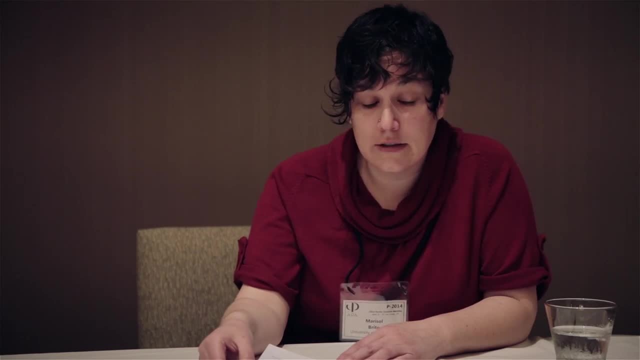 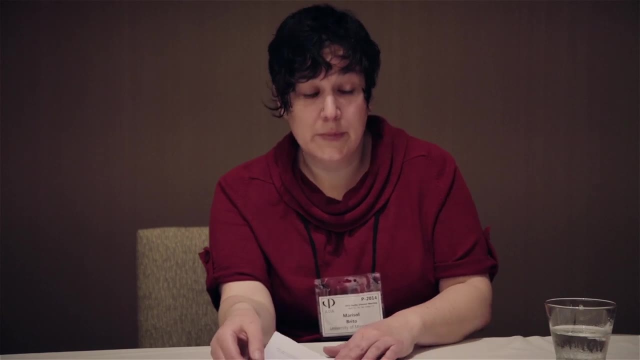 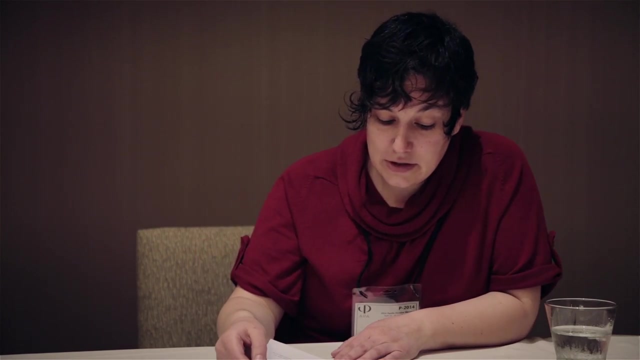 when they offer friendship as a meaningful way to connect and learn across difference. I will mention later that the many early childhood educators seem to have glimpsed or experienced this potential first hand, But for me, it's parenting that offers this position of epistemic privilege. 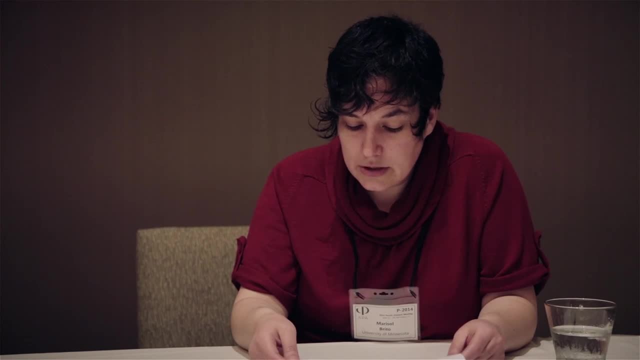 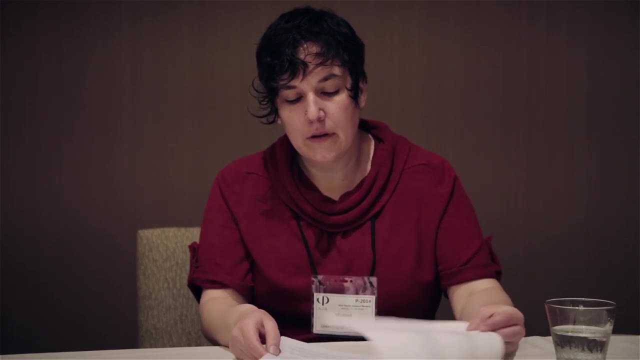 We often think colloquially that parenting is a privilege. Our children are so beautiful, so wonderful, and we can't imagine life without them. But I believe that's a very different model, And here I specifically do mean epistemic privilege. 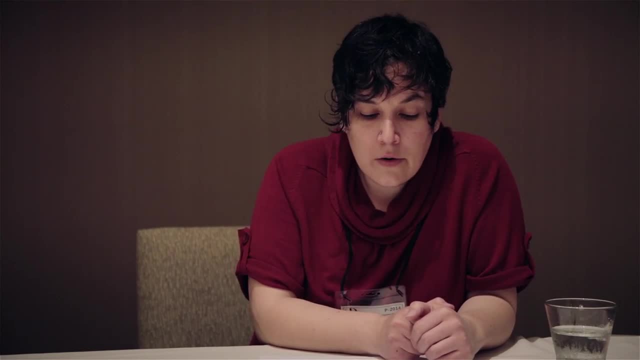 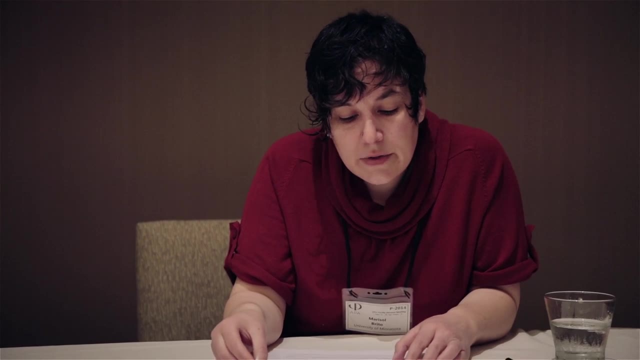 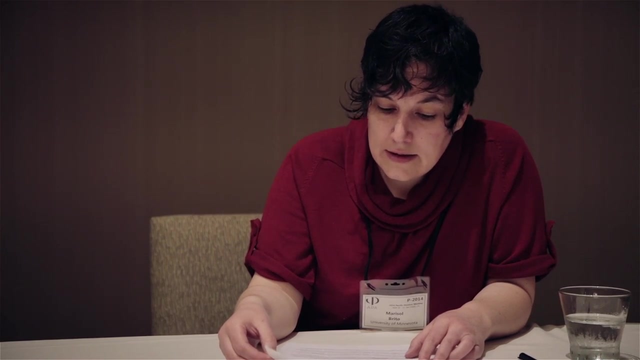 A chance to be in a position where one can learn and know and experience the world in ways unavailable or rarely available otherwise. A simplified explanation of how such privilege might work is illustrated on the handout. The general idea is that the intersection friendship provides. 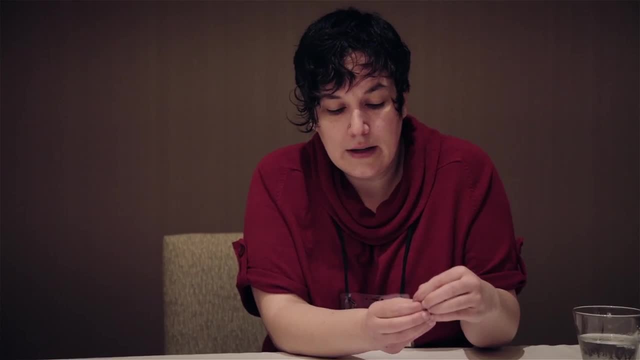 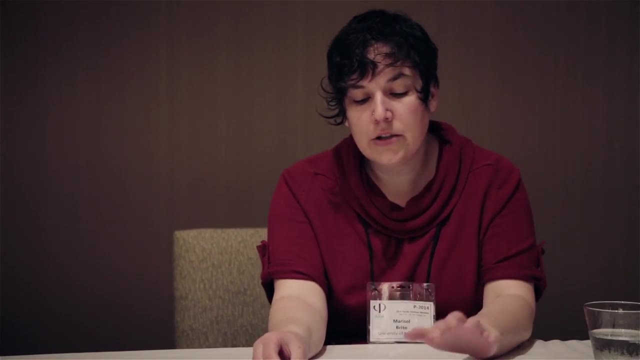 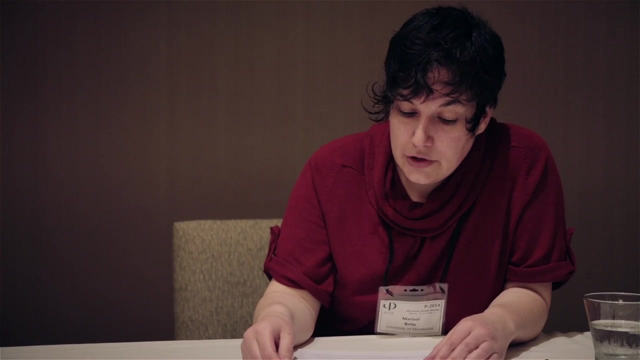 is an intersection where knowledge and care can interact and that, in turn, provides a space that can cultivate more richly formed thought and action than knowledge or care alone. To understand this, we might think of times that knowledge or care individually can fail us. 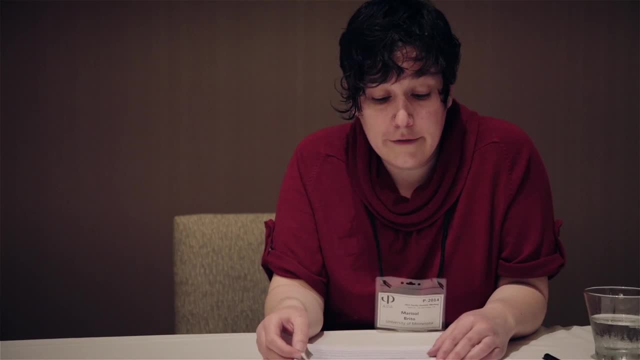 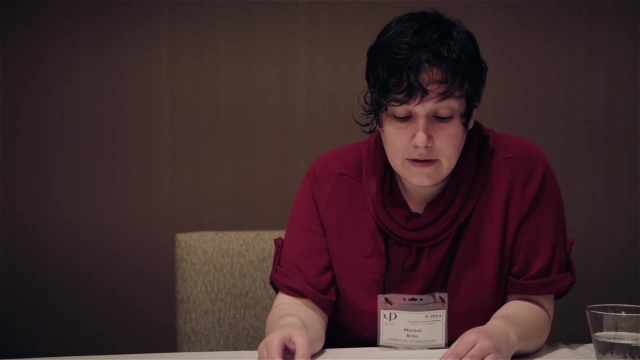 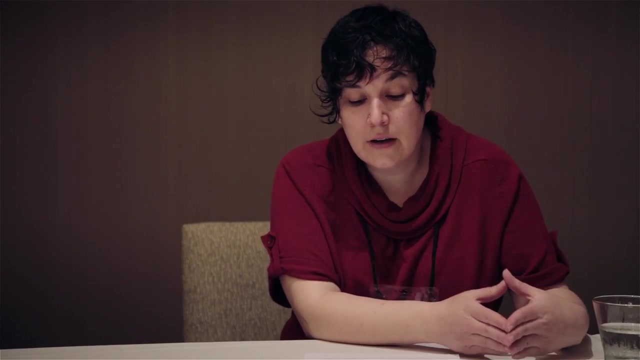 For example, one might know that many people in Africa have fewer resources but do nothing. Or one may be moved through care to send used clothing to Africa but lack the knowledge that such goods flood local markets and damage local economies. However, one can imagine that a more personal relationship with a person 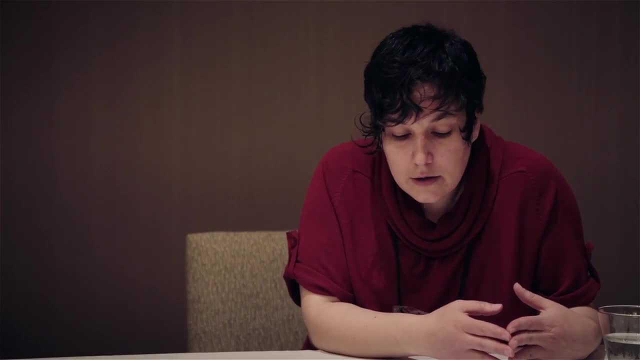 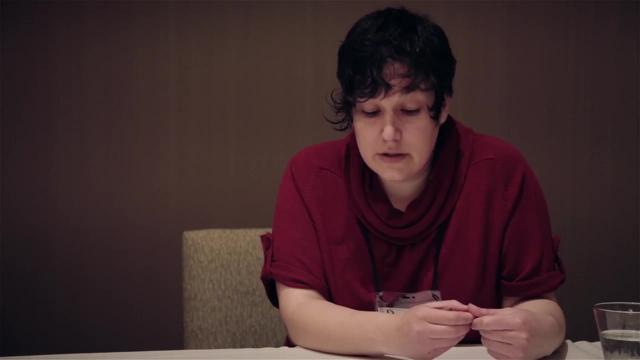 say from the Naroc district of Kenya, could cultivate not only an increased knowledge of the area and its needs, but also a sense of care that comes with a motivation to do something, maybe even to help educate other people to stop sending clothing to the Naroc district of Kenya. 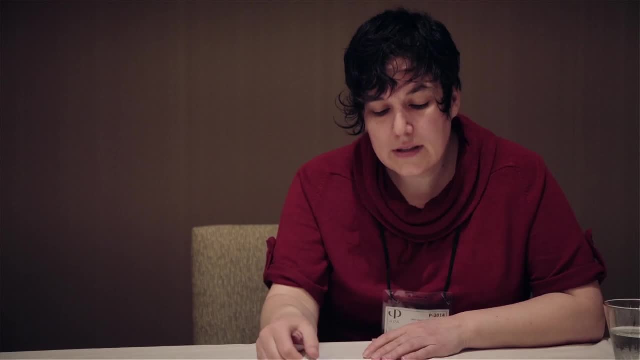 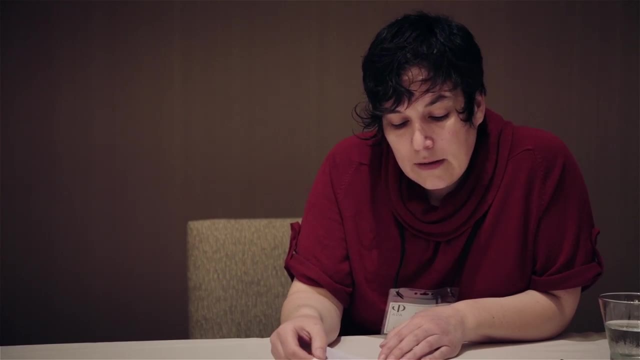 The possibilities, though, are endless. With this in mind, we might think of relationships across difference as a kind of radical act of resistance, one that allows us to move past the dominant narrative of who people are and what is needed in the world. 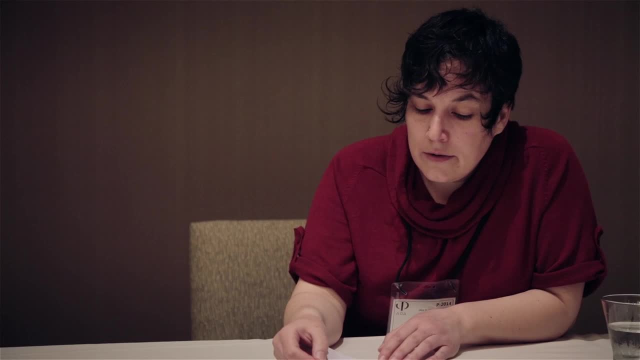 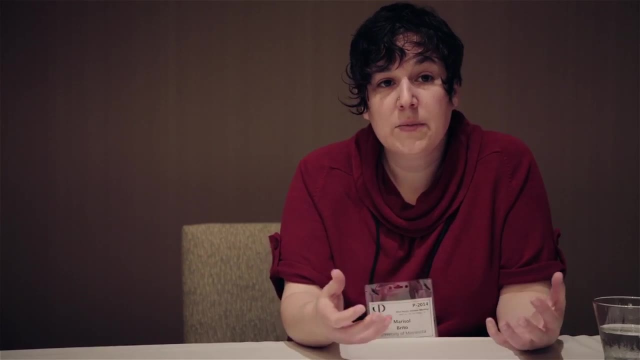 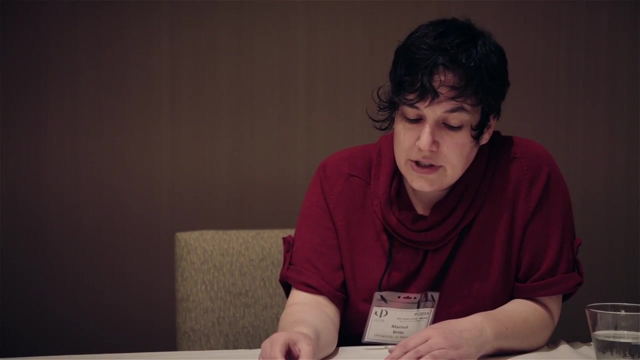 Returning to Ligonis, Spellman and the Hundred Languages, we can think of these relationships as making space for dialogue between languages or making space for other languages to be heard In this way. returning to the case at hand, we can think of friendships between adults and children. 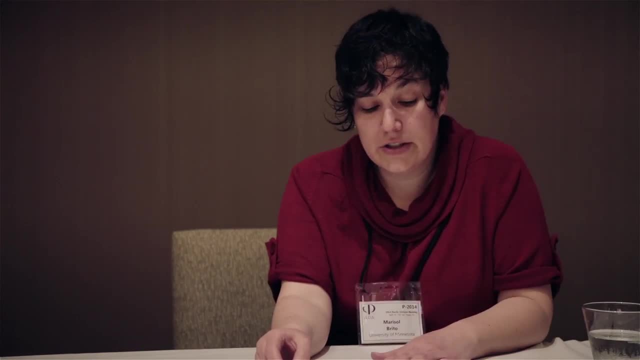 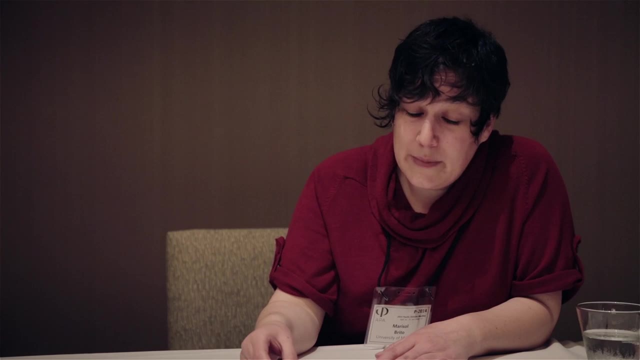 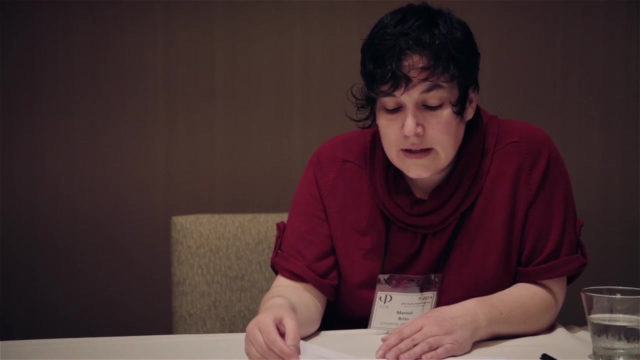 as a way to challenge pervasive societal narratives such as ageism. I know that in my own experience, the room that parenting makes for such a relationship- especially parenting on my best days, when I am able to most respectfully engage with my child- allows me to view my child as a fully developed person. 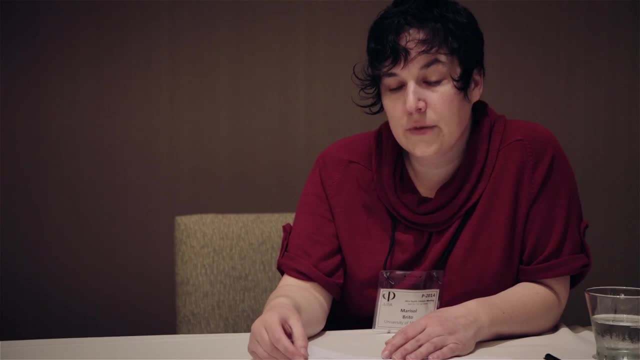 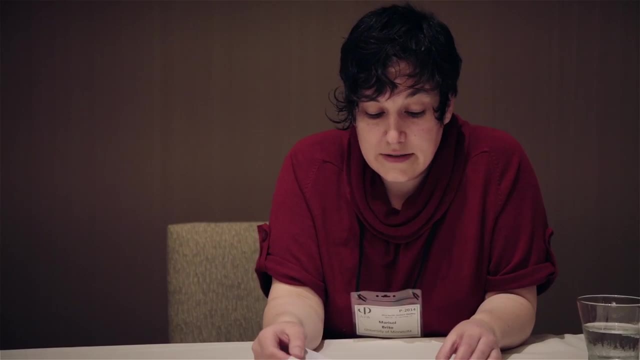 a person worthy of respect and able to teach as well as learn. The relationship allows me to stop looking down, to stop holding an impoverished sense of my child and, in turn, of other children's capabilities. It helps me to see children differently. 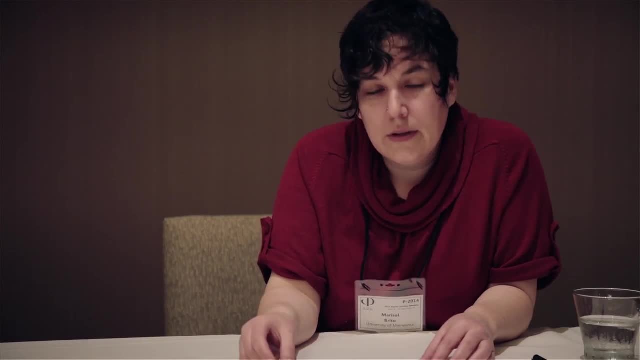 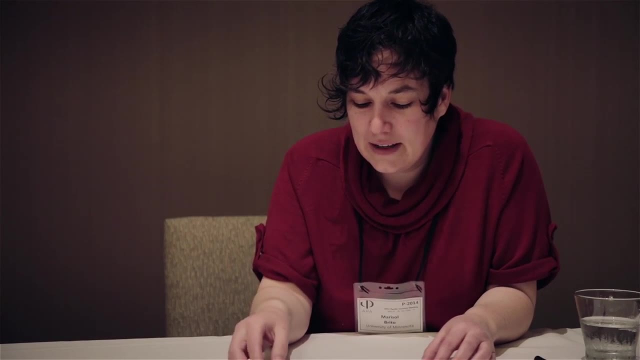 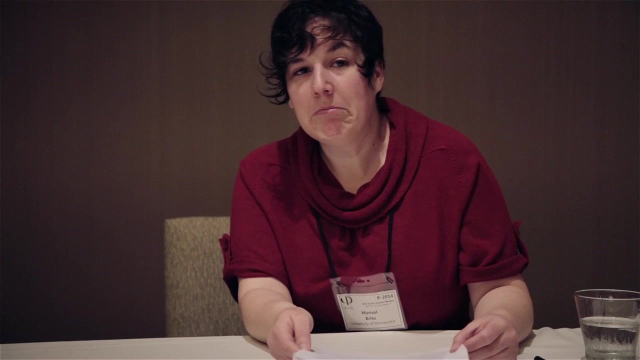 or as alter-abled as opposed to disabled. It helps me to find learning and growth which I would otherwise lack access to. Another way we might understand this, since we are a room sort of full of philosophers, is that parenting has taught me about agency. 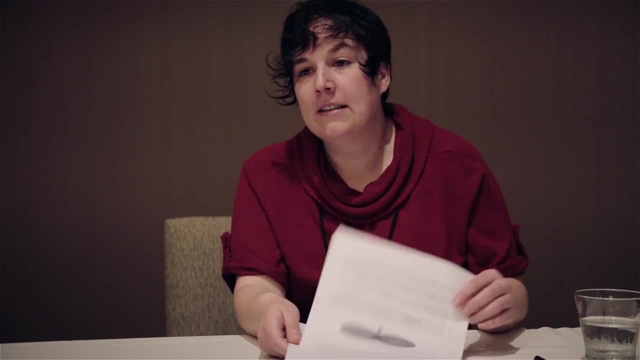 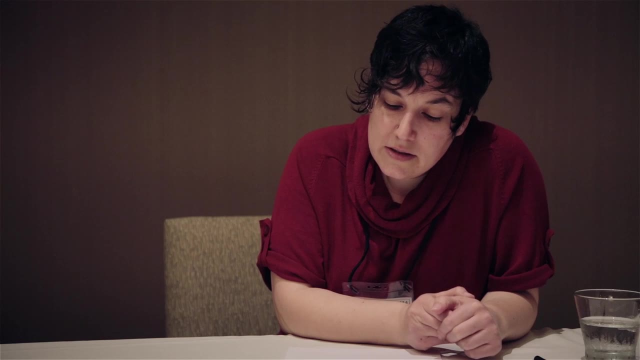 in a way that all of my studies and work with philosophy did not achieve. Others who have taught me, others who have had close friendships with children report similar experiences. For example, Gareth Matthews, who was an early advocate of philosophy for children, writes. 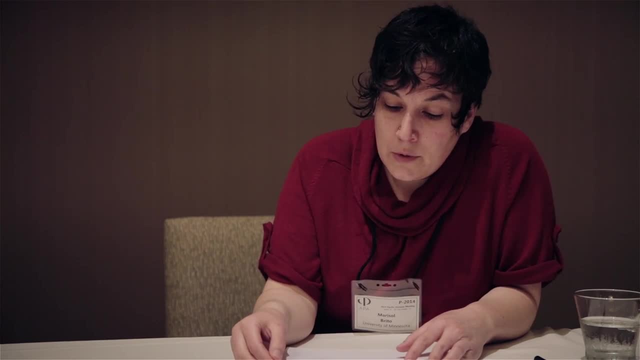 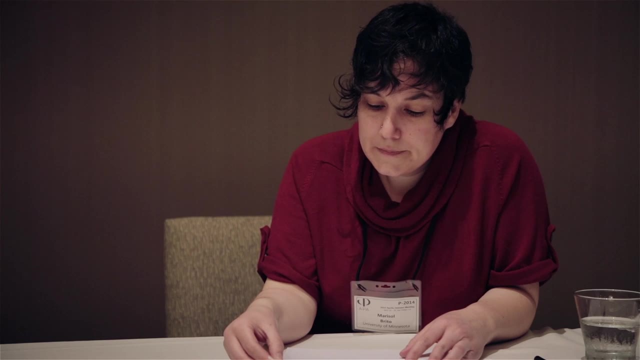 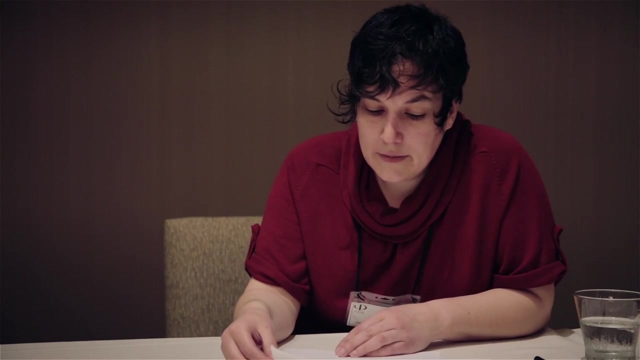 Children are people fully worthy of both the moral and intellectual respect due persons. They should be respected for what they are as well as what they can become. Indeed, we can learn from them and let them enrich our lives much more obviously than they can learn from us. 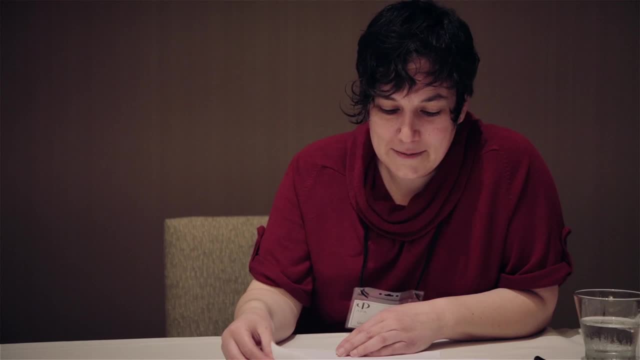 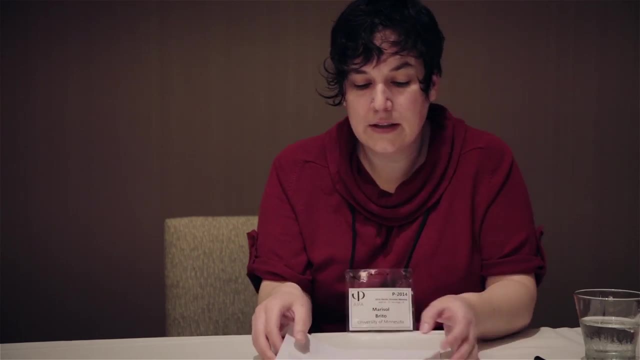 and enrich our lives. Oh, and let us enrich their lives. The parent or teacher who is open to the perspectives of children and their forms of sensibility is blessed with gifts that adult life otherwise lacks. I do not have time to go into detail about the many ways. 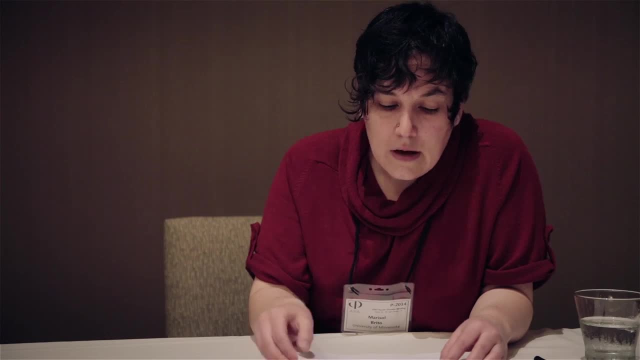 that friendship with children has influenced my life, but I will say that learning, or at least learning to endeavor to hold small children as fully developed in their own right, has changed the way that I see my young adult and adult students in the university. 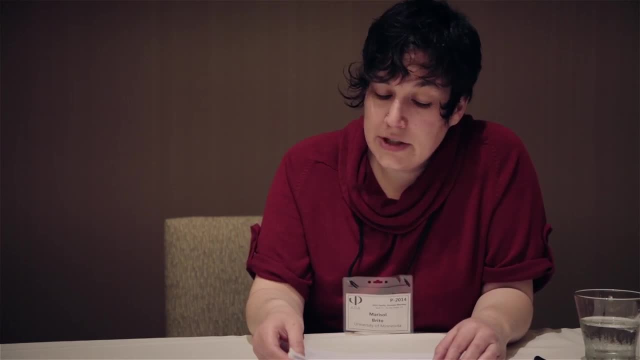 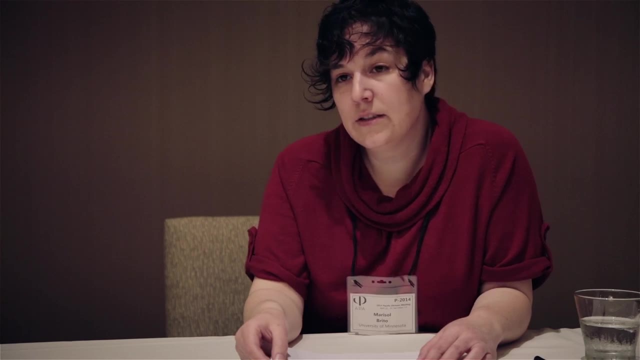 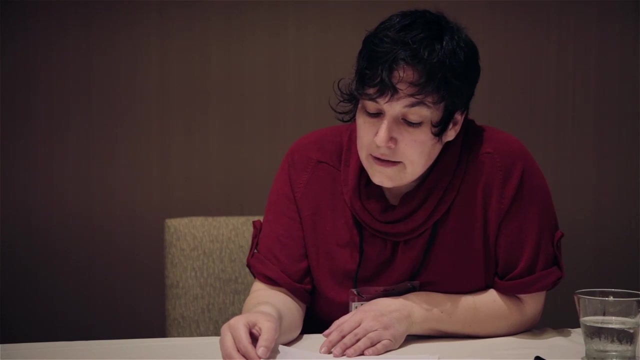 And it's pushed me to change my teaching practices so that, as a university educator, my classroom is more able to offer my students and their ideas and experiences the respect that they deserve. I will close with a call for change. Recently, there have been many discussions. 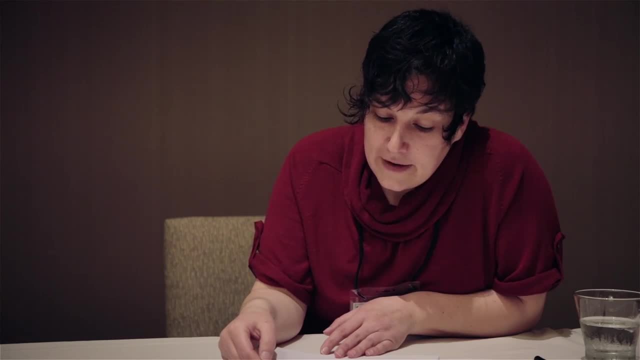 on the challenges women face in the academy. Among them is the fact that children can be a death sentence for a career, particularly the career of a primary caregiver, a role which often falls to or is chosen by women. However, if people with close relationships to children 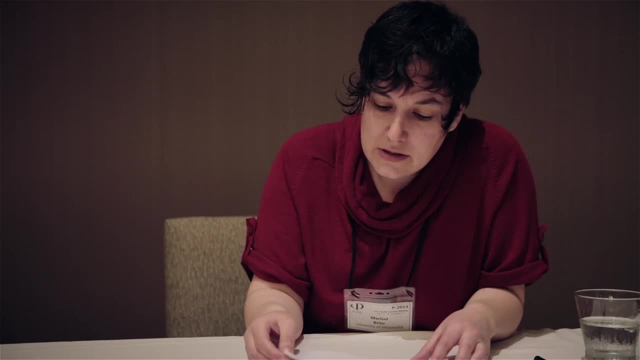 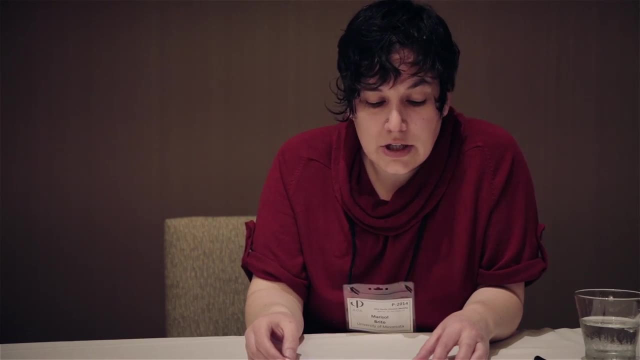 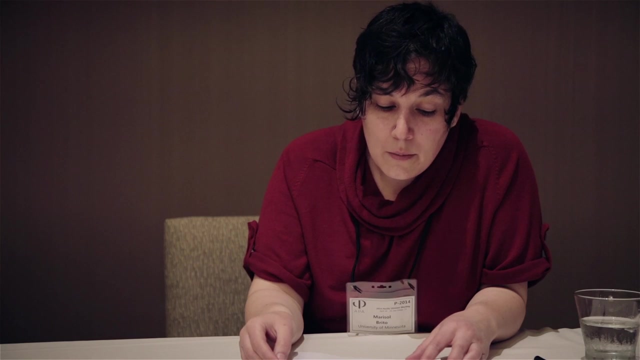 are in epistemologically privileged positions, positions that can inform not just their relationships to children but broader understandings of agency or teaching or who knows. then I would like to see more people with close relationships to children, more people being raised by philosophical children. 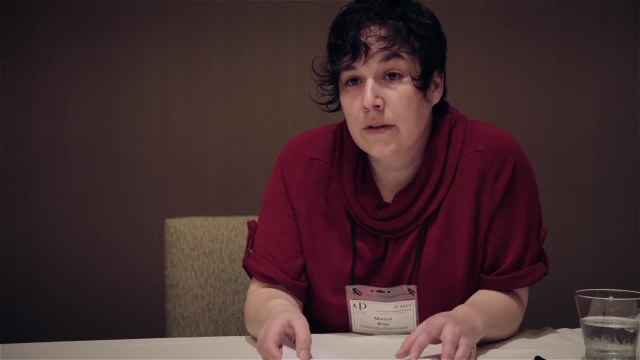 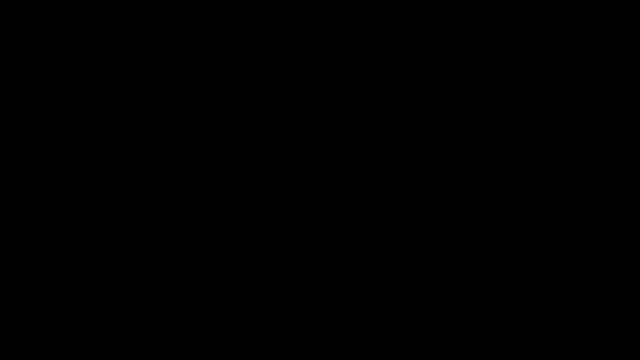 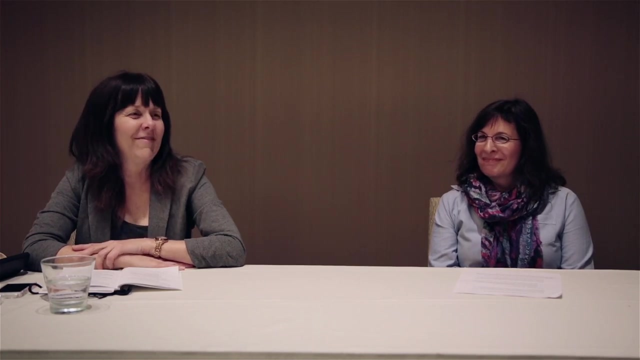 in the academy and in other influential institutions. Thank you. Our next speaker is Janet Moreland from the University of Washington, And her topic is how philosophy made me a better parent. Good morning everyone. So I want to talk a little bit about 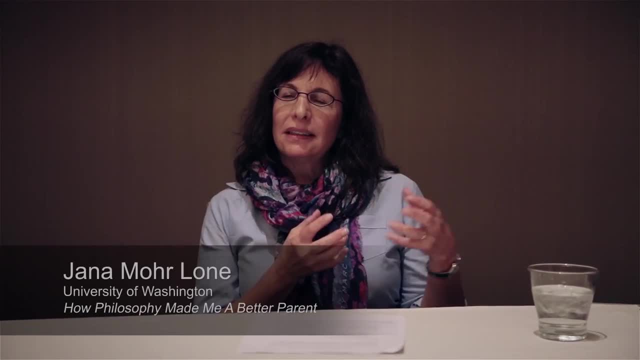 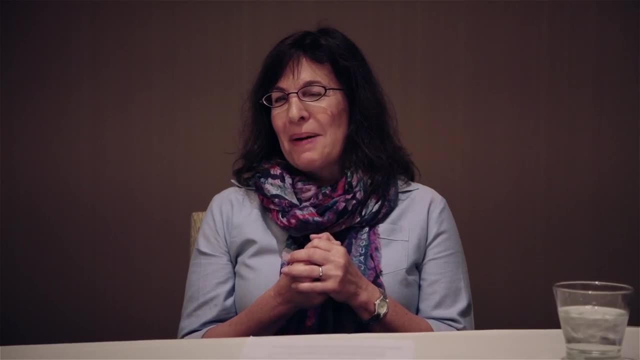 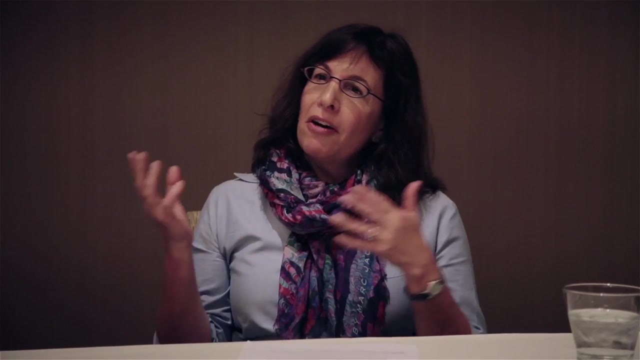 I think in some ways quite connected to Maricel's talk about how philosophy made me a better parent, if in fact it did My children. so I have three sons and they are all now 16 and up, So they're either out of, or sort of getting out of, the stage of childhood. 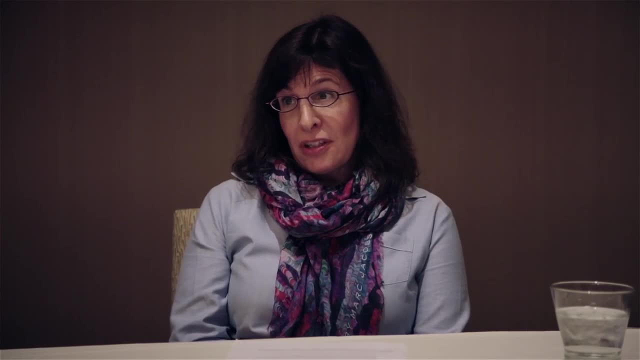 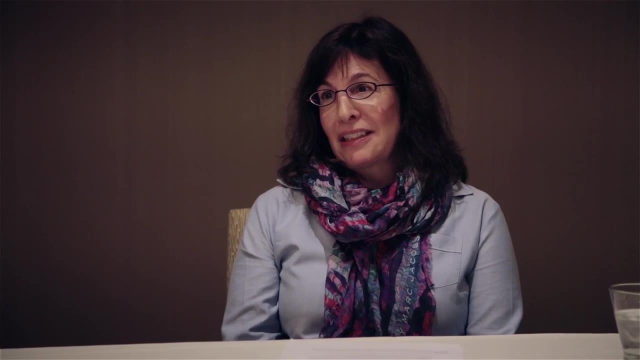 And when my first son was born I was a graduate student in philosophy and by the time my third son was born I'd finished the PhD and started my academic career. So you could say- I think my children probably would say- that they've grown up with philosophy. 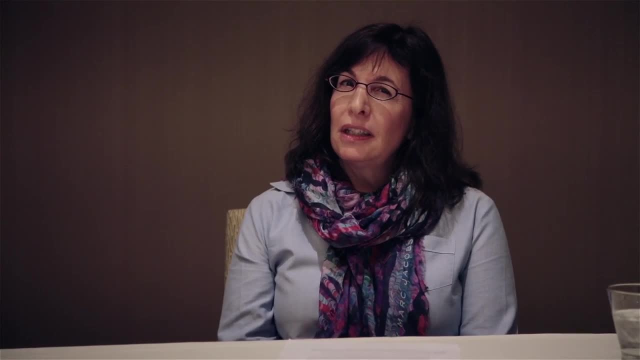 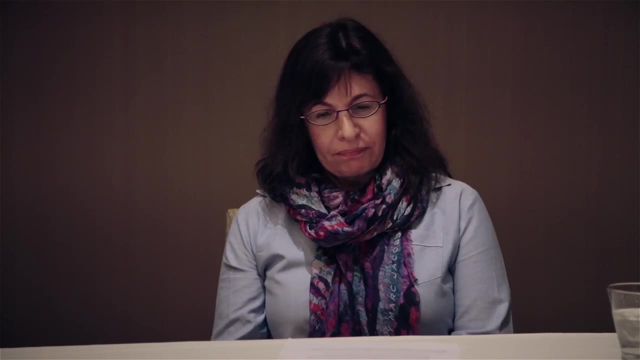 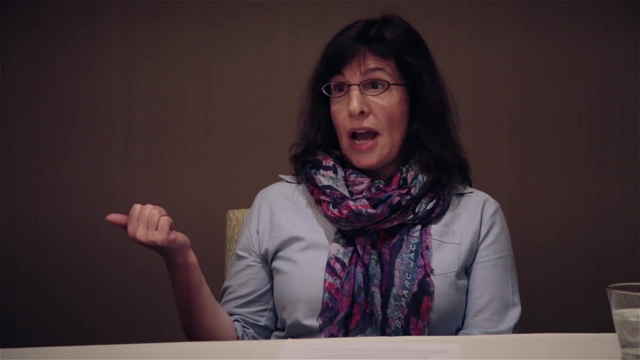 and that, and I think that in many ways, philosophy has become a core part of who I am as a mother. So how can philosophy make you a better parent? And there's a lot of possibilities, right? So here are some. Maybe reading the great works of philosophy makes you wise, right? 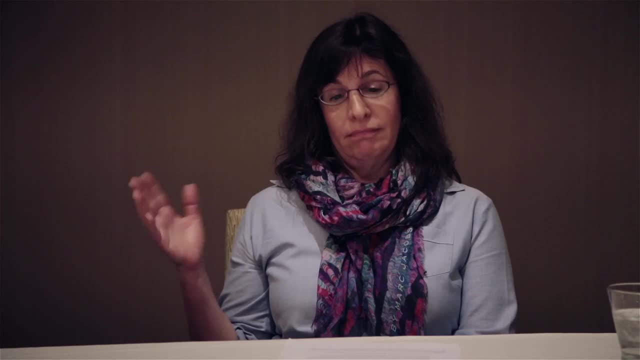 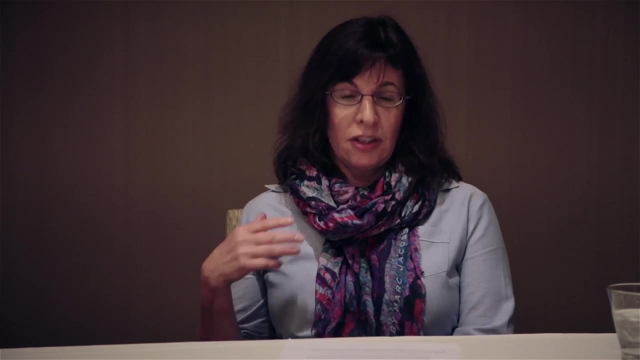 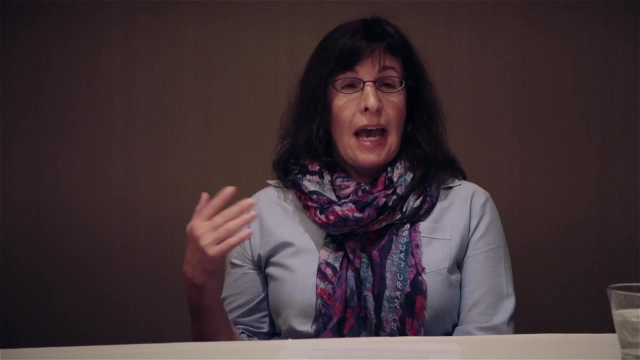 And so you're a more thoughtful, wise parent. maybe Philosophy enhances critical thinking skills, right, You learn to make arguments, to recognize assumptions, et cetera. so perhaps philosophy makes you a clearer thinking, a clearer thinker and one more able to see. 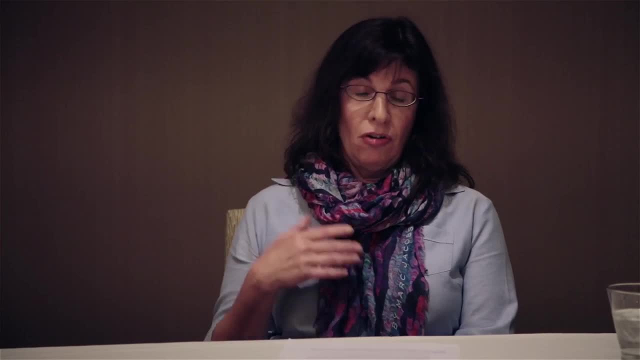 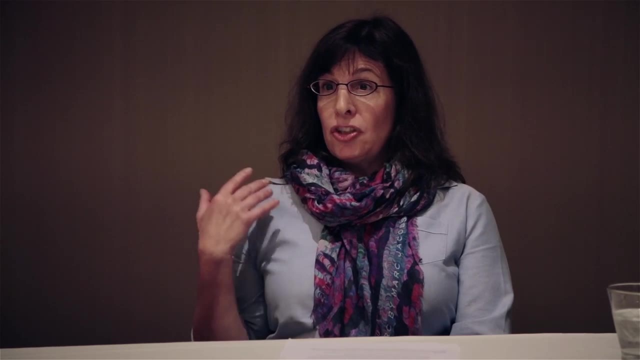 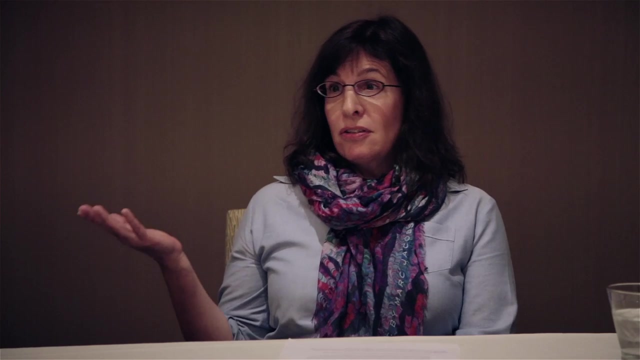 when you're making unfounded assumptions about your children or engaging in inconsistent parenting, et cetera. Third, engaging in philosophical arguments makes you maybe a stronger advocate, so you're able to be more of an advocate for your children. I'm not sure whether any of those are right or not. 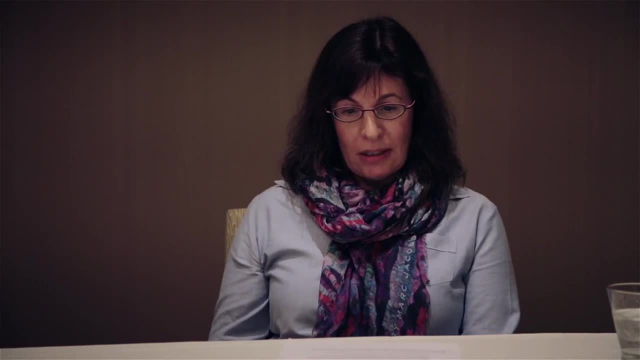 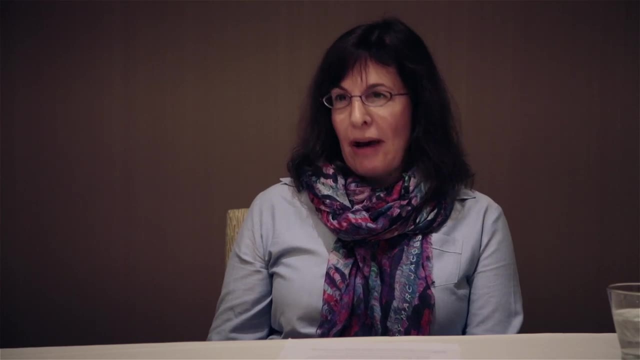 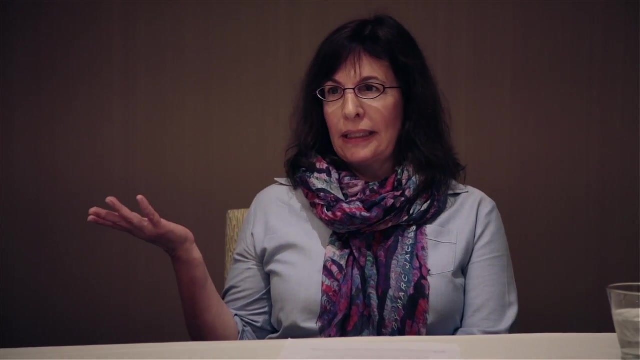 but they're not what I mean by philosophy making me a better parent. What I'm interested in is the philosophical encounter, the act of engaging in dialogue with your children about philosophical questions, not as the philosophical expert, but as a kind of philosophical companion. 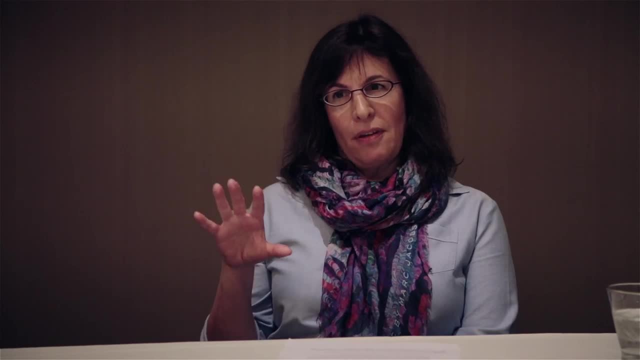 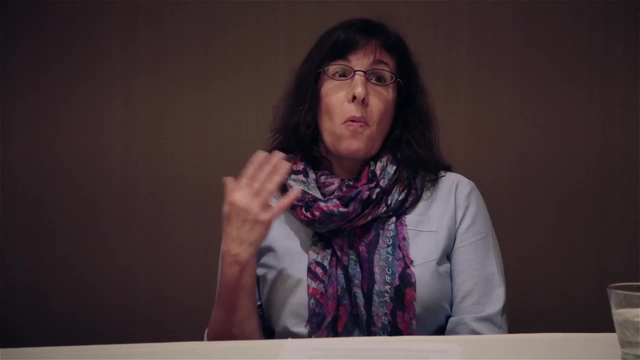 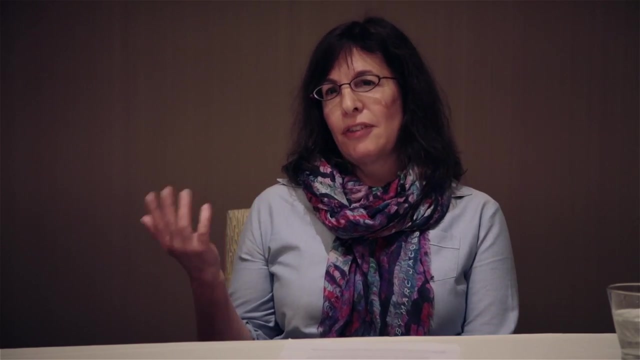 So it's not being a philosopher that made me a better parent, but philosophy that did so, And so I think I should say something, then, about what I mean by philosophy, because, of course, this is a somewhat contentious question. For me, it involves a very expansive view of what philosophy is. 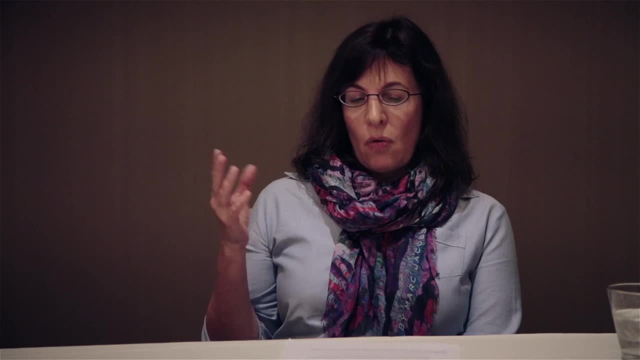 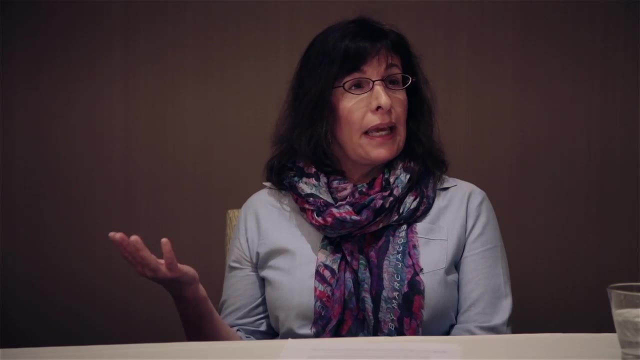 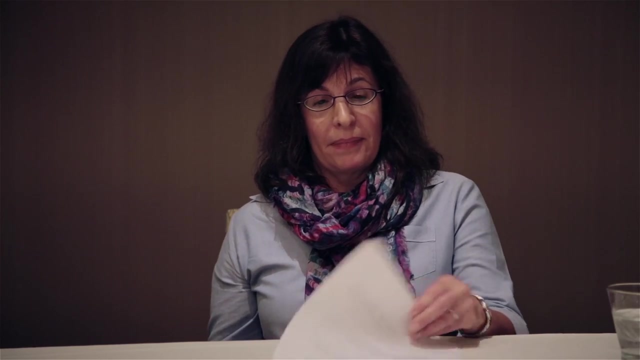 that sees philosophy as involving wondering about the large questions of the human condition, And I think this is an activity that most people engage in at at least some points in their life and that many, if not most, children engage in all the time. 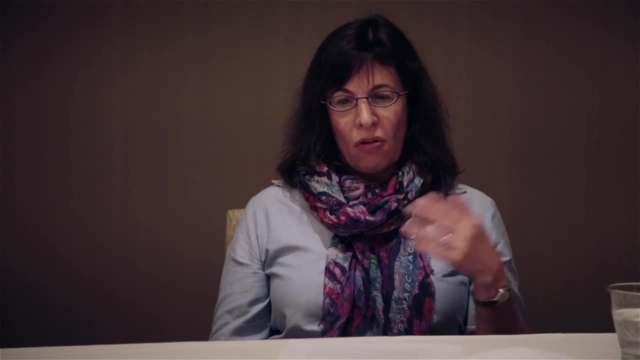 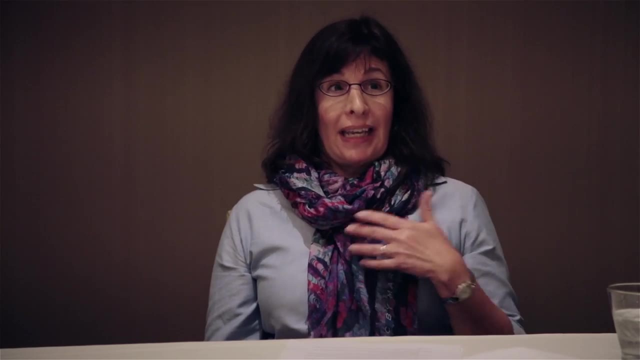 And so philosophical encounters with children don't require you to be a professional philosopher, and actually it can be hazardous, I think, to be a professional philosopher in engaging with children philosophically, in part because you might be tempted to be a little bit more pedantic. 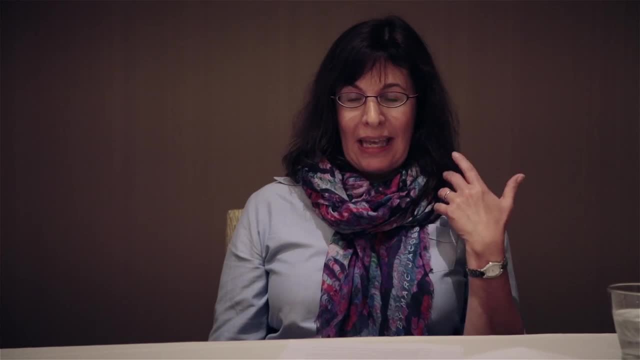 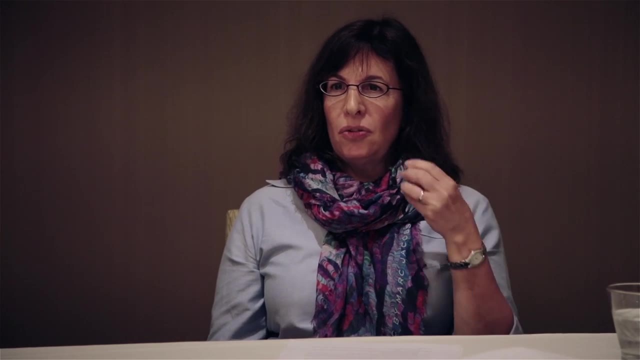 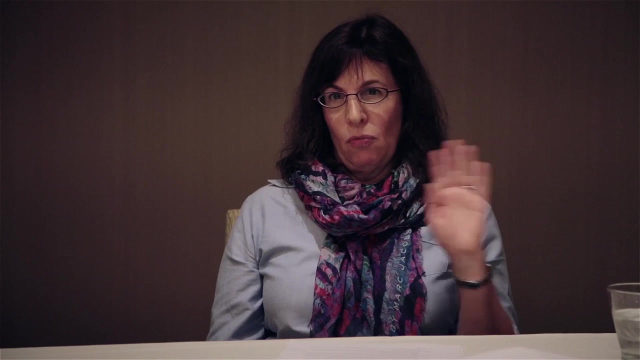 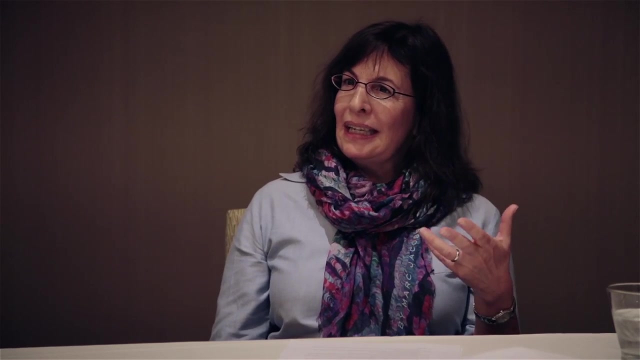 than if you weren't a professional philosopher. And I think doing so authentically with children requires a kind of sensitivity to their thoughts and questions and less focus on your own thoughts and questions or, even worse, your own philosophical answers. So it's really kind of a skill at appreciating the perplexity in life. 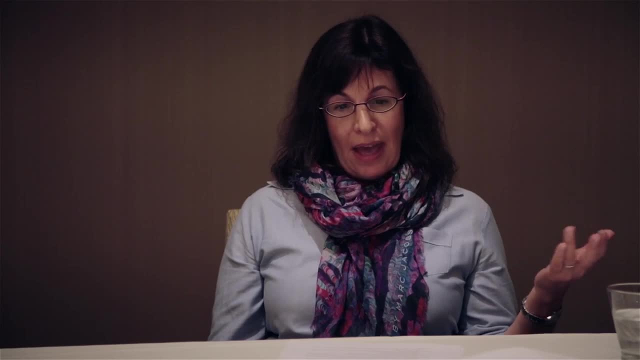 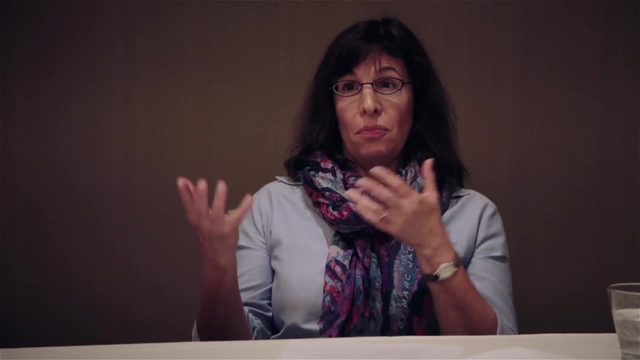 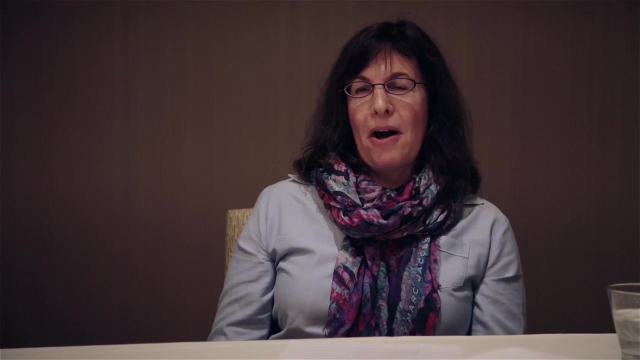 and really listening for children's awareness of that And having children's awareness of that open you up more to how much perplexity there is in just everyday life. So I thought I'd give you an example of a conversation I had with my children. 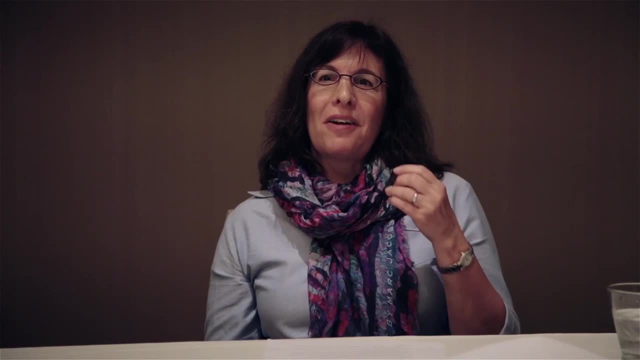 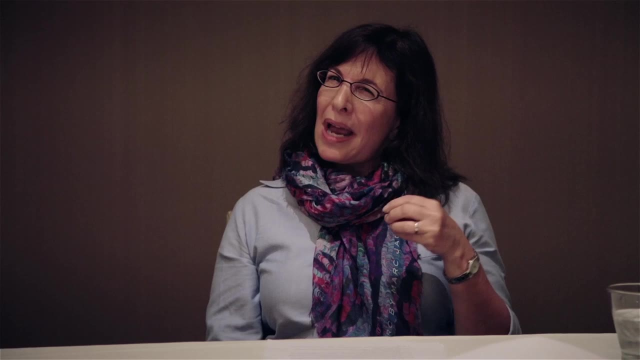 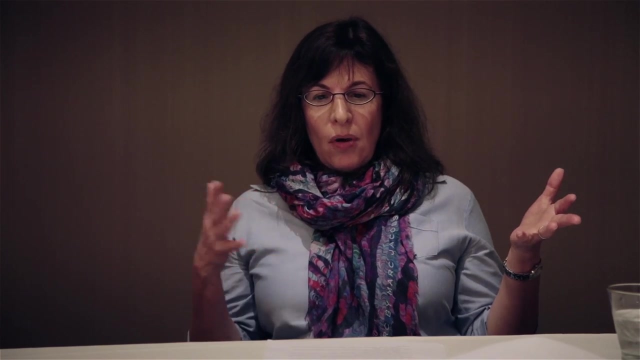 This is from my book, Because I think that one of the things, one of the things being a parent did was allow me to see philosophy everywhere in a way that graduate school really didn't do Graduate school, I think, in some ways, although I was a philosophy undergraduate major too. 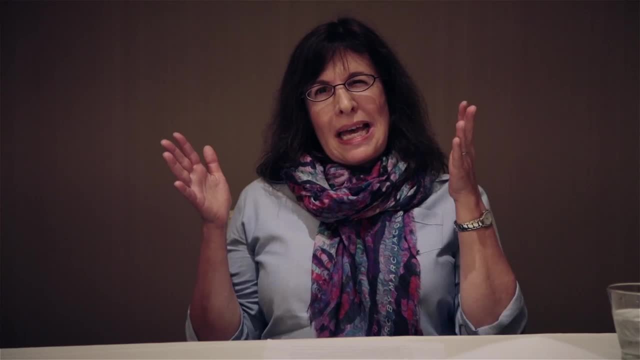 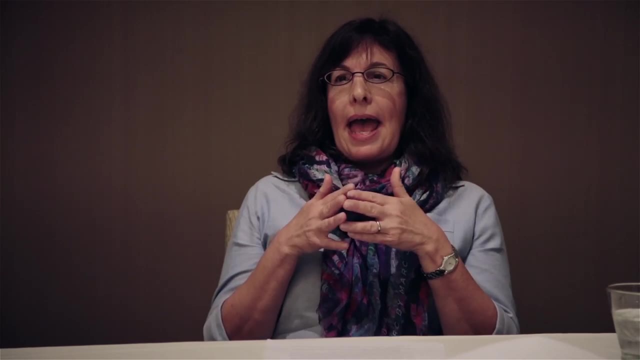 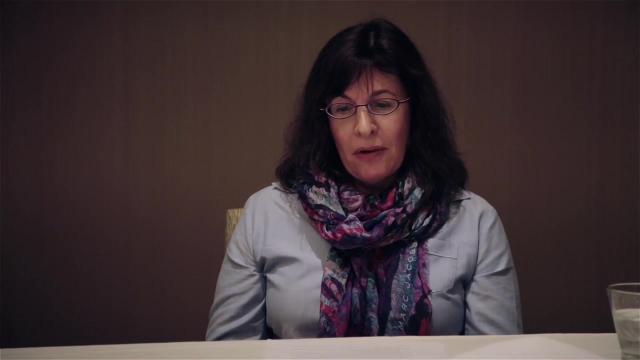 but to some extent, I think graduate school gave me a sense that there was a closed set of philosophical questions, or at least interesting philosophical questions, and being a parent really changed that perspective. My oldest son, Will, was around five. We loved to read Arnold Lobel's Frog and Toad stories together. 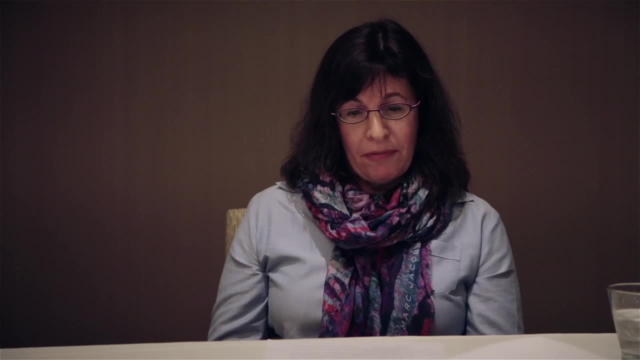 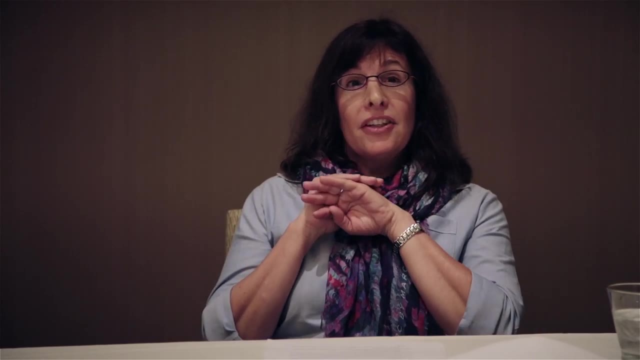 One evening we were reading the story The Dream from Frog and Toad together And for those of you who are parents of young children, if you don't know Arnold Lobel, he is wonderful for writing philosophically suggestive stories. He's one of my favorites. 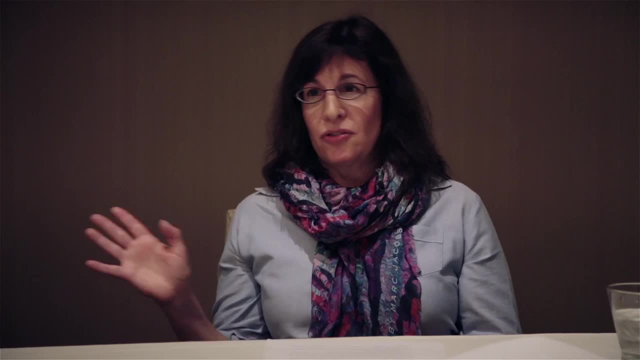 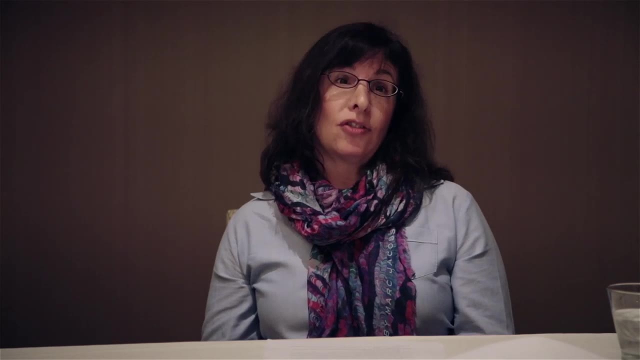 I use him all the time in classrooms and my children and I read those stories thousands of times probably. So we were reading the story The Dream from Frog and Toad together, and in the story Toad has a dream about starring in a play. 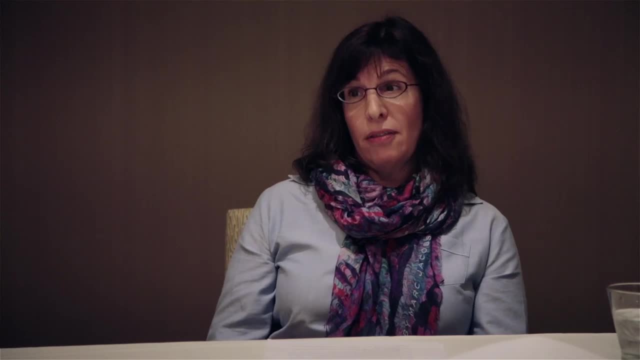 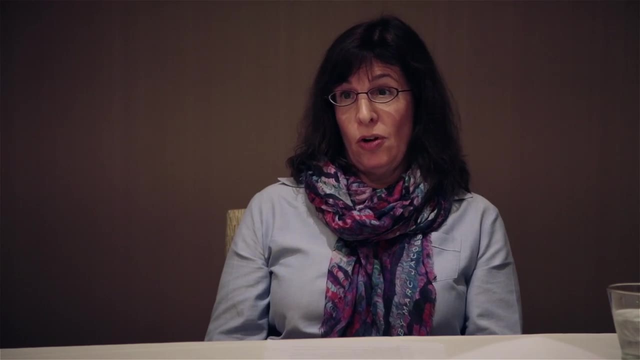 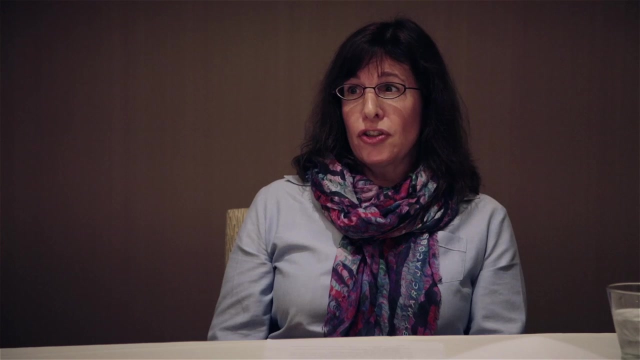 and in the dream, his best friend Frog sits in the theater watching As Toad performs. Frog starts shrinking until finally he can no longer be seen or heard by Toad And as Toad performs, he starts screaming for Frog, stops performing and starts screaming for Frog. 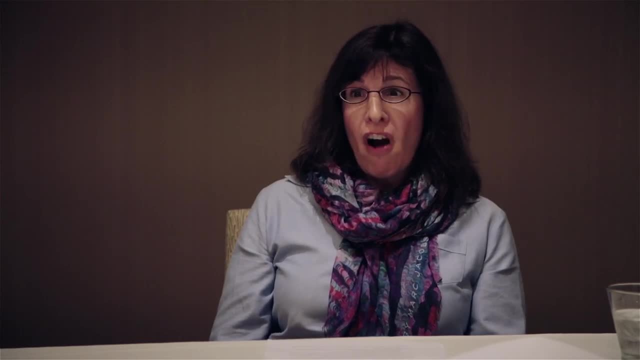 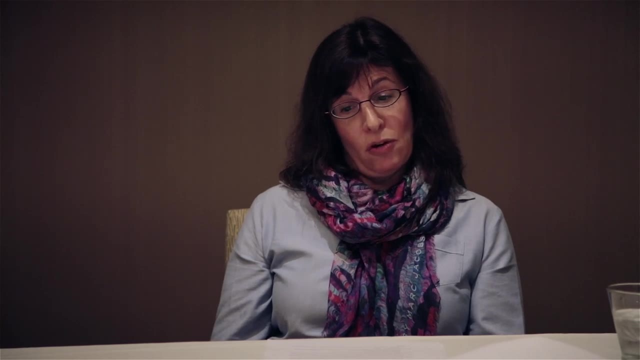 and waking up, there's Frog standing right by his bed. Frog, Is that really you, Toad? asks Frog. assures him that it is Toad, utterly relieved, spends a quote fine long day with Frog. So Will and I read the story. 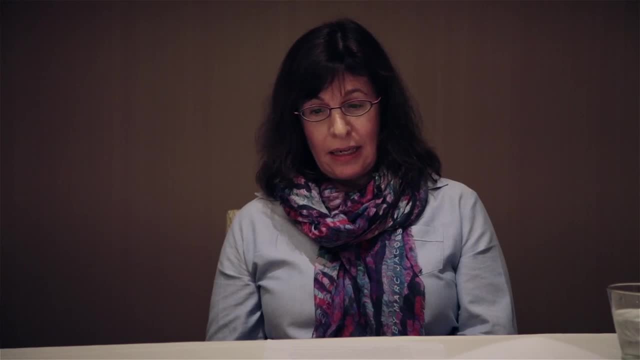 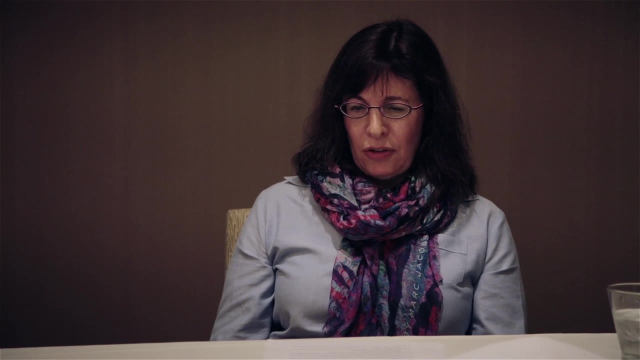 and we started talking afterwards about dreams, about some of the dreams he'd had and about how real the dream in the story had seemed to Toad. Did you ever have a dream that felt so real that you woke up and for a little while you weren't sure it was a dream? I asked: 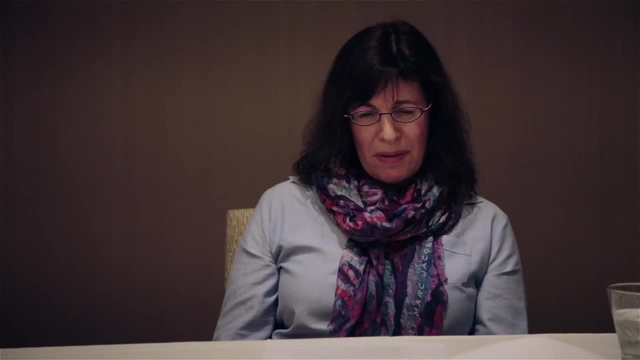 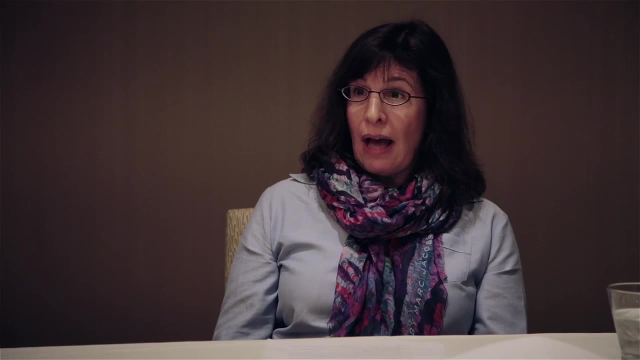 Yes Will responded. And then sometimes I wonder if I'm dreaming when I'm actually awake. I mean, could we be in a dream right now? What makes you ask that? Well, how do you know we're not? Do you think there are differences between the way dreams feel? 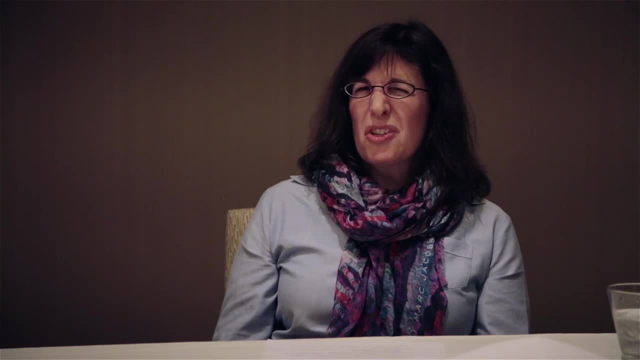 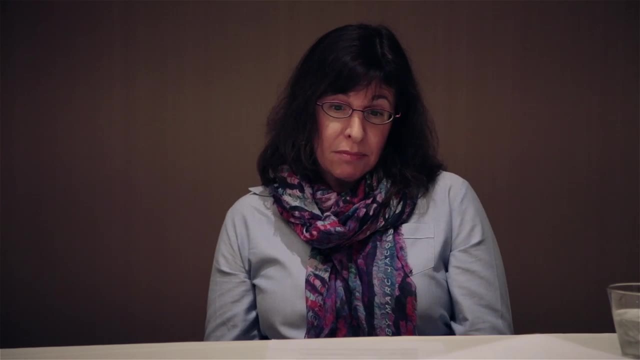 and the way being awake feels. I asked: Dreams usually feel weird, like things happen in them that would never happen in real life, But not always right. You said sometimes a dream feels so real you're not sure. later it was a dream. 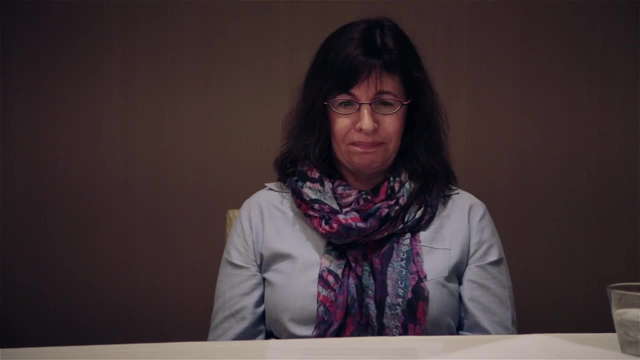 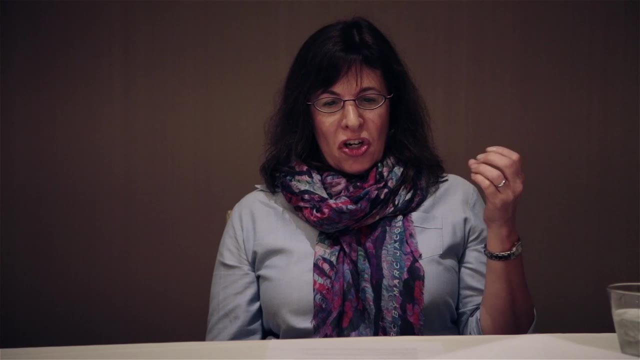 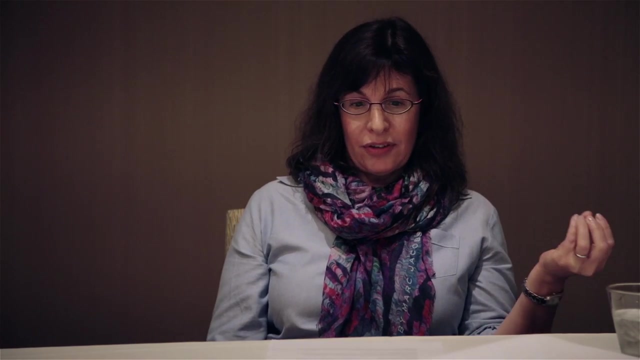 Yeah. so it could be that I'm dreaming right now. So I think, sort of having these conversations unfold created a number of moments, I guess I would say, for Will and for my other sons, And one of them is having the experience of having an adult. 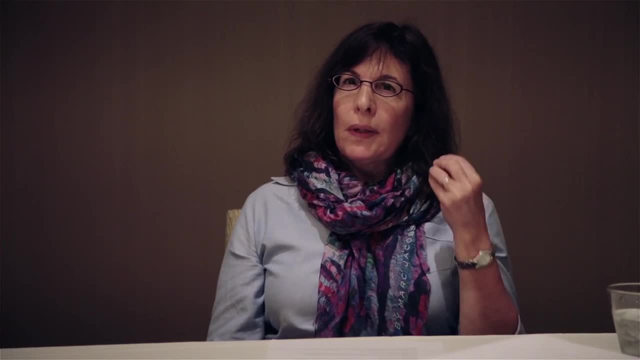 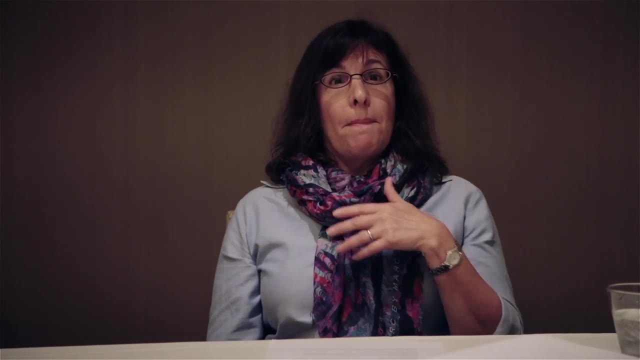 really listen to you. right, And really listen to you, not in the way of: oh, what an amusing thing is. my son said that I can repeat to all my friends. but really listen, because I'm really curious about who he is and what he's thinking. 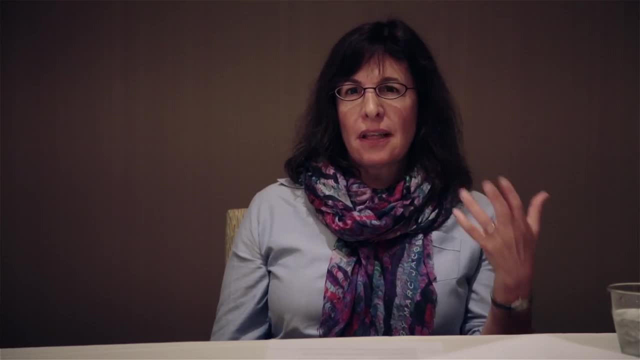 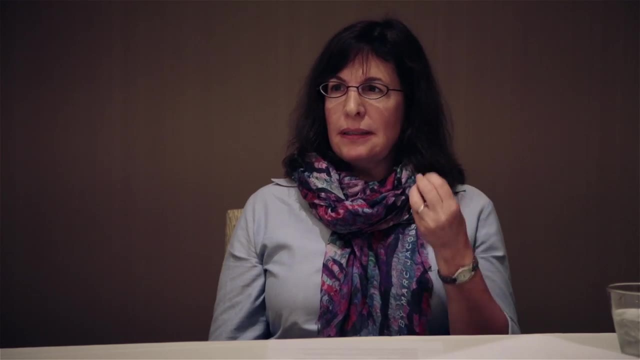 And I think that when you're a child, having someone listen to you in that way is not a typical experience and gives you a sense that what you have to say, what you think, the way you experience the world, is really worthy of attention. 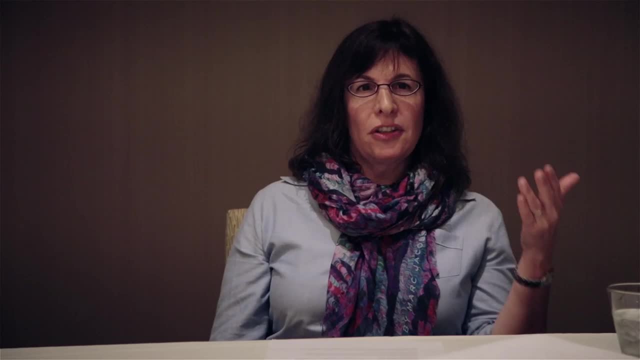 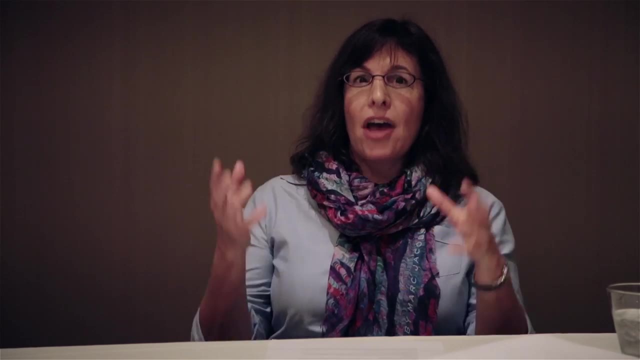 And I think there's reverberations of that experience that are very powerful for children and for the adults engaged in the encounter, because as you're having these conversations, you're seeing that there's- I mean, you know, there's- so much to learn from your children. 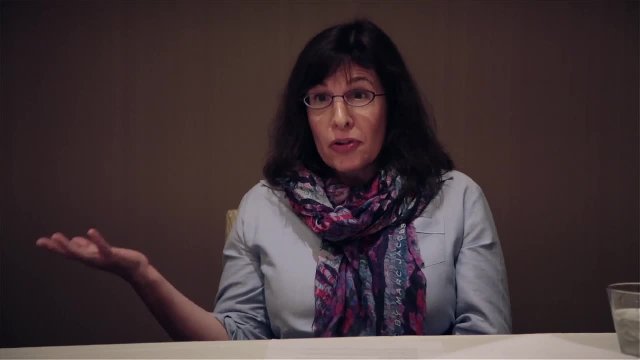 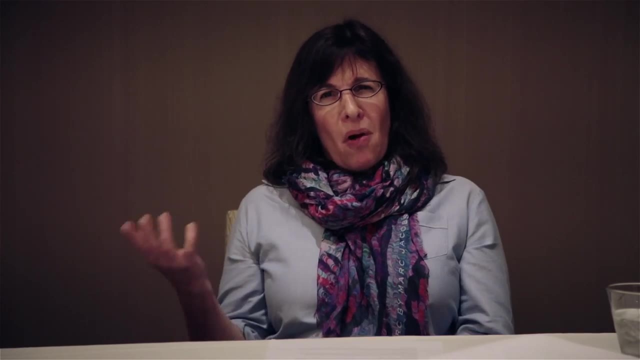 You learn how to be a better- hopefully be a better- person, right? Because parenting requires a lot of patience, a lot of diplomacy, a lot of juggling, a lot of care. But you also learn about yourself through these conversations. You learn that sometimes you make all kinds of assumptions. 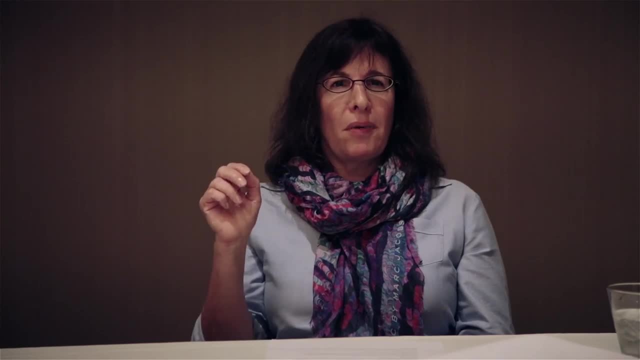 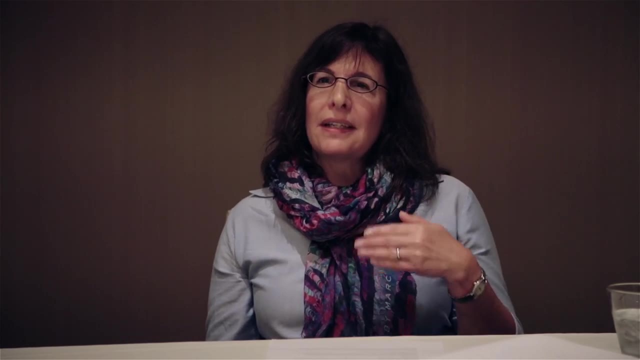 I mean you start off a conversation thinking, oh well, it has to go this way or, of course, that can't be right. I mean Marisol refers to some of this in the talk she gave today And one of the things that can happen. 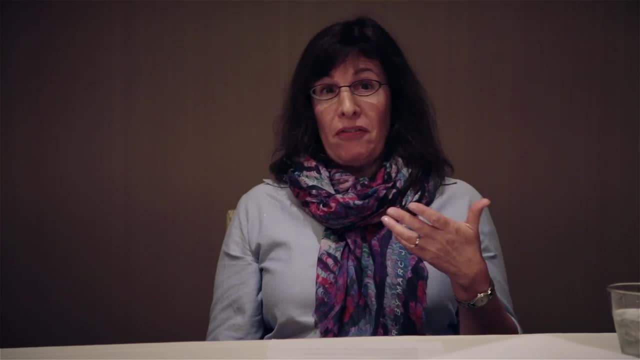 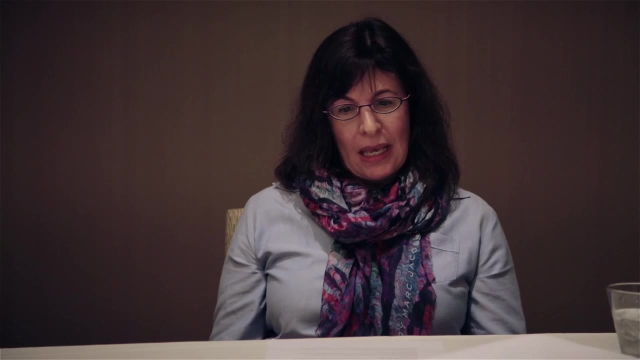 when you're really listening is that you start to recognize that you have lots of unfounded assumptions too, and that your children can really open you up to seeing them. So we all know that children ask these kinds of questions, right. Everyone's aware of the why questions right. 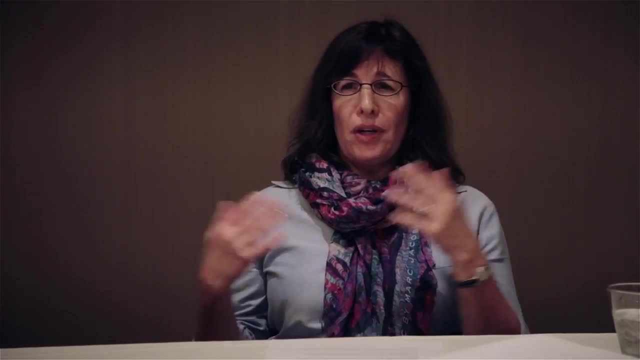 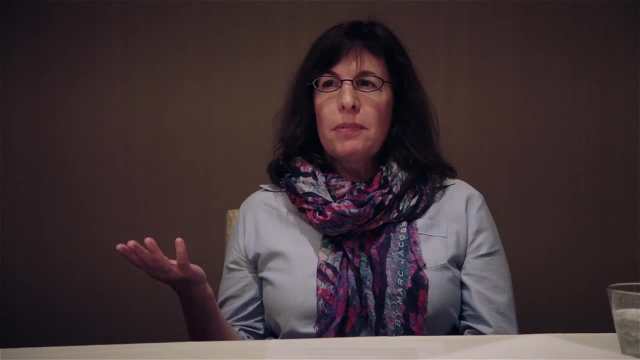 that four- or five-year-olds ask all the time: Why do I dream, Why do I have thoughts, Why should I be fair? And these are obviously philosophical questions, but most people assume children aren't philosophically capable. So why is that? 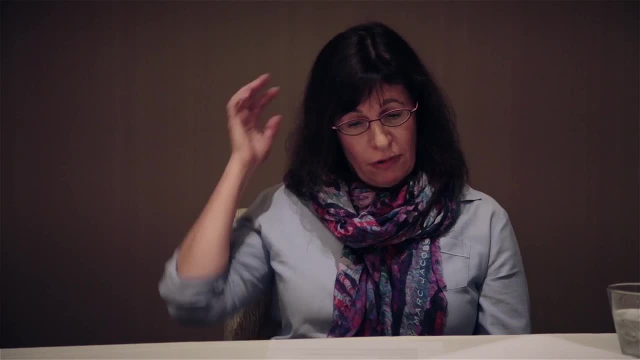 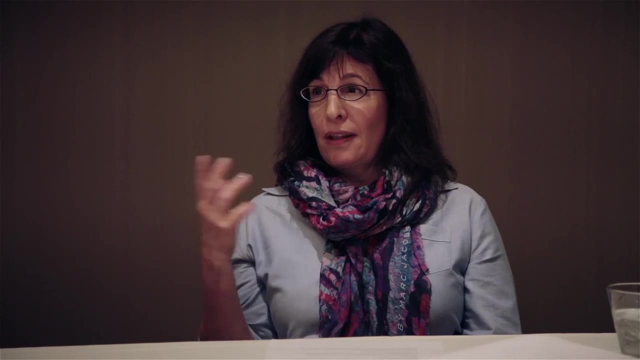 And I think there's two reasons. One of them is the reason that Marisol referred to a little bit, which is that children are typically underestimated, And I think in no area is that more true than in their capacity for sustained reflection. But I think also that 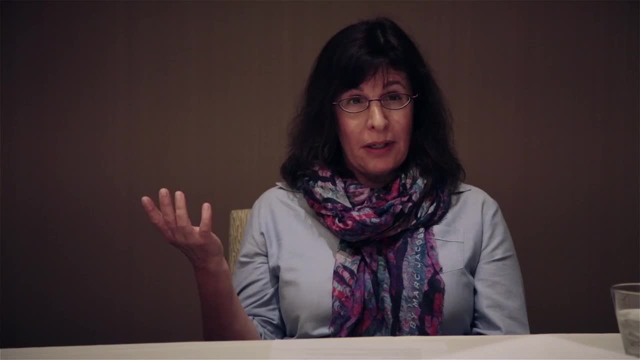 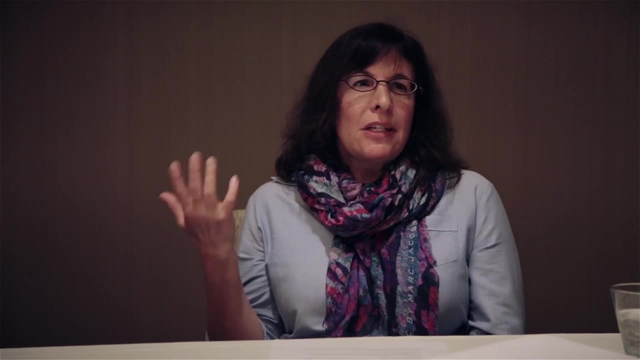 philosophy has become a kind of esoteric discipline that people think of as belonging in the academy, that is inaccessible, for which you have to have advanced degrees, and we don't see our ordinary musings about the world as involving philosophy. I mean, I hear this all the time right. 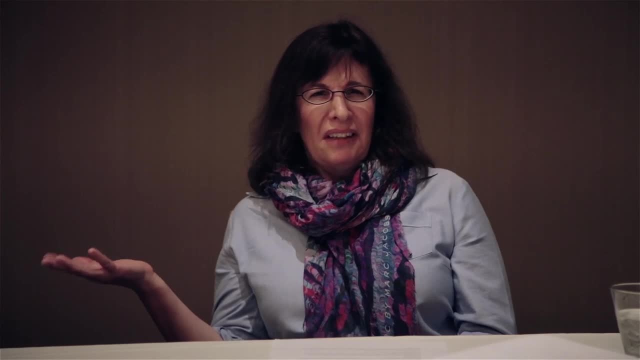 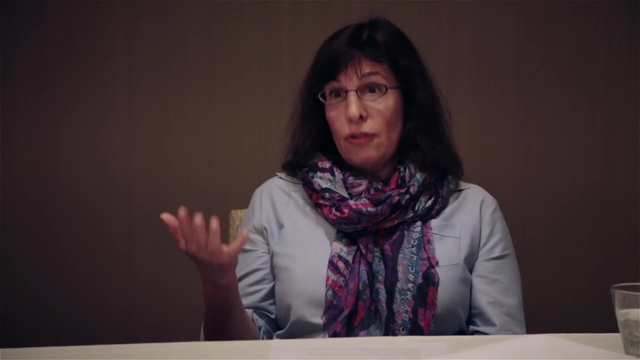 because I'll say to people: I go to schools and I do philosophy with children and they say: you know, how is that possible? How can children do philosophy? And then when I talk about- well, you know, children ask these questions. 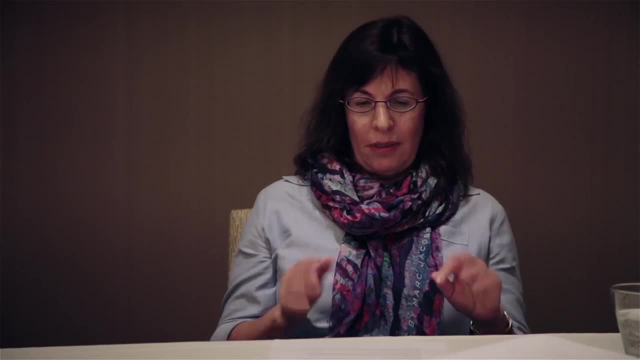 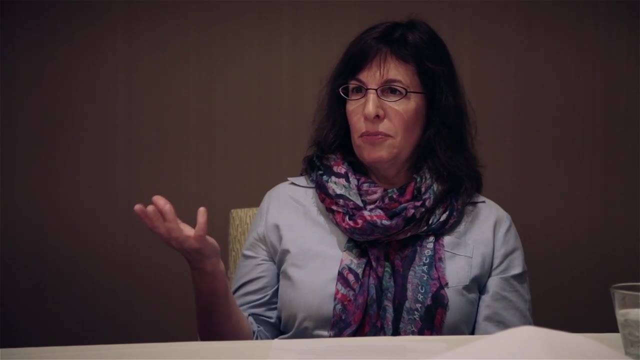 of course that's right, right. We just don't think of that as being philosophy, We think of that as something else, right? So as a result, we don't hear children's philosophical musings, because we've already assumed that they aren't there. 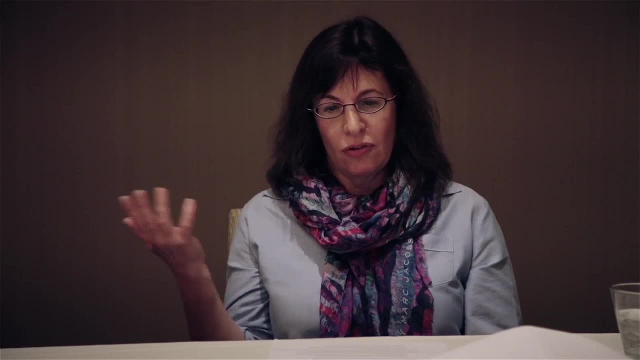 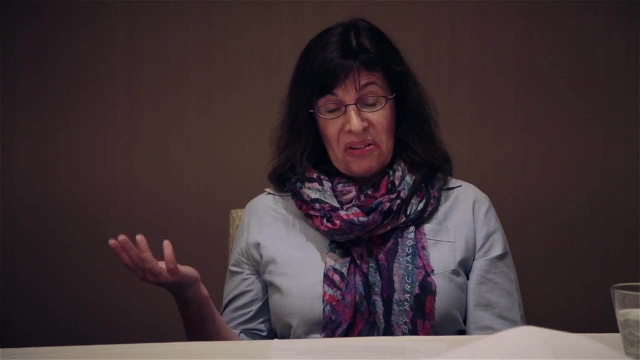 that they can't have these thoughts because they're too abstract or too difficult or whatever, And so when they do make them, children's questions and expression of ideas are treated either dismissively or condescendingly. right, There'll be a remark that a child can make. 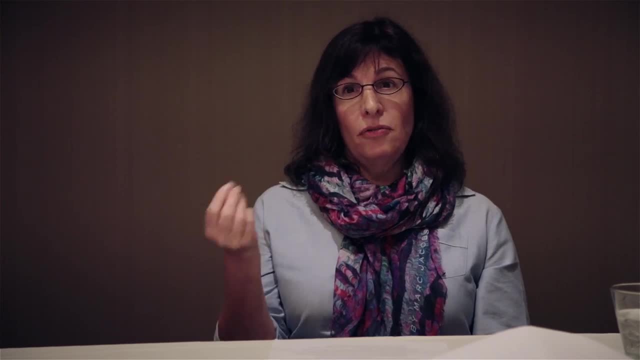 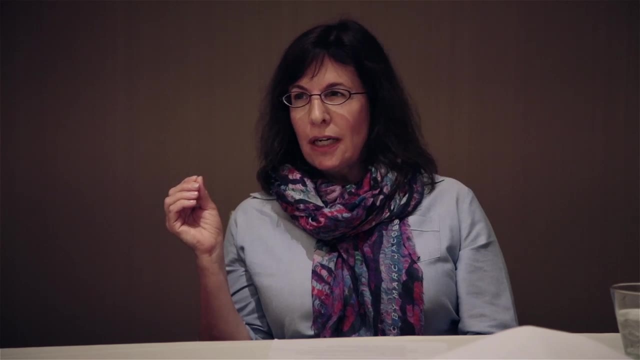 and the fact that the child makes it leads adults to find it amusing. Or I remember, even when I was a child, I would say things and some of the adults would say things that really irritated me, like: oh, what a little philosopher. 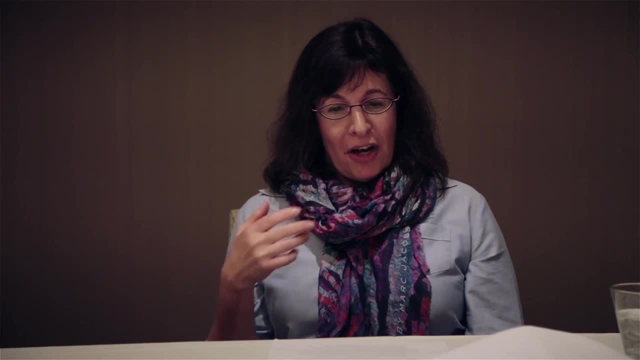 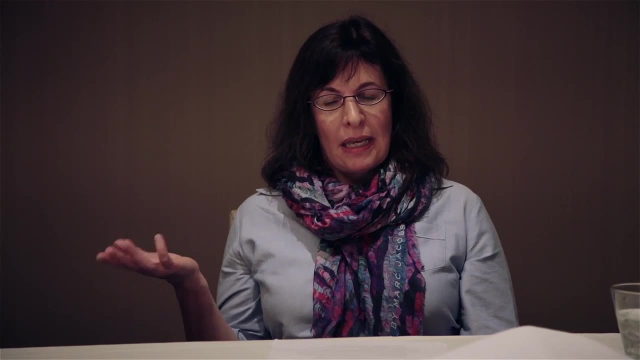 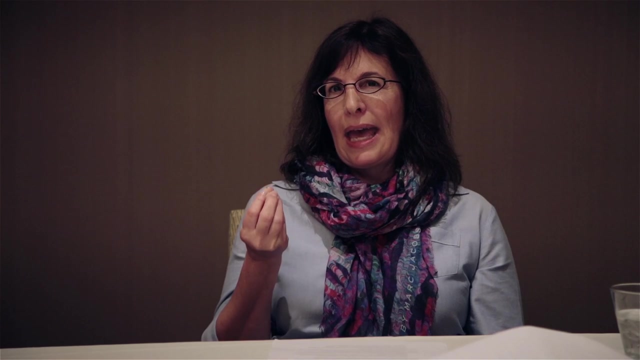 And I'd be like: you know what does that mean? right, And yet if an adult said the same thing, it would elicit a more thoughtful response. So I think there's something really important about taking children seriously And really listening to what they say. 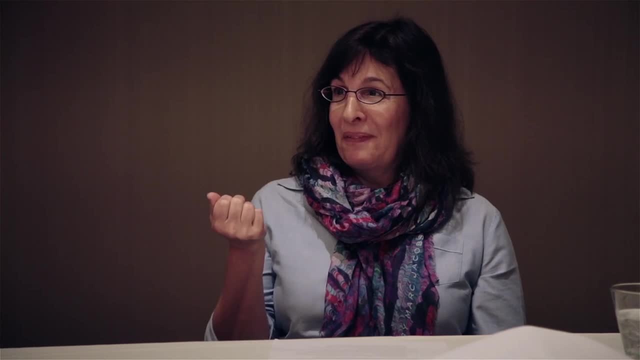 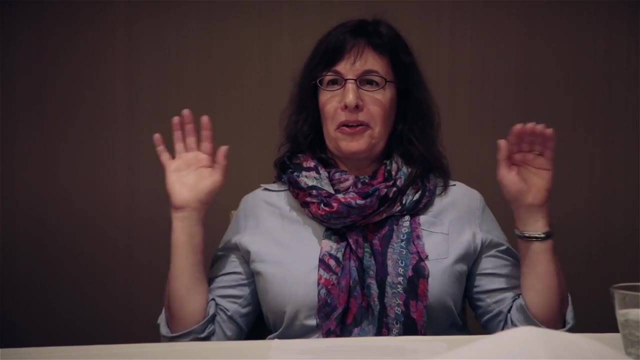 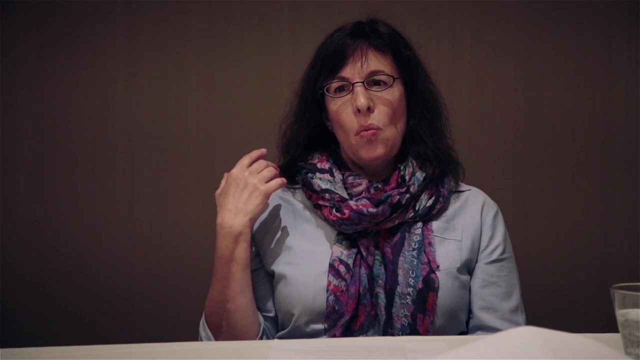 And that doesn't mean that we do it all the time right. It doesn't mean that in every exchange with our child we are the perfect, philosophical, calm parent. right, Because that's not going to happen. right. And it doesn't mean that we can't sometimes. 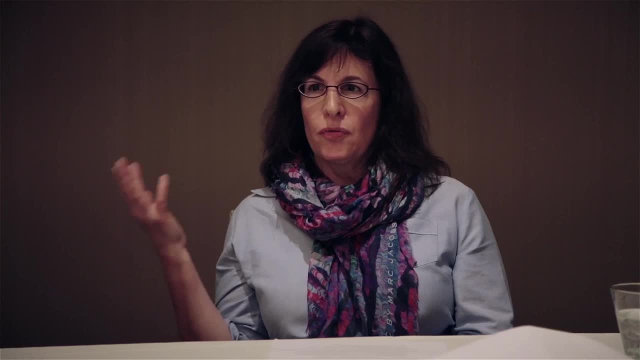 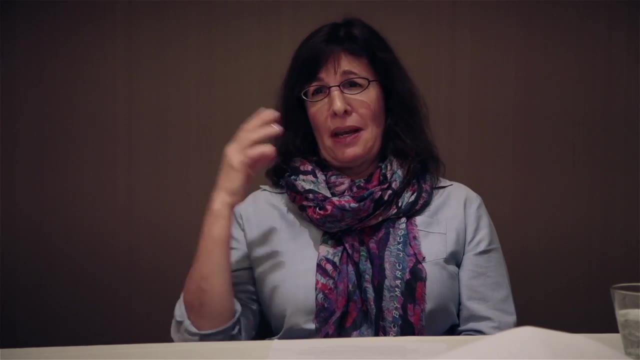 still be the authority figure. I mean, I would have conversations with my teenagers about the nature of rights and whether children should be able to vote, etc. But then I'd still be able to say, no, you're not staying out until 2 o'clock in the morning. 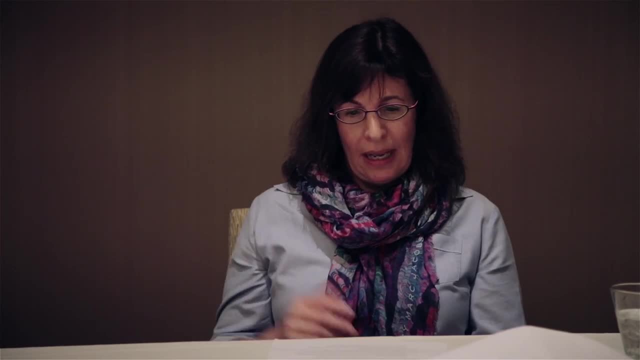 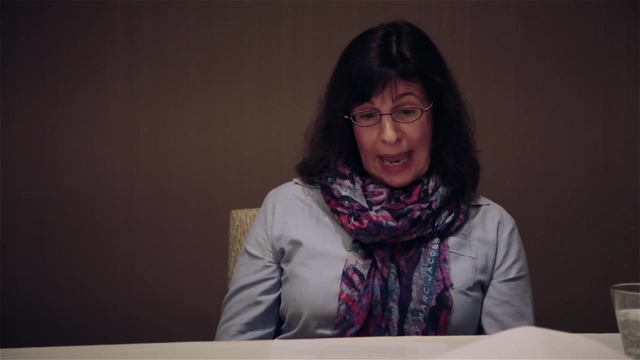 sorry, right, And that's okay, right. So I'll give you another example of a conversation with my middle son, David, when he was about eight. We were looking at a book about numbers and David commented that numbers are beautiful. 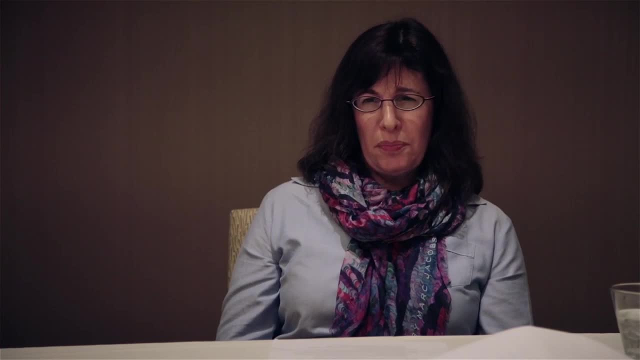 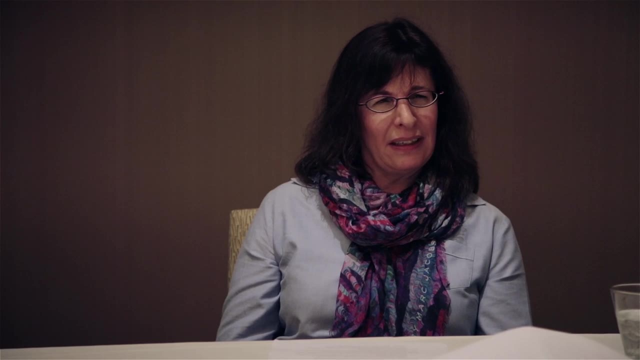 This is also a passage from my book. What makes you say numbers are beautiful? I asked David. They're just so perfect. he commented: All the patterns kind of like puzzles. What do you mean, I don't know, With number one? there's just one of everything. 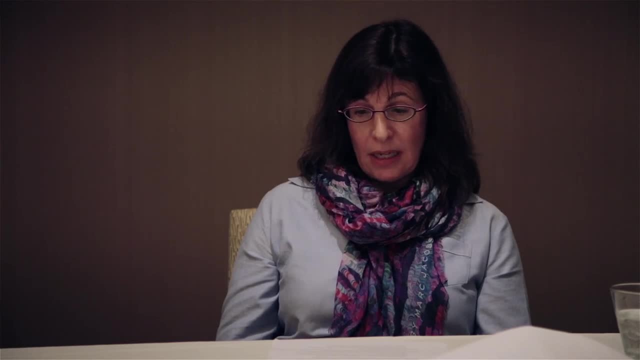 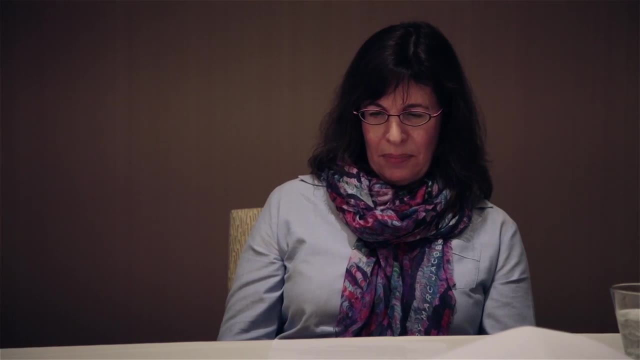 But then you go to two and there's two of everything, so everything doubles and the whole thing changes completely, And then it happens again when you get to four. It's one of those things that seems simple, but the more you think about it, the more interesting it is, isn't it? 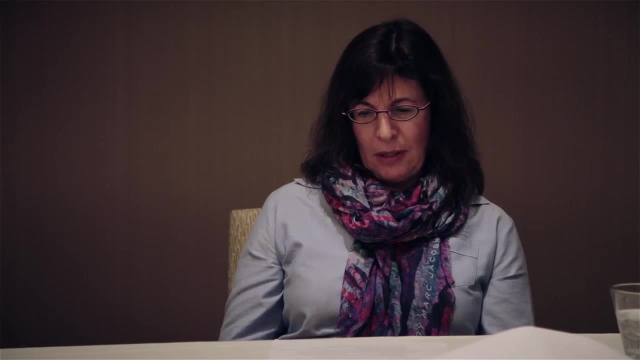 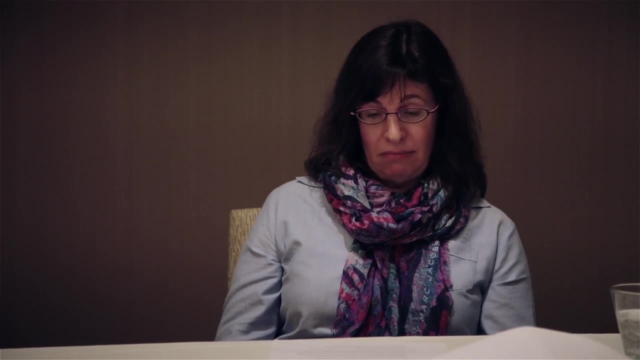 I responded Exactly. I love looking at these pictures and thinking about the numbers. So do you think numbers can change? They can be like art in a way. I asked. I think so. I guess. I mean, what makes something art? 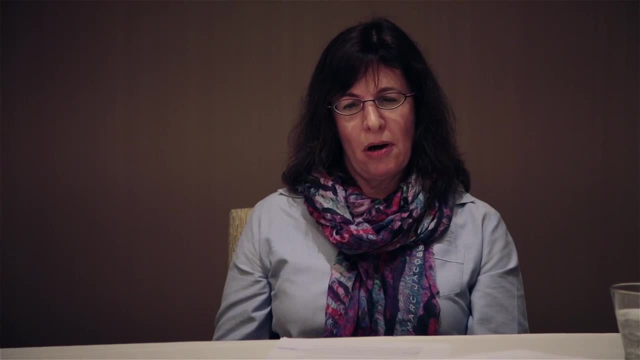 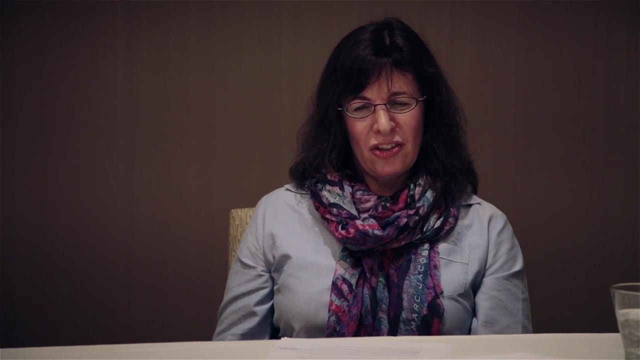 Well, is the book art? Yes, David paused. Maybe The pictures are beautiful, So is being beautiful. what makes something art then? Not sure, I mean, I think there are beautiful things that aren't art, Like what I asked. 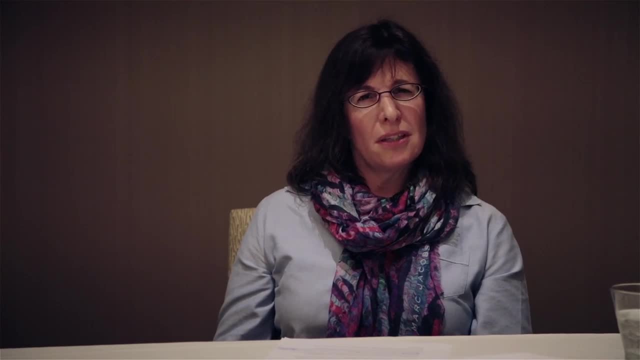 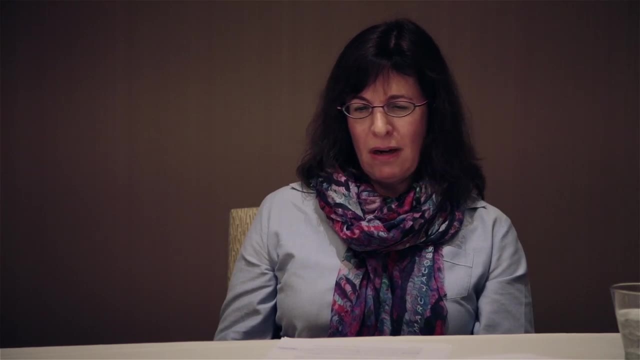 Like flowers and trees. Why can't flowers and trees be art? I think art has to be made by a person. he replied It just can't already be in the world. But numbers aren't made by people, So can they be art? 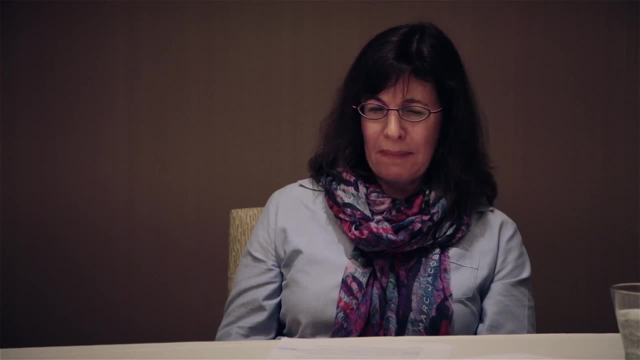 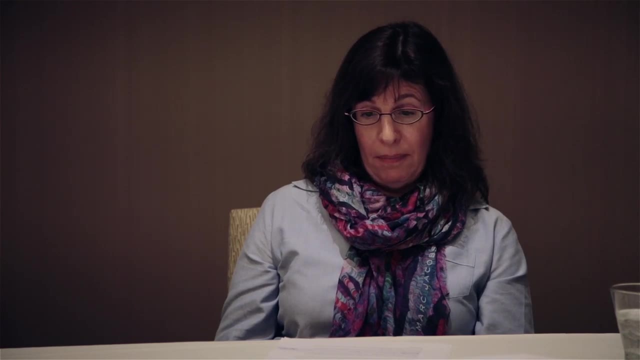 Maybe not, But they can be beautiful. So maybe something can be beautiful and not be art. But can it be art and not be beautiful, I wondered. I'm not sure about that one, Mom, But probably yes. I mean, I don't think rap is beautiful exactly. 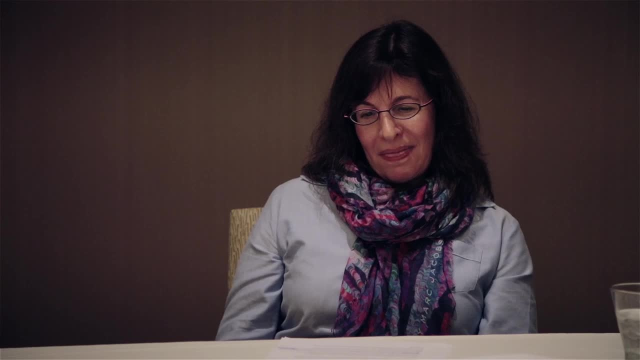 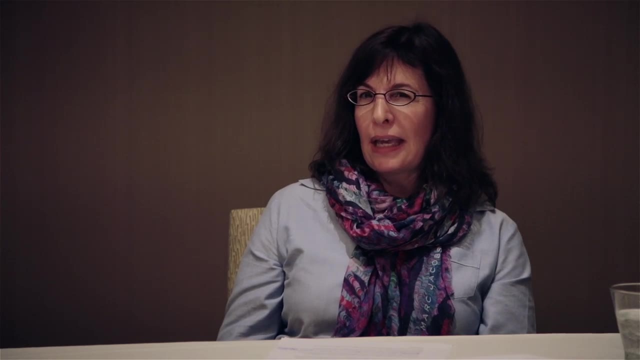 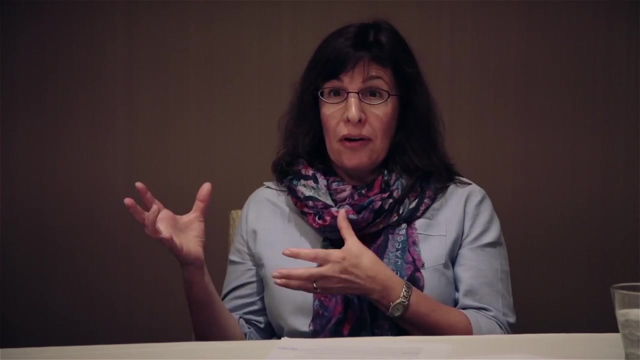 But I'd say it's art. So in talking about philosophy with kids, we play a different role, I think, as adults, than the one we ordinarily play in their lives, And perhaps that creates the tension between having to get out of the house. 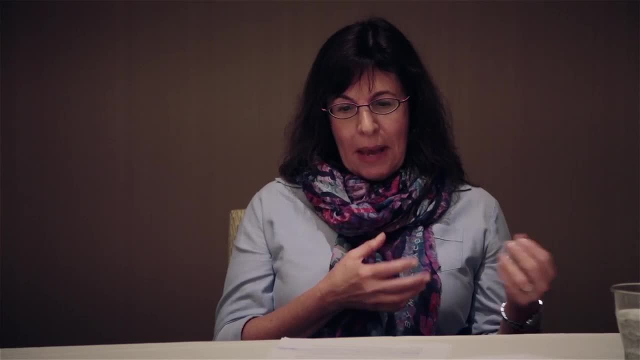 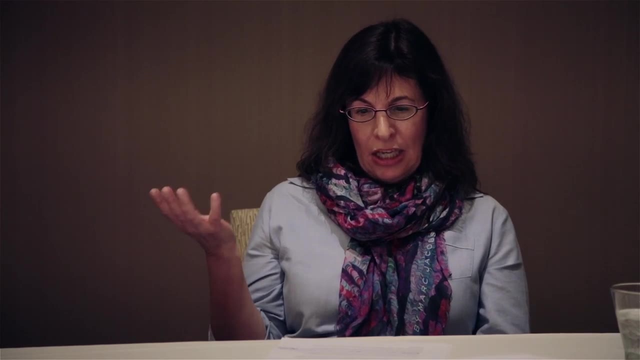 and wanting to have these kinds of encounters with our children, Because when we're doing, when we're trying to engage with them philosophically, be a kind of philosophical companion to them, our role shifts from the person who has to get us out of the house. 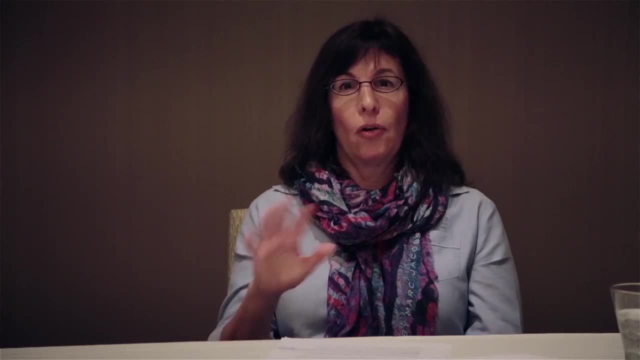 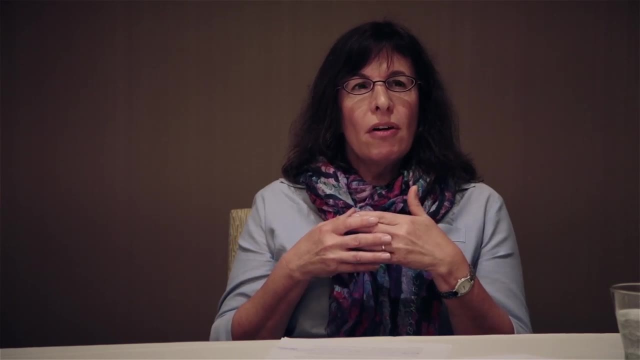 or has to teach you how to tie your shoes or make sure you eat right or whatever, to a kind of- like I say- companion, a kind of co-inquirer, And so we are way more equal in these exchanges than we are in many of the kinds of exchanges. 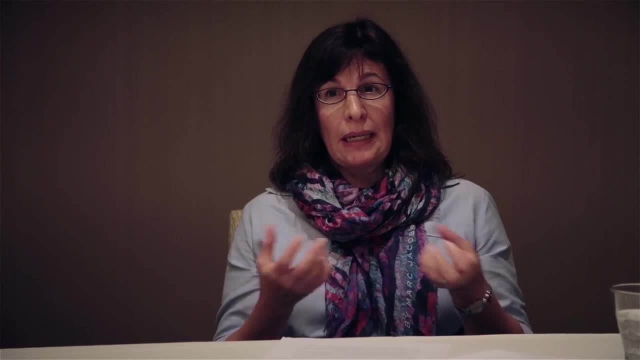 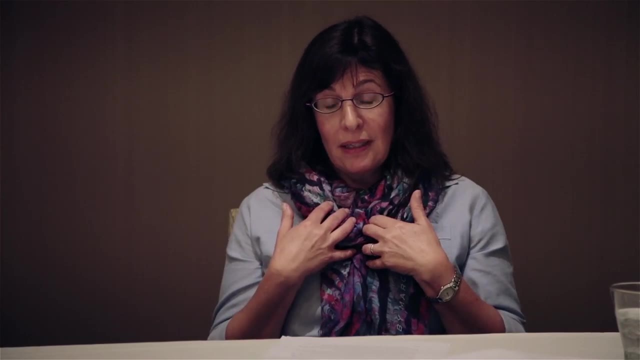 we have with our children, Because we're both bringing something unique and important to the enterprise, so that the enterprise would be much different if either of us were not involved. We, as the adults, bring presumably a greater conceptual sophistication, a longer life experience. 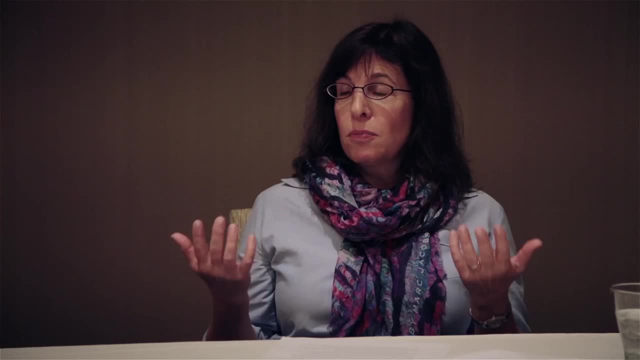 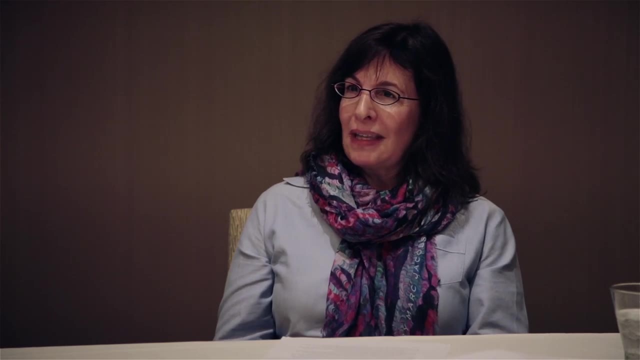 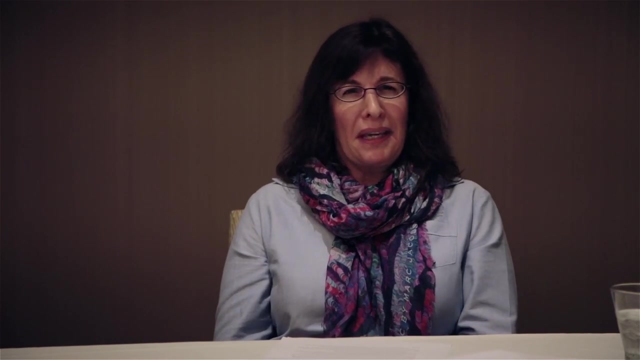 And children bring this fresh perspective, this openness to exploring all possible views, this kind of being newer in the world, and a playfulness. They don't take this as seriously, maybe, especially if we're philosophers, as we often tend to. For them, it's a playful thing to think about these ideas. 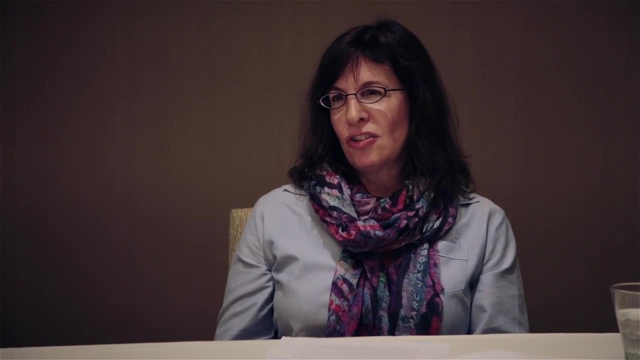 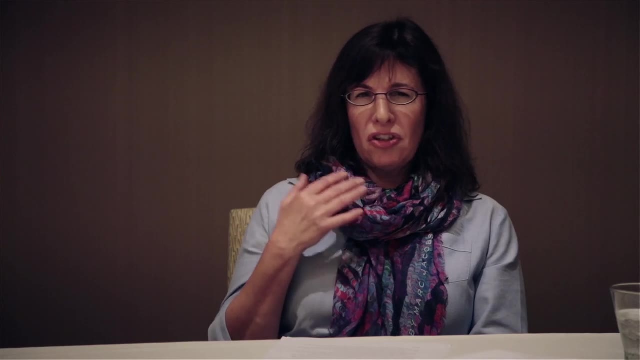 And so what? sometimes we characterize as children's naivete becomes a strength, because they're unafraid to think about a question imaginatively, to try out something that seems wild or different, And they're not as worried about making a mistake, particularly young children. 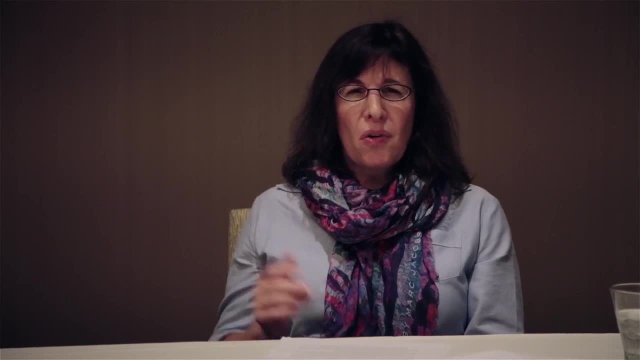 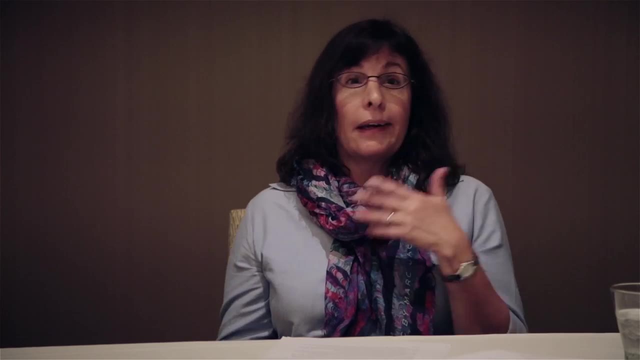 children, I'd say under like 11, not as worried about making a mistake or sounding silly as adults tend to be. They don't have to show how philosophically sophisticated they are. They could care less right. And so that conversation allows. 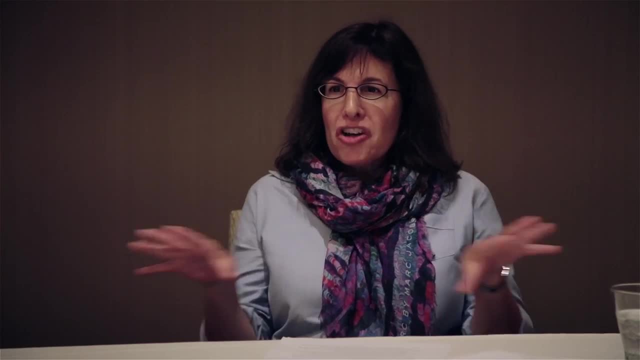 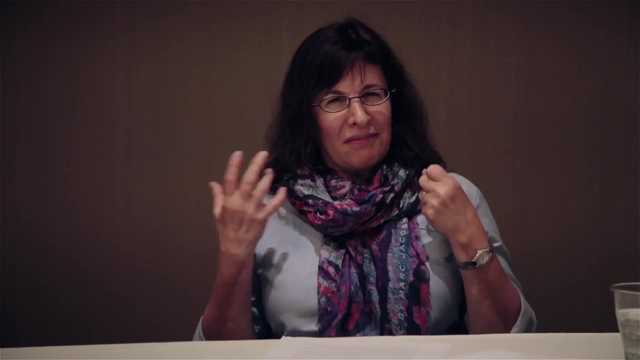 for kind of a depth and openness, because there's no posturing right, There's no some of the conversations that we have in the academy. I think sometimes can we just like say what we think really you know, And with children you're able to just do that. 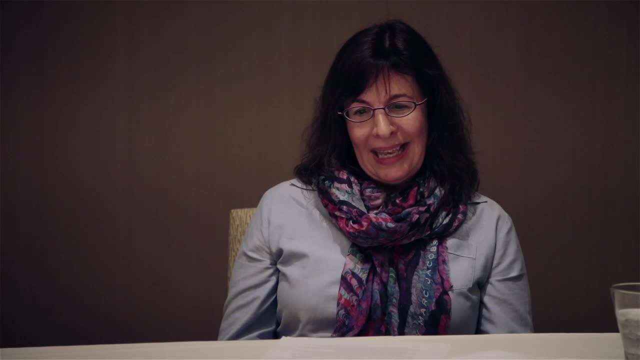 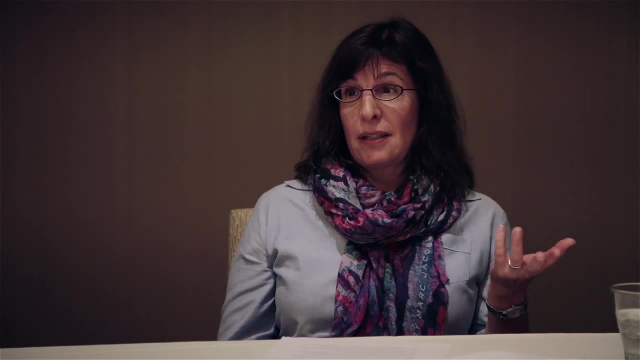 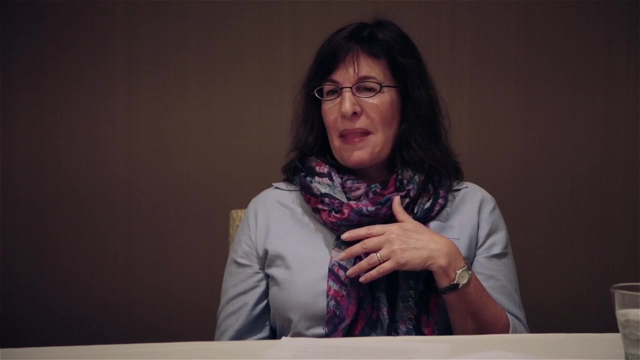 and there's something marvelous about it. So one of the ways that I found, as a parent, that I often engaged in these kinds of conversations was through children's stories And, as I've said before, it was a wonderful discovery as a parent to see how philosophically suggestive 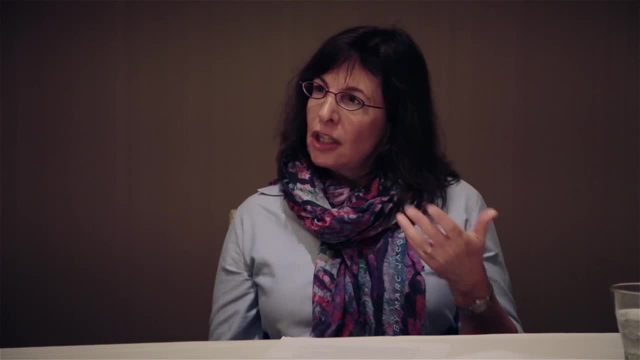 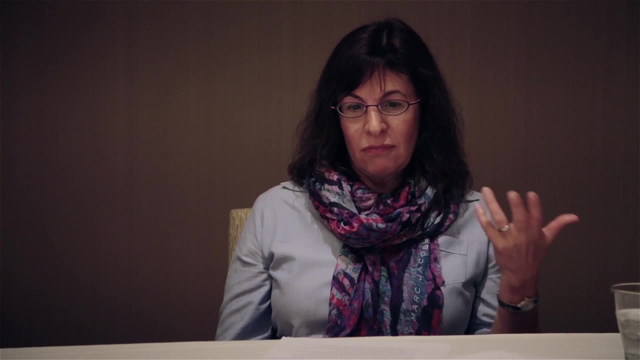 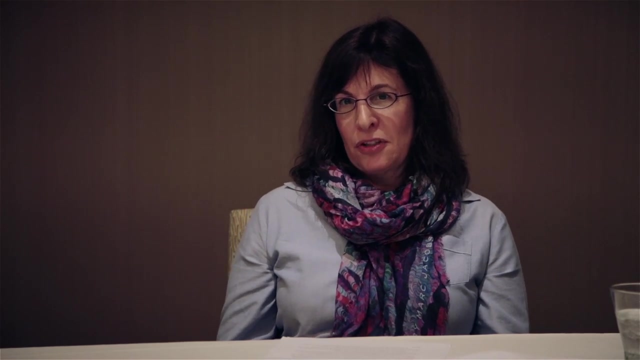 most good children's literature is, And it's clear to me that children's authors get that children are philosophically capable in a way that other adults don't quite understand as well. So here's one more example. Charlotte's Web was one of the stories that. 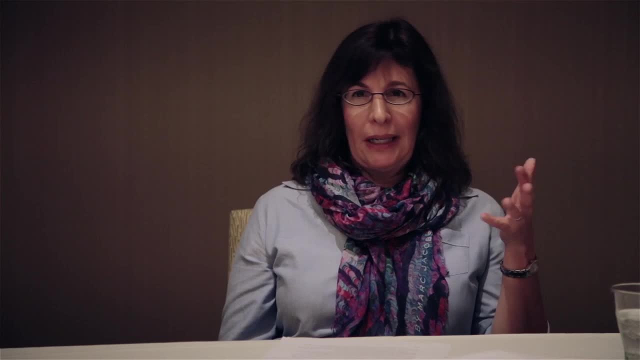 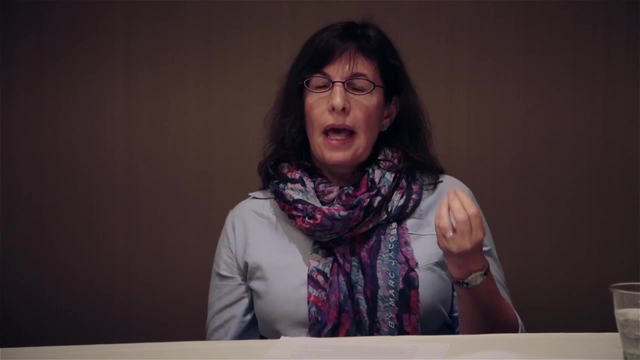 the books that I read with each of my children when they were probably around not quite ready. Death is a really important topic for them. They really think about death a lot. They want to try and they want to talk about it. They want to try and understand what it means. 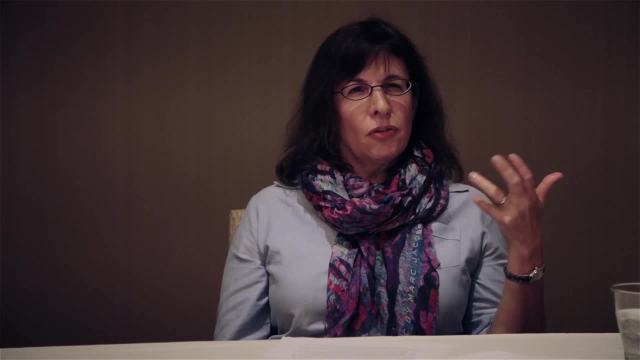 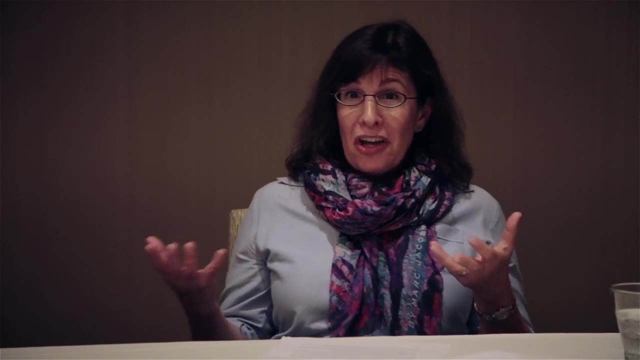 for their lives, that they're going to die, that the people in their lives are going to die, And adults are often really afraid of this topic, right, Really, really kind of we don't talk about it with each other very much. 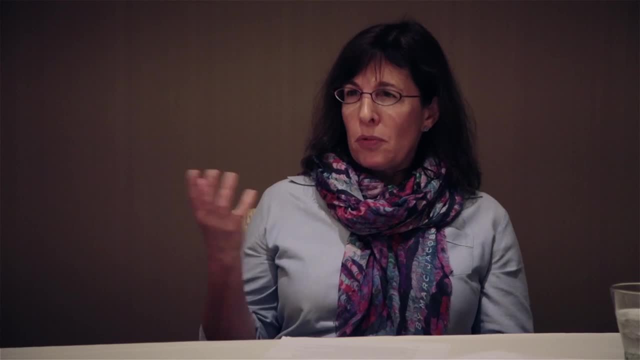 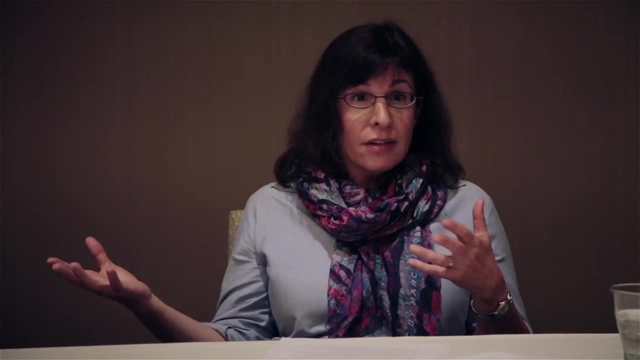 We don't really aren't really often comfortable. People will say to me: do you talk about death in classrooms with kids? You know, the schools let you do that kind of thing right, But about philosophy? and then we get sort of 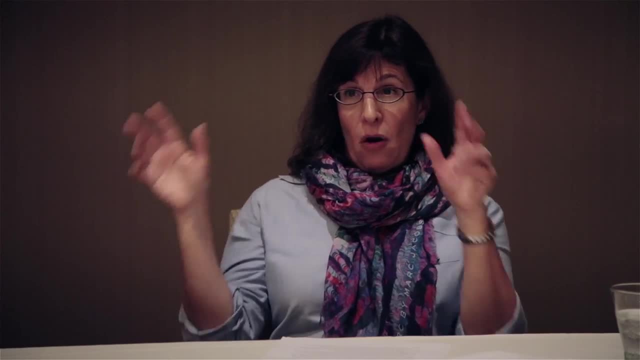 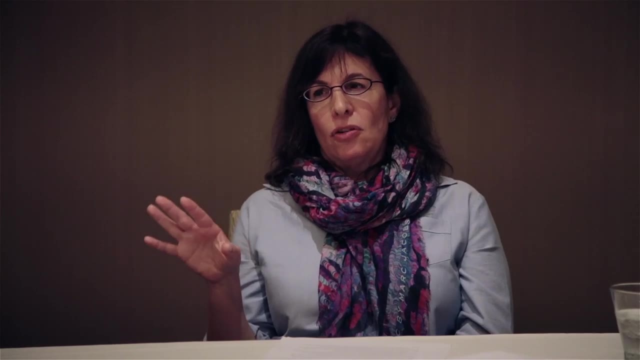 what are the questions you wonder about? In one class we have like a wonder box that they put in their questions through the week when I'm not there, And always many of the children ask questions about death. So, and I think maybe one of the reasons- 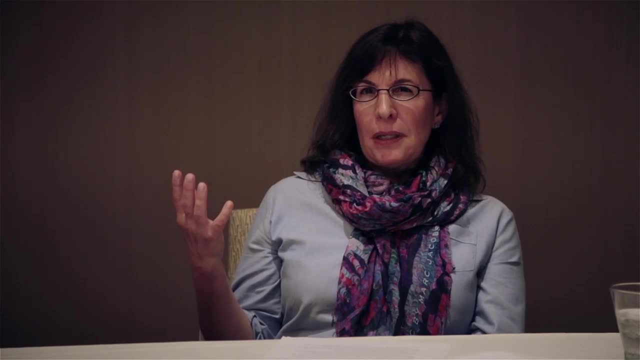 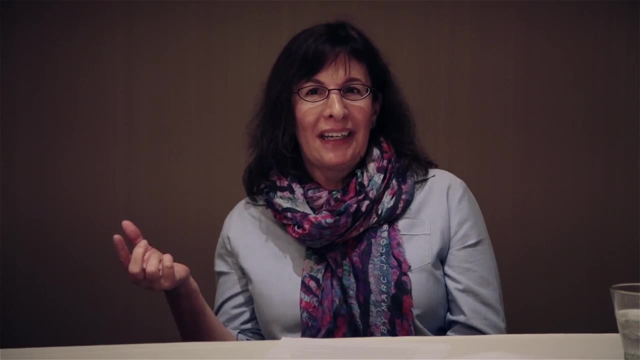 we don't want to talk to them about it is because we feel like we don't know what to say, right, We don't really have the answer, But that's actually the opening, right? I mean because it isn't that they want us. 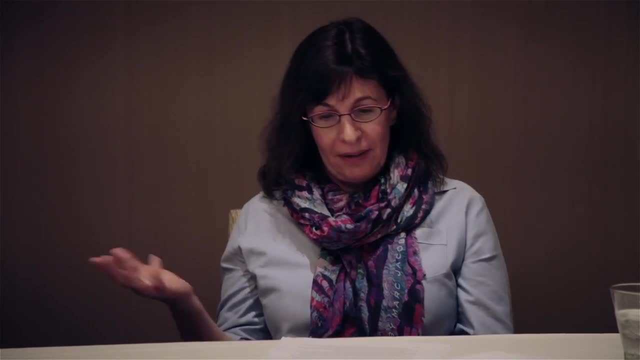 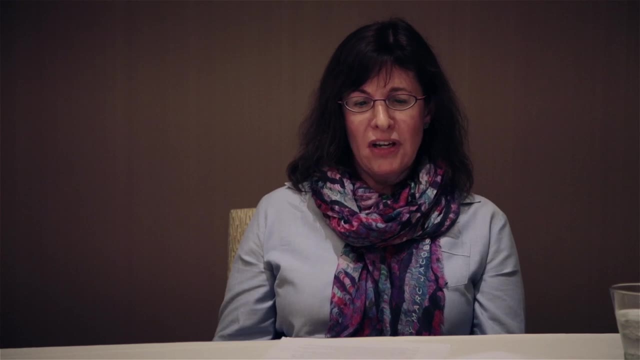 to talk at them about it. They just want to talk about it, right, They just want to think about it. So anyway, in this conversation with Will, I asked him if he thought that Charlotte lived on in any way, And he said: yeah, you know, maybe she did in a way. 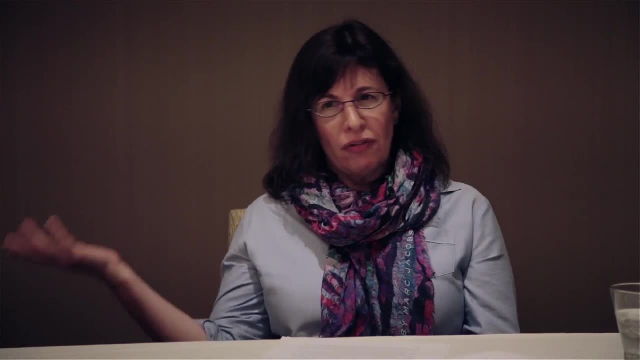 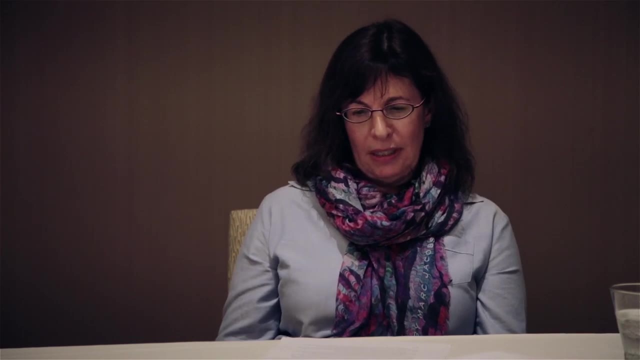 And we talked about how you know she could live on through her children and future generations of spiders. But he said: you know, but it isn't like she's still alive, It's just that something like her keeps living. And I said: what does something like her mean? 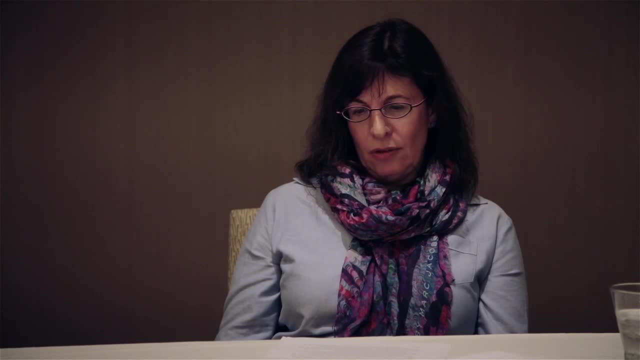 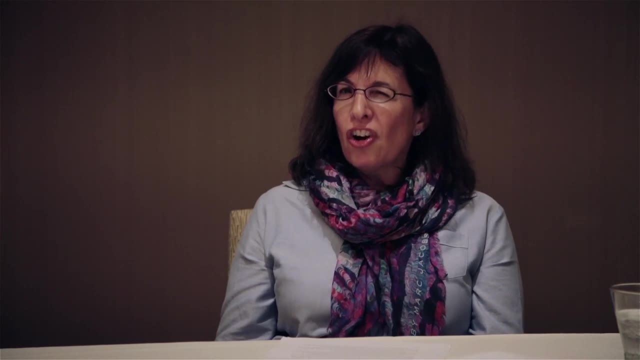 Well, maybe something like how smart she was or something about her like that. That's the same in some of her children And then maybe some of their children. But that isn't her, It's just the way she was. that then her children might have too. 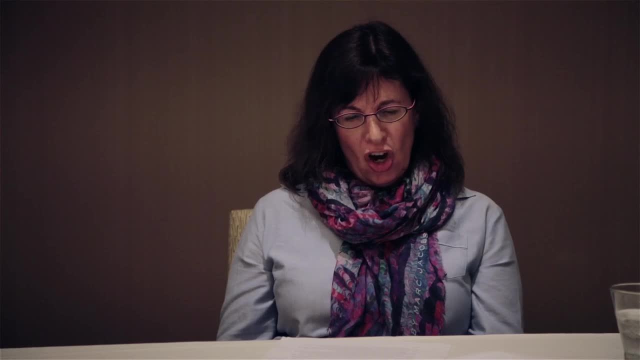 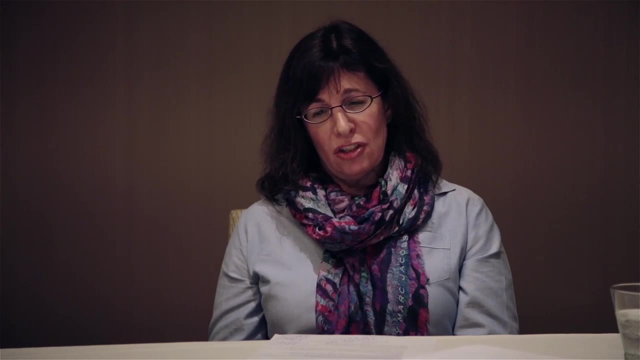 So when you say it isn't her, what would be her? Could any part of her be still alive? Well, her body isn't alive anymore. So is Charlotte her body. If her body is dead, then no part of her is alive anymore. 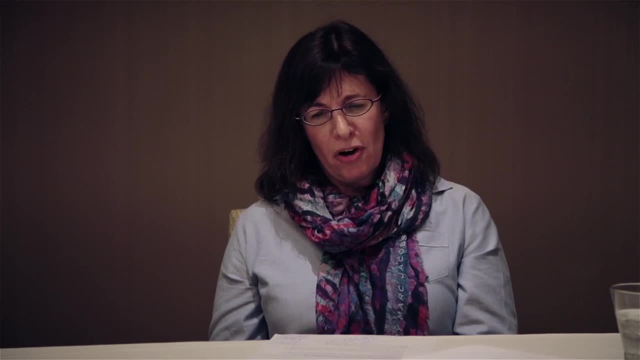 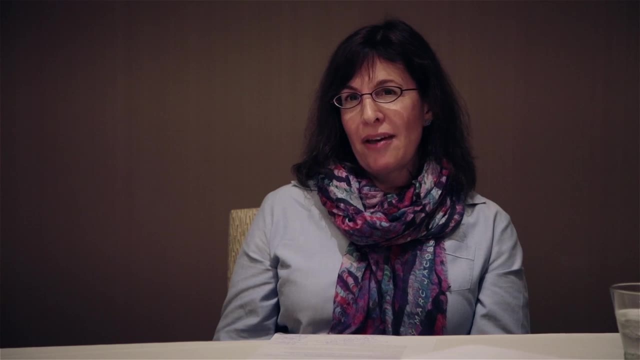 I don't know. I mean, yes, her body's dead, But maybe some part of her could still exist. So these kinds of questions, these kinds of conversations created, I think, for me now that my children are grown or close to grown. 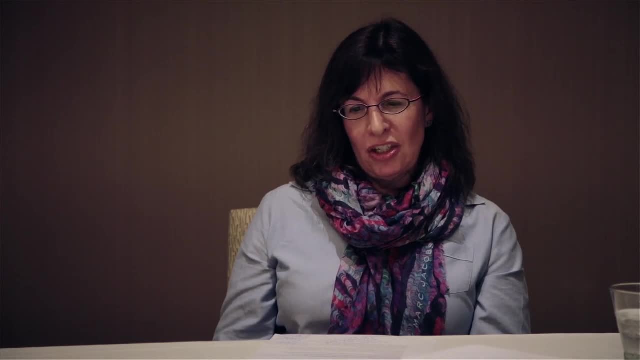 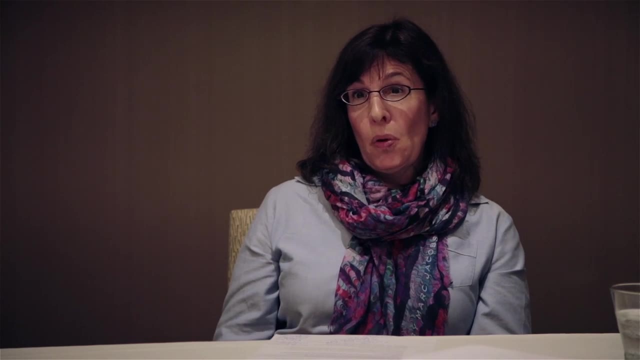 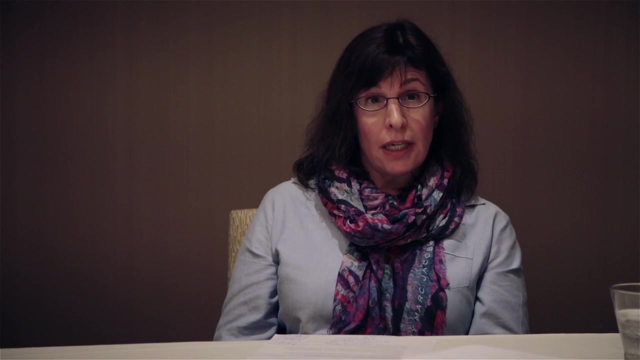 a really different dimension to our relationship. And I think now, looking back- and I mean their teenage years for me were really wonderful, I have to say. I mean I was sort of terrified of those years because I was really an awful teenager. 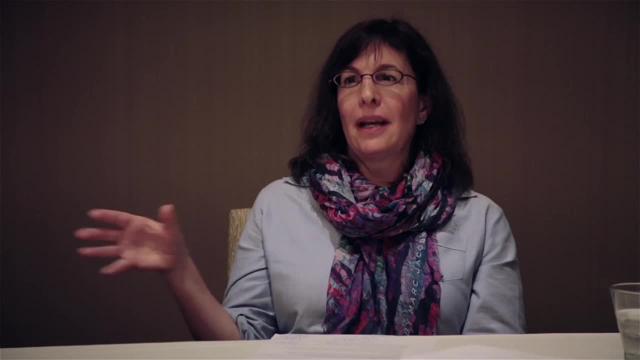 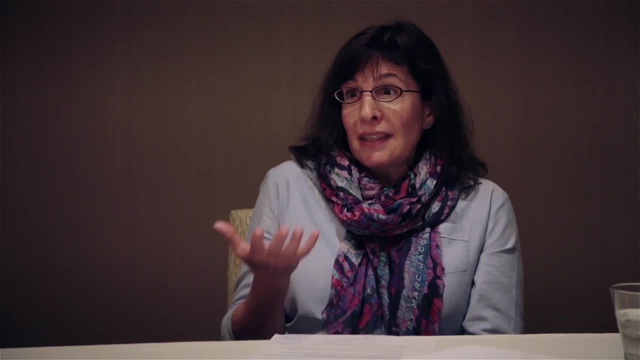 And at least I mean I say that because that was the story in my family, And I think back and I think, well, you know, so I don't know right why that was the way it was, But I was afraid that this would be. 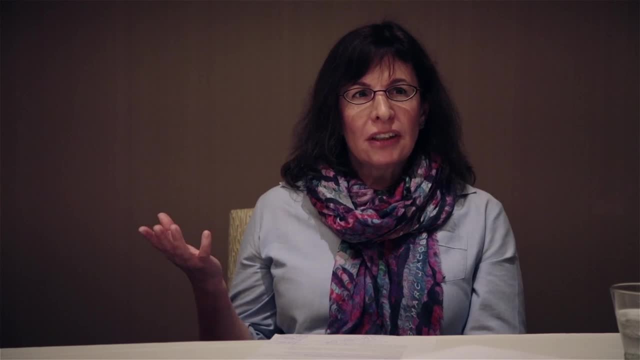 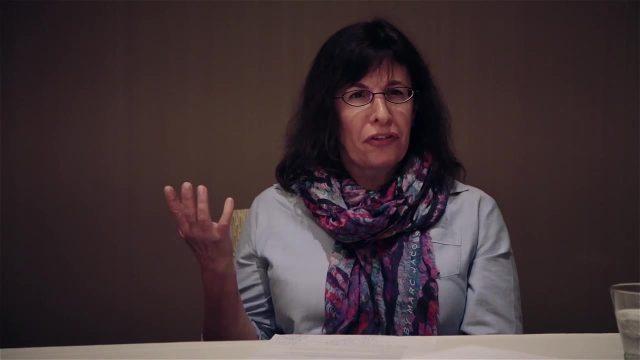 a very challenging time for me as a parent And it actually well, it certainly had its challenges. It was and is- as my youngest is 16, a wonderful time, And I think that part of the reason it's wonderful is because that period say: 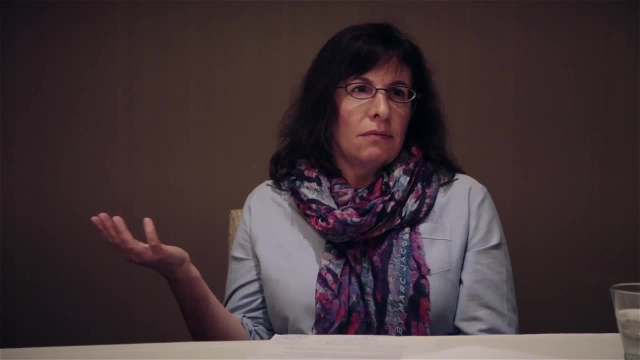 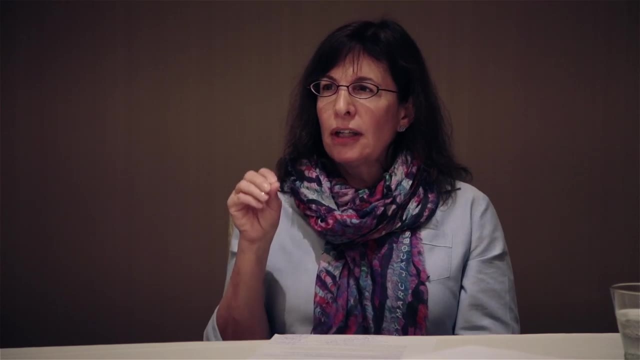 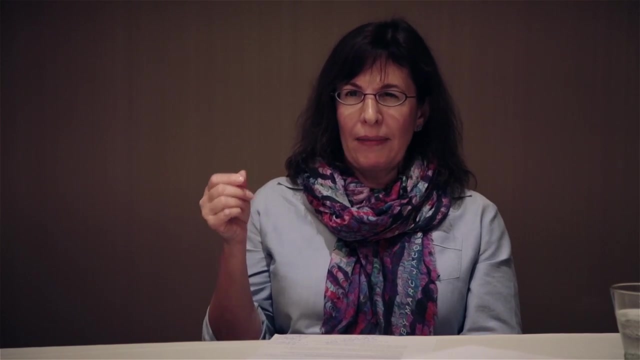 between- I don't know- 12 and 20, is when they are really kind of developing a critical consciousness about social practices, And so the way you live your life is of real interest to them, right, And they want to know. 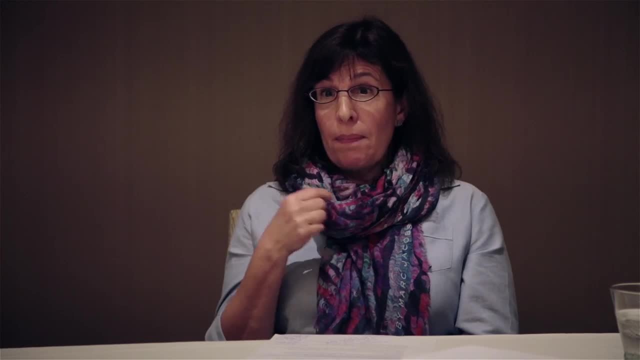 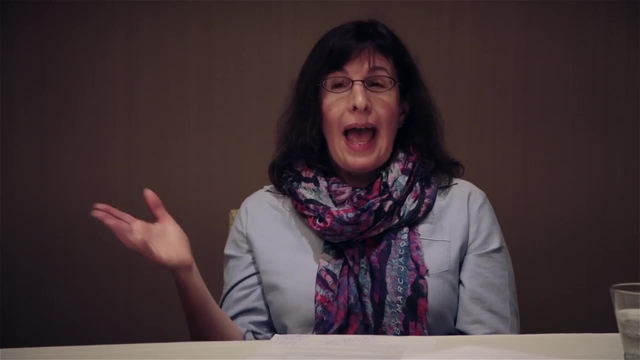 why do you do that? Why do you do that? And when I was growing up, that sort of unfolded in me being very critical of my parents, Like why would anyone live like that? And you know you're the right. 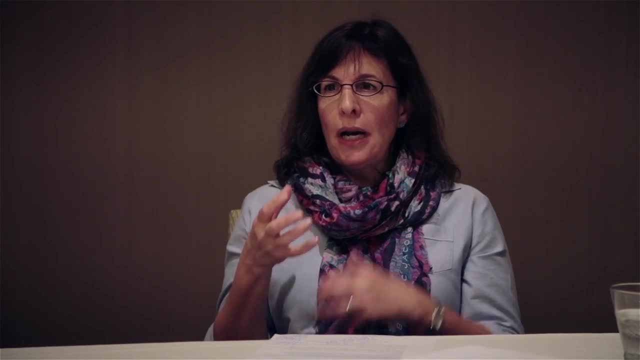 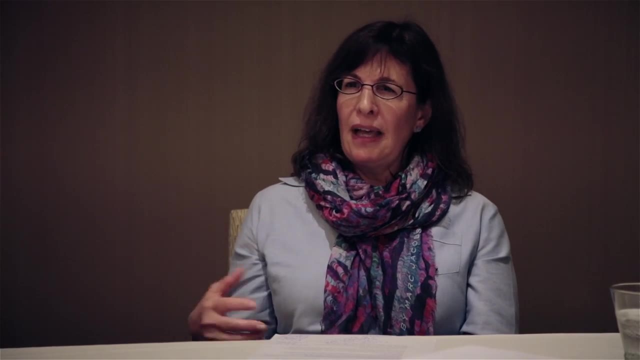 And, but with my boys it was much more. this dialogue. that was really. that was really wonderful for me. I mean, they would just want to talk about like: so why do people feel like they have to wear certain clothes when they go to females? 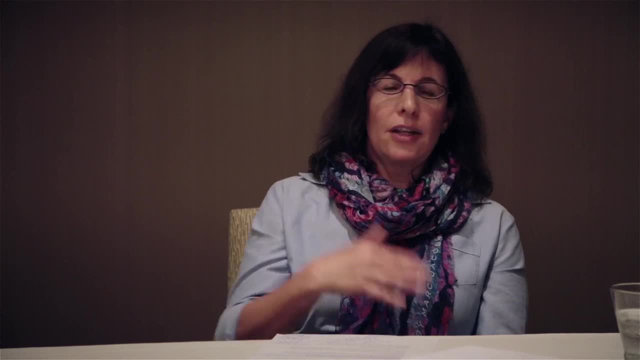 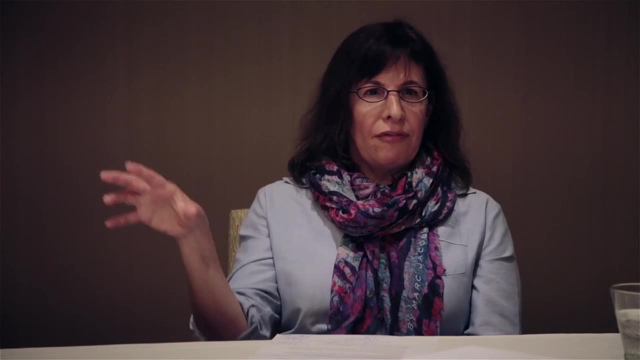 Or why do people look at people who are dressed a certain way and then make these assumptions about them? Or why- you know, what is it about family dinners that we have to do this in this way, Or whatever right? And instead of it being kind of 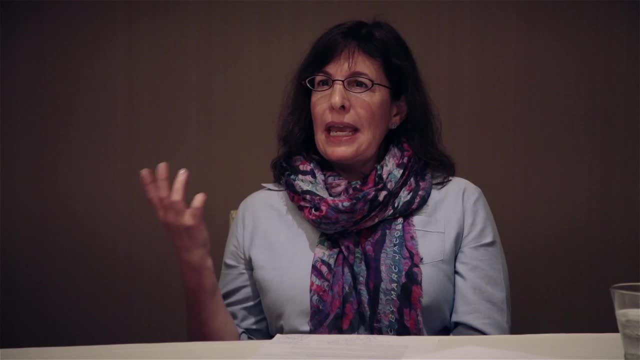 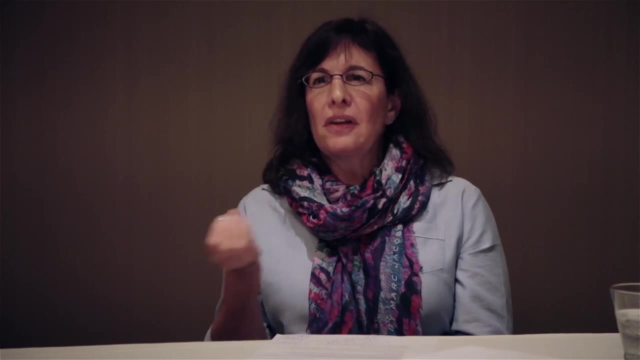 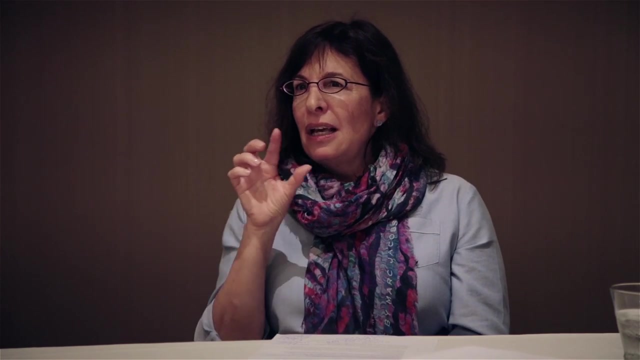 a conflict-ridden experience, which was what my recollection was. it was this really, really fun experience of like a lot of exchange about the world, And I think that part of it is that having these philosophical exchanges over a series of 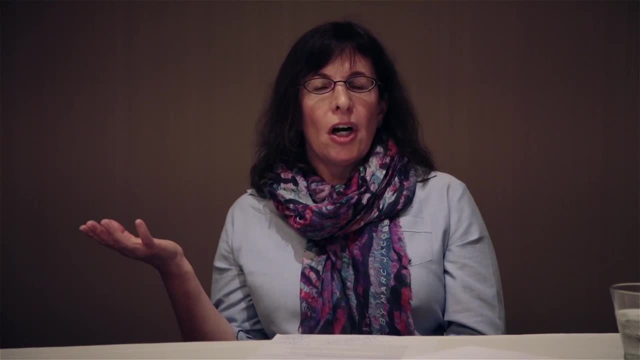 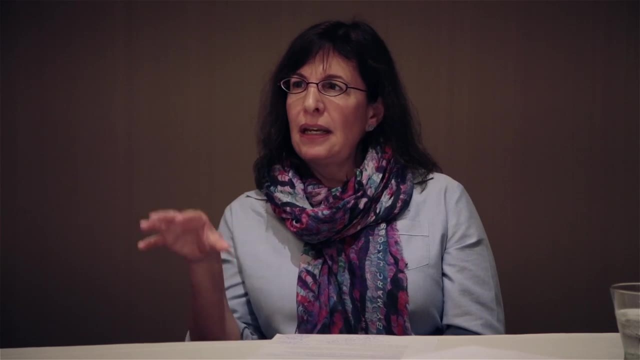 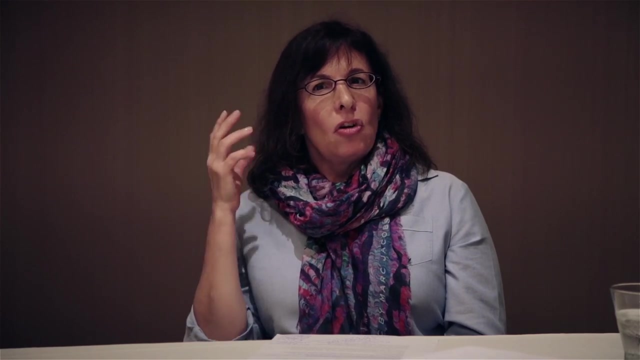 over the years of their lives, as long as they can remember, gave them the confidence that what they thought and said and the way they experienced the world and the questions they had really mattered And that they would be taken seriously. I mean, I remember when I was a kid. 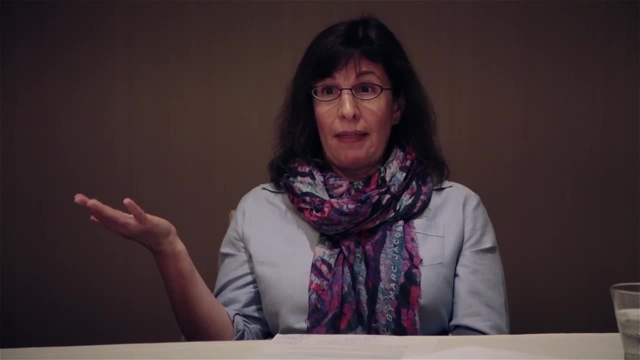 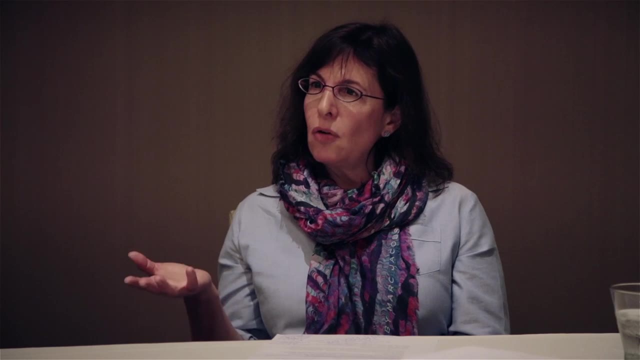 asking some questions and my parents laughing at me, right, And thinking, okay, that's not going to go anywhere, right. And my boys, I think, didn't have that experience right. They had the experience that when they had a question, 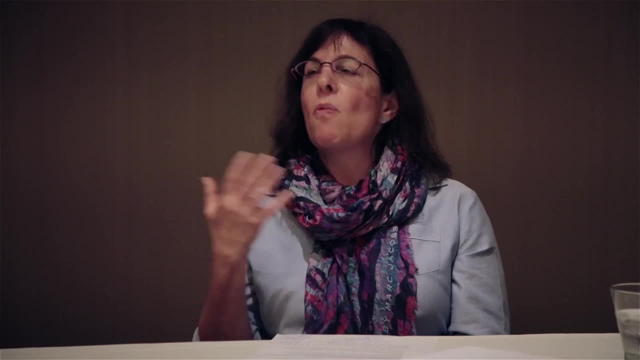 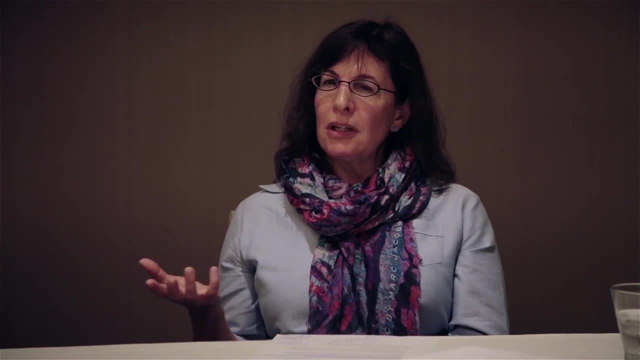 it was like it was taken seriously And they watched my husband and I grow up with them right. They watched us learn from them And I think that's a powerful experience when you're young: to see that what you say can change someone else right. 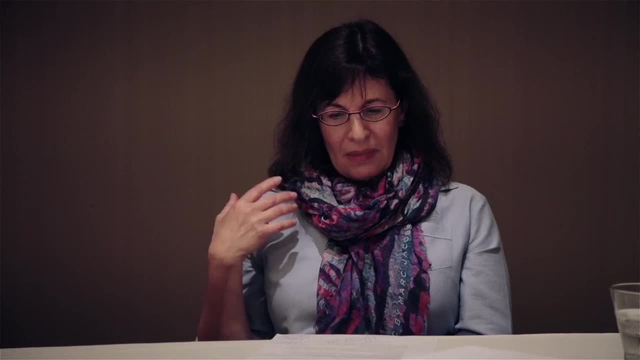 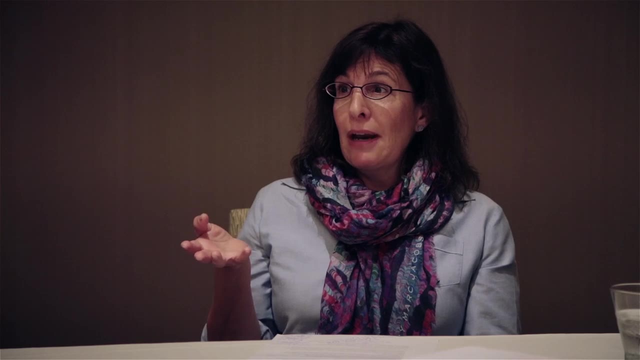 Can make someone think about something differently. So I guess I would say: maybe it wasn't philosophy that made me a better parent, I guess it's my children who made me a better parent, But philosophy was really a wonderful ally in that process. 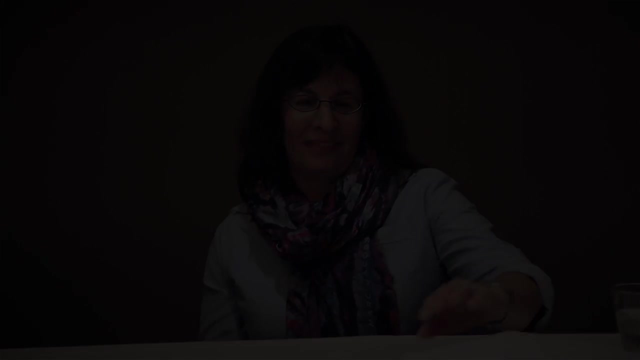 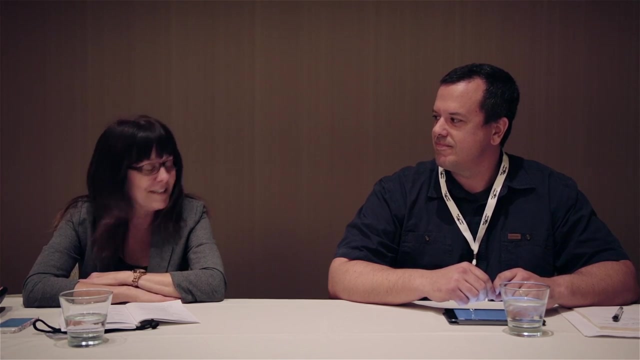 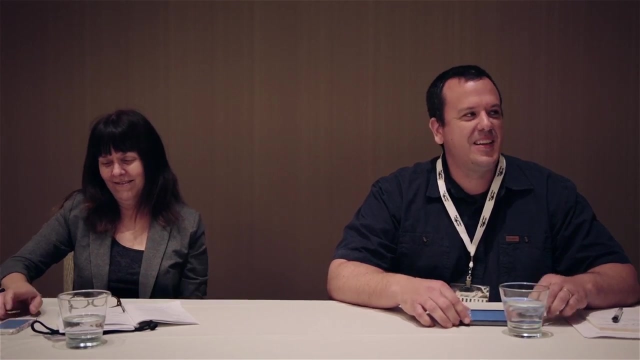 Thank you. Our next speaker is Kyle Robertson from UC Santa Cruz, And his paper is on, or his talk is on, learning with a philosophical toddler. Thank you. I wanted to thank Dr Morelone for inviting me to be here and for all of you to be here. 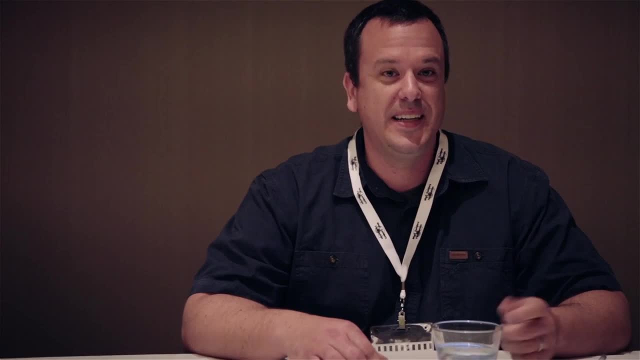 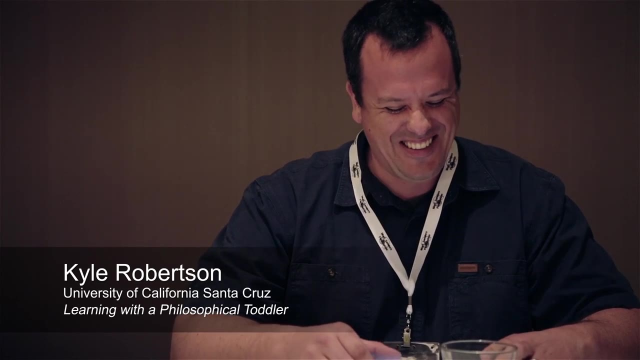 So I can talk about two of my obsessions in the last three years, which have been philosophy and my three-year-old daughter. So I'm going to be talking about much younger kids than Dr Morelone talked about. So I want to admit at the start: 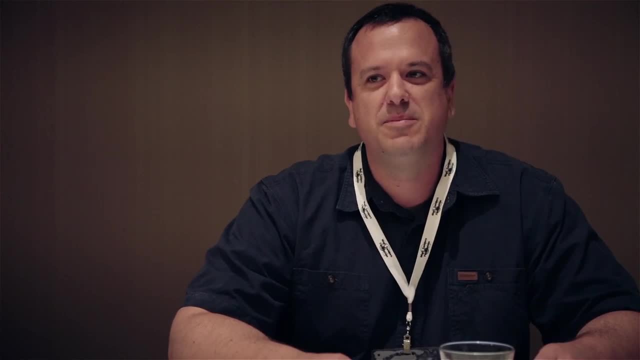 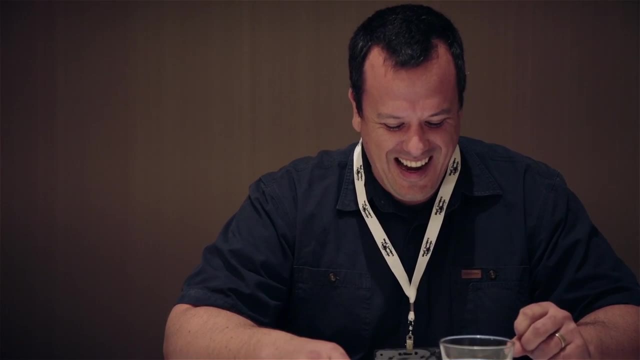 I'm not an expert in the topic of raising a philosophical child. My daughter, Zella, is almost three And that's not a crazy coincidence. It's the same Zella that's in Marcel's handout. Any success claim at this point. 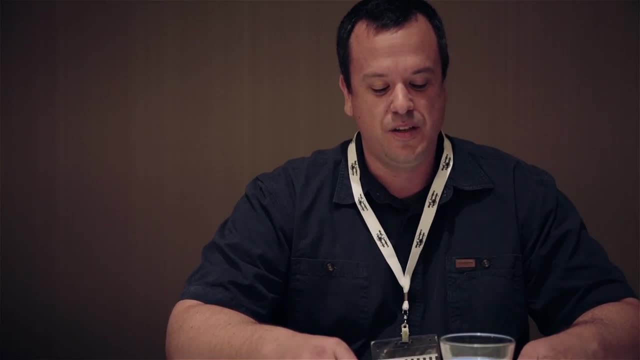 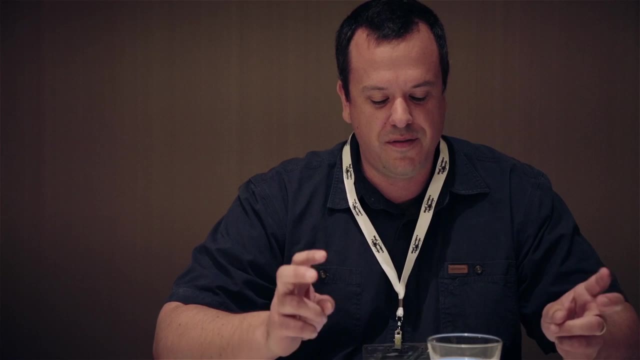 would be premature. I am, however, trying to raise a philosophical child, But in preparing for this talk, I wondered what the difference is between raising a quote philosophical child and raising a quote good or happy child. Every parent I know wants a happy child. 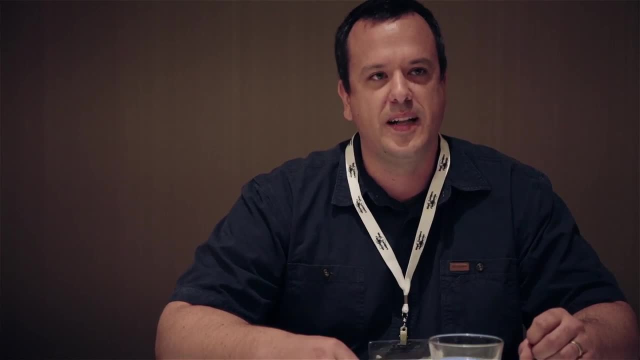 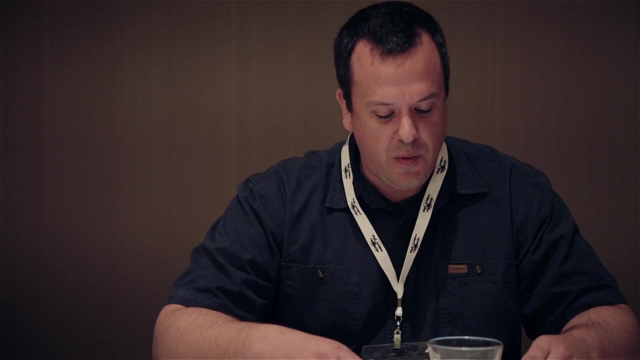 We often compliment kids and their parents by calling them good. What is it that makes a child philosophical? Is it something we actually want? And if it's something we want, is it something we can cultivate? Or are some children just naturally philosophical? 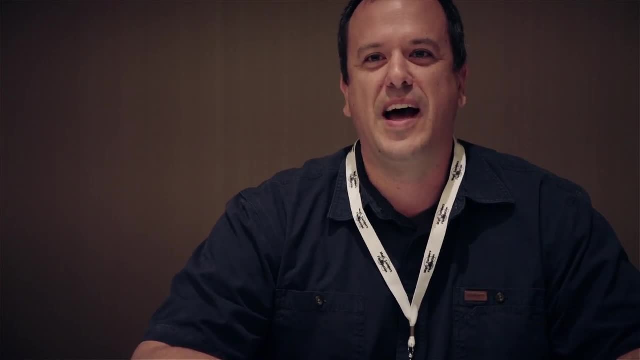 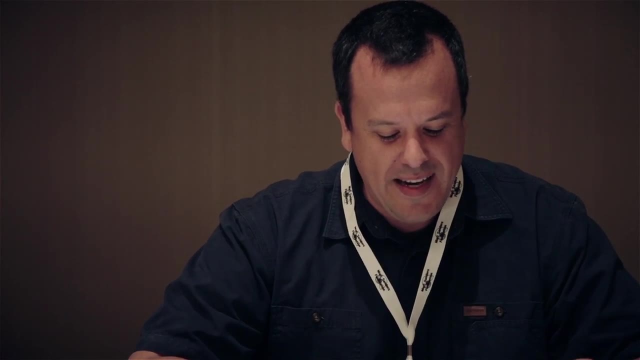 I thought of that recently when there was a website posted: Help My Child as a Philosopher. A group of philosophers, including Peter Singer, posted this To try to get clear on some of these questions. I'm going to talk today about episodes with my daughter. 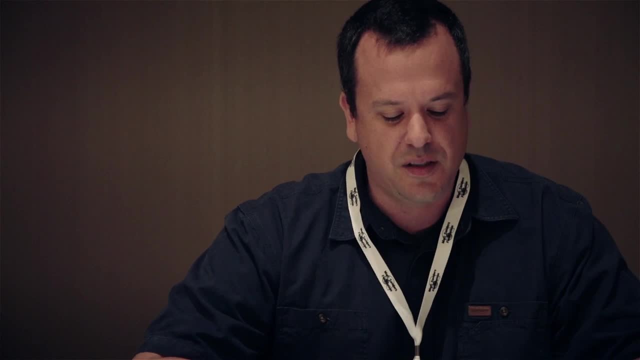 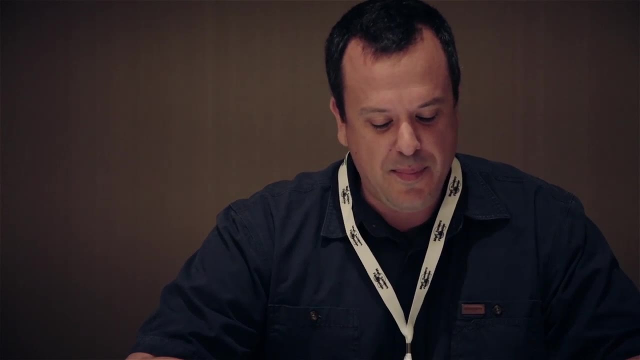 where there seemed to be a tension between raising a philosophical child and other norms associated with raising children. Through these episodes, I'd like to argue that thinking about raising philosophical children does add something to the notion of raising good or happy children. It helps us focus on raising children. 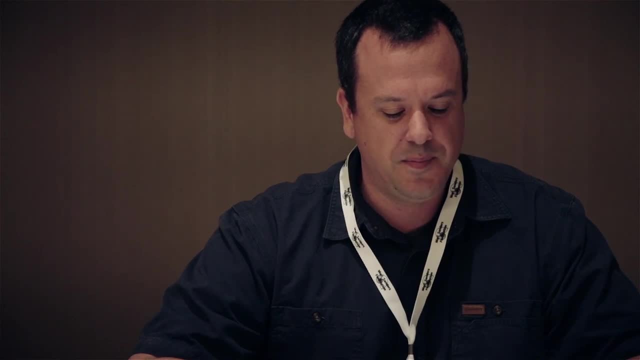 that have the agency to grapple with the world, as it is A basic sort of practice that I qualify as philosophical, is thinking critically about things that are generally taken, or supposed to be taken, as givens. It's part of philosophy to view conventional wisdom. 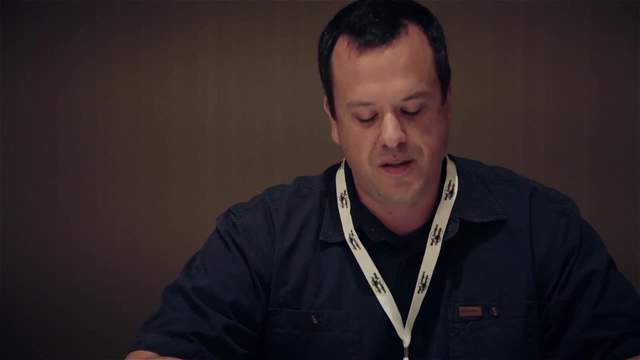 as open to questioning, And this is an attitude I certainly want Zella to possess, But it's an attitude that is sometimes in tension with how we relate to toddlers. There are obvious contexts where most people prefer their toddler not to be reflective or inquisitive about givens. 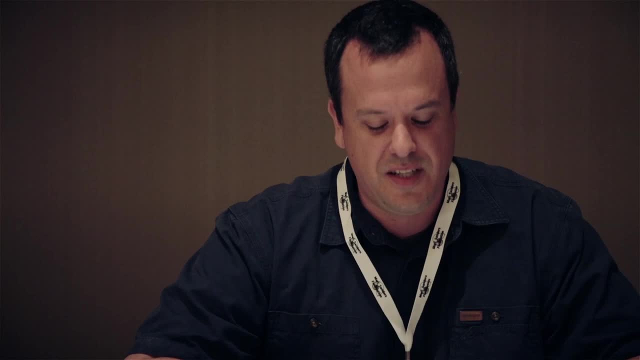 Some seem to me pretty clearly good times to limit inquisitiveness, such as when a rule of safety like don't run into the street, is involved. Some seem obviously bad times to limit inquisitiveness, such as when a parent limits a little boy's desire. 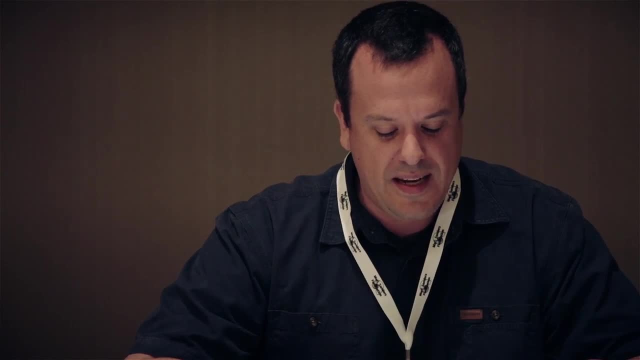 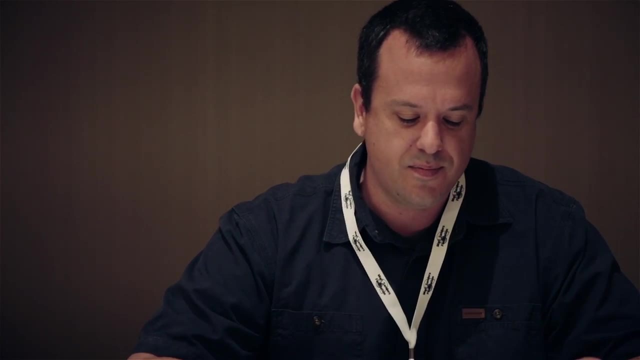 to play with dresses. I'd like to focus on one case where I will argue. thinking about raising a philosophical child might encourage us to change commonly recommended practices. So one of the pieces of advice circulated among parents, at least in Santa Cruz, California. 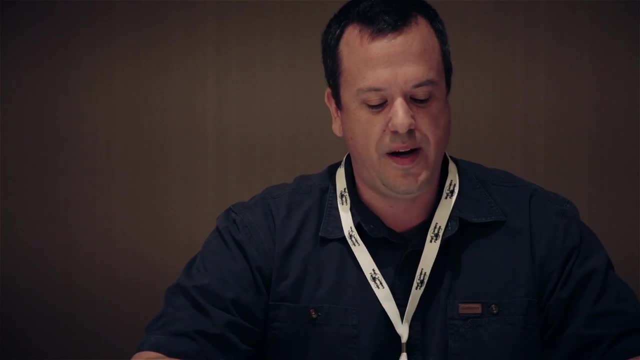 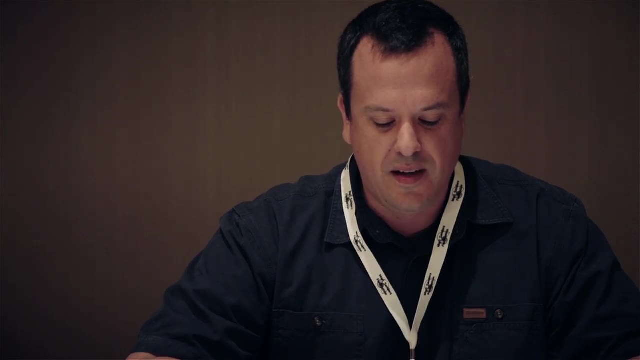 is that we ought to buy our children quote open-ended toys so that they can engage in imaginative play. We're told, for example, to buy simple colored blocks rather than branded dolls or stuffed animals. So a representative blog post says: quote active toys, make passive babies. 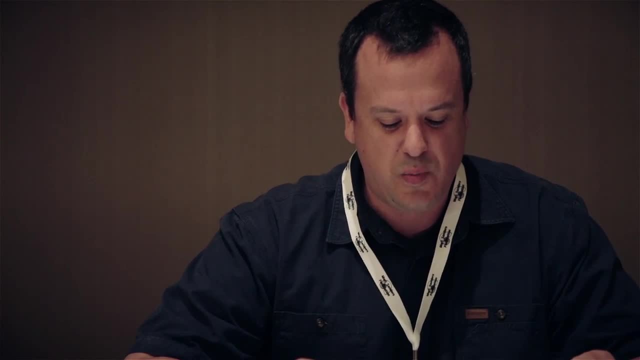 Open-ended toys don't do anything. They don't ring, They don't light up when a button is pressed. In other words, they don't play for the child. The child is free to do all the playing by himself, Even though they might seem. 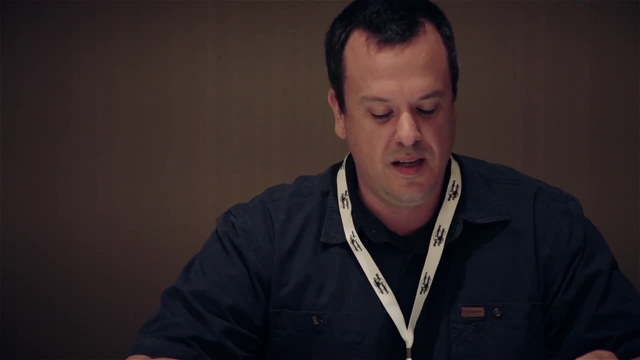 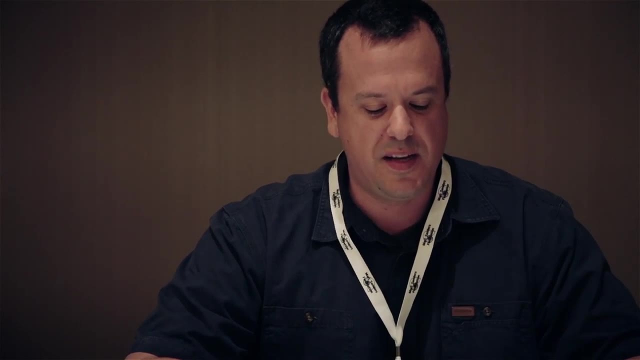 boring to some. to us they contain endless play possibilities. The more passive the toy, the more active the playing. How empowering for a child to know that what happens in his play is entirely up to him. Another passage from RIE founder Magda Gerber on a post. 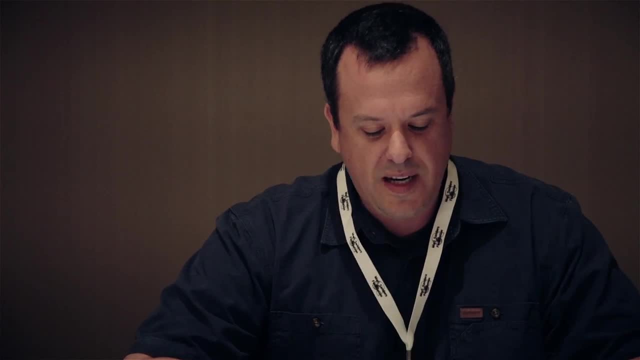 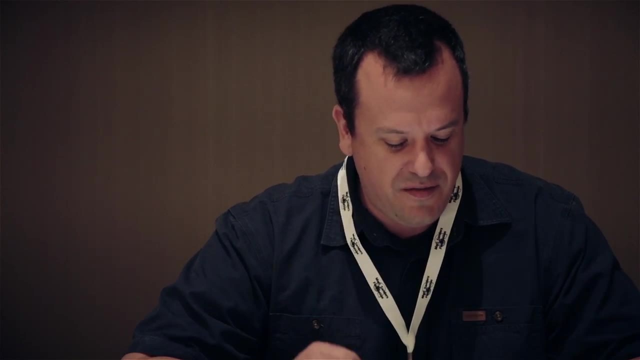 on recommended play objects. She says: what do all of these recommended play objects have in common? None do anything. They will only respond when the infant activates them. In other words, our active infant manipulates passive objects. In contrast, entertaining kinds of toys. 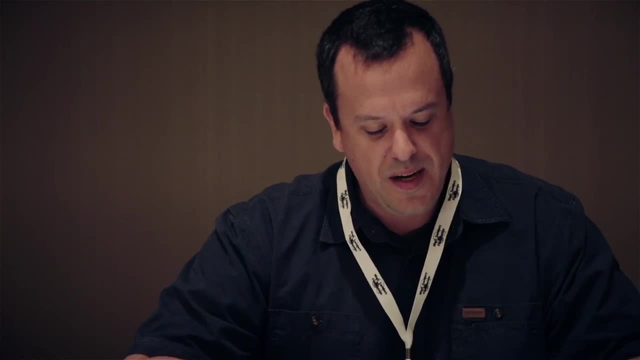 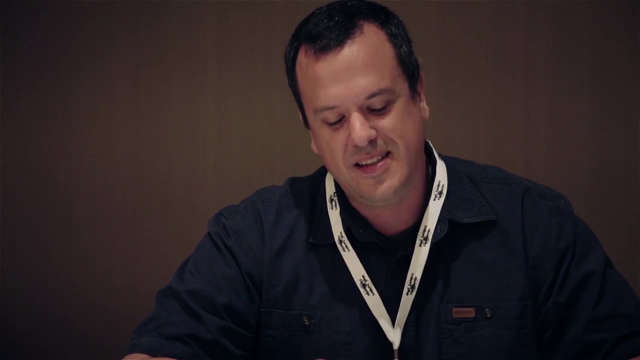 such as mobiles or, later on, wind-up toys, cause a passive infant to watch an active toy. This trains the child to expect to be amused and entertained and sets the scene for later TV watching. So Gerber uses the term infant, but in the post she was talking. 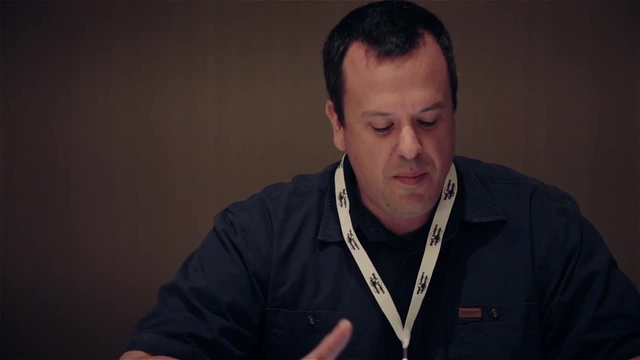 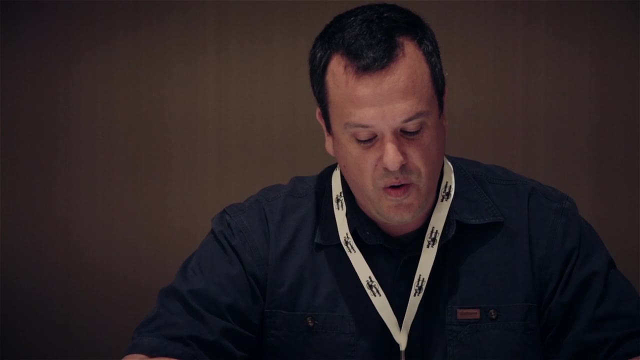 about toddlers as well. So there are many things to say about toys in play, and there may be many good reasons to give children simple, open-ended toys, Not the least of which is that noisy electronic toys often drive the parents crazy. But I think the reasons given 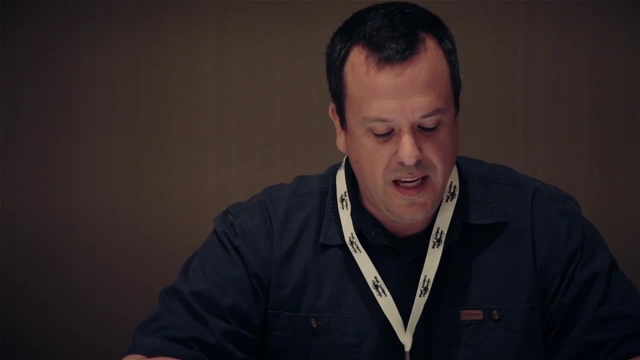 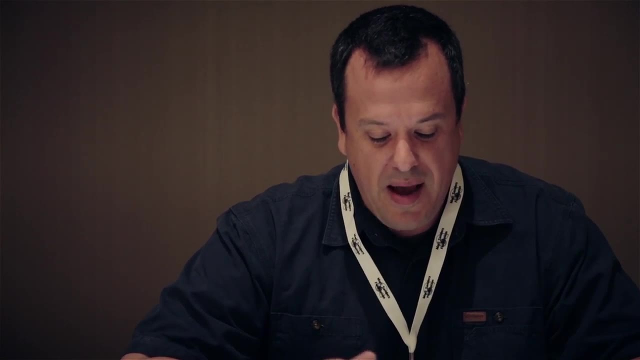 in these passages are wrong, And thinking about our children's philosophical capacities helps us to see this. The blog post claims that simpler toys will allow children to play imaginatively and self-directedly, rather than having the toys quote, play for them. Gerber claims that toys 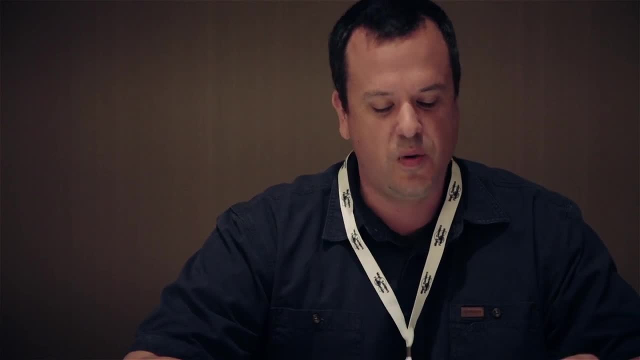 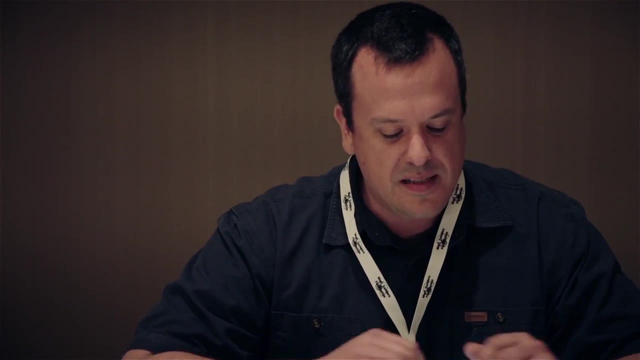 that move on their own quote, cause a passive infant to watch an active toy. It certainly seems true that active toys can be interacted with passively, but Zella seems to play freely with anything that I give her, whether it lights up or not. 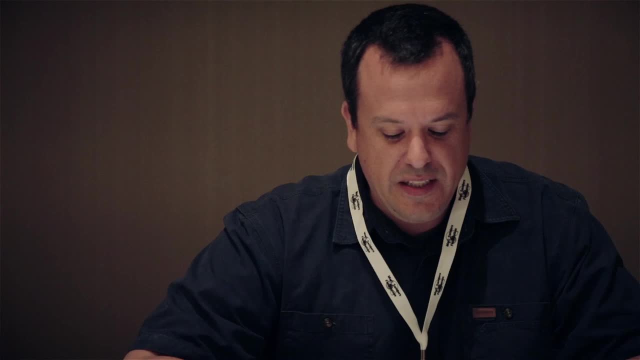 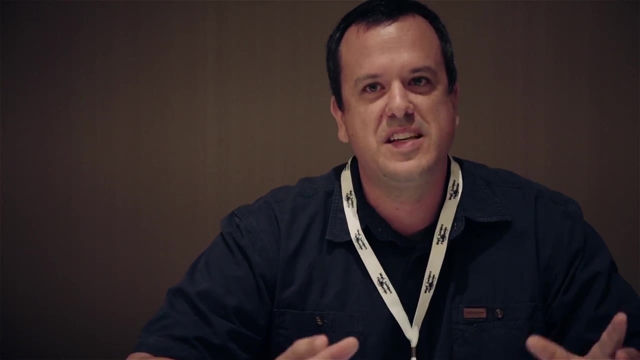 She uses it for her purposes In one of my favorite early videos of her, because, of course, we video everything that she does. she's about 14 months old and she's standing at one of those Fisher-Price plastic tables that light up and have a ton of different. 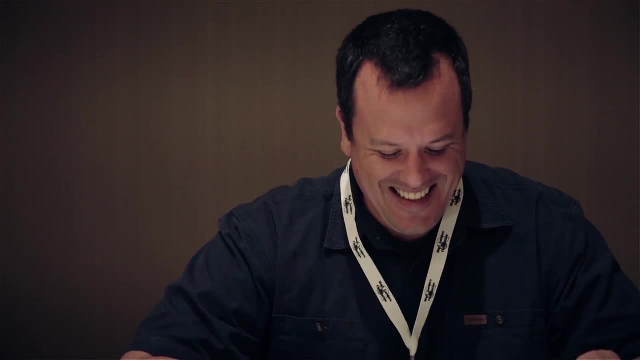 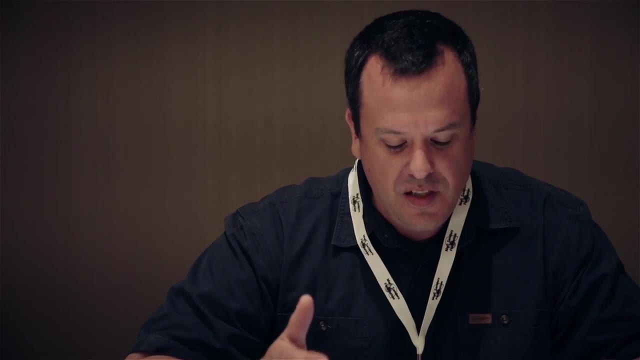 sounds and songs. Right, yeah, it's all the parents. It's exactly the sort of toy I think that these posts are objecting to. But what she doesn't like is that. what she does in this video is she is obsessively pressing. 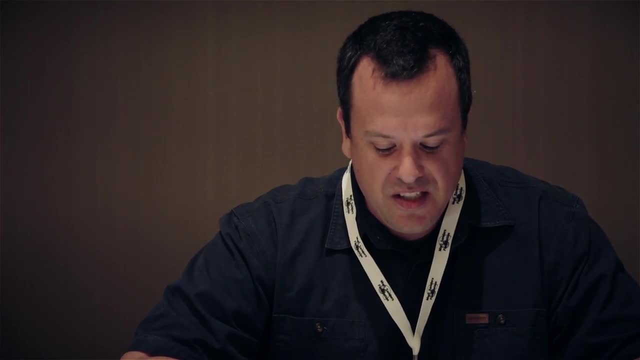 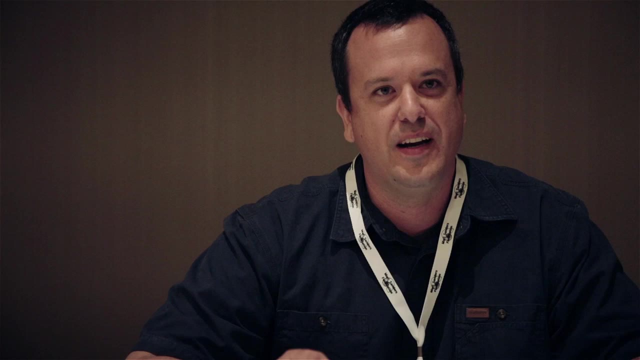 actually two buttons so that she can dance to her favorite song. So she gets really annoyed when it plays a different song and she figures out how, exactly what sequence of buttons it takes to get it to play her favorite song. And that wasn't trivial. 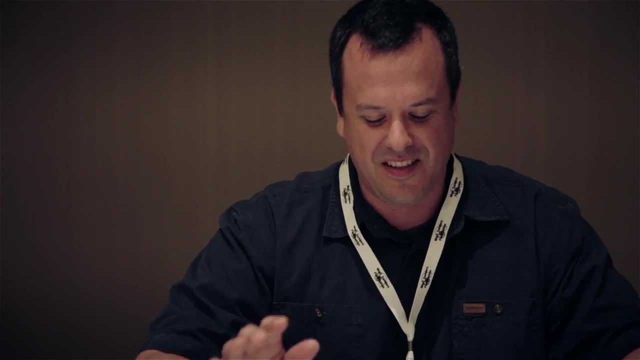 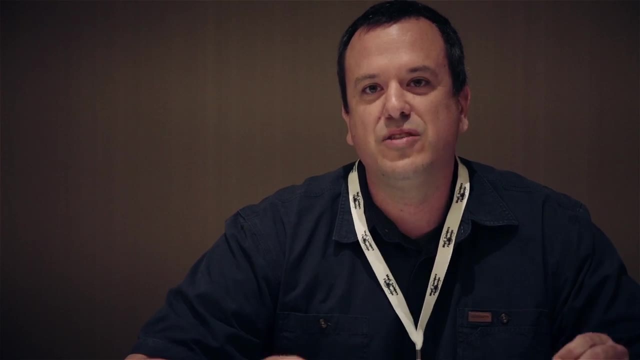 It was about seven different button presses. You know you had to cycle through the songs to get the song to quit. Another example: Gerber in particular discusses how active toys set the scene for later TV watching. The idea, I guess, is that active toys 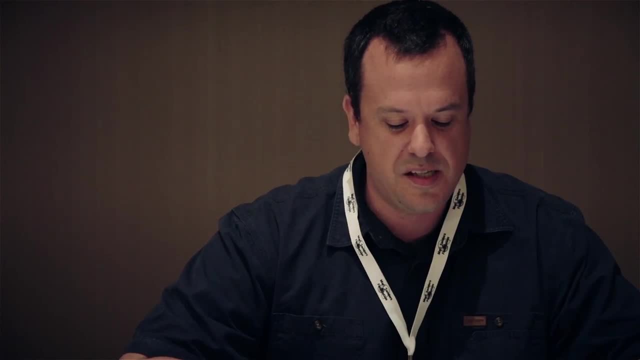 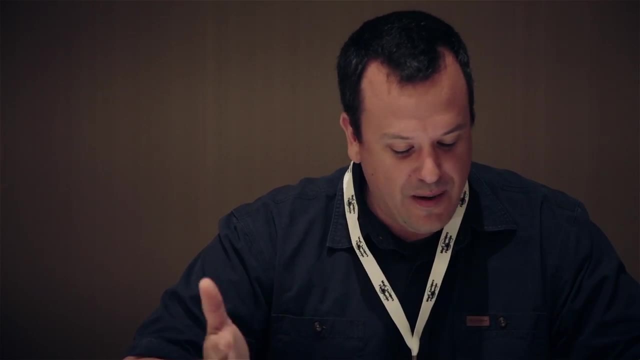 habituate us to passive patterns that fit passive TV watching, But the causal link seems weak. Zella has grown up in the age of touch screens like my iPad. Every parent we know, every parent she knows, has a smartphone and an iPad, And from the ages. 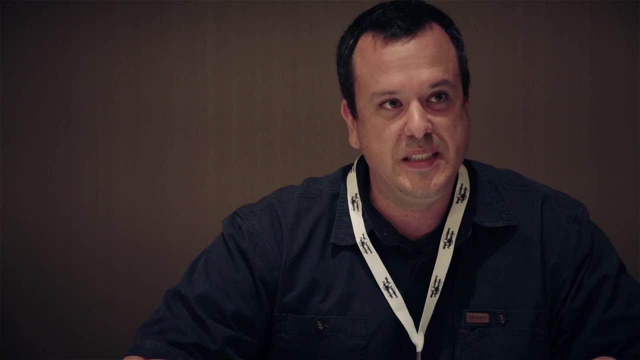 of one to two. we had to keep Zella away from big screen TVs, therefore. She did not seem to comprehend that you couldn't manipulate them by touch Right. She learned that screens are for interacting, not for watching. Big screen TVs were not safe. 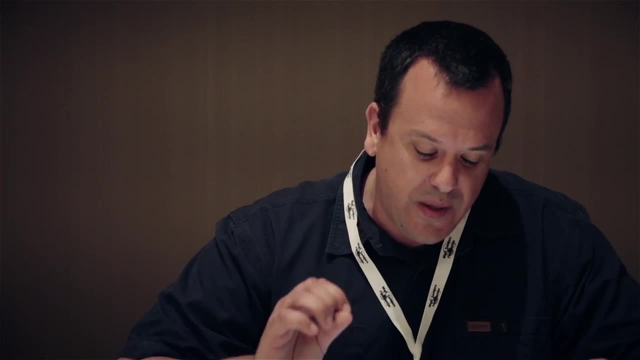 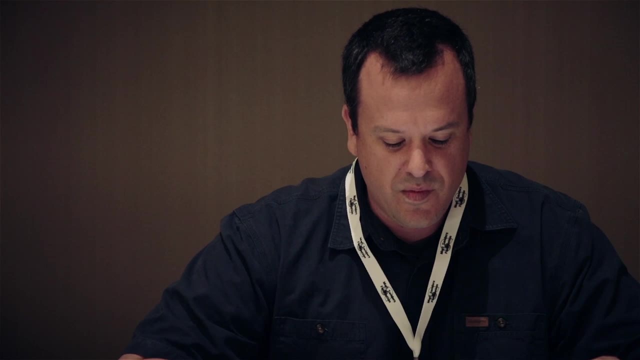 as long as they were within her reach. And she quickly, but also she quickly- lost interest in non-interactive TVs. So if a TV was just showing her something and she couldn't do anything with it, she got bored, She walked away. 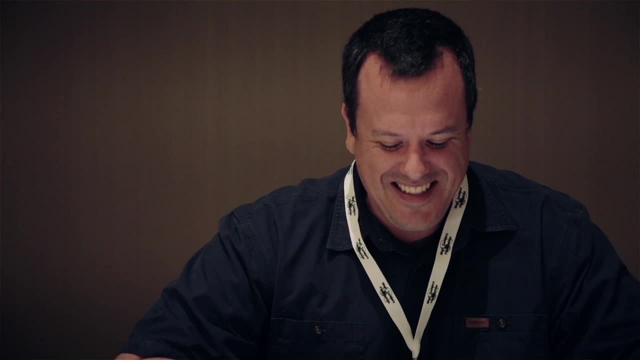 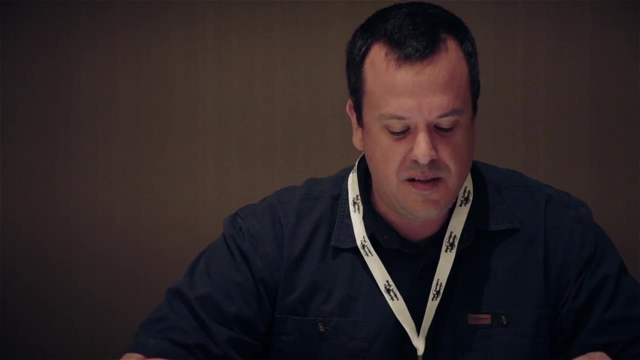 I do not mean to accuse the open-ended toy lobby, if such a thing exists, of ludditism, Though I think a dislike of technology is probably at least the partial motive for some of this. So I want to use a simpler example. 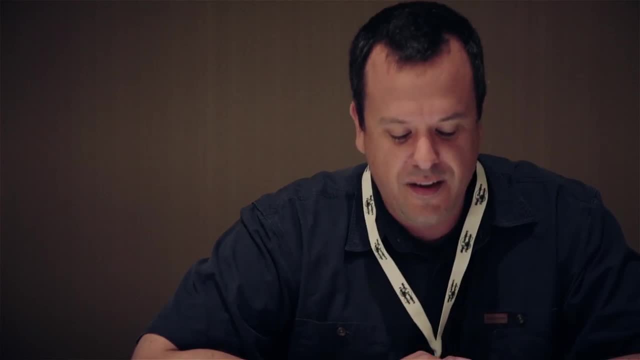 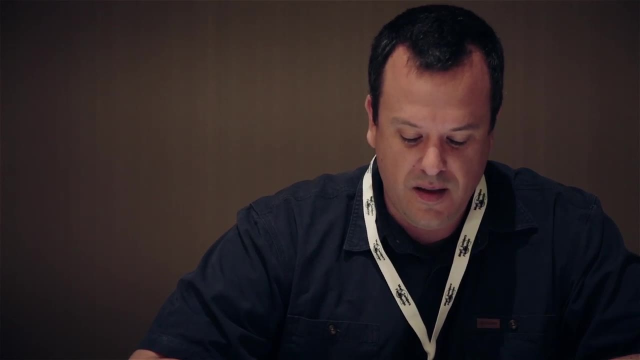 to help illustrate my point, An object that Zella regularly plays with that has a standard, culturally dictated interaction pattern is a book. I doubt that books that open-ended toy advocates have in mind is a bad toy, although I think that books not so long ago 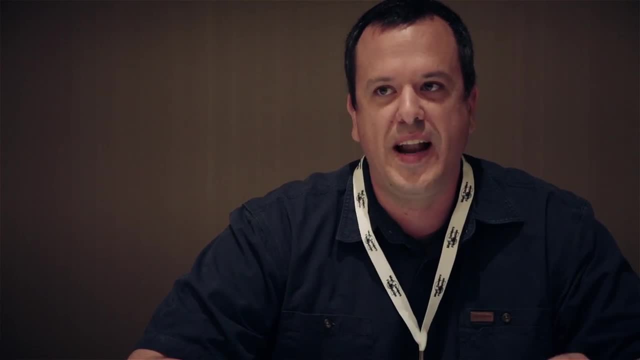 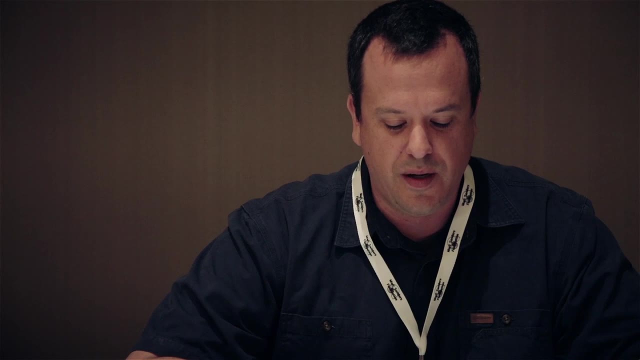 played the role that TV and electronics often play now in taking children away from more natural play. Regardless, books have a fairly obvious and correct manner of interaction: You sit and watch while an adult reads you a story, or read them yourself, once you learn how. 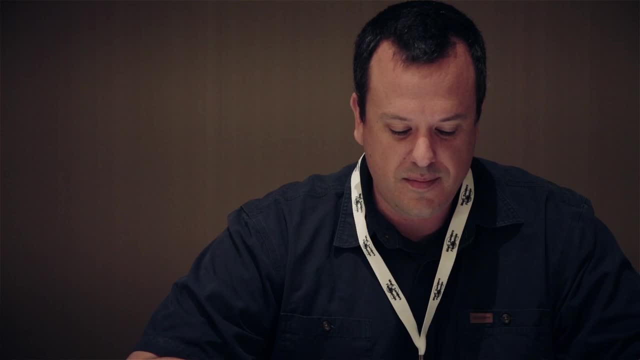 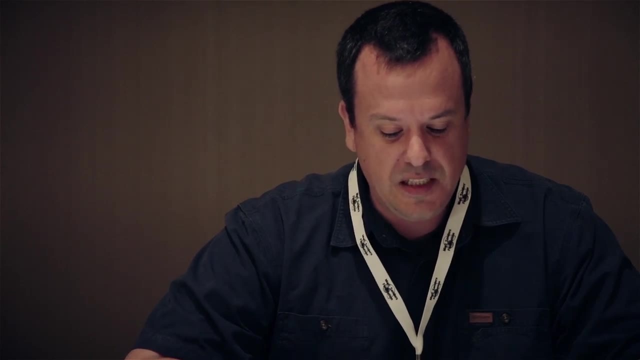 Books are generally performed or read and not played with, And yet Zella has taken it upon herself recently to ask questions of the characters in the books and seek a response By this. she asks the characters on a page a question and she expects a response. 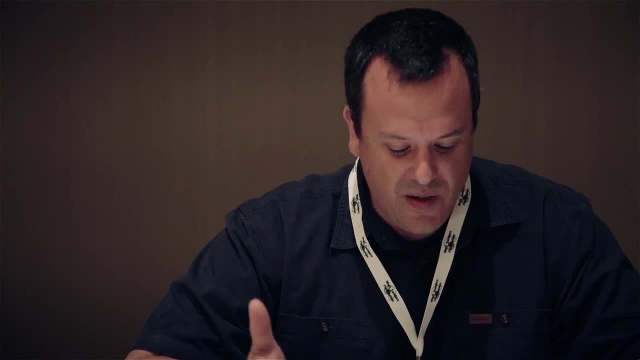 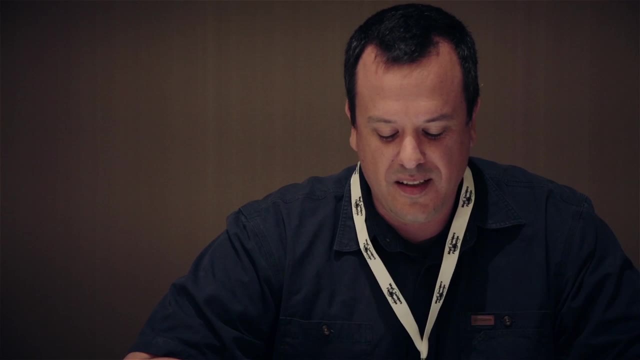 from that character. She wants to know why they did something where their mom is. what is their favorite color? I'm not entirely sure how it came about, but my best memory is at one point she asked me why a particular character did something. 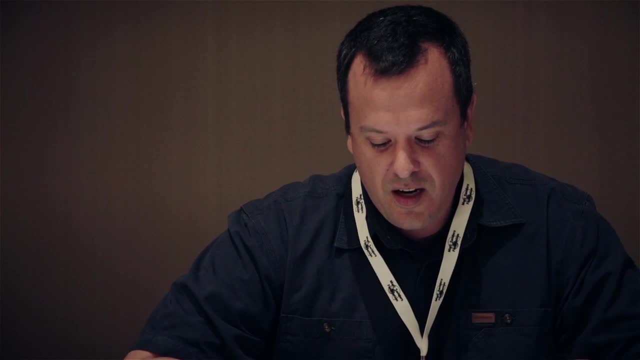 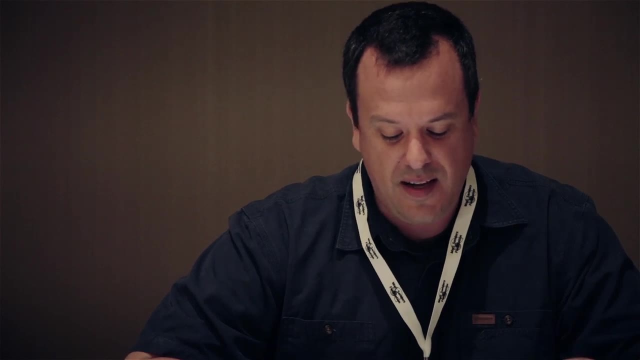 and I offered: well, what do you think they would say? So she asked the character what they would say and my wife and I began speaking back, as if the book were responding. The conversations we have in this way are fascinating. For example, 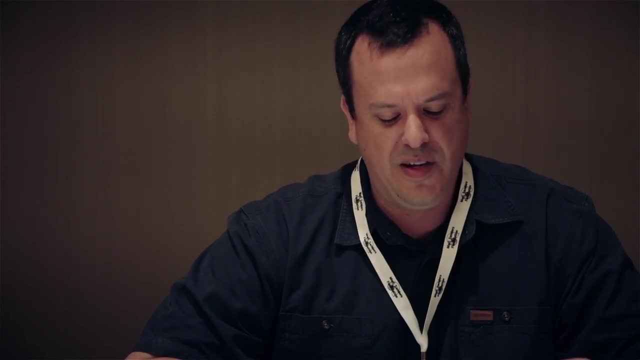 we often get to the point where the character has the intention to do something and Zella will reply: but you're on a page. you can't do that. It's not clear to me what things are prohibited because you're on a page. 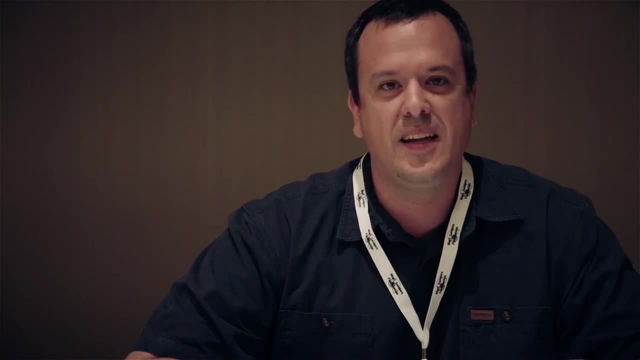 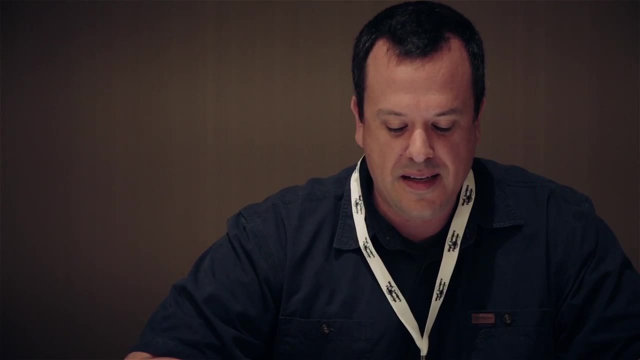 but she knows. In short, she has found a way to incorporate wildly imaginative play into the context of just reading a book. In all of these cases, I think that the worry about what sort of toy is best is more a barometer of our feelings. 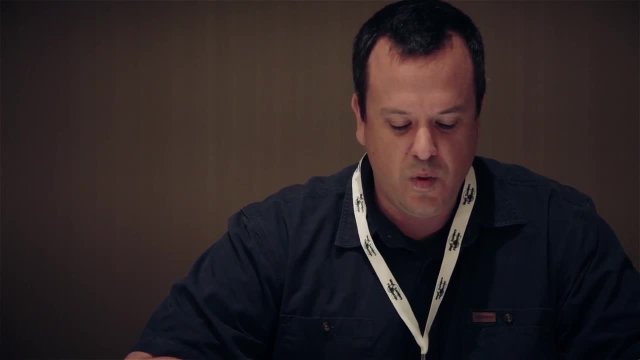 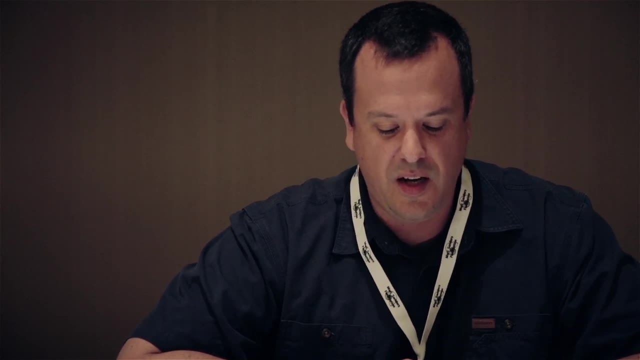 about our own creativity than it is about how best to nurture children. We're worried because we categorize objects so clearly according to their function and we cannot imagine all the things that our kids might do with non-open-ended toys, And our thoughts here are based on true phenomena. 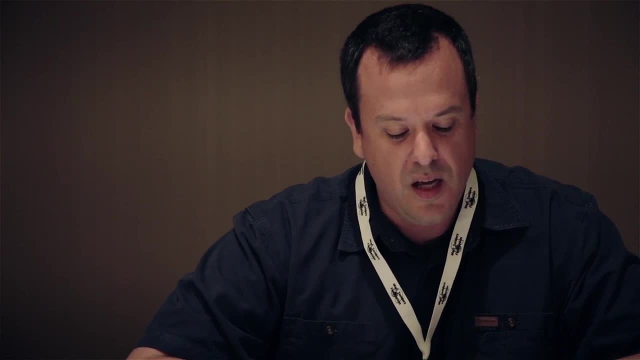 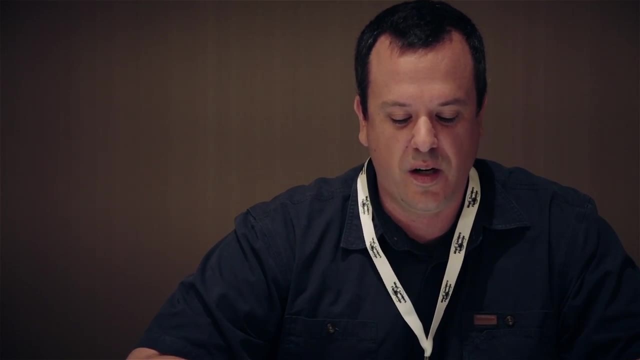 I think Once we decide what something is or how to use it, we tend to continue as if it is the only thing the object is good for. Ellen Langer and Alison Piper, for example, have done interesting work showing that the way in which an object 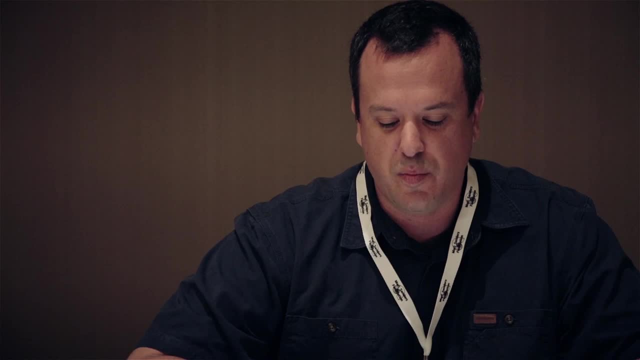 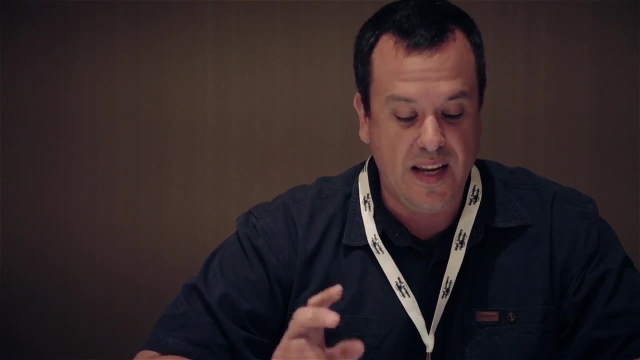 is presented to someone influences how they will see the object as fitted for certain purposes. They've done studies introducing people to an object with a simple linguistic variation. Either the object quote is something or quote could be that same thing. So in one iteration 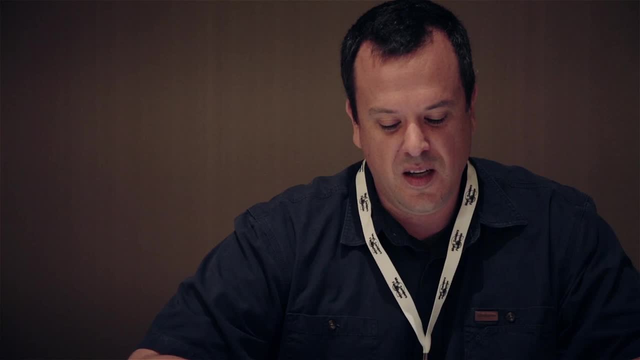 an object either is a dog chew toy or could be a dog chew toy, They then create experimental conditions in which there is a demand for that object under a different description. So in the dog chew toy experiment they created a demand in the experiment for an eraser. 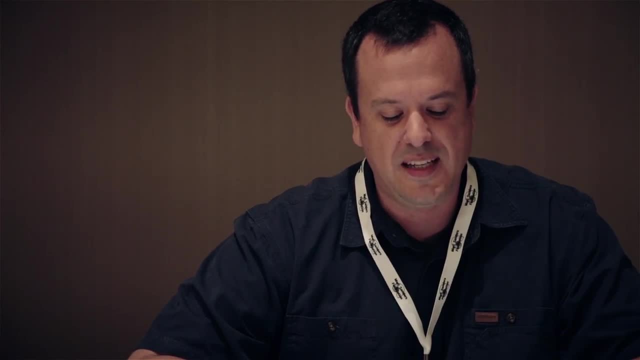 The effect was profound. None of the subjects told that the object is a chew toy saw that it could also be an eraser. 40% of those told that the object could be a chew toy suggested that it could also be an eraser when needed. 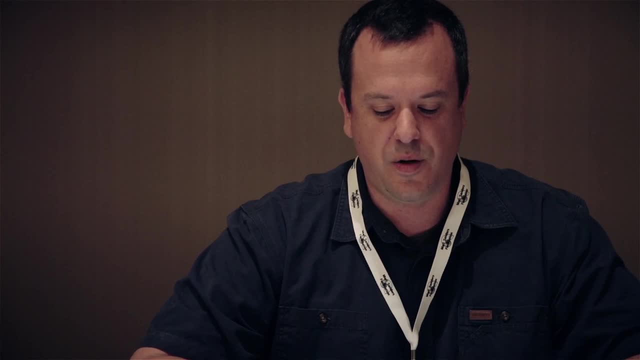 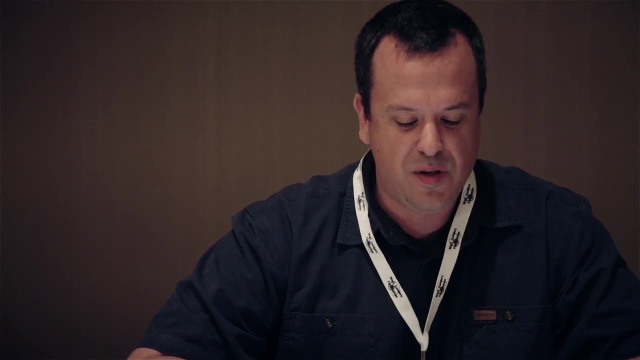 I think that something very similar could be going on with Zella and her toys, That is, she pays very close attention to how I interact with objects, how I offer them to her or how they are presented by other adults, And when I play with Zella. 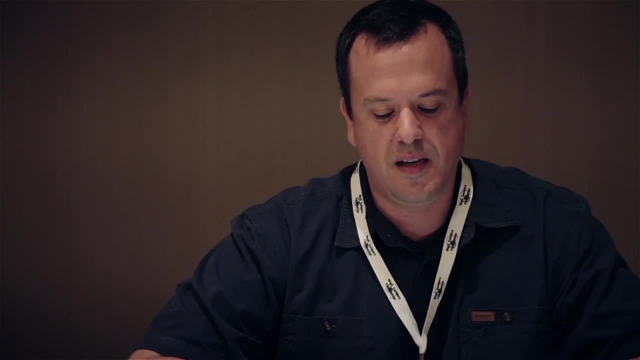 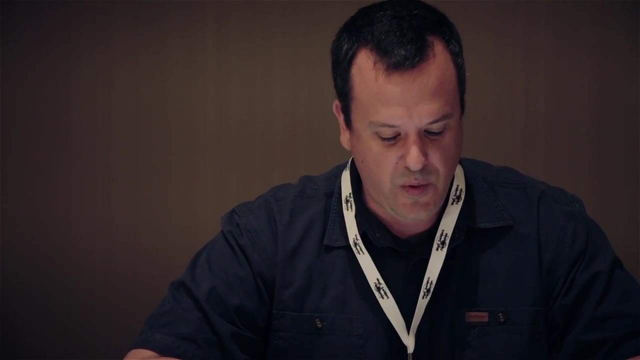 I think it matters much more how I interact with her and her toys than it does which toys I give to her or let her play with. In particular, she seems very sensitive to when I give her an object for something and when we examine an object together. 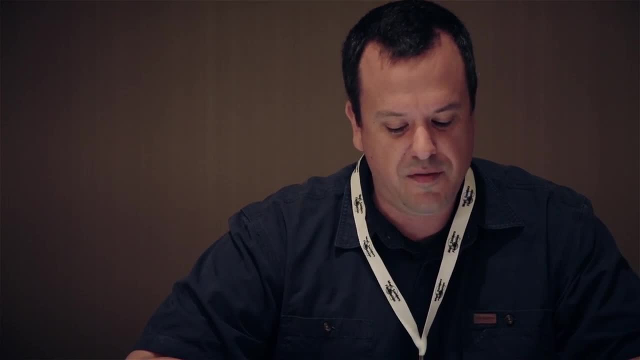 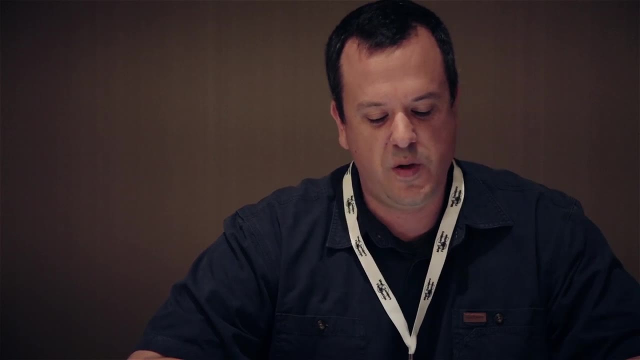 and its function is left up in the air. she is very sensitive to that. This seems to me a fundamental aspect of raising a philosophical child: trying to understand and respect the agency of our children and give them space within which to exercise that agency. 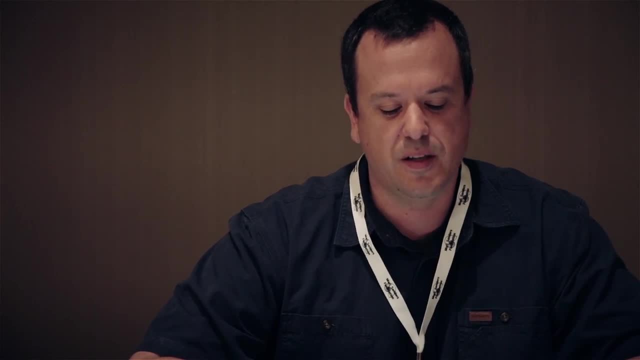 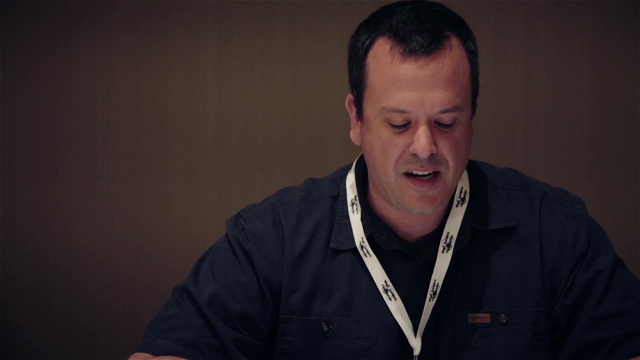 This agency does not reside in objects, but in Zella, and my focus should not be on manipulating her environment in order to make her do particularly favored activities. The sort of philosophical inquiry I'm after here is an activity. it's not a reaction to a particular situation. 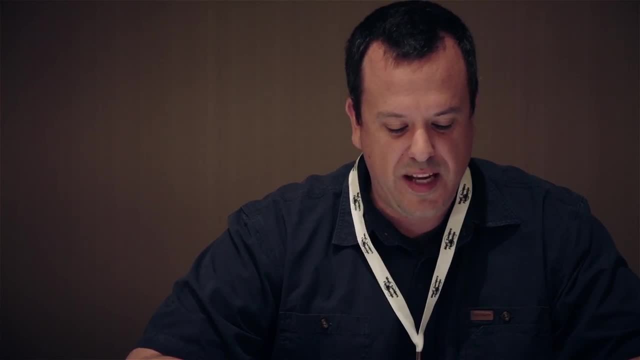 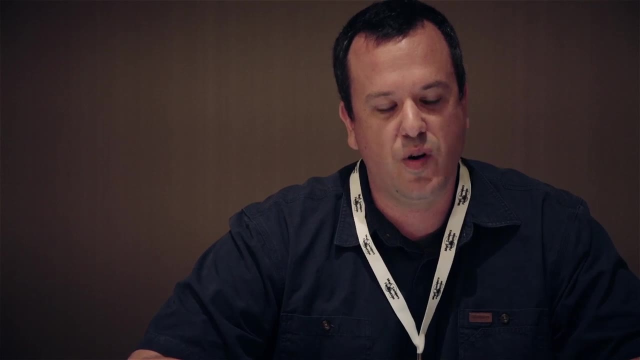 A child may play creatively with a non-descript block because there is nothing to do with it but imagine. but it's not clear that this makes a child generally more imaginative. Priming imaginative play may run the risk of teaching children that imagination is to be elicited. 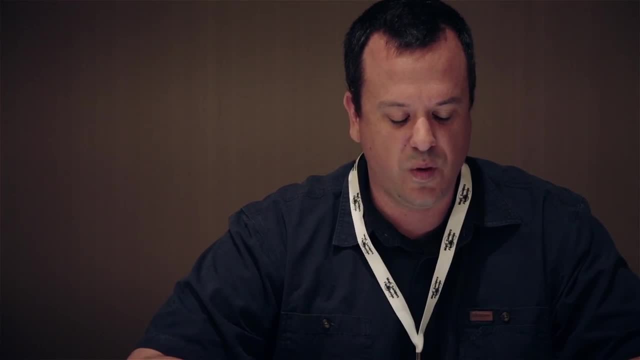 as a reaction and not brought to the world as a mode of being. We cannot change the world so as to elicit the best reactions and experiences from our children, as much as we might like to do that sometimes We can only help our children to better grapple. 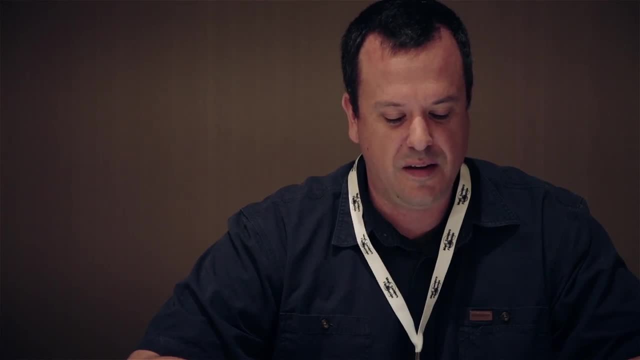 with the world as it is, And this is what I think might be most important about raising philosophical children. We focus on enabling our children to deal with the world as it is and not as we create it to be for them. One line of objection: 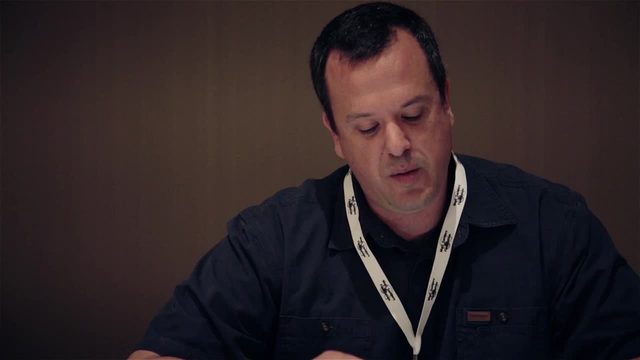 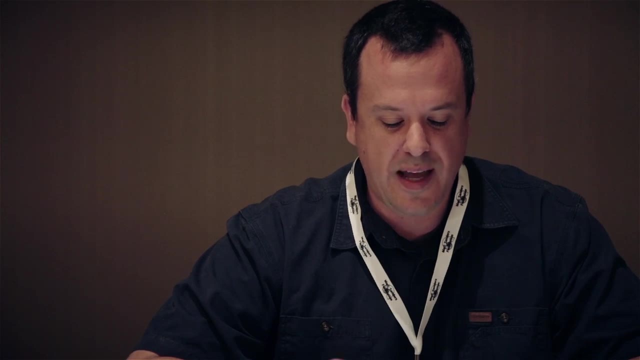 to these claims about toys might be. children don't yet know how to play in any particular way, or at least children of one and two, So we must encourage or induce them to create a play in order that they learn how rewarding it can be. This echoes arguments. 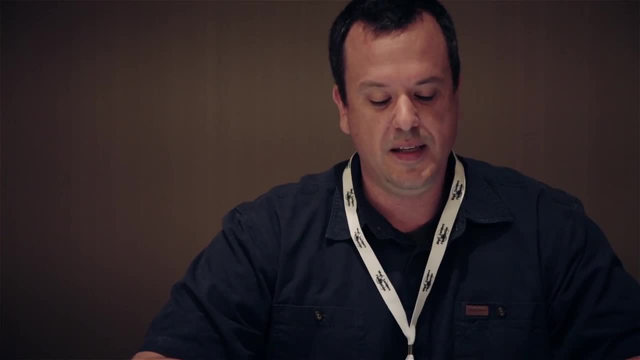 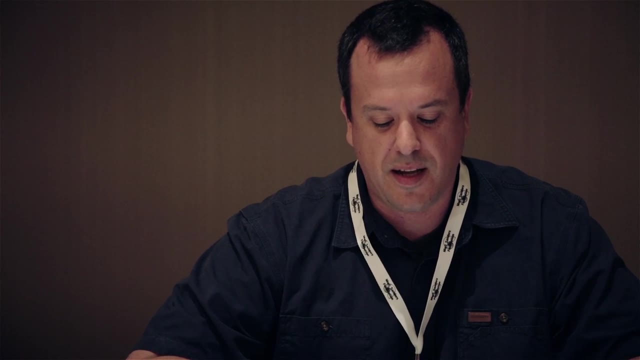 in virtue ethics, where I think that most children need to be induced to temperate behavior in order to appreciate its value, because it is not naturally attractive to curb one's desires. It's what Aristotle says. He says, quote: the many, especially the young. 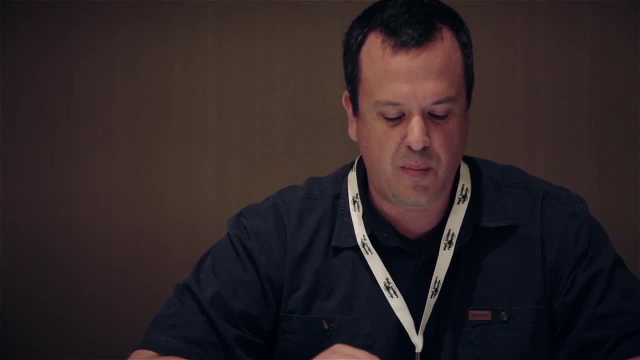 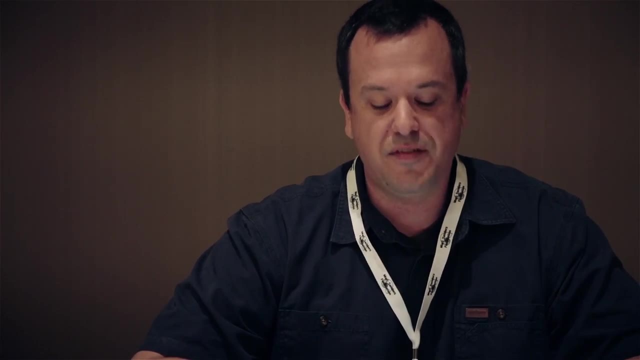 do not find it pleasant to live in a temperate and resistant way. That is why laws must prescribe their upbringing and practices, for they will not find these things painful when they get used to them. This might be the case. I often ask Zella. 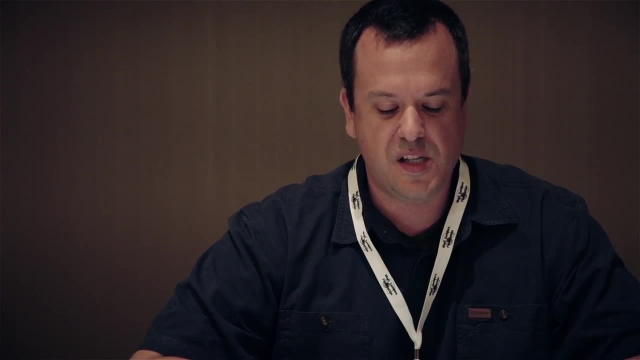 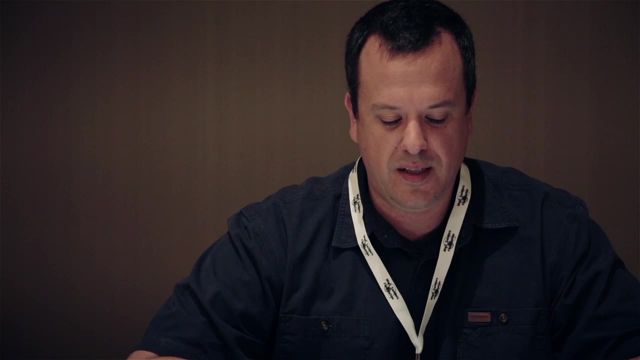 to try things in the hope that she finds them pleasurable or rewarding in such a way that she can make them. But I hate the notion of inducing her into action or behavior by limiting or manipulating her environment, And I think it's unnecessary for imaginative play. 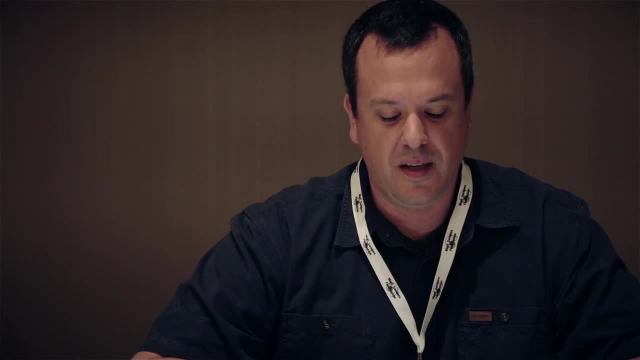 In general. until I met Zella, I had a lot of unexamined notions about what a toddler is capable of doing. For example, when she was about one and a half, just learning to speak in more complete ideas and phrases, I was talking to her. 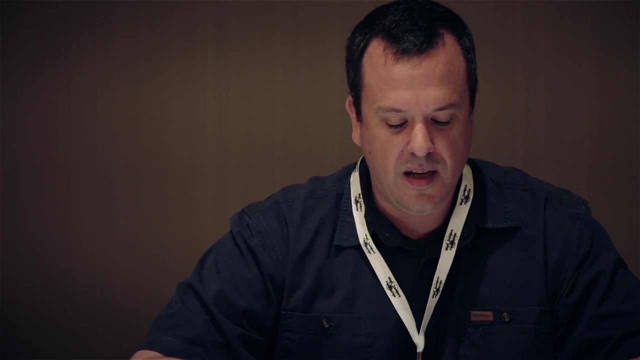 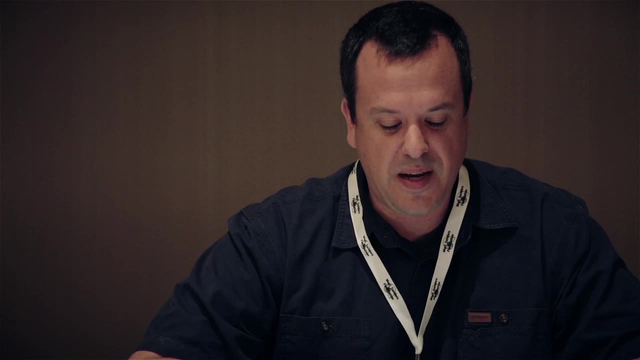 about why she could not eat medicine. I had a cold and I was taking some cough medicine. I told her something about it not being for her and she exclaimed: it must be spicy. She had recently decided that she didn't like spicy food, and her urge to explain 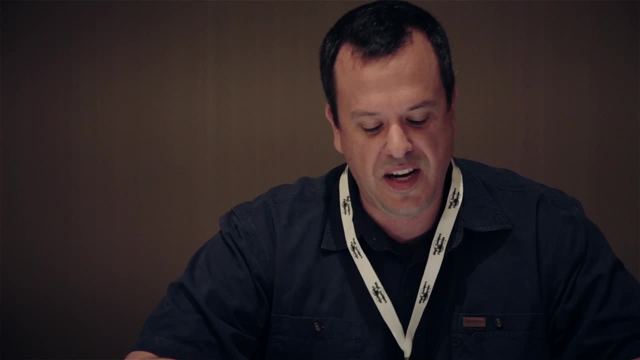 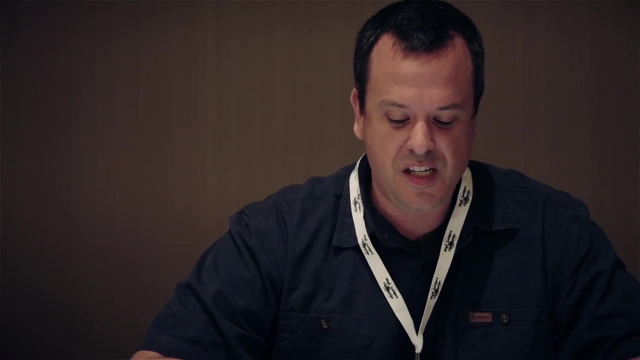 her world at that age blew me away. She cleverly inferred the best explanation she knew for why she was not able to eat the medicine. Not only was she interested in causal explanation. as a one-year-old, she was capable of reasoning about a novel situation. 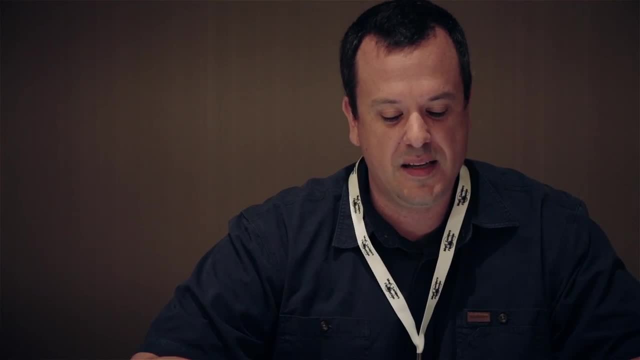 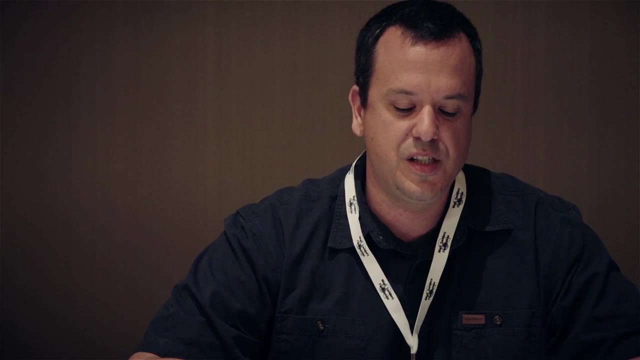 She was generally capable of much wider and more agency than I realized. The reasoning about open-ended toys may stem from a similar sort of underestimation of the capabilities of young children in the world. With regard to imaginative play, for example, I've had many engaging. 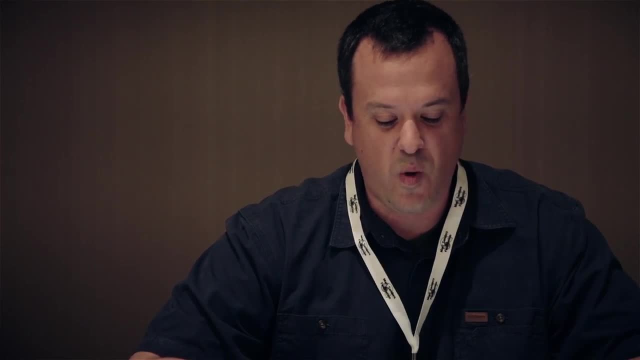 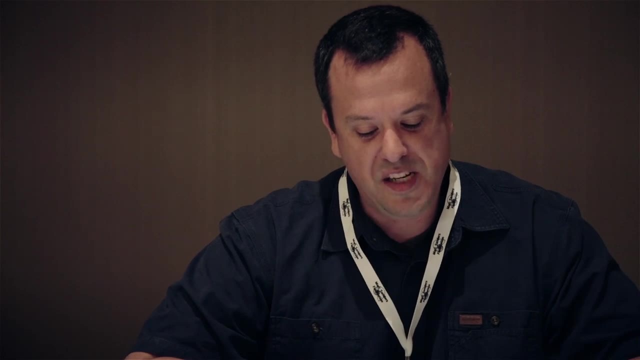 conversations with Stella about imagination, what it means to imagine something, why it is fun. She is quite explicit about imagining herself in myriad roles. So, for example, I returned home from teaching many times in the last month or two and she declares to me: 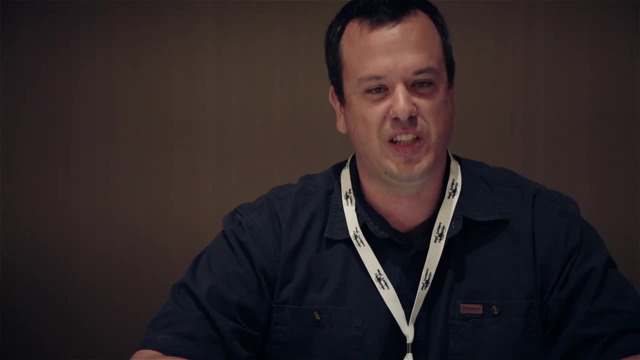 I'm Anna and begins to sing Italian-sounding gibberish at the top of her lungs. So she's channeling Anna Netrebko, her favorite opera singer, and trying to sing O mio bambino caro, her favorite aria. 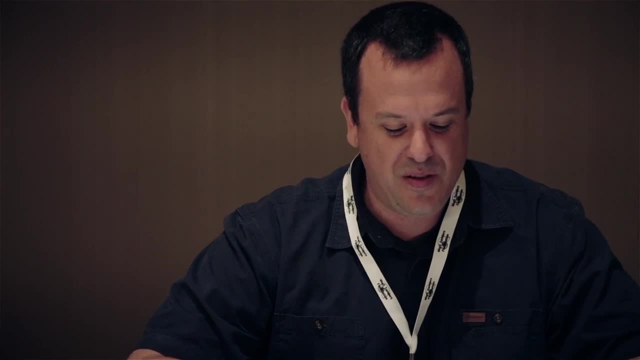 And she says she actually has the tune down quite well and will strike the pose Netrebko strikes at the end of her favorite YouTube version. A short list of objects that she has used as a microphone shows, I think, that she is decidedly. 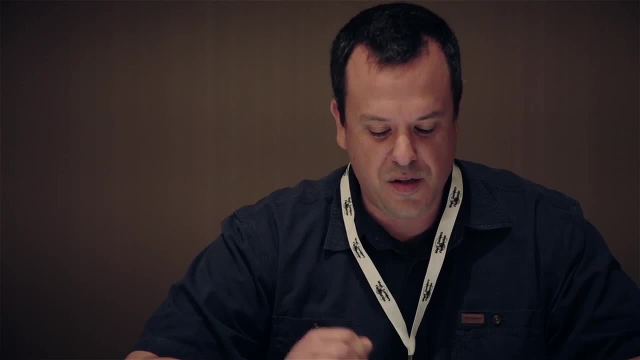 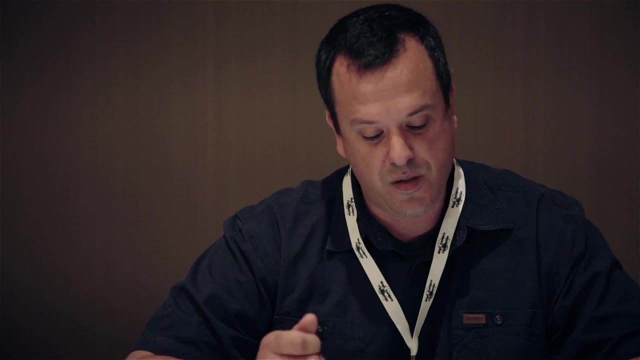 uninterested in an object's apparent intended use or open-endedness. In the last month or so, she has used a foam roller for stretching an air pump, a flashlight, a kaleidoscope, a chopstick, a remote control, a dinosaur toy. 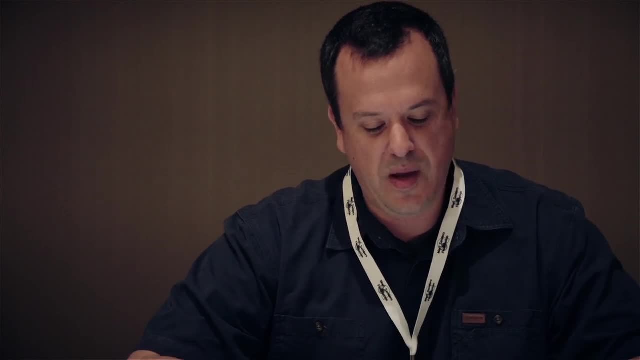 a wooden piece of toy train track, a light-up Halloween spinning toy and the cardboard tube and the paper in the bathroom. So all of this imaginative play was self-directed and arose from her listening to and watching some of the same things on TV that my wife and I watch. 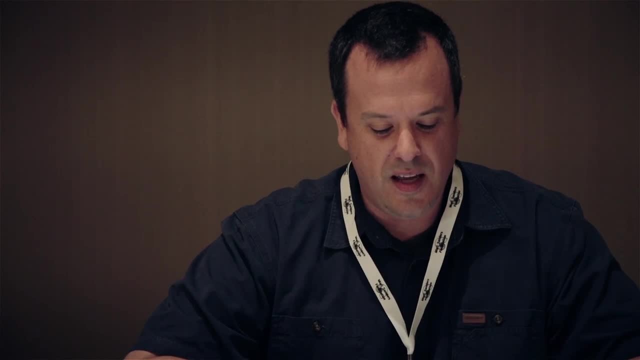 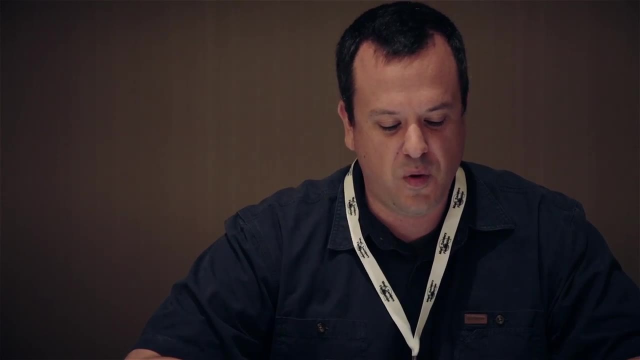 and hearing grandma use quote her real voice. So her grandma was a professional opera singer. In general, she does not seem to be looking for the objects in the world to suggest to her how to interact with them, but rather looking for objects that can serve. 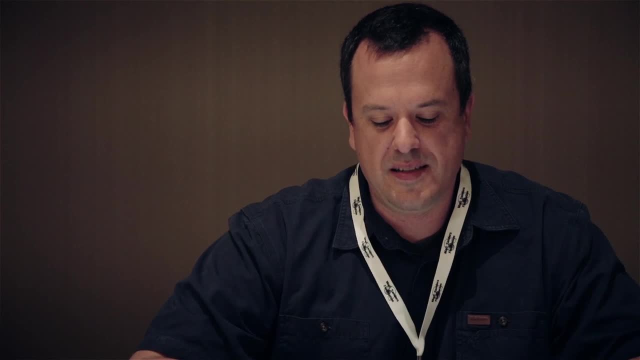 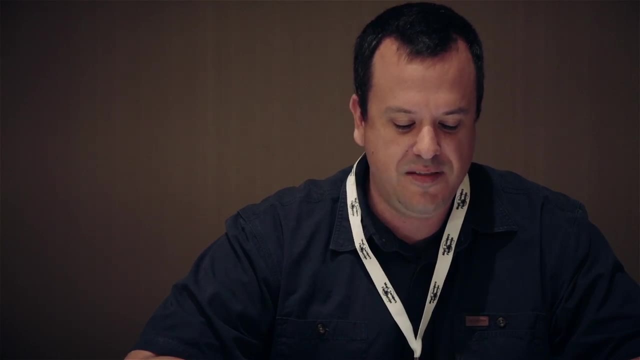 the interactive purpose she already has in mind. So, to conclude, I want to try and answer the question that I have in front of me. Perhaps what raising a philosophical child adds to raising a good child is that it can help us focus on our own sensitivity. 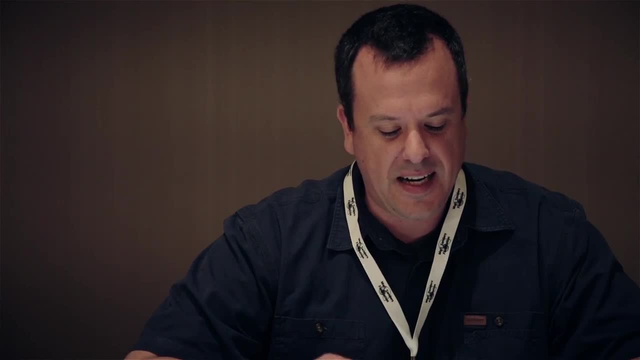 to the agency of and empathy for the perspective of our children. Many people act in many contexts as if raising a happy or good child can be forced upon a child. The children can be manipulated, so to speak, towards those goals. But it would be odd. 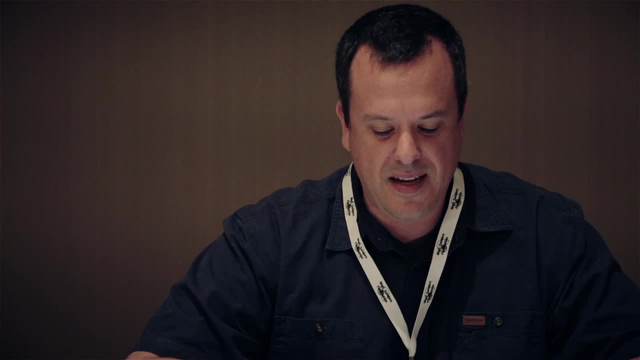 to think that we can manipulate a child to be philosophical. Being philosophical seems to necessarily involve the active agency of the child And so perhaps, explicitly, this focus on raising philosophical children can help us focus on and respect the agency of children. And I want to throw out 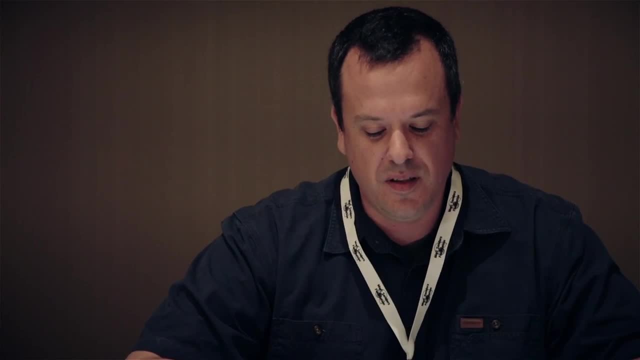 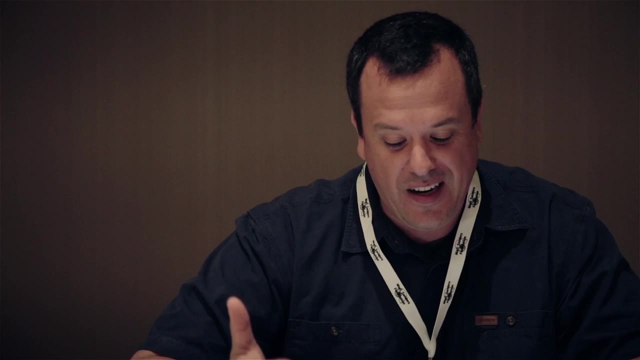 one final example, if I have time, where I think this set of terms could be helpful. So I've been concerned, as a parent of Zella, with the social norms surrounding tattletales. It can be difficult for a parent, or at least it has been. 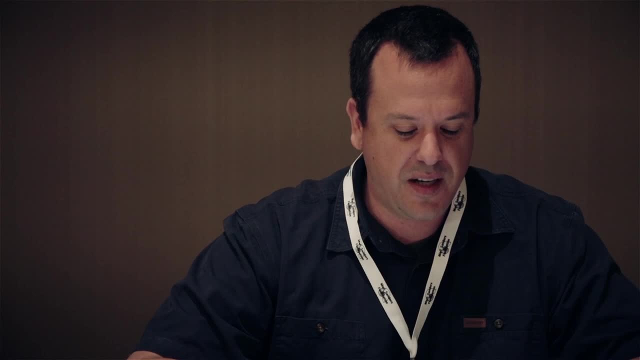 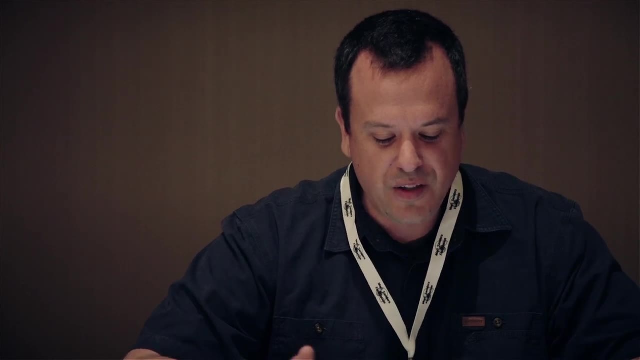 for me to know how to help her approach, balancing her own power to resolve conflicts with her safety and her right to make her own choices about her body and what she wants to be doing, And the dialogue around tattletales has been unhelpful. 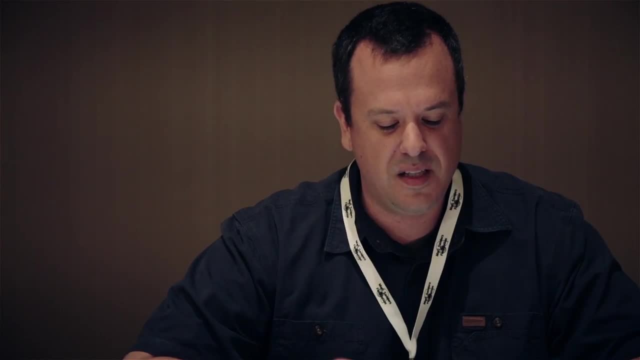 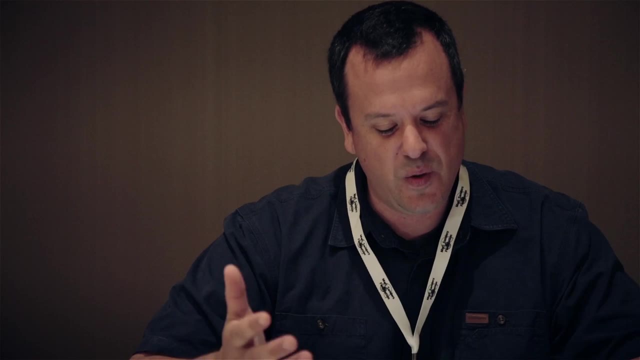 to me in part because I think it suffers from the sort of misunderstanding that a focus on the philosophical child might help cure. So there are many webpages, for instance telling parents how to deal with and discourage tattletales. But what's wrong? 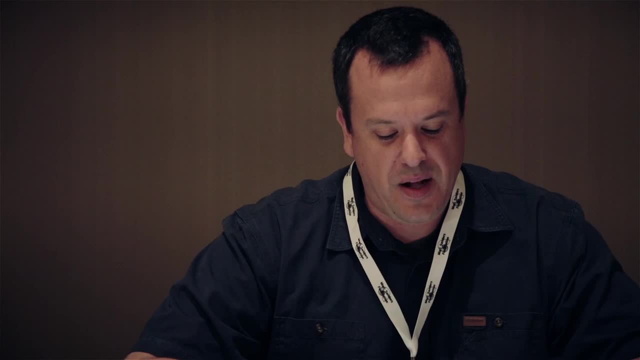 with tattletales. It can't be that kids speak up about things they perceive as wrong, because speaking up when things seem wrong is a basic quality of a decent person. Do so with humility and kindness, sure, but speak up, It seems rather. 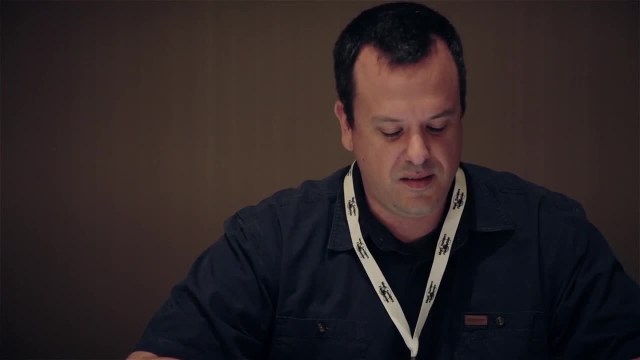 to me that the problem is that kids' judgments about rules, infractions are incorrect or their judgment about the proper response to an infraction is off, But in that case it's a perverse response to ask kids to simply be silent rather than help them. 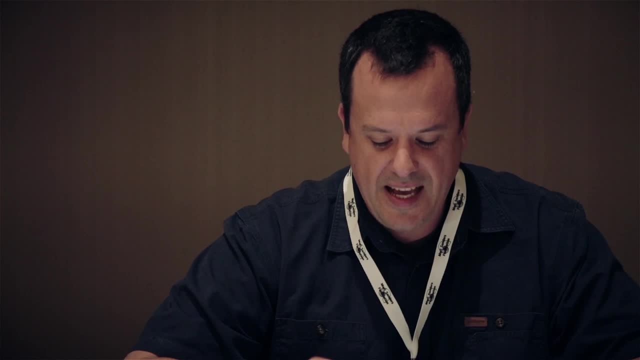 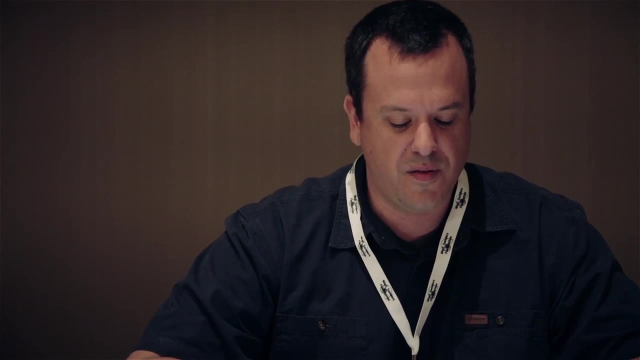 understand more about the rules and how to interpret them. The general norm of discouraging tattletales fits in some ways with the notions of happy and good. Children are rewarded as good for not tattling, regardless of the reason, and children are often told 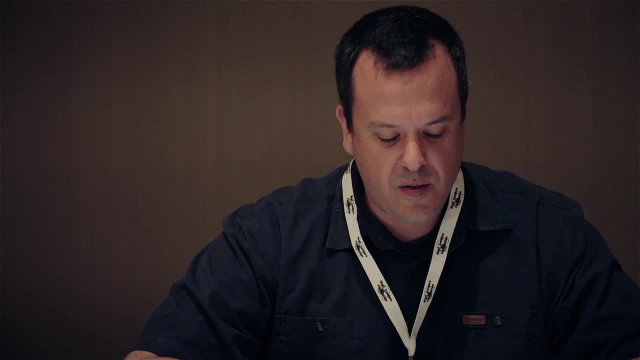 that nobody likes a tattletale, But it's hard to imagine taking a child's philosophical self seriously and treating tattletales in this way. We would rather want to talk to a child about what's going on. Why is it important? 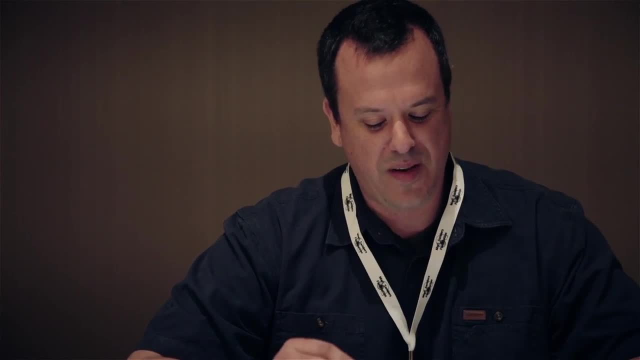 for them to report an infraction? Do they want to help solve the problem? How does it make them feel to see what they're reporting? That is, someone interested in raising a philosophical child would encourage their children to openly discuss the complex issues of power and curiosity. 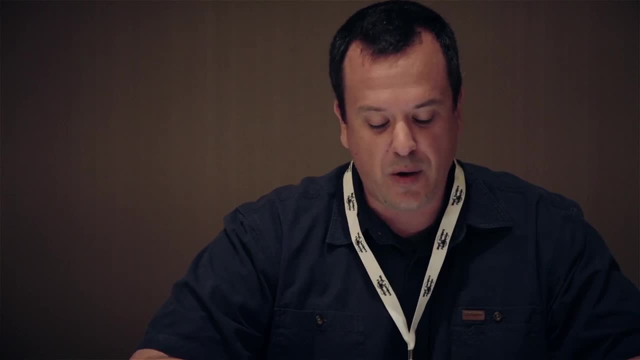 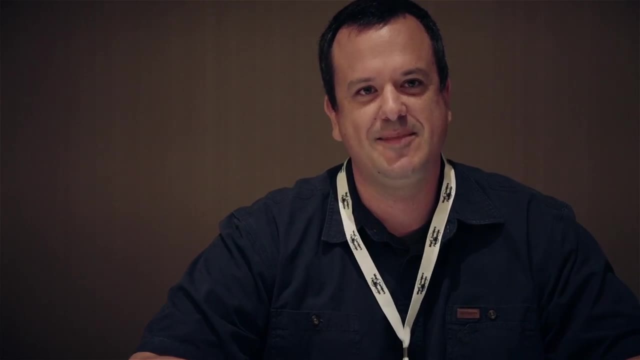 that characterize a preschool classroom, And one of the most powerful things I have learned from Zella is that kids are much more capable of having these conversations than I imagined. Thanks, Our next speaker is Sarah Gehring from the University of Washington, And her talk is: 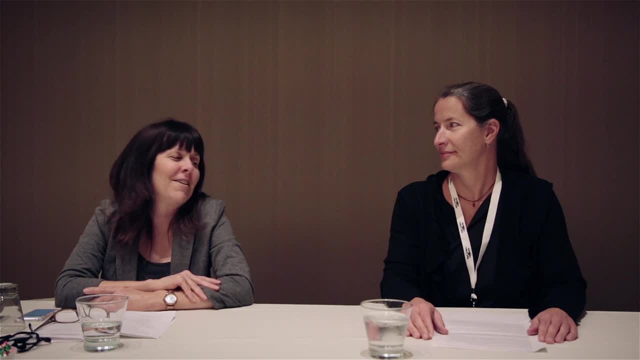 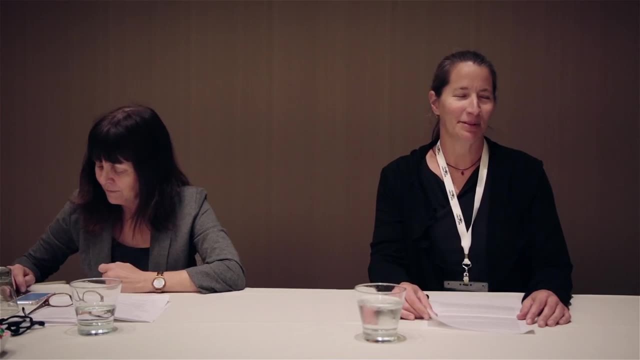 Oh, the Things You Can Think on Being a Philosopher and a Parent, Thanks. So I worry a little bit that my talk is going to be what Jana said was reporting amusing things. my son says that I can tell all my friends, But I'll at least. 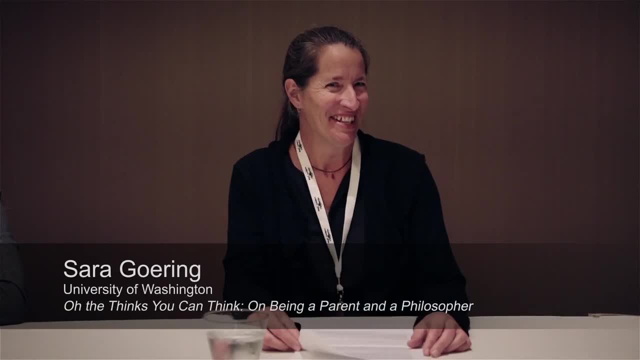 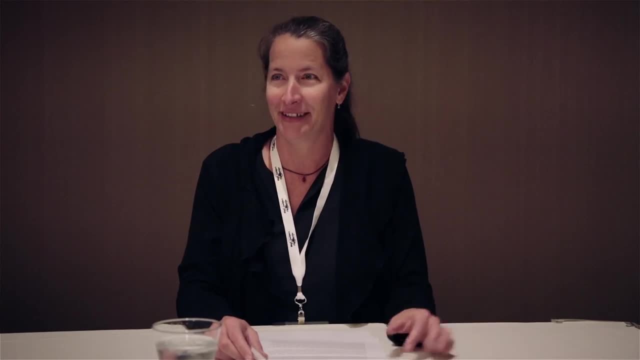 be the light moment here then, But that's something that I'm going to be talking about at the end of the talk. If that's not really what I mean, it's just that I'll probably have a lot of those stories, So any parent knows. 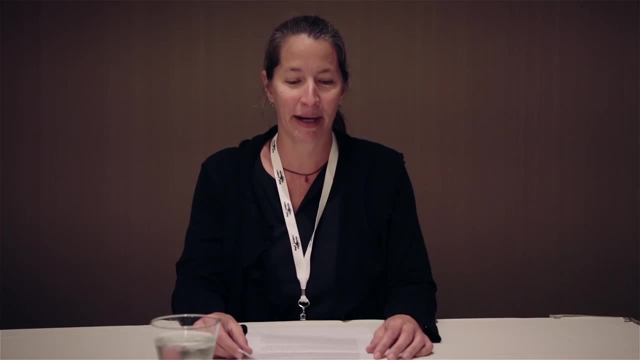 that once your kids can talk, there's no telling what kinds of things might come out of their mouths or in front of whom- Often embarrassing things that you don't want shared outside your home. Sometimes we react to the strange, interesting and funny things they say. 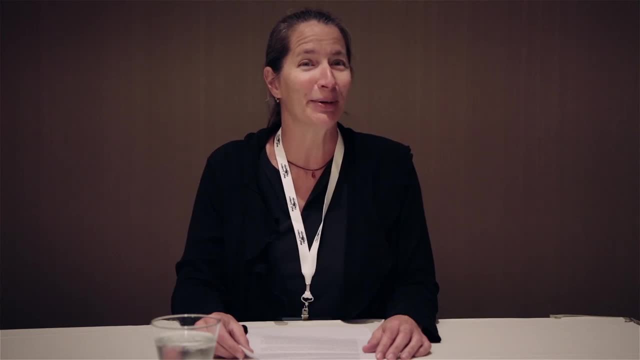 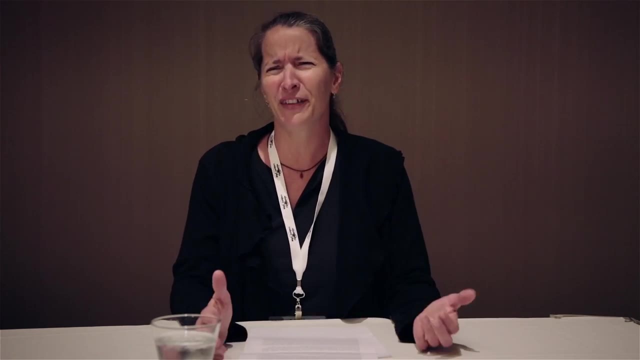 with humor. Indeed, the show Kids Say the Darnedest Things and, if you don't remember it, Bill Cosby was the guy who ran it. It's funny, But it feels a little strange because the kids are up on stage and then there's. 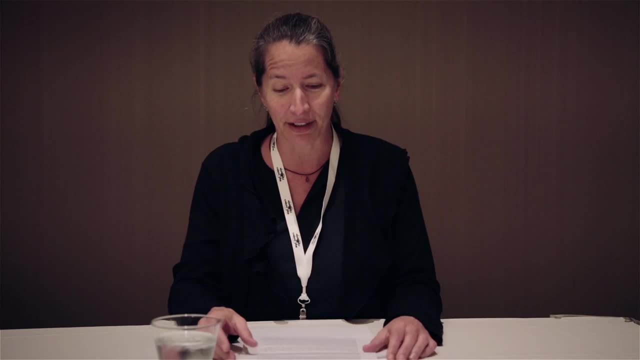 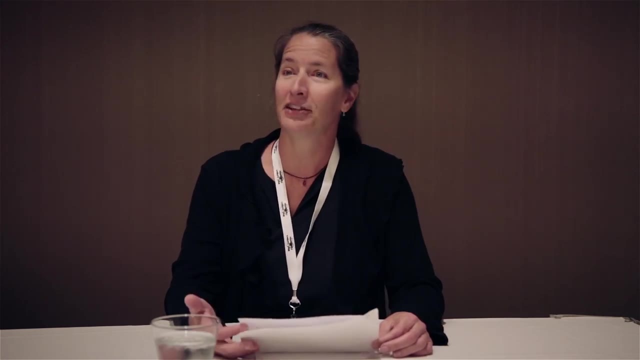 this whole audience of adults laughing and there is an odd dynamic that goes on there, But still it shows kids are thinking in interesting and funny ways. If that whole show could be there, I certainly understand the response. Kids say funny things and every parent 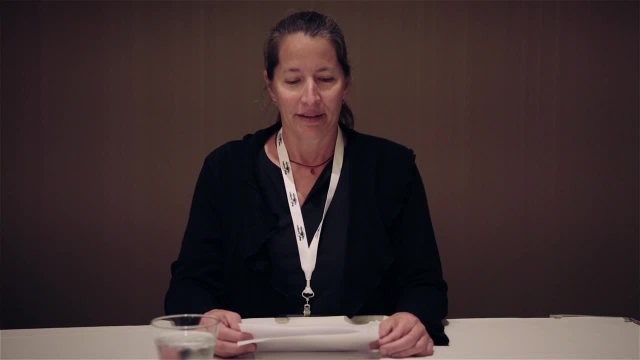 has to take some humor in those to make up for the times when we're crying. So the laughing is fun behind the odd things they say, because often I think if we take a bit of time we'll discover a much richer and more fascinating story line. 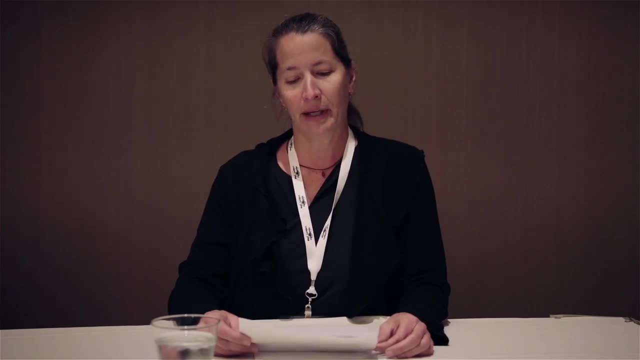 than we expected if we just look at the superficial humor in it. So in my time on the panel I want to talk about how and why parents- and I think this is true of both philosophers and non-philosophers- can appreciate and engage the little oddities. 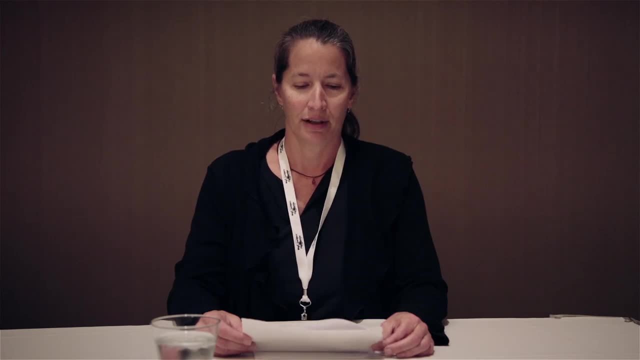 and gems that slip out of their children's mouths. and I should note, maybe as a side note, I do think all kids have philosophical capacities, but some definitely bring it out more regularly or without any assistance. So the most recent of the oddities, I have a five-year-old 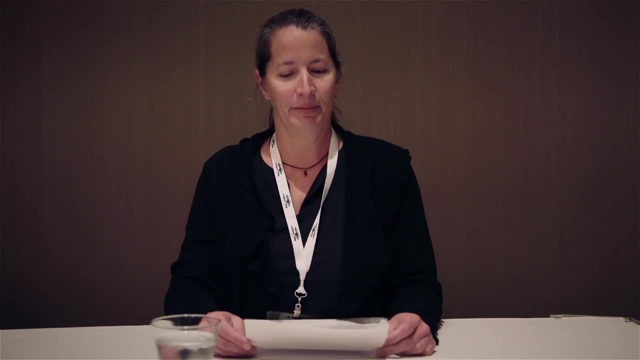 son and a nine-year-old daughter. The most recent of the oddities I've been faced with came from my five-year-old son just the other day, Mommy, he said, sitting in the kitchen in a battle between L and 12, who do you think? 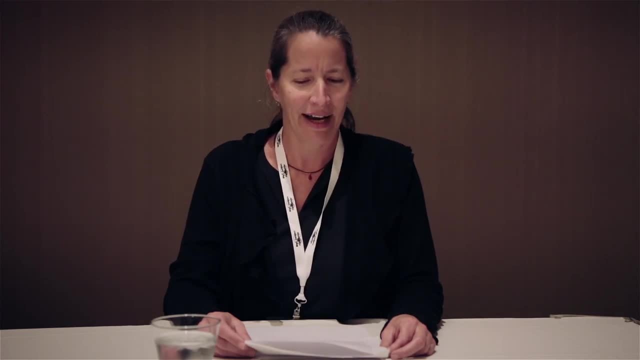 would win. I admit it had never crossed my mind that L and 12 might be capable of battle, never mind at war. It seemed nonsensical to me, but he'd clearly been sitting there thinking, exploring the options. I paused and chose a feasible route. 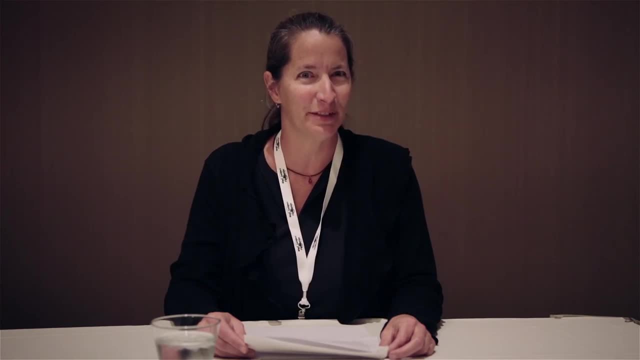 L, because in Roman numerals L is 50 and 50 is bigger than 12. and then I asked him what he thought he paused thinking. I don't know, but I would sure like to see it. It was clear that he wasn't convinced by my answer. 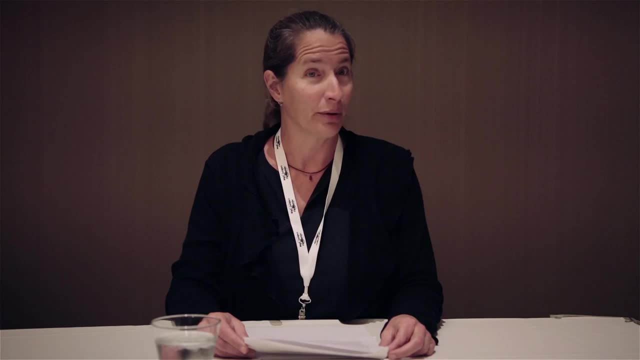 possibly because he doesn't know what Roman numerals are or didn't believe me that L could be the same as 50. But I think part of what was behind his not being convinced was that being bigger didn't need to mean that L would win. 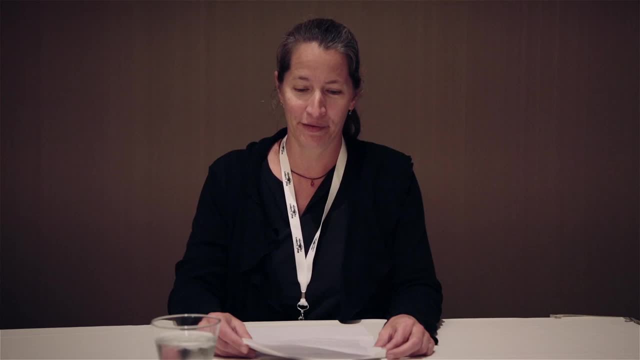 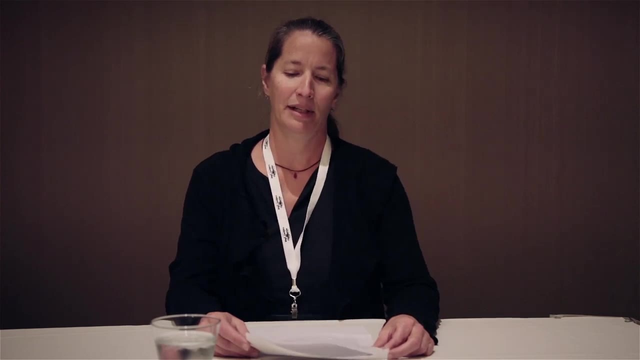 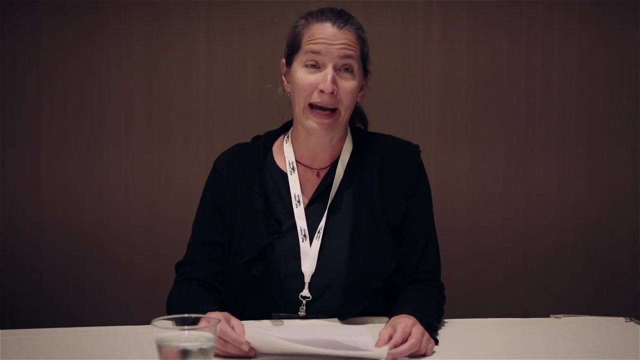 David beat Goliath. the mythical mouse can bring down the elephant, and children certainly like to remind us of that. Indeed, my point in these comments is that the ideas of children, their thinks, in Dr Seuss language can be not only strange and wonderful and funny. 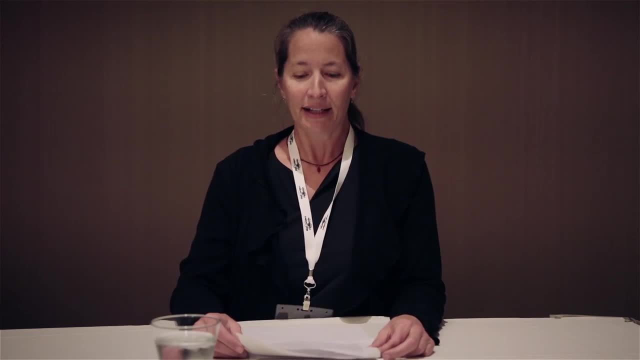 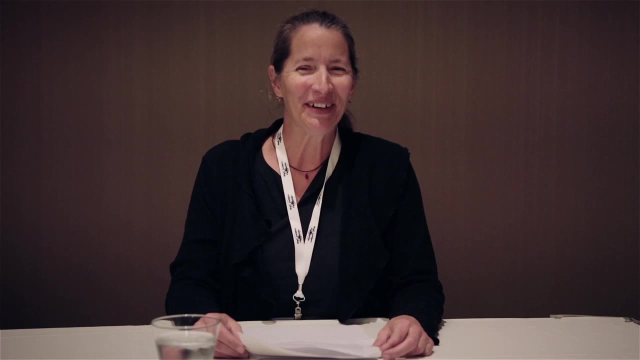 but powerful and provocative as well, and they're worth cultivating. I found, actually, that my son is filled with interesting philosophical questions, though I have to admit I may be a little bit overly attuned to it, so one day I picked him up in the backseat. 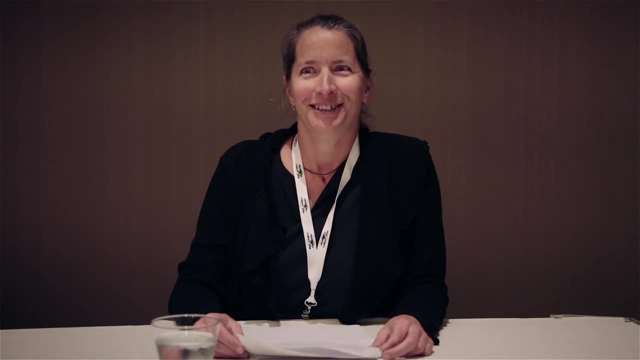 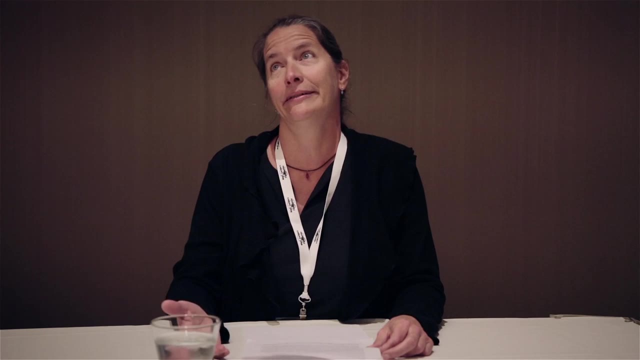 Mommy, am I free? And I thought, oh wow, he was probably three or four at this age and I said: what did you say? And as I said what did you say, My daughter said: well, you're not in school anymore. so I knew that I had heard it. 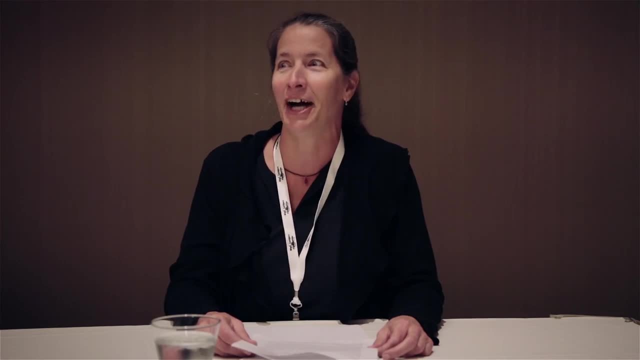 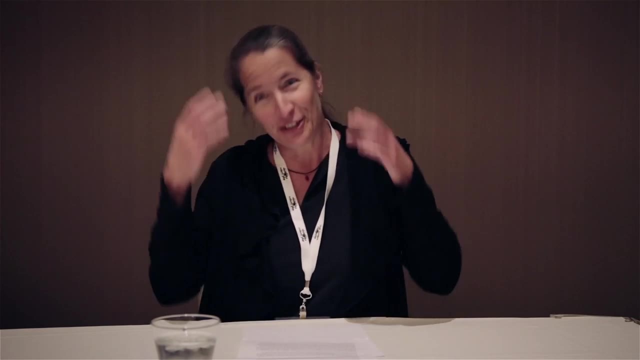 right, and I said that is a really interesting question and philosophers talk about it all the time- and it depends on what you mean by free- free to do anything uncaused, or do you mean causation goes through your head and then your body does things that you're actually? 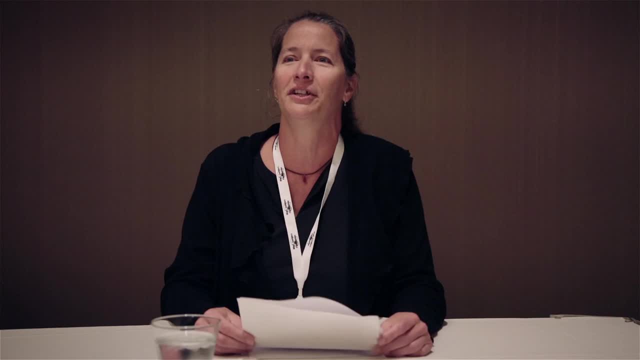 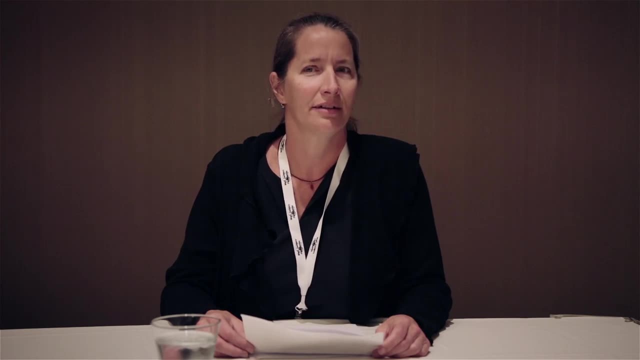 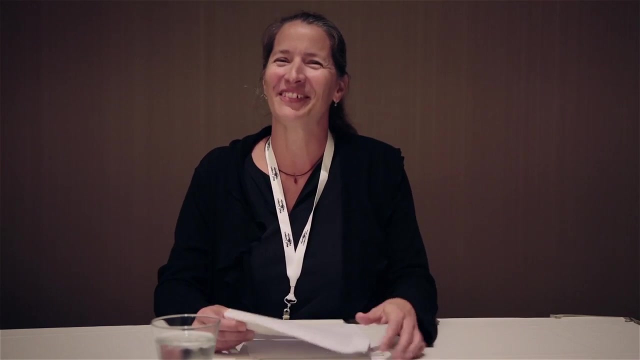 wanting to do, even if your body is determined in some way. it's fascinating. people have talked about this for years. he paused, thinking: okay, but how old am I? Three, right, I'm free. oh right, different question. we were not talking philosophy at that point, so I'm a little bit. 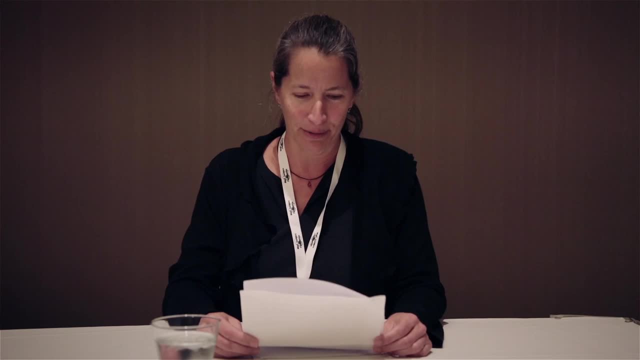 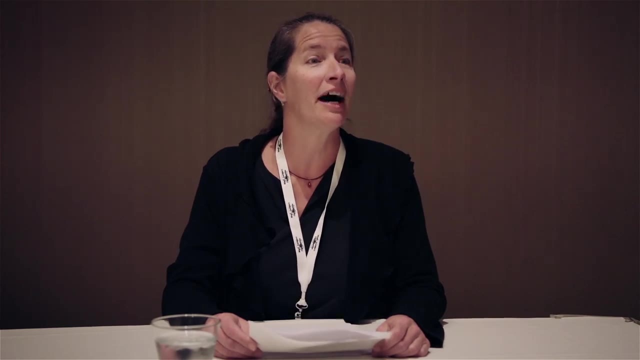 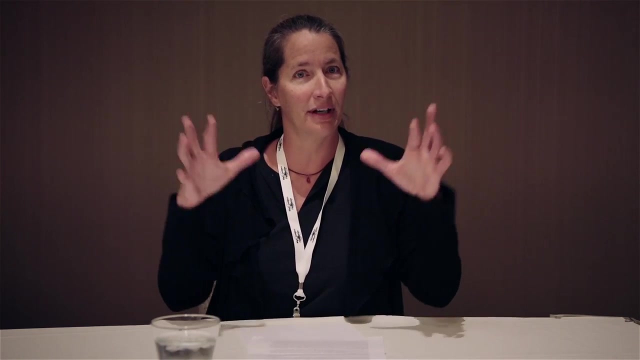 overly attuned. I recognize philosophical conversations now and I'll say I hear them mainly in two places, in the back seat of the car when we're going somewhere, just because there's time right and your mind isn't necessarily on any particular thing, and definitely at night. 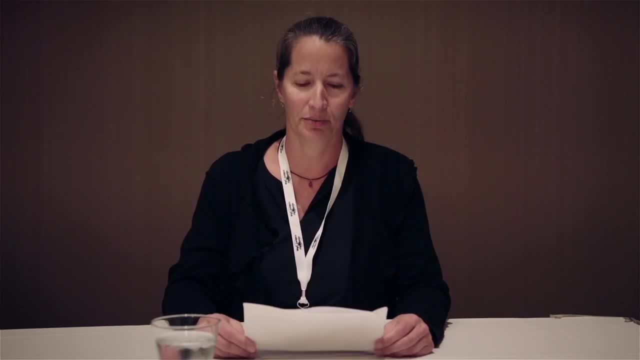 going to bed when the world's kind of getting quiet and you know we aren't attending to external stimuli, we're looking internally as we're going to sleep and it's so. it's so dark, it's so dark, it's so dark. we're trying to understand. 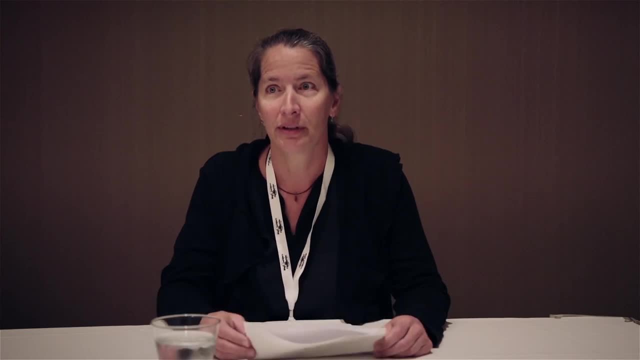 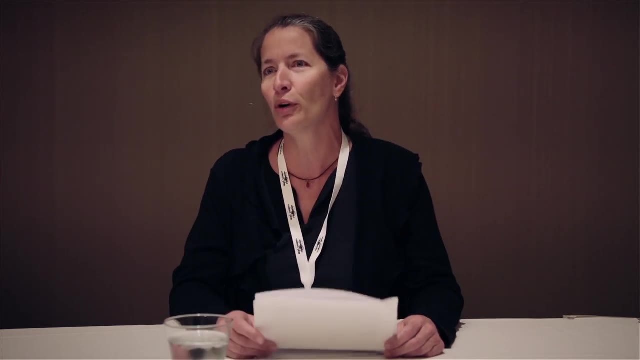 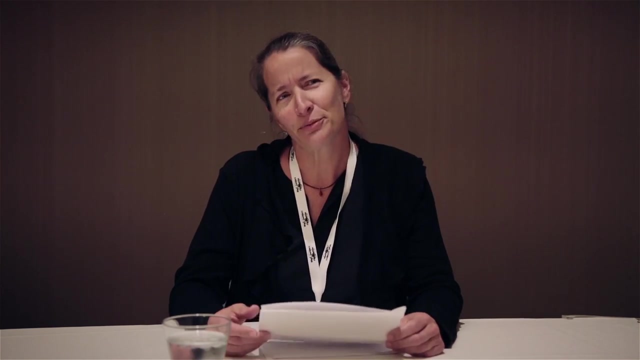 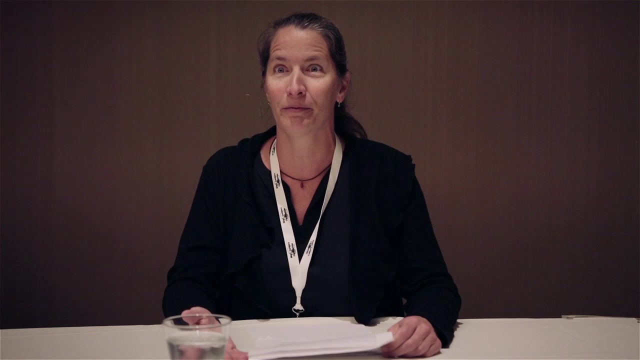 all of that and it's so dark and it's so dark, but we're trying to understand all of that, and so we're trying to understand that. and so here's a question about: are there several places in the world where do we have certain uptime? Where did the concept come from or where is it anyway? 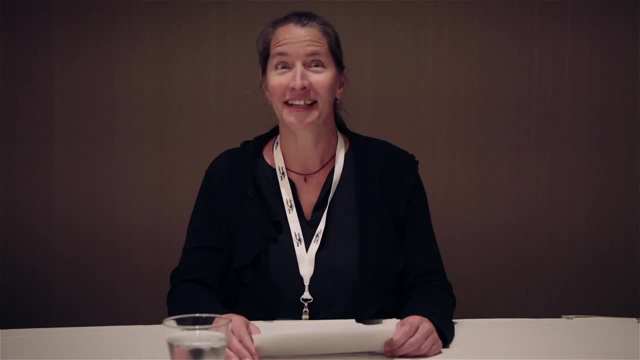 I thought: oh, this is a really good question. We had a little conversation. I said: I love that you think about these things. You know, I love to hear about them. These are things philosophers talk about a lot, right. 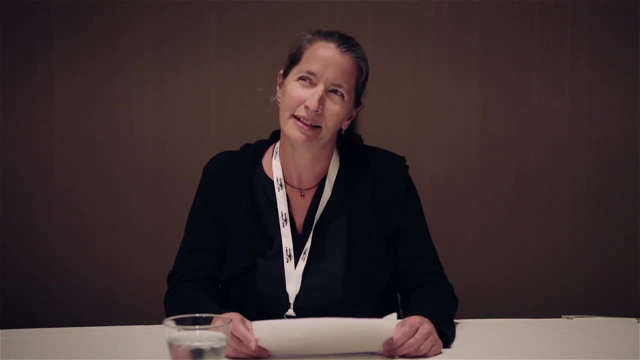 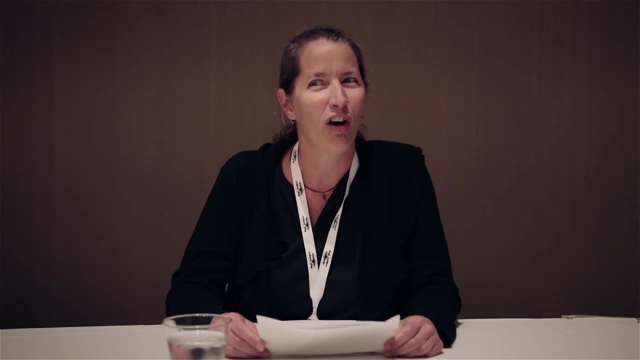 trying to figure out the way the world is. And he said: so can I tell you a secret? Yes, you can. Yes, yes, He said. I think about these things all the time in my head And I have lots of questions. 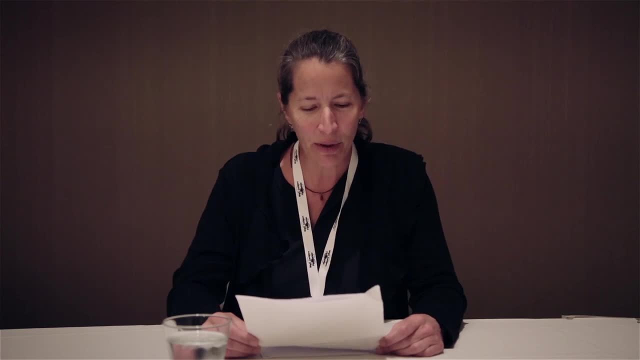 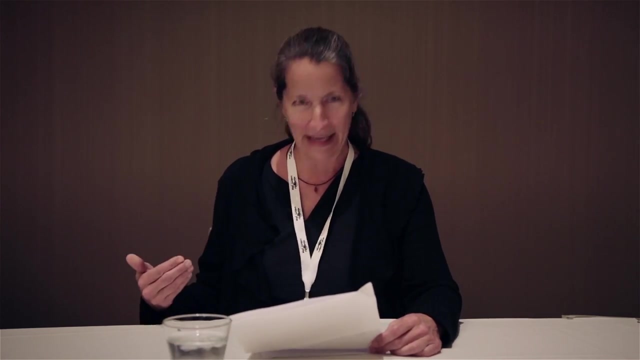 I said: like what? Like what are brains And how can we move our bones And how do we stay together? Like why don't we just fly apart all the different parts of us? And then he got started again. How is it possible for an egg and sperm to come together and make me? 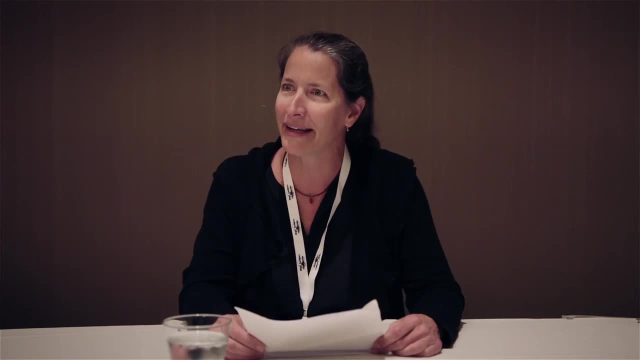 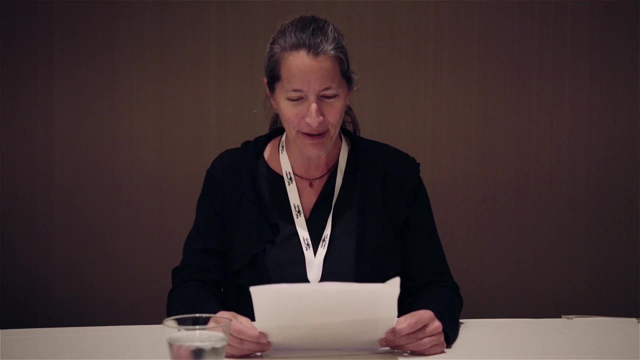 He looked at himself: How could that possibly be? And why am I here, Why are you here? And it went on right, Just question after question, Question after question. These were all secret, So we talked about those ideas for a little bit. 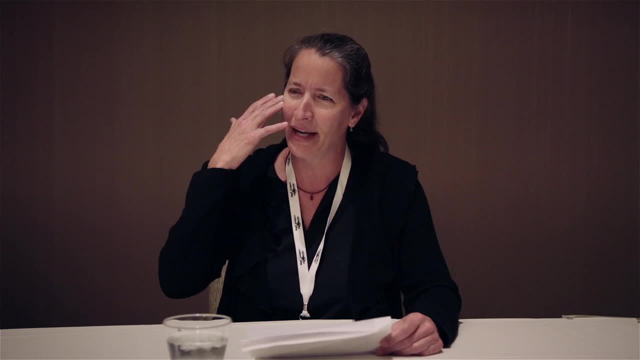 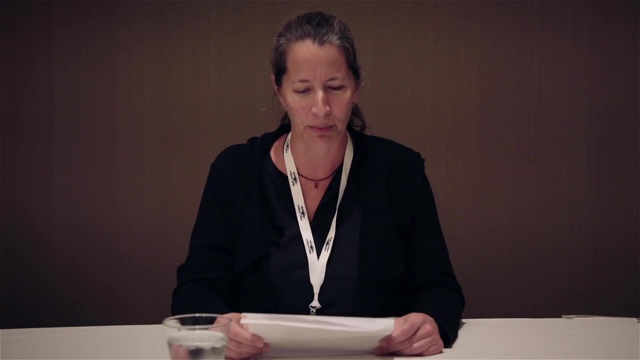 All fascinating right Another one was: how can I think up here in my brain and then move my toes? How does that work? How can I have this thing here and then something else in a different part of me moves? Then I asked him why he wanted the fact that he has them to be kept secret. 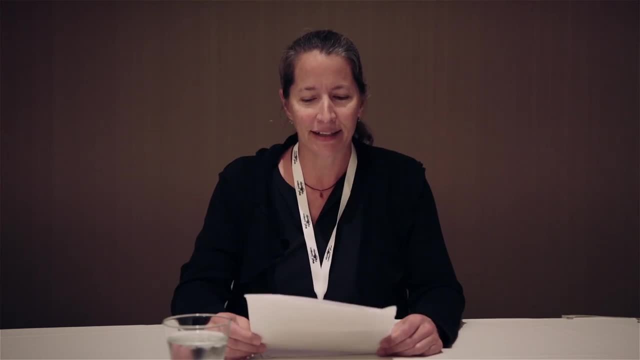 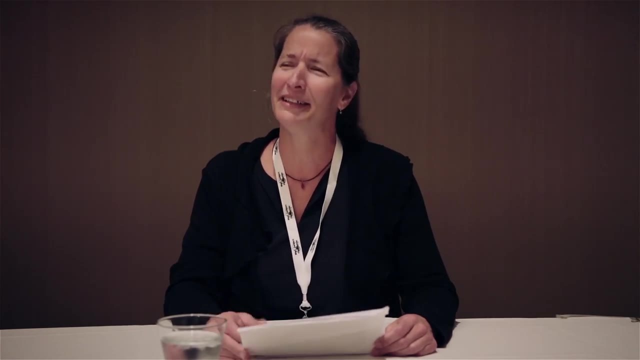 And I have permission to say it even on camera. And he said: because I don't want people asking me about them all the time, I just like to think about, I don't, he's a, he's an individual kid, He's not so social and he doesn't want to be bugged by other people. 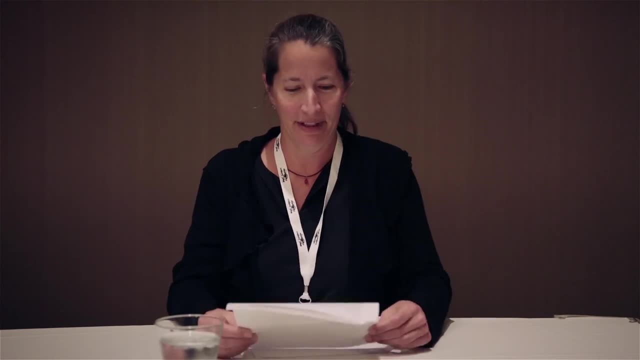 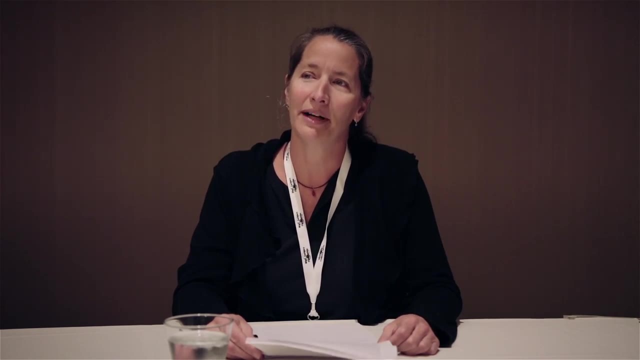 But if you don't ask him, then we're good. So don't ask him if you see him later. Um, after we had that initial confession out of the way, I started asking him at night. What have you been thinking about today? 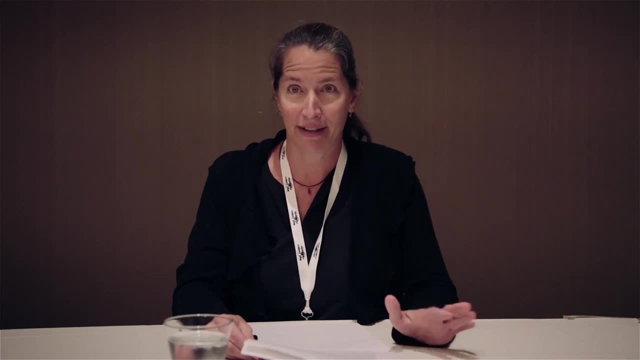 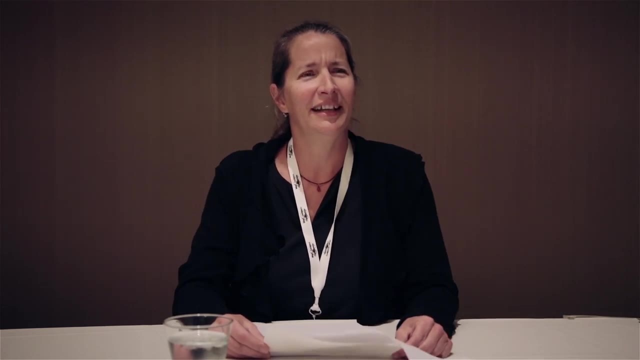 What kinds of things have you been pondering? It was okay if I did it, just not other people. Sometimes he didn't have much and he just preferred to hear a story. Um, but other times he he had really interesting things. 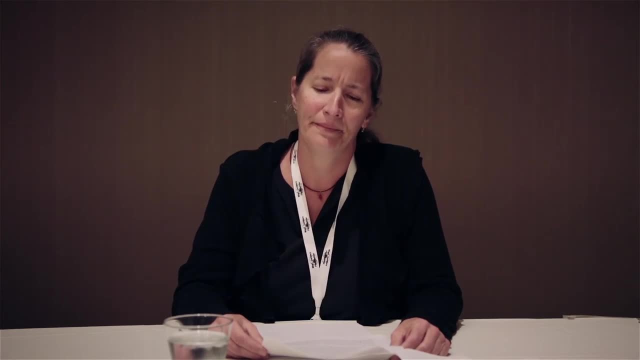 To say, for instance, he he told me one night: did you know that I have a knee? that's not my real knee, but it can still hurt. No, it's a knee in my mind and I can think of being poked by a nail and it hurts. 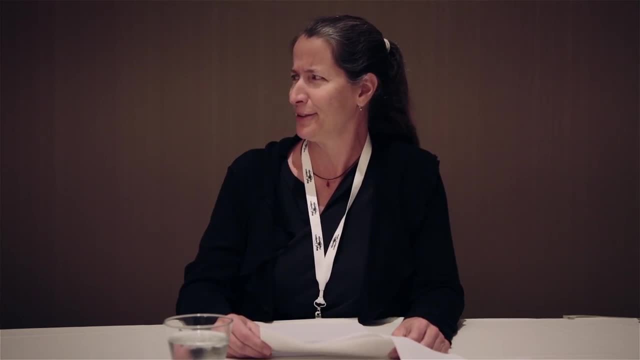 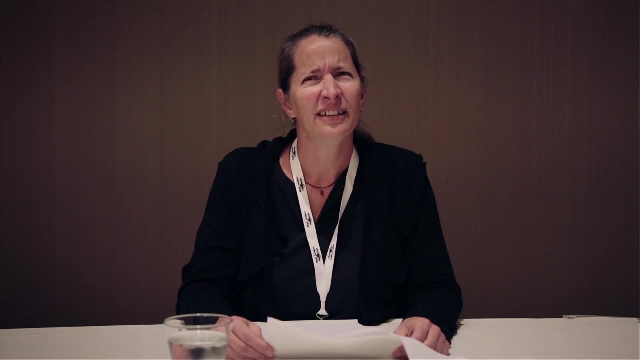 I thought this was interesting. I don't really do philosophy of mind, but I thought really, does it hurt? Does it really hurt when you think about being poked in your mind's knee? And he said: yeah, not the same as when I'm poked. 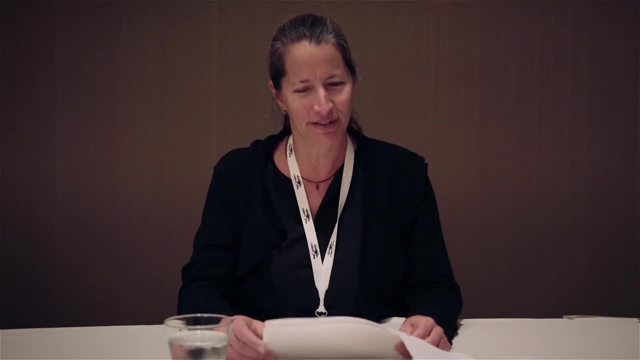 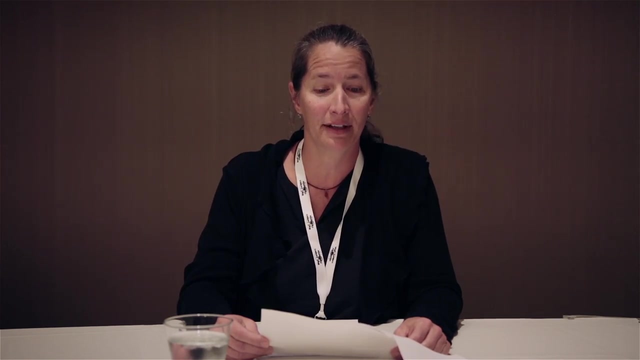 Am I real knee? But it does hurt I it feels something in my brain. As I would ask him, he would pause, focused inside his head, trying to figure out what to think and how to say what he was thinking. This is one thing I've found in talking with him and with the kindergarten philosophy classes I've been doing recently. 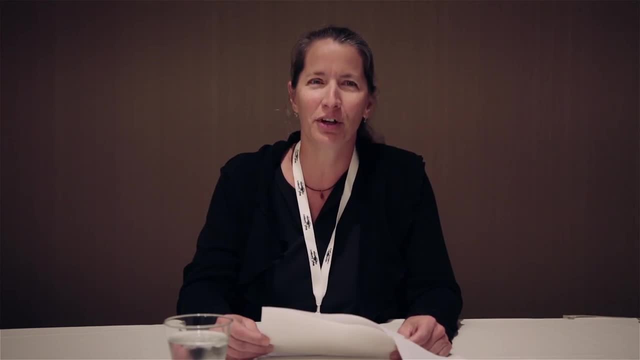 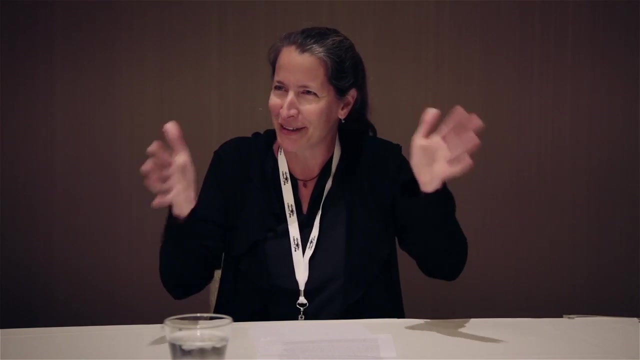 Often young children have really big ideas, but they struggle to articulate them. They stumble over words. They start to say one thing then pause realizing it. They don't quite get the point across. They try another way. They struggle again. Sometimes they use their hands to try to show you right there. Italian in nature. 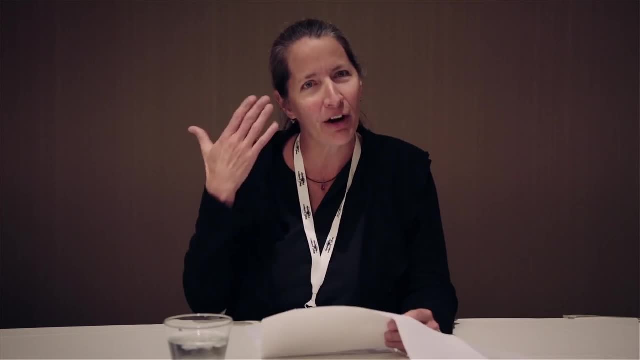 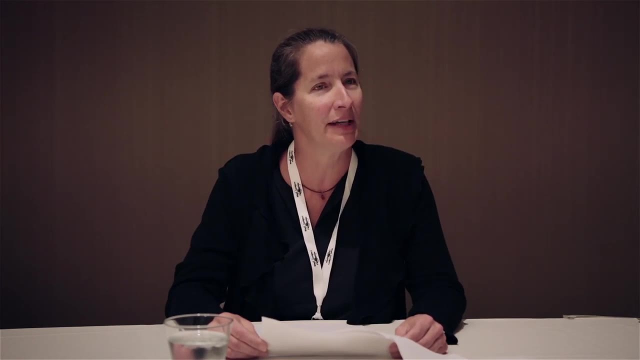 They want it. They can't quite get it into words, right, But they are really having these big thoughts that are up there. when we pause with them and give them time to struggle and listen patiently and attentively, We show them that what they're working on is important, that it's worth the effort to try to articulate. 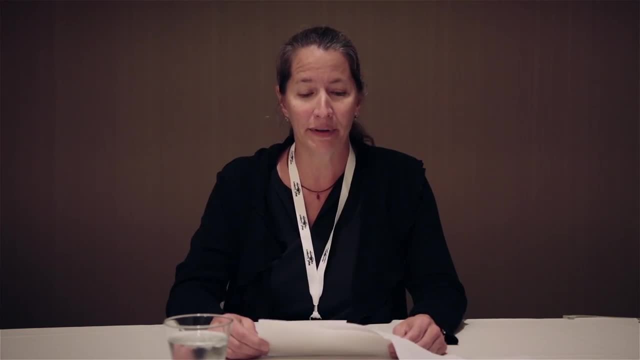 Sometimes, of course, we can offer them language- Uh, that might Help, and they latch on to the language, grateful for that little bit of help. but patients will often pay off, because what we think they're trying to say often turns out to be not the case at all. 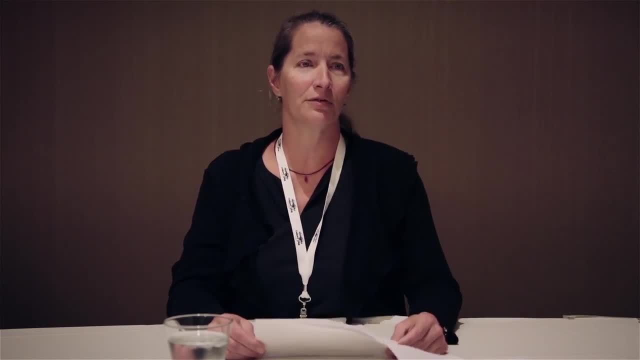 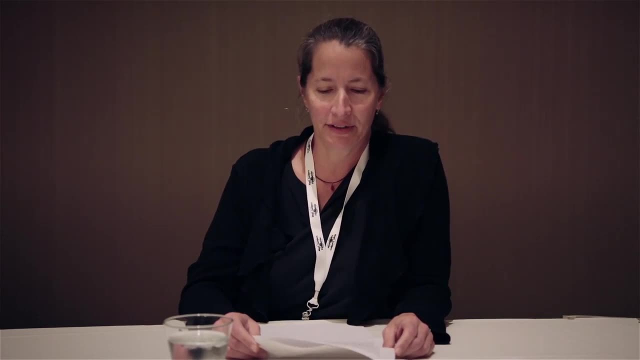 We can learn new things, then, about philosophical questions from talking with them and being patient for them to articulate their own thoughts. In a recent session with kindergarten students, for instance, we read Frog and Toad's The Garden. Um, in that story, Toad envies Frog's garden, which is beautiful. 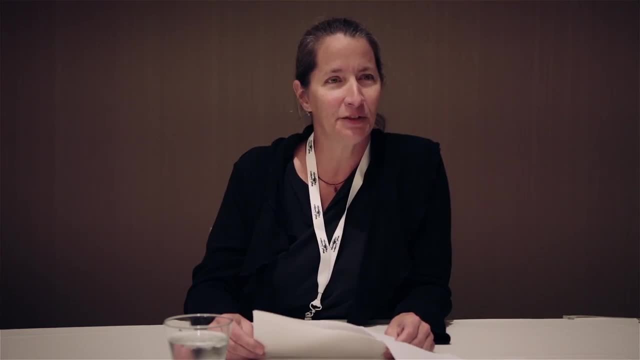 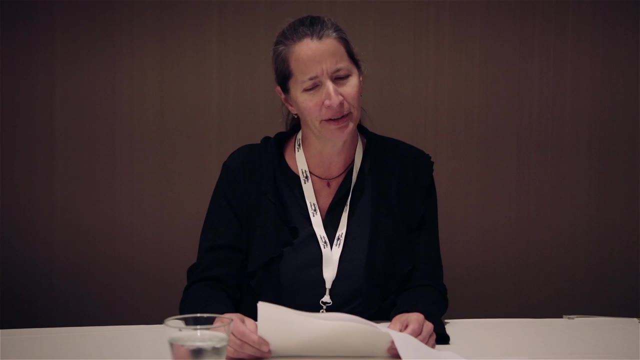 So Frog gives him Some seeds to plant, Toad plants the seeds and he's frustrated when they don't immediately start growing. So he starts yelling at them: start growing seeds? He puts his face closer and closer to the ground. They don't listen. 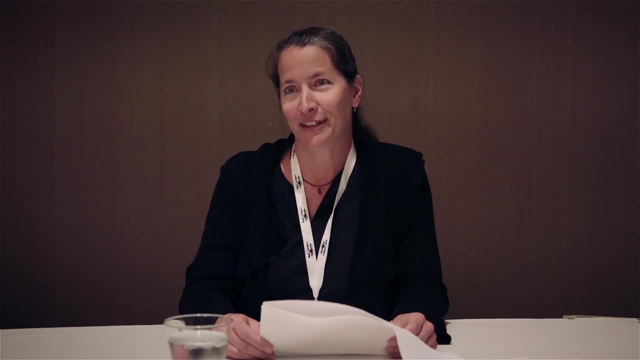 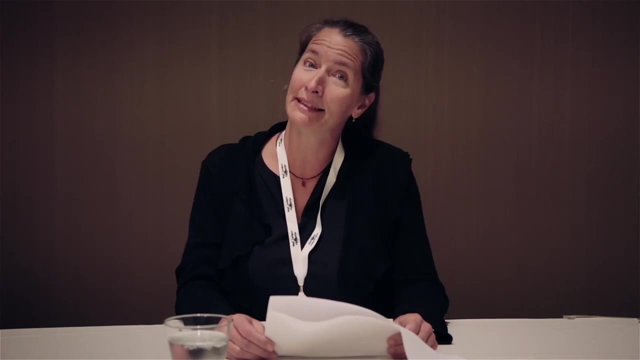 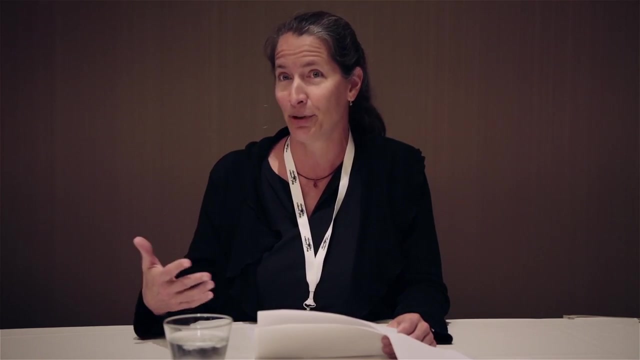 And so uh Frog says: you're scaring your seeds, right, You have to not scare them. And Toad thinks: well, what wouldn't scare them? Maybe if I read them a story, maybe if I take candlelight out at night, maybe if I play music to them, recite poetry to them? he does all these things over a number of 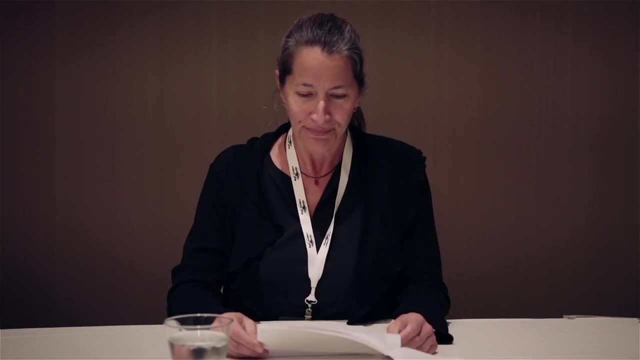 Days with a whole cycle of sunlight and and rain. And, what do you know? the seeds come up. and he says at the end of the story: you were right, Frog, it's really hard work to grow a garden. And the kids all laugh, of course, because they know something about gardening. 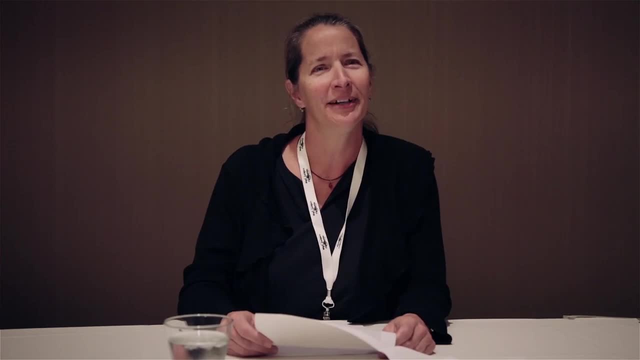 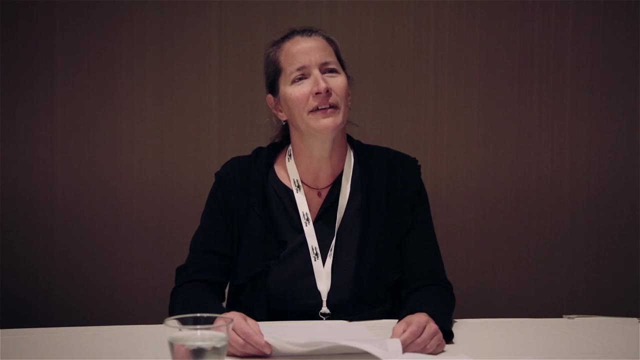 They all have seeds that they've planted in their classroom and they know that the singing and the playing music and all that sort of thing didn't do anything to bring these, these seats up. So we ended up having a conversation about patience. Was Toad impatient with his seeds in his garden? 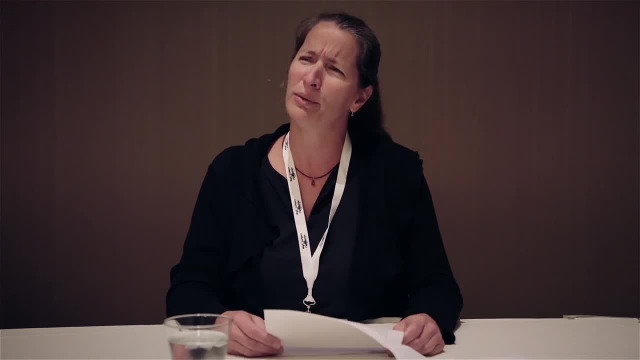 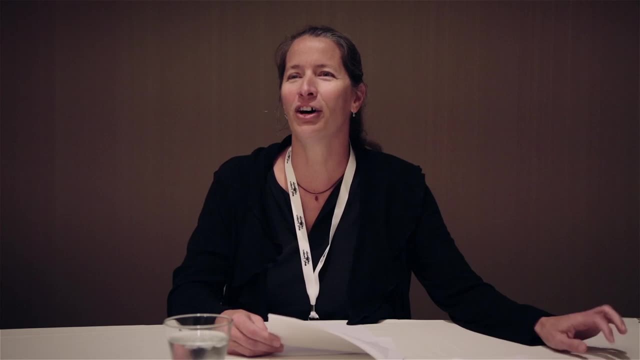 Why was he? Do you know about impatience? Yes, they knew, He said. so what? what is patience exactly? It's waiting, He said, but you can wait impatiently, right, All signs of tapping your foot, waiting impatiently. 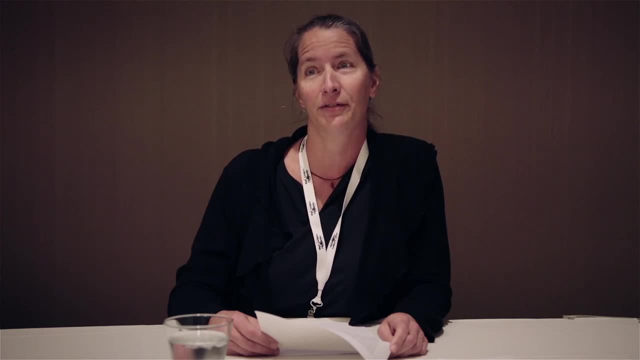 They said: right right, So patience is waiting calmly for something. And then we got into a discussion about whether, if you wandered away from the thing that you're patiently waiting for, that still counted as patient. Right, Right, So patience is waiting calmly for something. 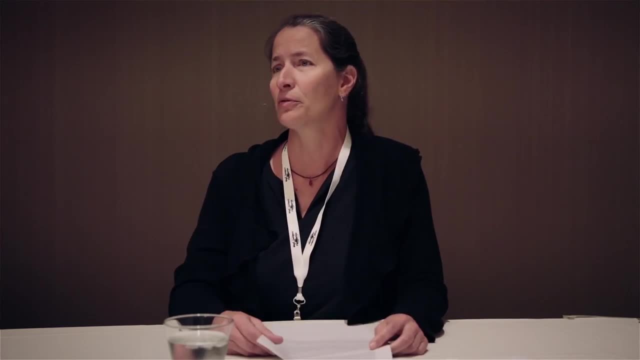 So one little girl said she would be impatient, She would get home from school and her dad was making dinner and it was taking too long and he told her to wait patiently, And so she would go do something else like play a game or read a book. 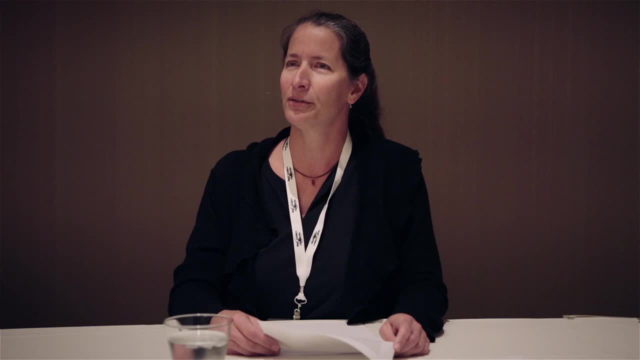 And I said: but does that count as patience if you're not actually waiting? Oh, I was waiting. I was just reading a book too at the same time, And most of the classroom agreed right. That's a good. that's a good example of patience. 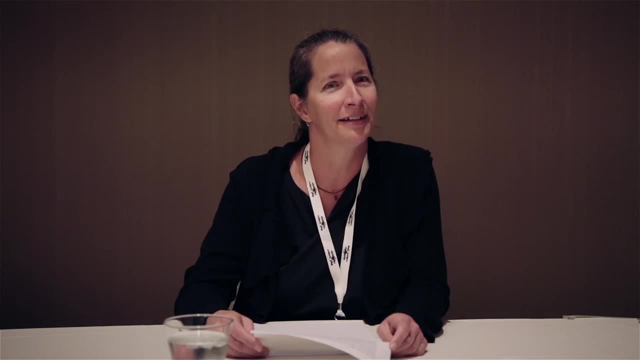 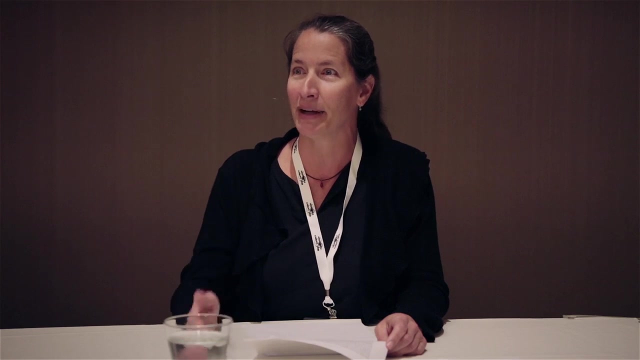 And then it came up: well, what if you forgot that you were waiting For the dinner because you were so engrossed in the thing that you were doing? right? Does that still count as patience? And I'd say a good number of them thought that was the best example of patience, because you wouldn't even be going back to your dad to bug him to do it faster, right? 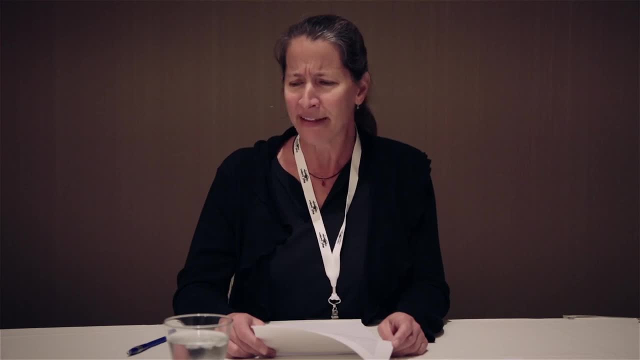 You would just be completely focused on something else. And the other group of them said: no, no, no, that's not. you can't be patient anymore if you don't even know what it is that you're waiting for. You don't recognize that you're waiting at all right. 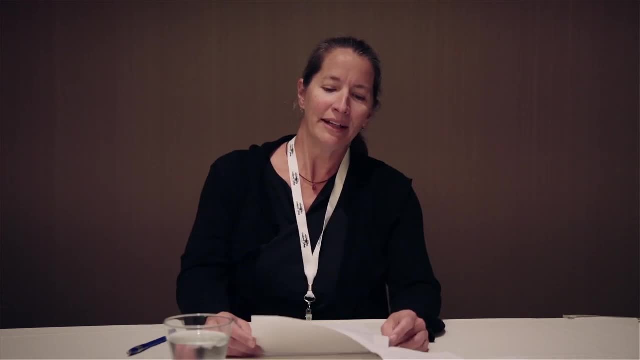 There's no waiting, There's no way that it could be the same sort of thing And we ended up having a really interesting back and forth where they wouldn't right, they're five-year-olds. they wouldn't even let me get in. 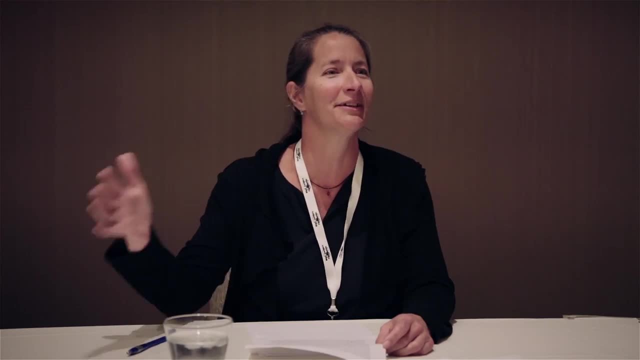 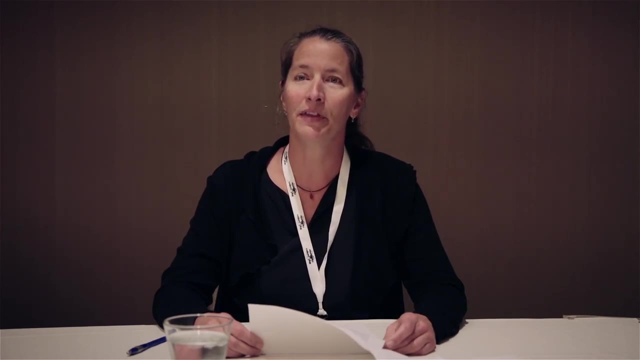 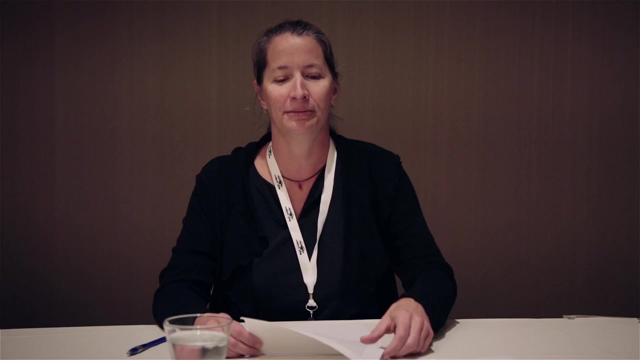 They were arguing with each other. I disagree with Elijah, because you know here's my reason. And then we got to the question of whether or not one could be too patient, And some of them really thought that forgetting what you were being patient for was a sign of being too patient, overly, extremely patient. 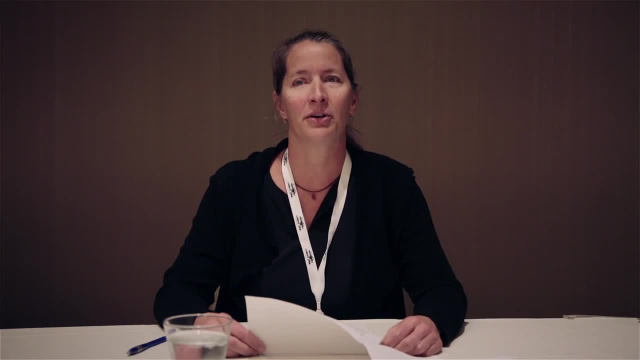 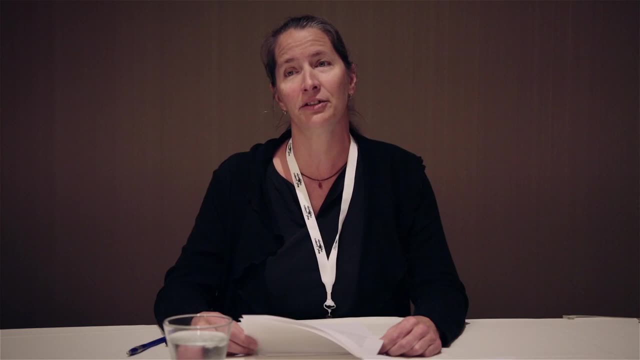 And others thought again that it was that still counted. It was counted as having some level of patience there. And we started thinking about different examples And we had done a unit on Martin Luther King Jr And so we talked about how he said his people had been too patient, waiting for laws to change. 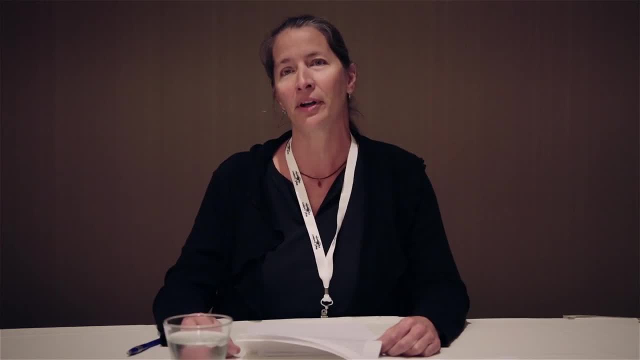 And they really picked up on that and they started thinking for themselves about examples in their own five-year-old lives where they would have the experience of having been too patient. So again, I think I went into it not having really thought that much about patience at all. 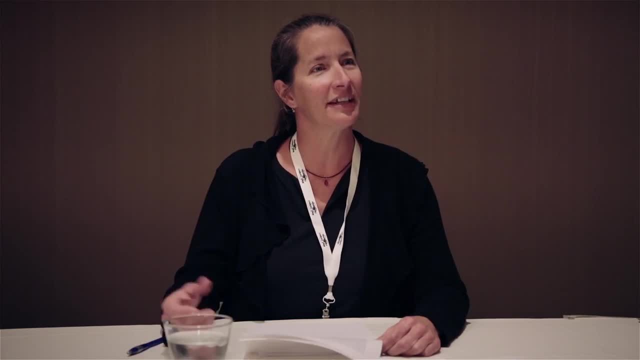 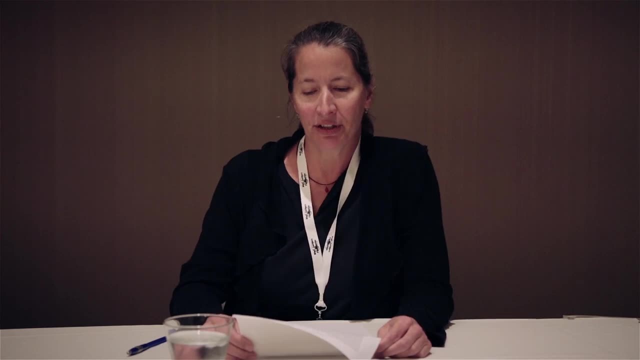 And discovered that there were these interesting features of patience that they could bring out that I wouldn't have been aware of before. Okay, Engaging a child in a philosophical discussion is also a way, I think, to get to know him better. Although we spend time with our children, we observe them astutely, we talk with them about our shared experiences and plans, so much of their inner lives is inevitably hidden from us. 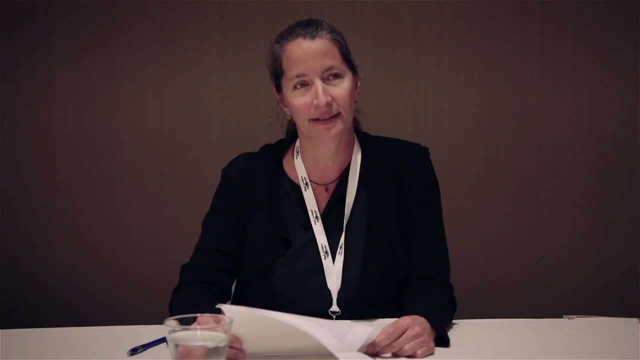 Talking philosophically with a child allows us access to some of the curiosities and concerns they might not confess In other circumstances. like many families in our household, we struggled with getting our kids to sleep in their own beds, after enjoying a cozy family bed in the early years. As the weaker parent of the two, I occasionally relented and let the kids have sleepovers with me. when my partner traveled for work One night, curled up in my bed next to me, my son said: do you know why I like to cuddle at night? 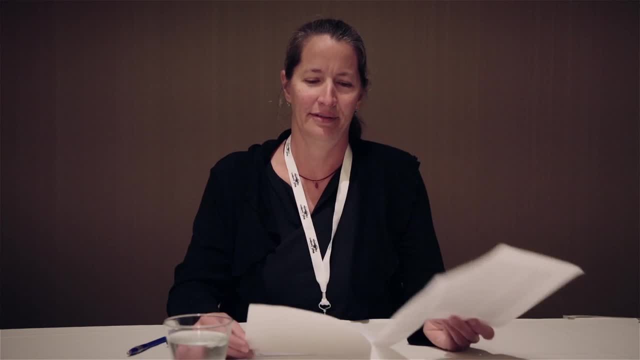 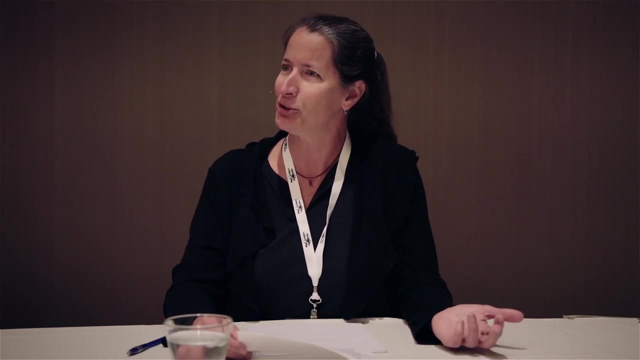 Because then I feel completely safe. I didn't have any idea. I didn't have any idea He wasn't feeling completely safe. He has a cool loft bed. It has Lightning, McQueen sheets- Right. It is exactly the thing that he wanted and loved. 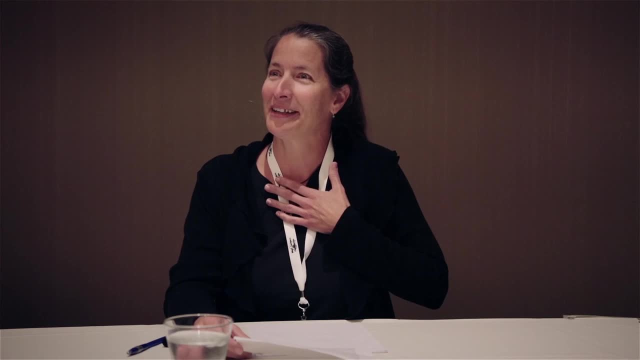 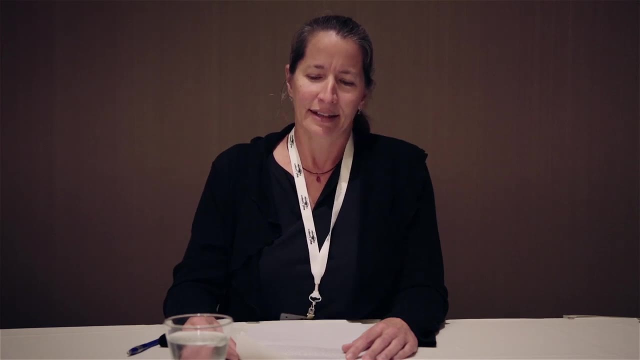 We talked about it a little. I love that he felt completely comfortable. but why would you not feel completely comfortable in your little bed that we've made for you? He said I wanted to know what scares him. He said dreams he might have shadows on the wall, funny noises. 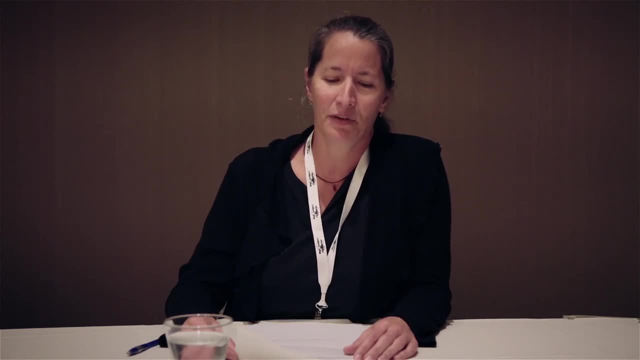 When I suggested that he think about it, he said: I don't know. He suggested that he think about good things as he's falling asleep. He should focus on the positive as he's going to sleep. Think about your birthday, Think about your friends at school. 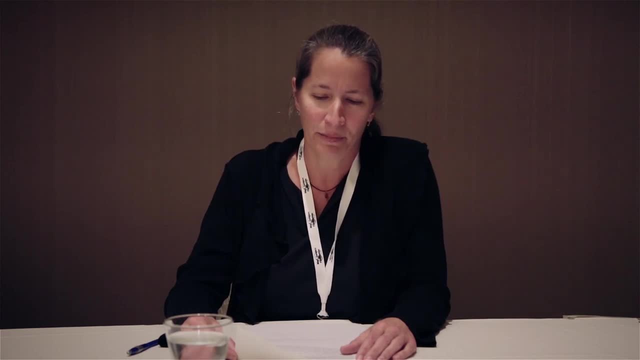 He told me it doesn't work because- and this is a quote- I don't control my brain at night. Oh, I said, As you might imagine, this led to an interesting conversation. What does control your brain at night? Does anyone control your brain? 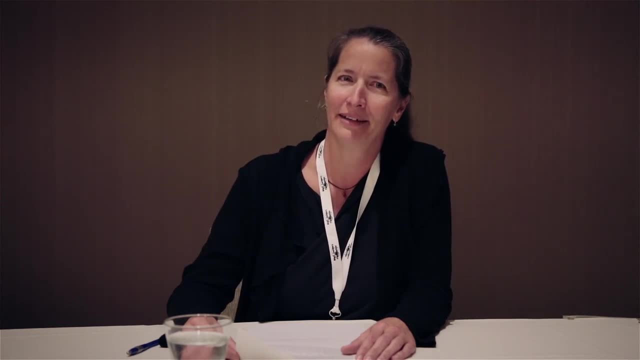 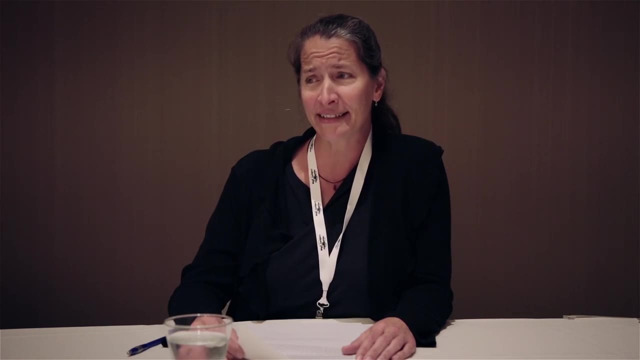 Who are you if you don't control your brain at night? Are you your brain? during the day? Are you different from your brain? We had this fascinating discussion. I can't say that it soothed him at all or made him feel more safe in that bed. 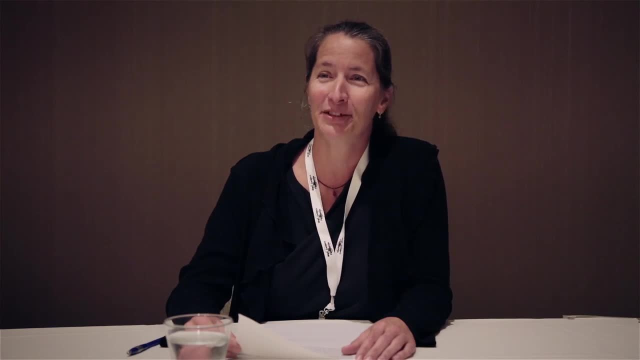 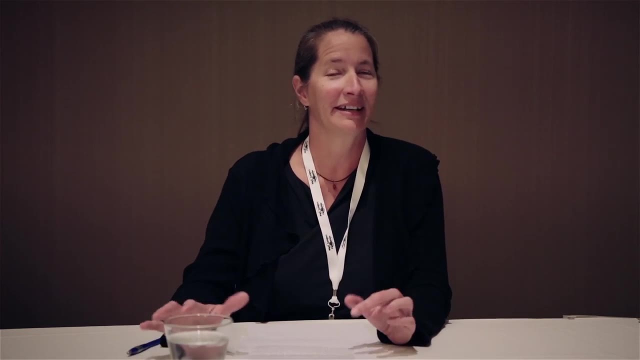 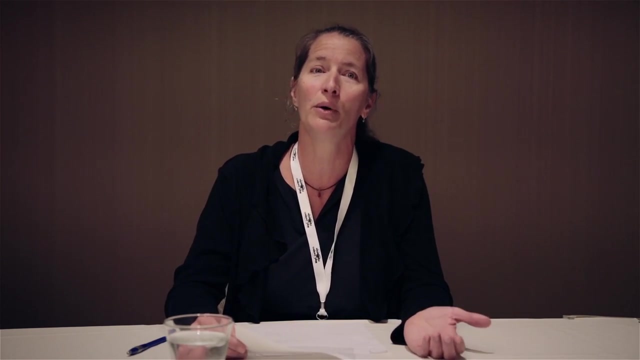 Like most new students of philosophy doing philosophy- we were talking the other day with Dan doing philosophy- we're sowing confusion. often We're getting them to question assumptions they've always taken rather than making them feel safe. But I do think he felt better knowing that other people wondered about these things and worried about these things and thought about them in similar ways. 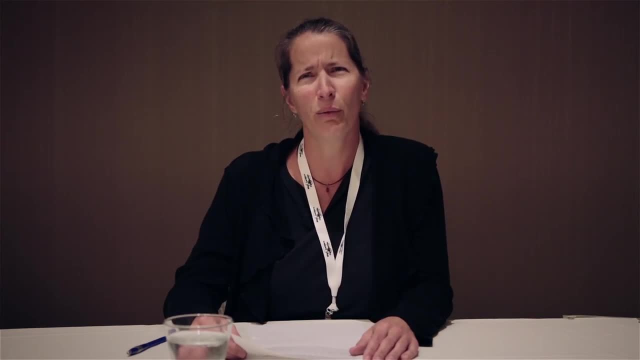 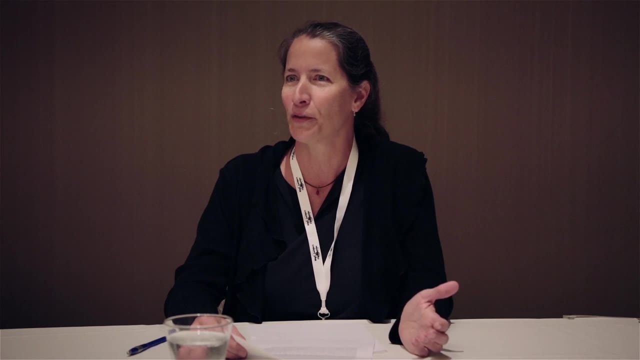 It also made me question a thing or two. So first, why do we have this traditional sleeping arrangement and family norms? Why do we have a whole industry of books that are about the Ferber method and how you can let your kid cry it out at night so that they'll sleep in their bed? What's going on right in our culture where we think that is the appropriate thing to be doing? And secondly, how does the situation look from the perspective of a child who wonders why the loving parents who are helping all through the day abandon him at night, when he is most scared to be alone? 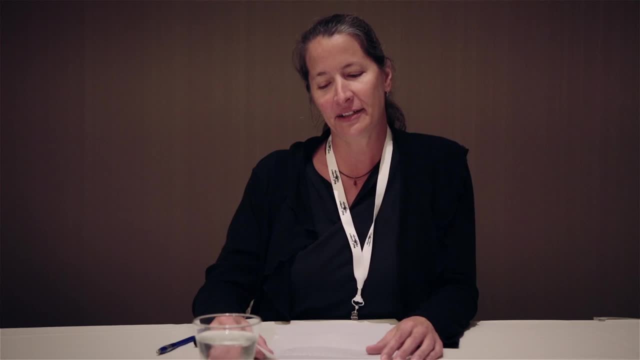 Some of the consequences of raising a philosophical child, of course, are not obvious short-term benefits for the parent. Count on your children to find counterexamples to any claim you make and refuse to listen to the purported truisms you repeat, having learned them from your own parents. 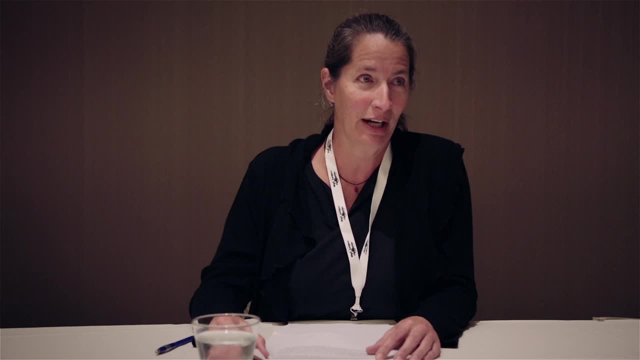 This point is important. This food is good. You need to eat it. Be grateful. Yes, blueberries are blue. They'll be met with such parries. as tastes are different. You cannot know how this tastes to me because you cannot be in my head. 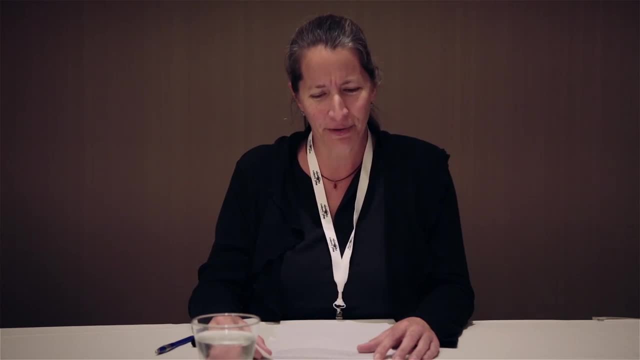 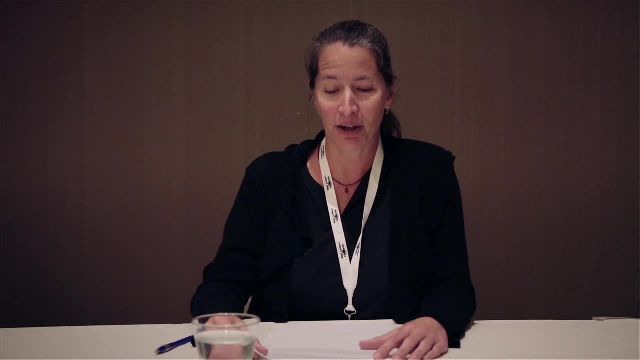 Of course, they probably say that anyway, even if you weren't a philosopher raising them, But it seems like it happens a lot more often when philosophical thinking has been encouraged in them. My daughter, for instance, has become the queen of saying: that's just the way you think, mommy. 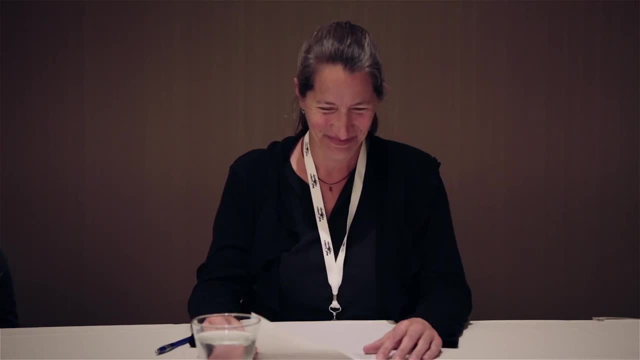 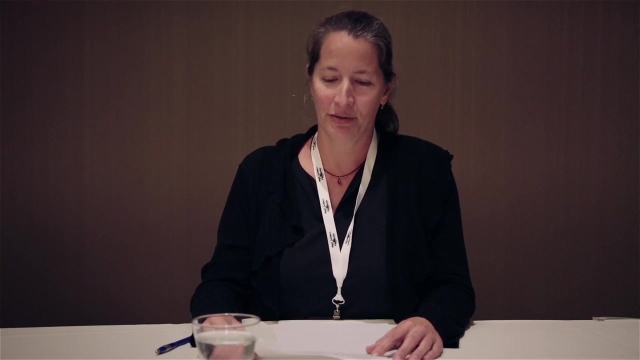 Try to see it from my perspective for a minute. They also explore potential arguments to thwart your authority. As a funny example, I guess I told my son you can either have a small sleepover party, birthday party with a few friends at our house. 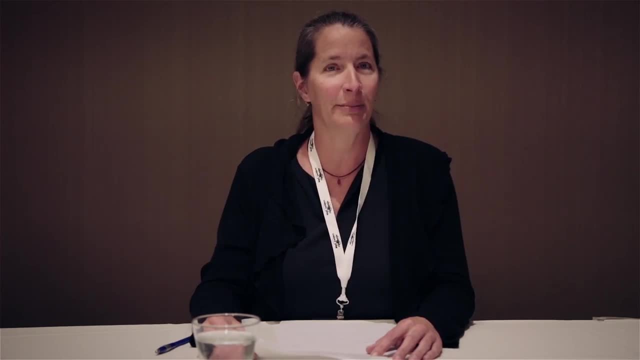 or you could have a larger birthday party with the whole preschool class at a bouncy house. This is a common thing in Seattle, But not both. Why not both, he asks. Yes, Funds and parental sanity were, of course, at play, but I also told him that if we did the big party, 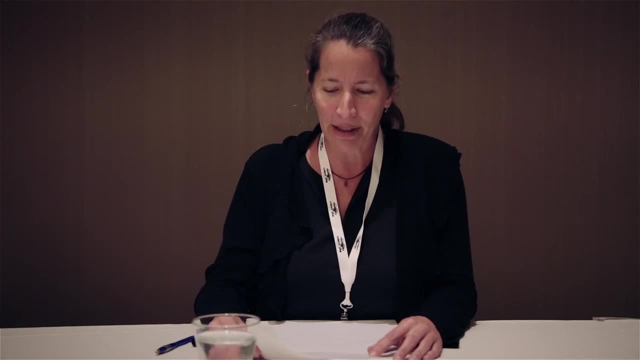 I don't know what I was thinking, but this is what came out of my mouth. If we did the big party and some friends learned that others would get to continue for a fun sleepover and they weren't invited, they'd feel sad. 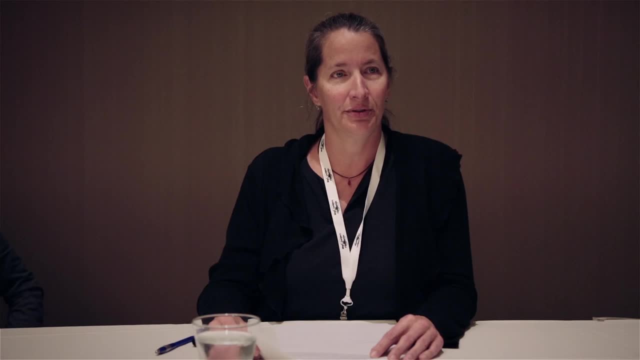 We should avoid making our friends feel sad. so he had to choose. He pondered this and then said: but missing just a little of the party is better than missing the whole thing, And if we have a small party, most of them won't get to come at all. 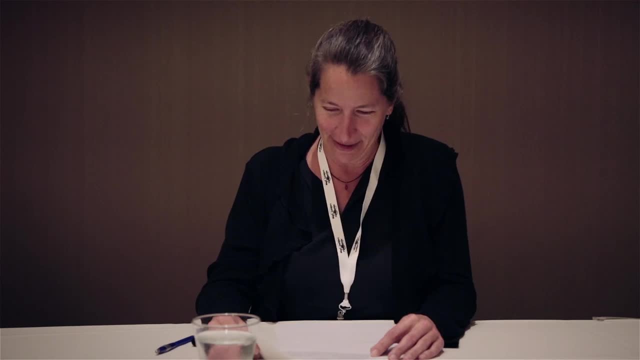 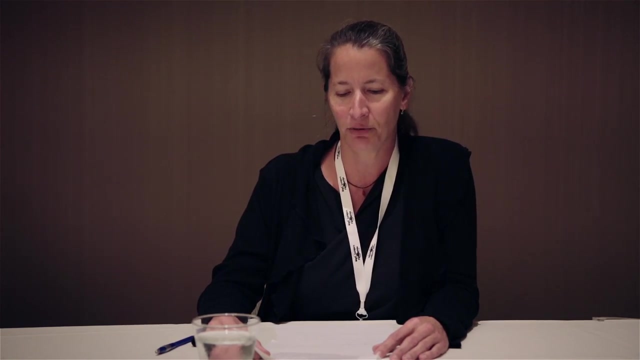 I was forced to fall back on the parental sanity defense. Raising a philosophical child offers daily reminders of the need to sharpen our own arguments and reasons or reassess our reasons, But to my mind it's a distinct pleasure as well For the kids. they learn through dialogue, through practice and reflection. 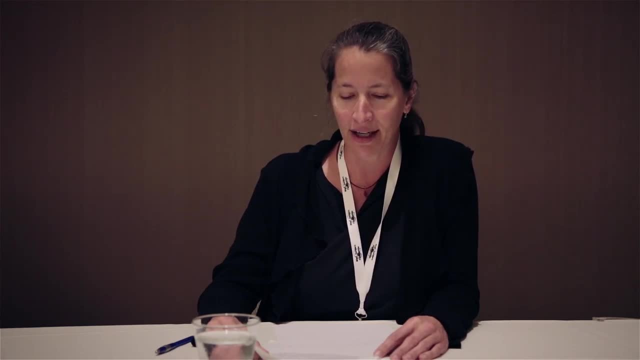 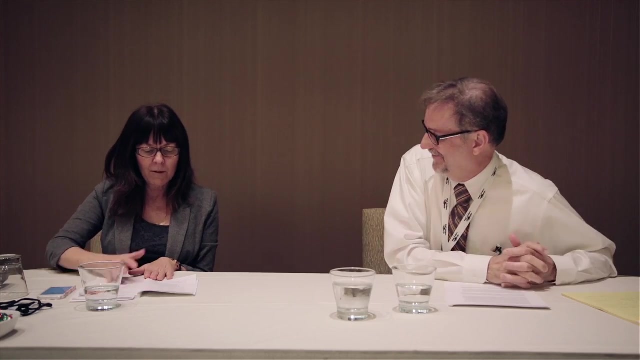 to think carefully, articulate their thoughts, recognize and consider other perspectives and share in the ongoing process. They learn from the project to figure out how things are and how they ought to be. Thanks, Okay. so our final speaker is David Adams from Cal Poly, Pomona. 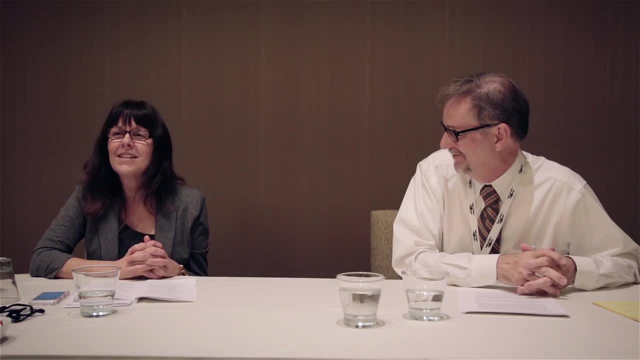 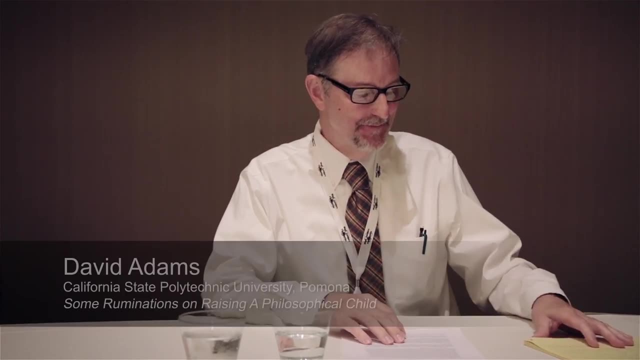 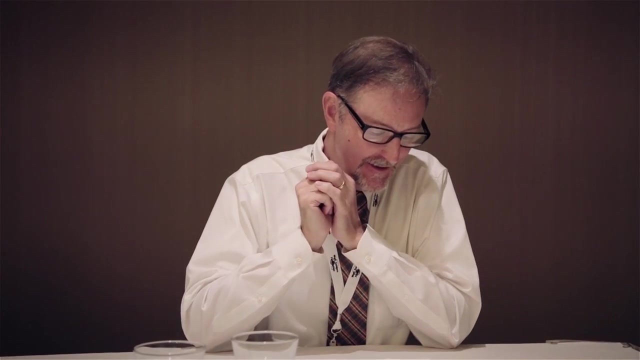 and his talk is Some Ruminations on Raising a Philosophical Child. Okay, thank you. So I'm older than my co-panelists and listening to all of the great stories that my co-panelists have told me, you know sort of the phenomenology of raising a child. 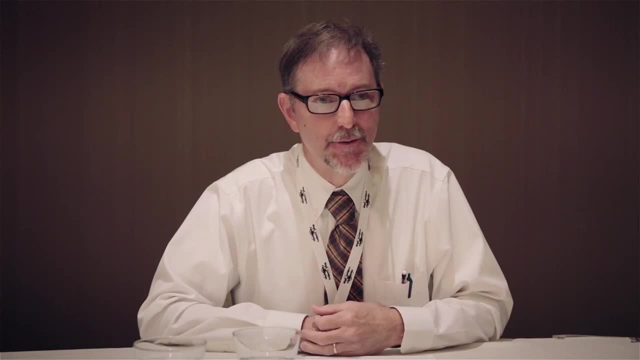 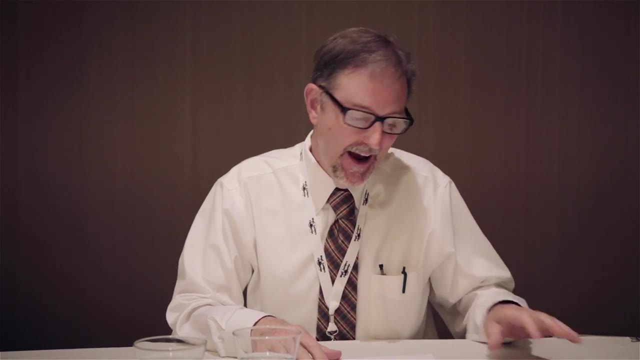 My wife and I have three kids. They're all now in their 20s and 30s. So I remember some of these discussions, but not as many of them as I would like to. So I kind of took a different way of thinking about the topic of our panel. 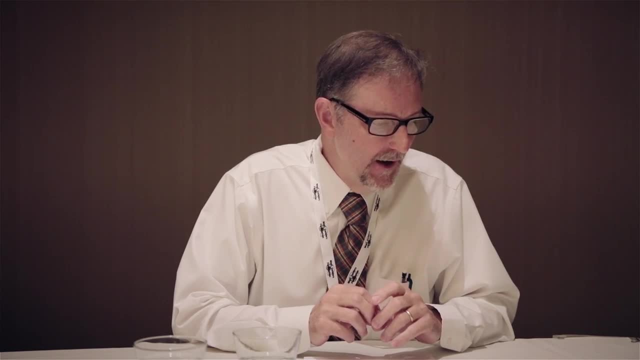 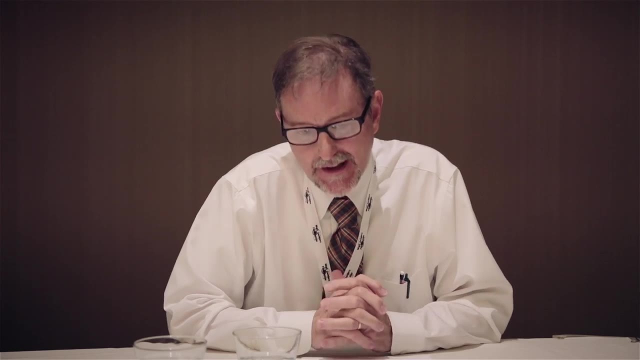 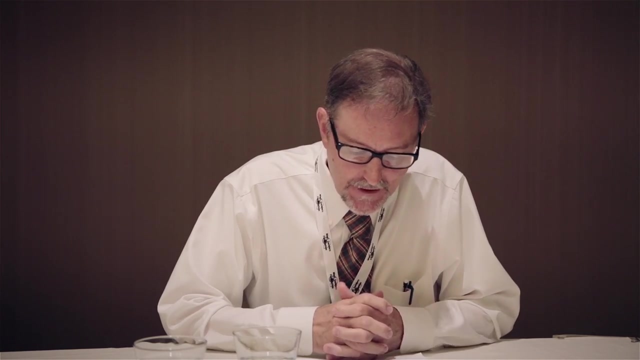 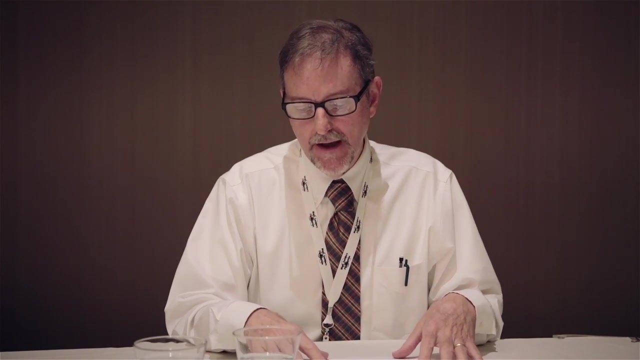 Raising a Philosophical Child. My oldest daughter is a historian, My son is soon to be an attorney, My youngest daughter is a musician. They're all capable, self-reliant professionals. So I put to myself this, you know- question that was raised by our panel. 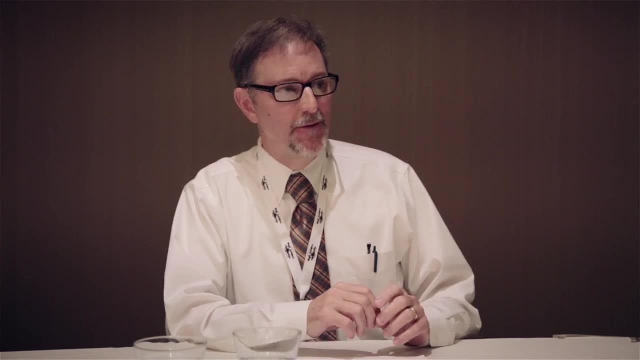 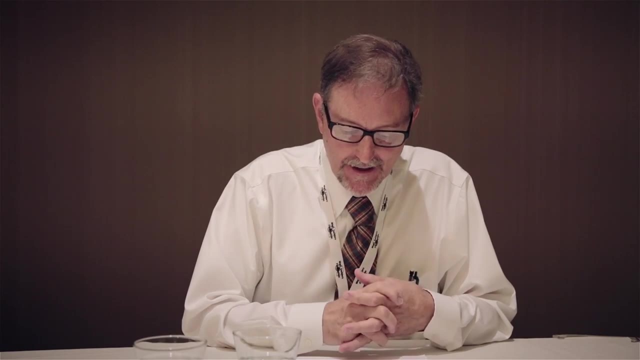 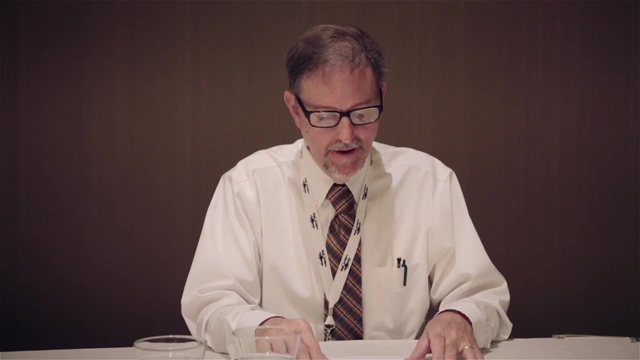 And my question was: did we raise philosophical children? And I confess that I wasn't sure quite how to answer that question. Each of our kids is headstrong and independent and is accomplished at expressing his or her own views, arguing for what he believes capable of reflecting upon her ends in life. 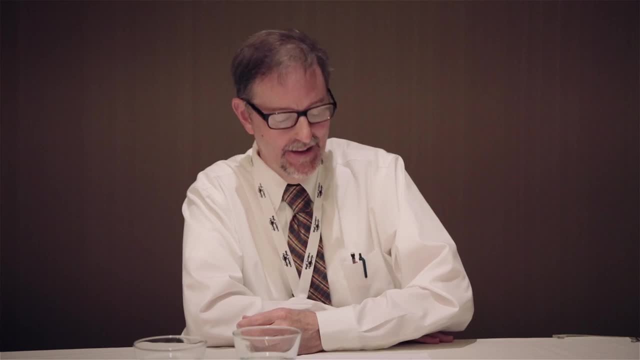 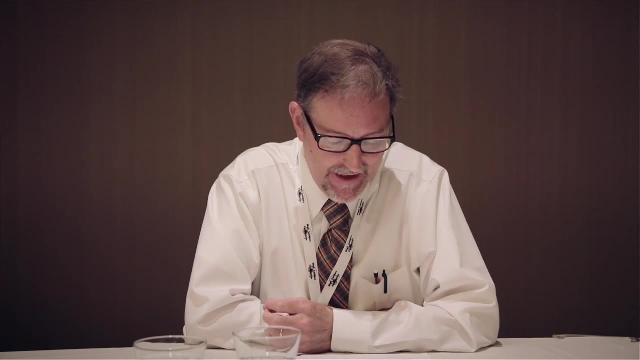 Is that enough, you know, to answer my question in the affirmative. Our son, Aaron, majored in philosophy in college and gave serious thought to whether he should do postgraduate work in the field. No, I told him he shouldn't. 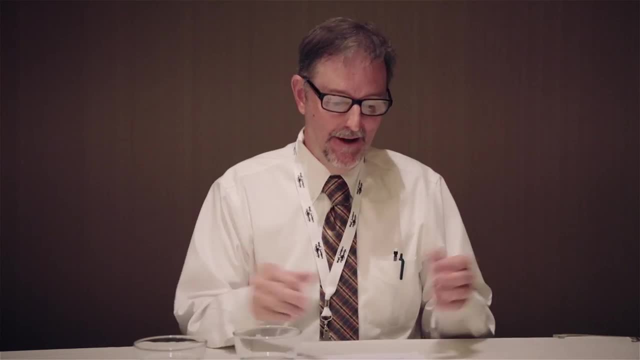 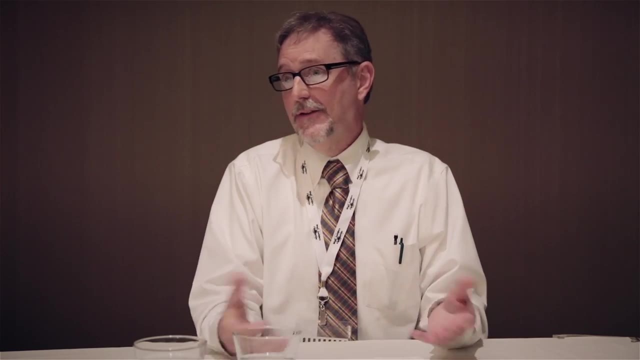 And I didn't give any major proof that we gave him a philosophical upbringing. So to address my puzzlement, I found that I sort of wanted to get clear on what it means to have raised a philosophical child, And my strategy was to sort of think about that in the context of 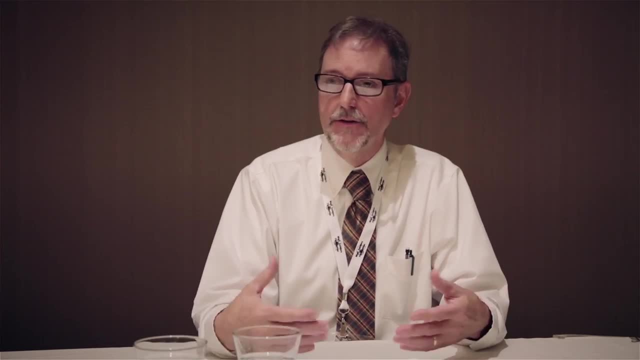 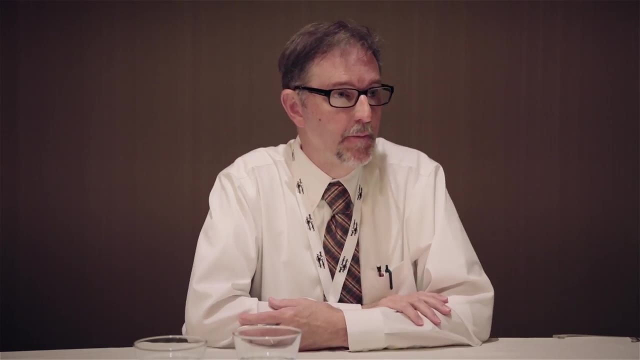 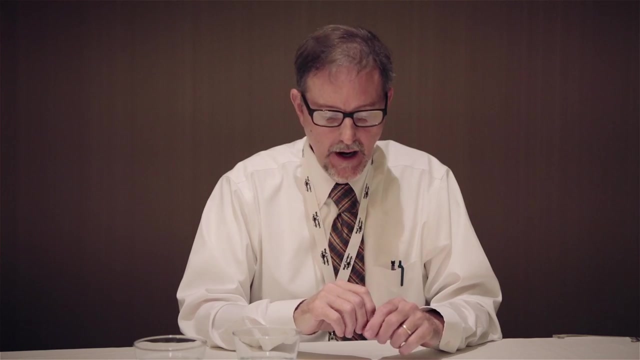 maybe a more familiar parental undertaking. So I thought about raising a musical child. so what might that look like? And then I tried to think about what opportunities that might have for my philosophy. So I suspect that for some parents, raising a musical child means bringing up your child with the aim of making her into a musician. 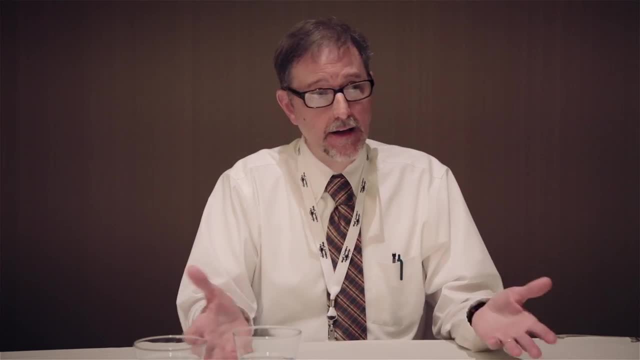 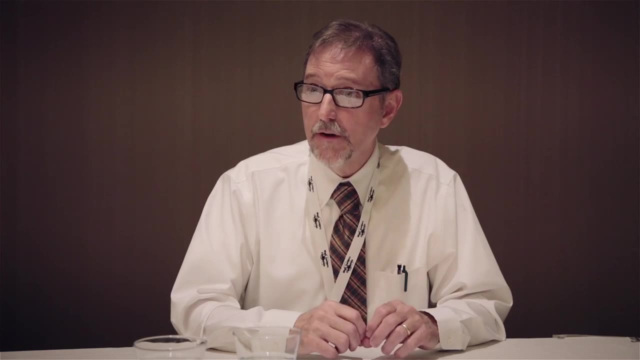 And I've met not a few parents for whom I think that was kind of a defining parental undertaking. So similarly then we could imagine a parent for whom raising a philosophical child means embarking upon sort of a project to make your kid into a philosopher. 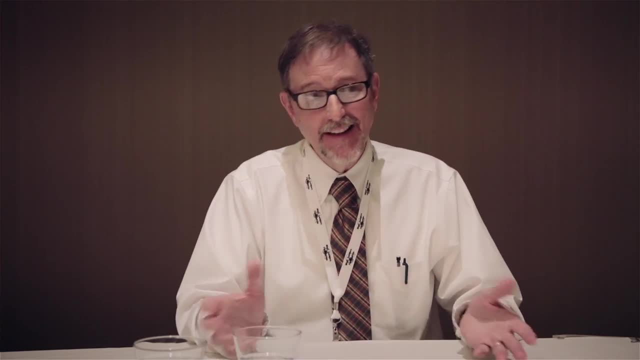 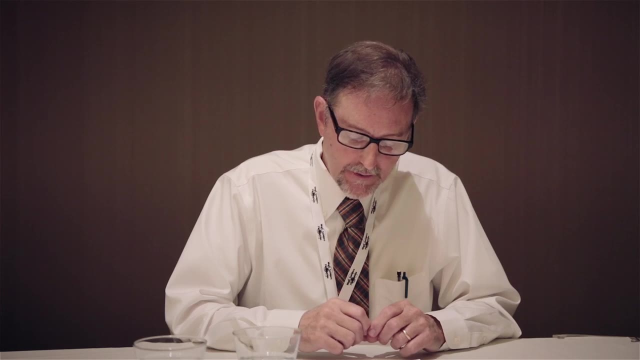 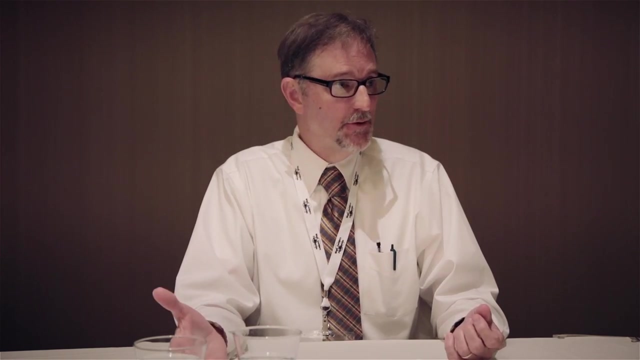 I think we would be wise to reject that idea or that conception of what raising a philosophical child amounts to, For the idea of pursuing that as a project I think is difficult to motivate in ways that aren't kind of disturbing or troubling, And you might consider a couple of ways in which that could happen. 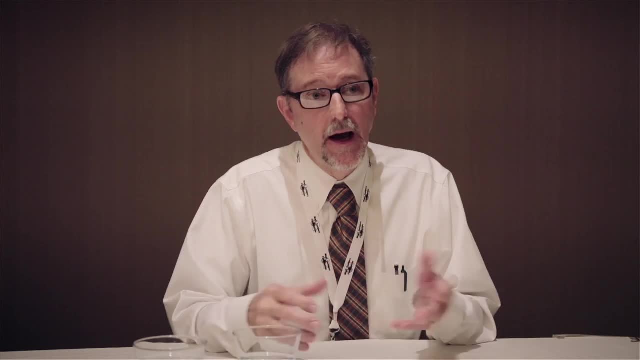 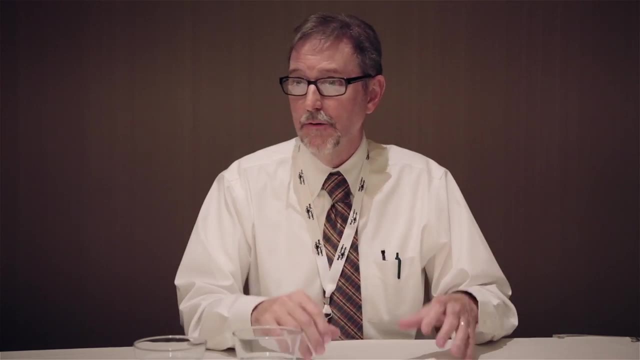 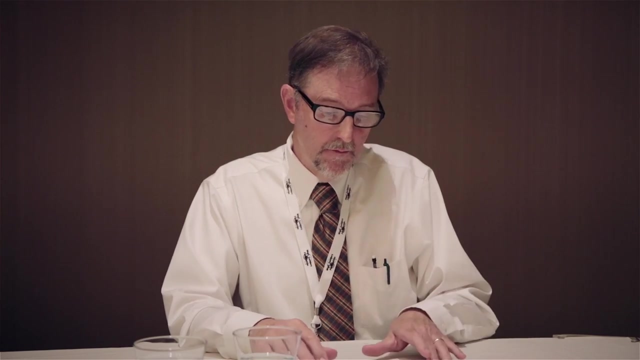 So a parent, for example, might set out to bring up his or her children so that they hold what the parents, what the parent believes to be or takes to be the correct views regarding some dimension of life that's important to the parent. So the understanding of this understanding of rearing a child, I think is most obvious in the effort to bring up religious children. 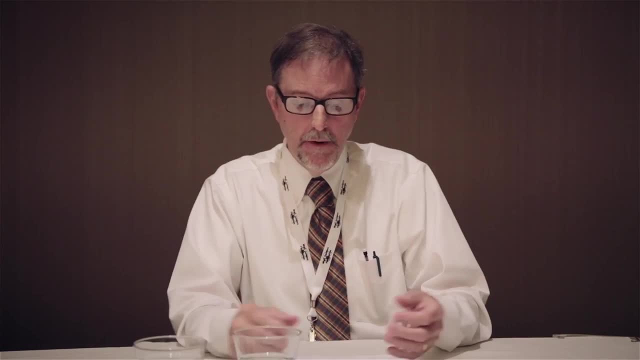 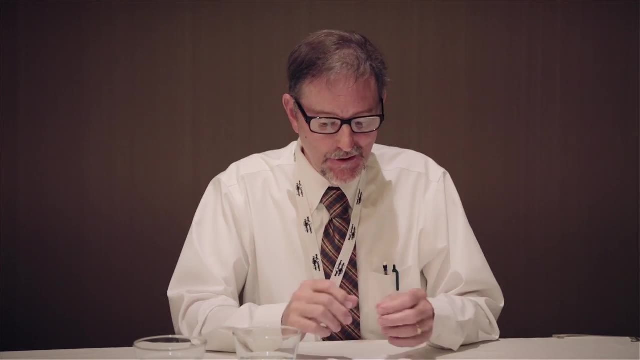 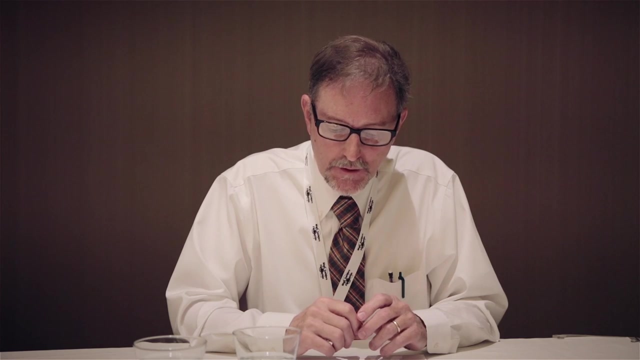 Where the goal is often to have the child take up the doctrines and the beliefs that the parent favors. Something similar, I suppose, could happen in the musical case, And again I've encountered some especially domineering- Domineering parents, I guess I would describe them- who raised musical children, apparently with the aim of having their kids. 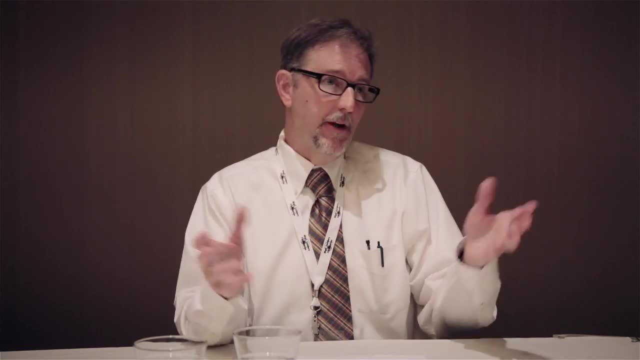 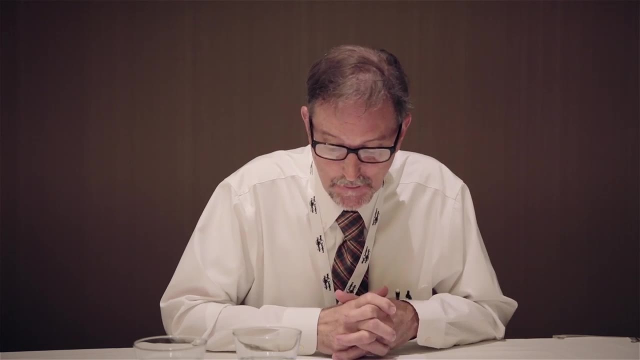 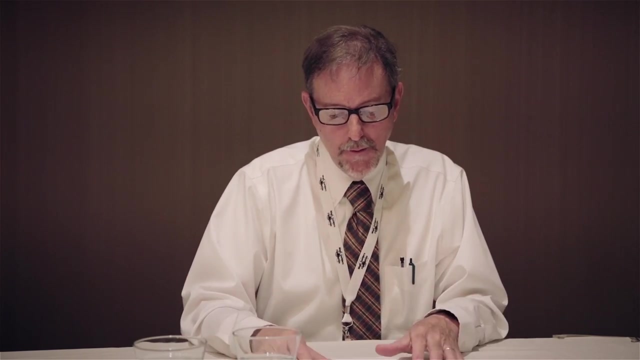 embrace what the parent regarded as sort of the correct musical aesthetic, To disdain hip-hop, for example, in preference to orchestral- you know- repertoire, or to prefer Bach to Bjork or Bruckner to Beyonce. So in like fashion we could try to imagine, I guess, a parent whose idea of raising a philosophical child. 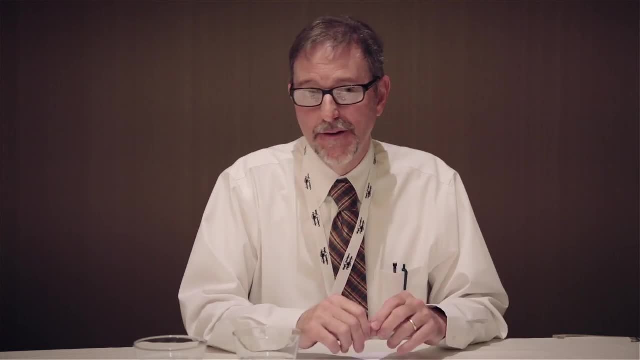 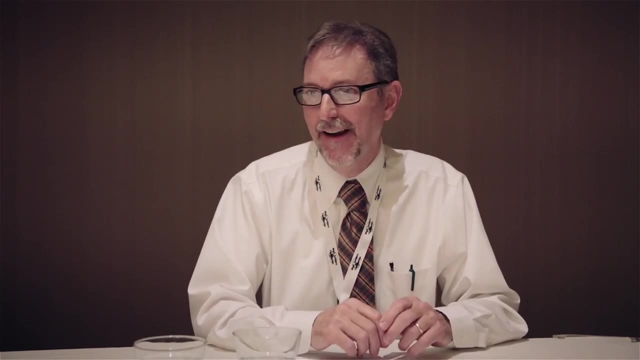 means that they're going to have to raise a philosophical child, And that means having the child adopt the parent's favored you know philosophical positions, So you know, suppose I raise my kids to believe in, you know, epiphenomenalism, say, or to be compatibilists. 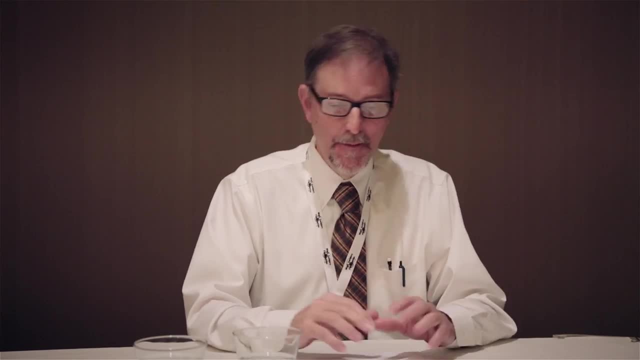 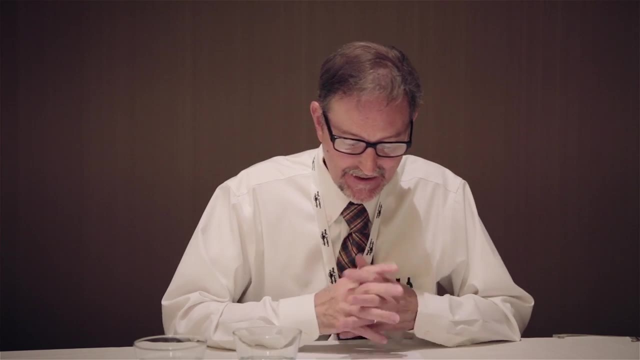 And so you know, I accordingly, you know, compel them to memorize arguments for compatibilism and admonish them that it's not a wretched subterfuge. you can't not understand it. Warn them of the evils of hard determinism. 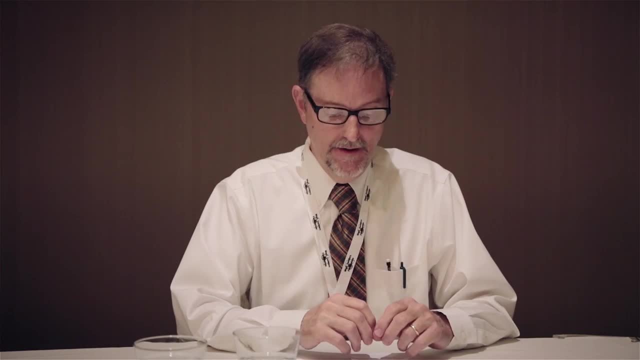 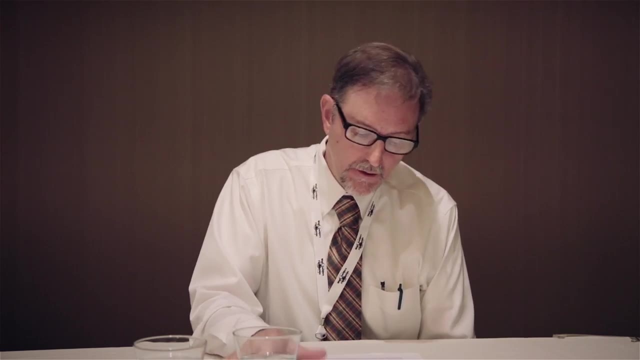 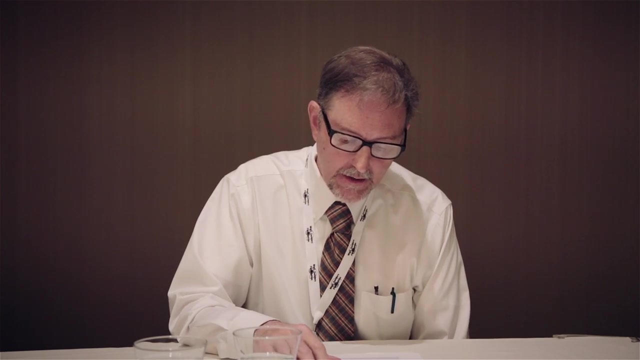 Well, I mean, it's easy to see why. that's kind of a misguided acknowledgement, You know, silly project, Just as we want our children to love particular types or styles of music as a result of their own, I guess, sort of realizations about what moves them aesthetically. 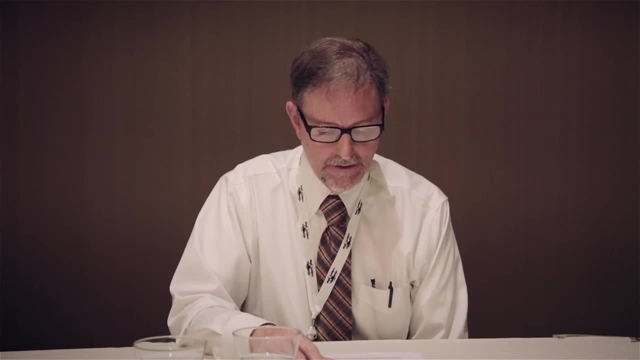 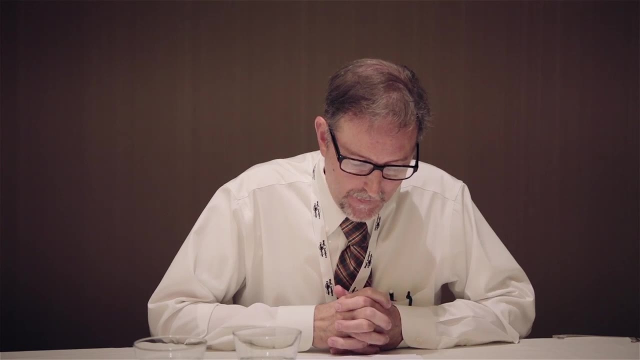 so we want people to take up particular philosophical positions, obviously in a way responsive to reasons and not because somebody has told them to do it. So that doesn't seem promising. Another equally suspect reason, I think, to raise a philosopher flows from: 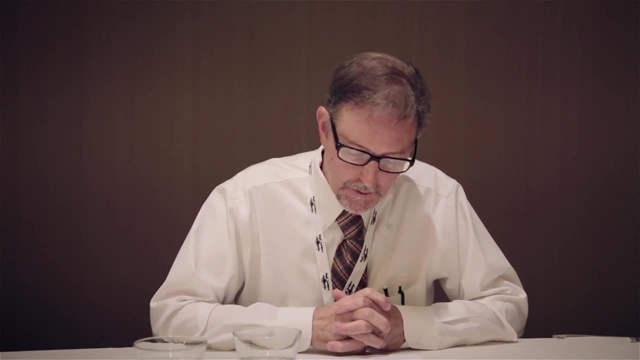 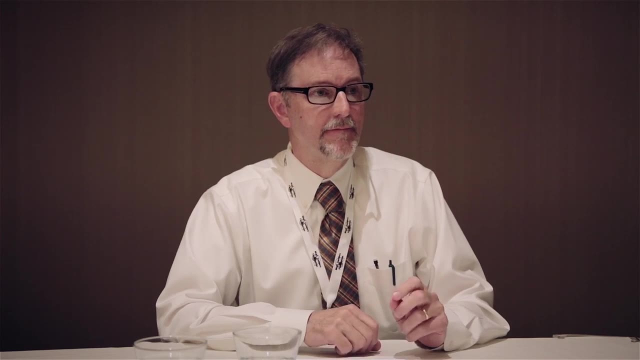 From a specific desire. right, I want to raise my child to be a philosopher or a musician, whatever, because I want to raise someone, in all significant respects, just like me, right? So that project, of course, is disturbing because of the reasons that I have for pursuing it. 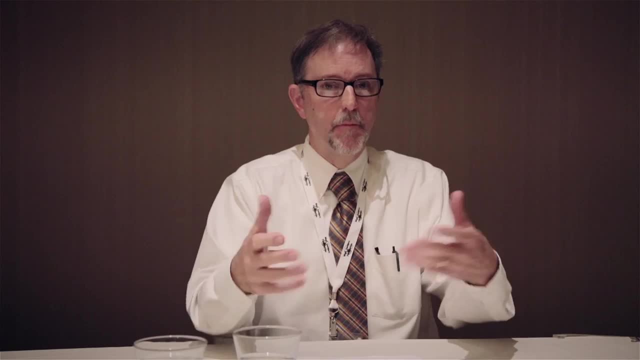 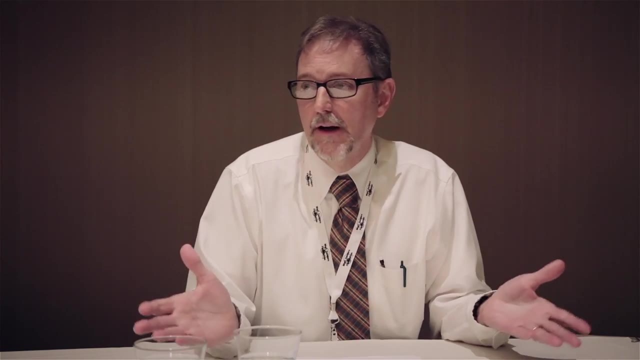 as well as the likely effect upon a child of a project inspired in that way. So on the face of it, you know my impulse there is just manifestly narcissistic, right. I mean I want to you know sort of self-congratulate. 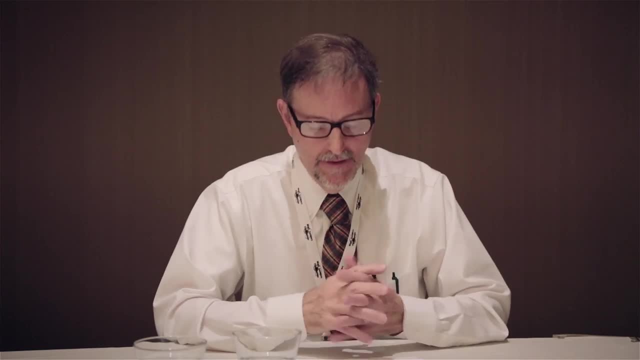 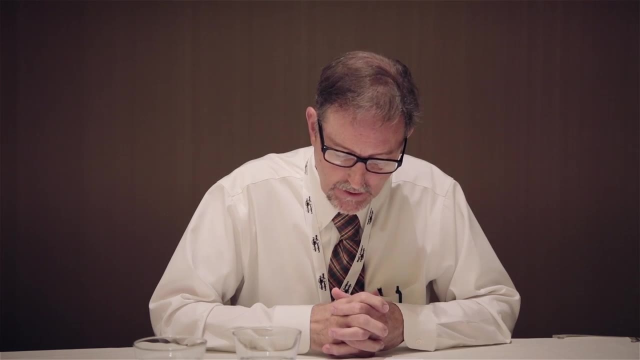 I mean I want to have a self-congratulatory desire, to have kind of a mini-me running around. Not surprisingly, the impact on a child of a project, that kind of self-involved undertaking, is almost certain to be a life dominated by a stifling set of expectations. 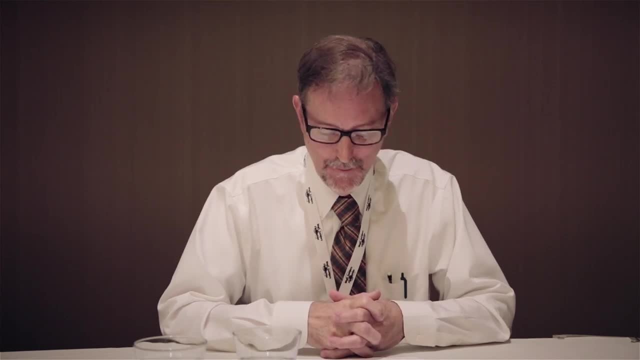 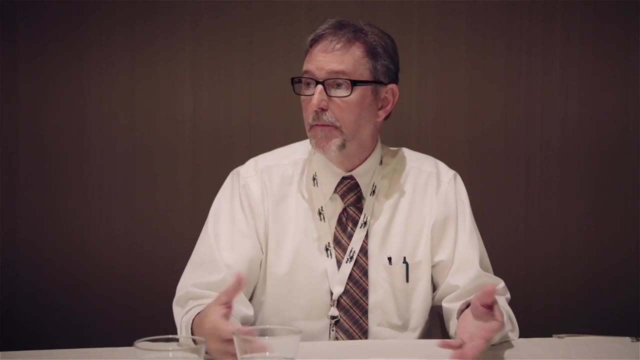 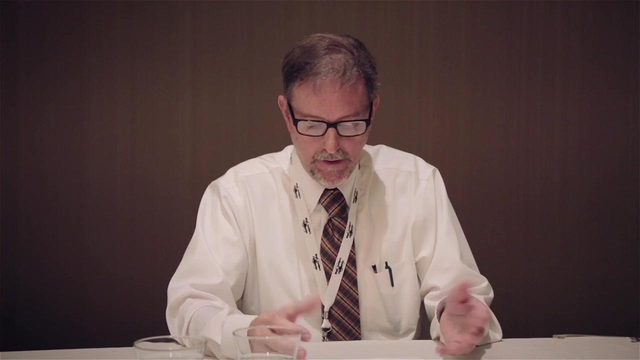 Why didn't you get an A in that epistemology seminar? Why can't you play that concerto at tempo? So a life confined by such demands arguably undermines the proper conditions for the formation of genuine autonomy. So if raising philosophical offspring is not best conceived as rearing philosophers, 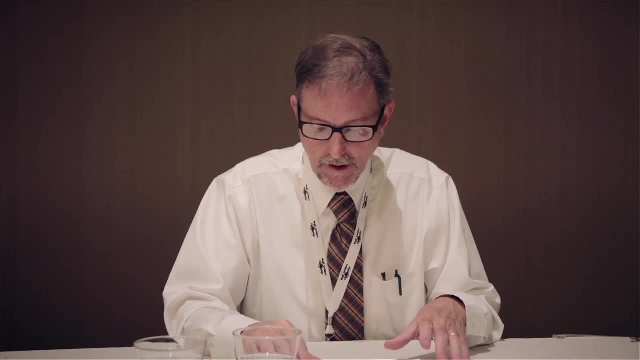 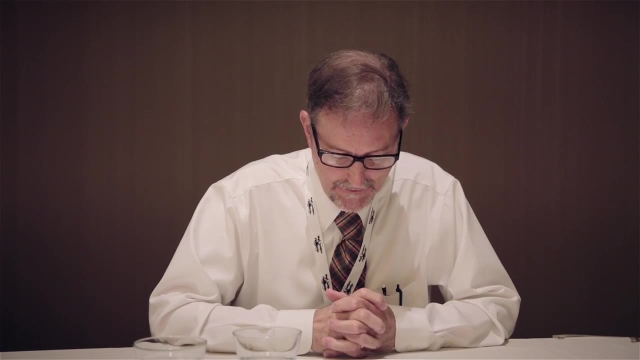 then how else might we think of it? So, a few months ago, I'm a grandparent, you know I'm getting old, but we were visiting my oldest daughter, Aubrey, who has a seven-month-old, And so I asked her: you know, do you think that I, you know? 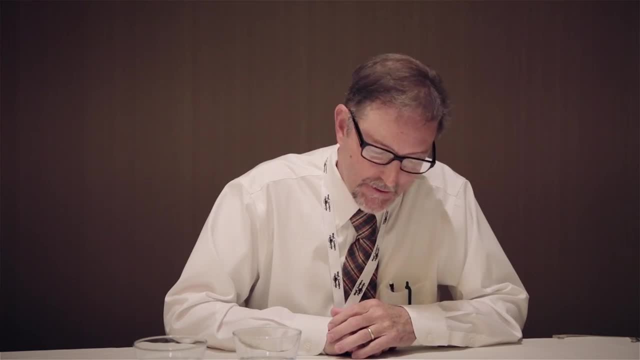 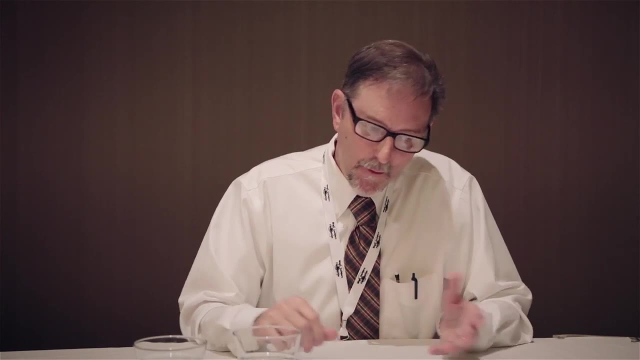 raised you and your siblings to be philosophical. And she thought for a minute and she said: absolutely, Just look at how relentlessly we argued, We argued with you about everything. So her implicit, I think, conception of raising philosophical offspring you know. 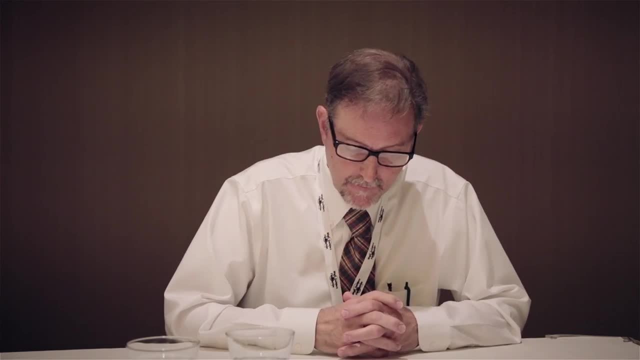 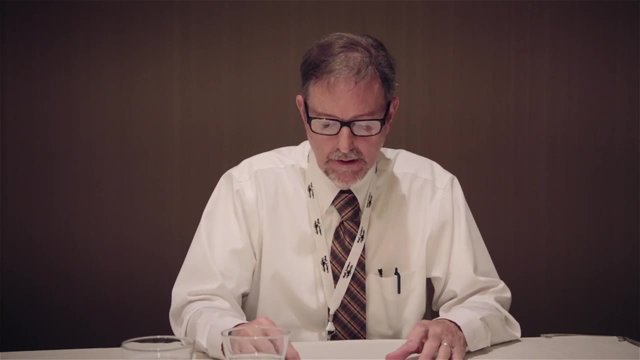 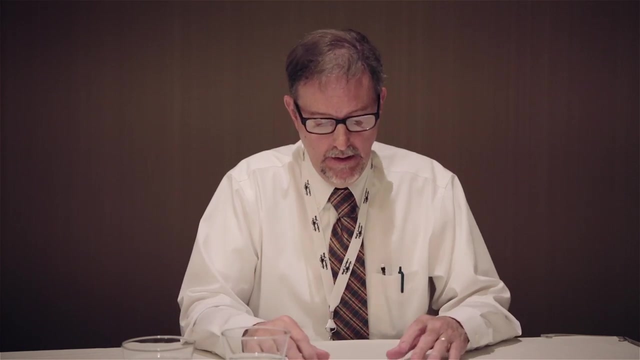 which is entirely familiar to most of us, I think traces back to Matthew Libman's early efforts to try to promote the inclusion of philosophy in school curricula, stressing that doing philosophy with children is, or consists in, imparting fundamental reasoning skills, nurturing capacities. 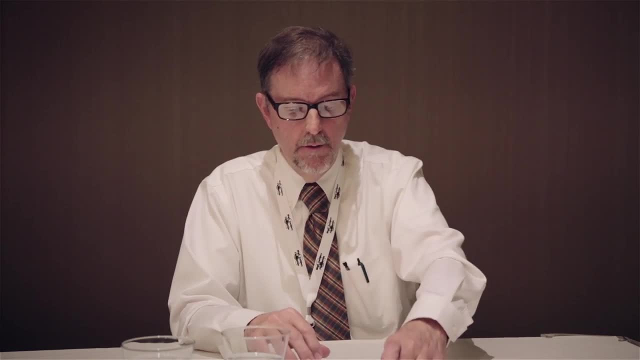 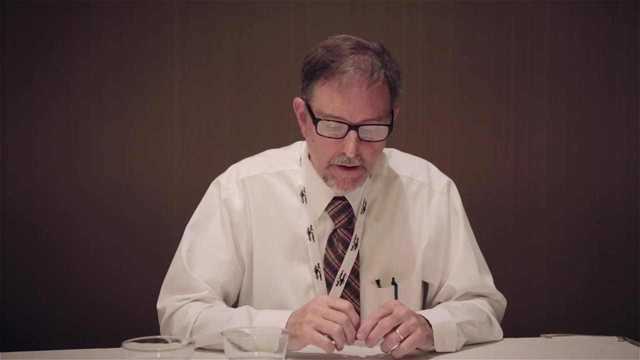 to develop and develop and develop, To discern assumptions, to see entailments, to notice implications, to be sensitive to the nuances of language. And those skills obviously grow, the necessary cognitive equipment required of critically aware, independent adults, people capable of thinking for themselves. 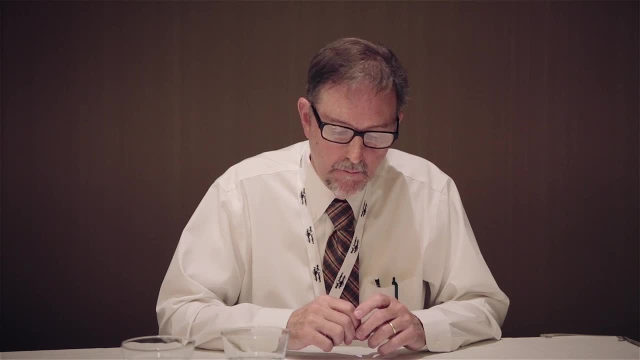 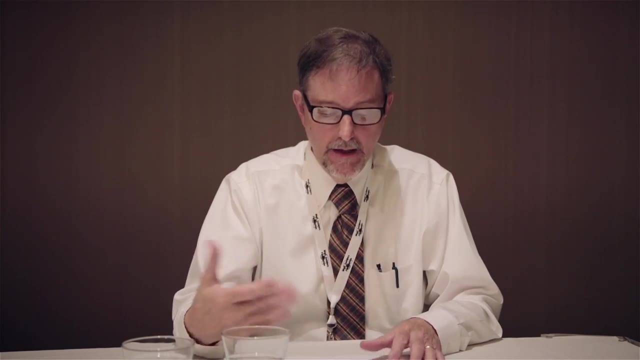 So that's a kind of instrumentalist conception of doing philosophy with children or raising philosophical offspring. Doing philosophy with kids is an undertaking that parents have good reason to engage in because it has important payoffs, Since decent parents and teachers are not able to do it. 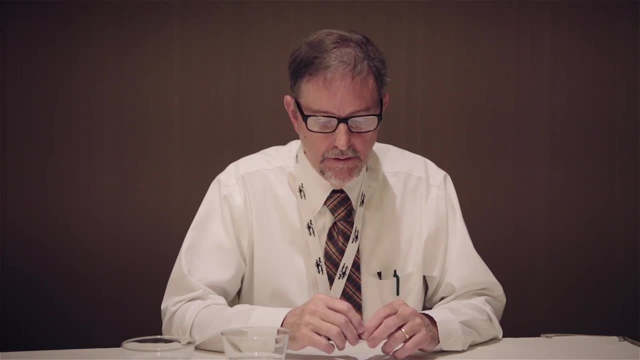 they're not able to do it. So that's a kind of instrumentalist conception of doing philosophy with children or raising philosophical offspring. And if teachers want their children to have those skills and display that array of fundamental reasoning abilities, then it makes good sense to raise philosophical children. 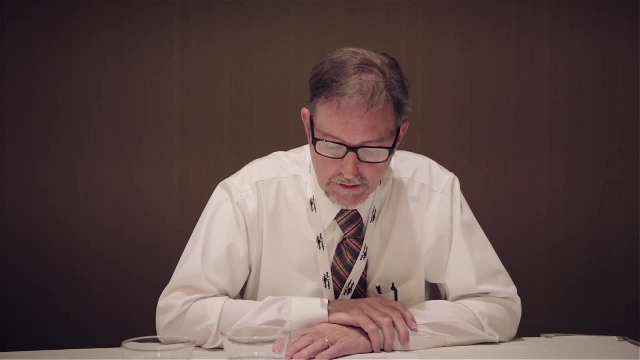 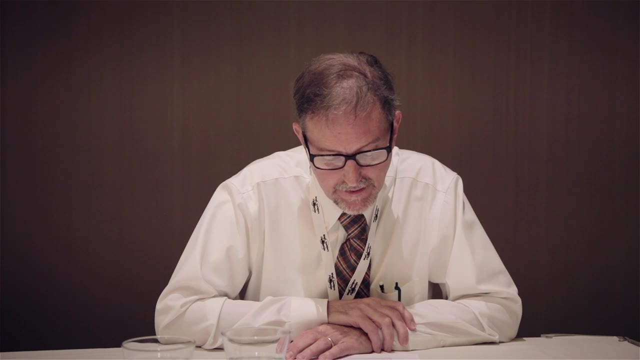 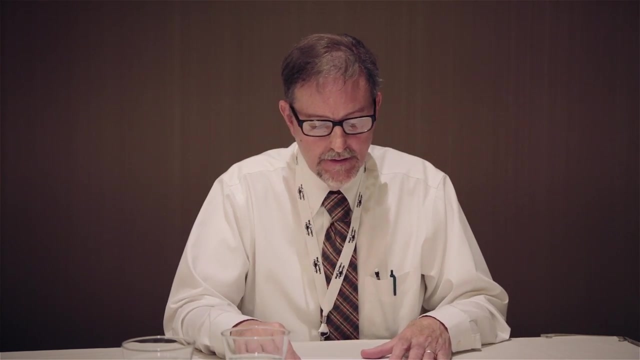 Now, I think none of us would obviously downplay the importance of developing a child's analytic, problem-solving and critical reasoning skills. The acquisition of them alone, I think, cannot fully capture or explain what it means to raise a philosophical child. And that is because, as I think Jan and Norman makes clear in her book, 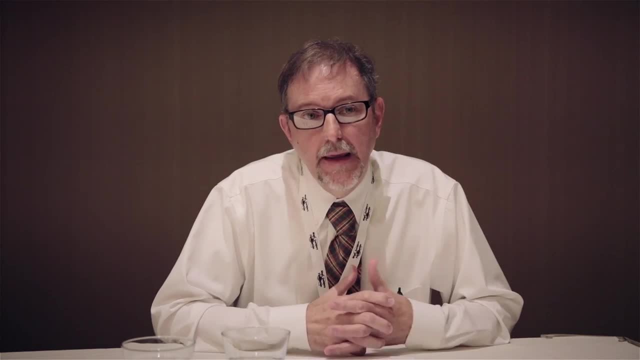 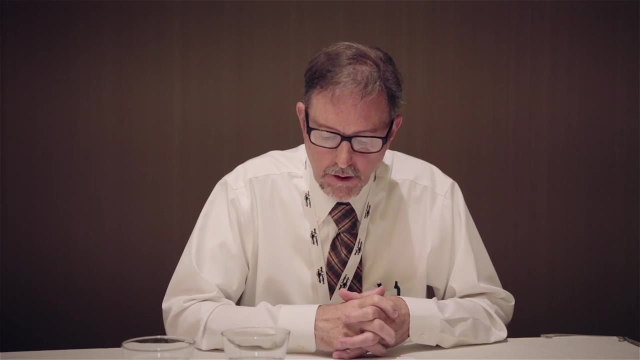 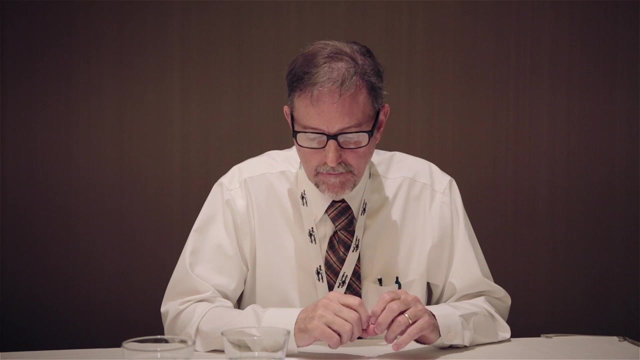 in her book doing philosophy with children. making their upbringing philosophical consists in more than simply cultivating within invaluable reasoning skills. It also, and crucially, means instilling a certain set of desires and attitudes in our children: A desire to challenge received assumptions. 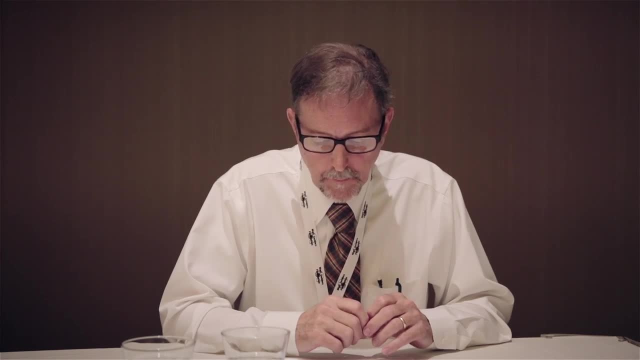 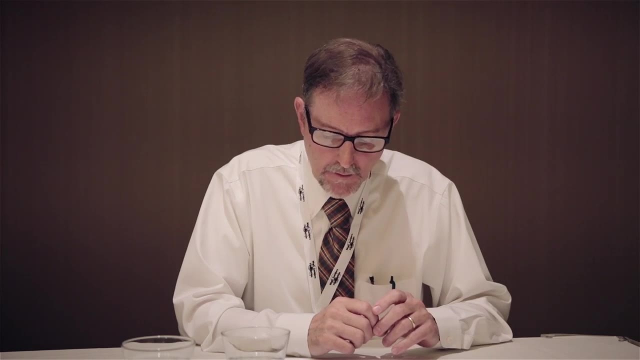 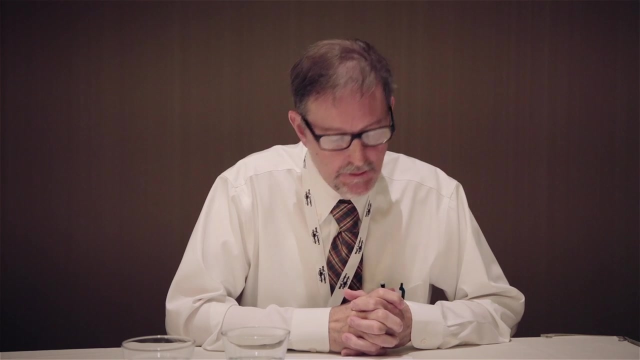 an eagerness to seek truth through careful reasoning, a preoccupation to pursue questions lacking final answers, and the disposition to regard life and the universe as strange and mysterious. That raising philosophical children involves shaping a child's preferences and attitudes in these ways is not, I think, surprising. 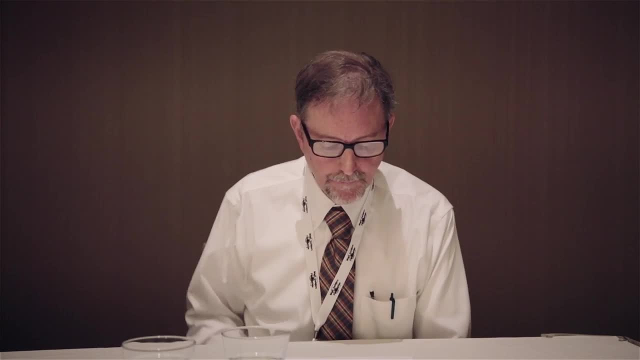 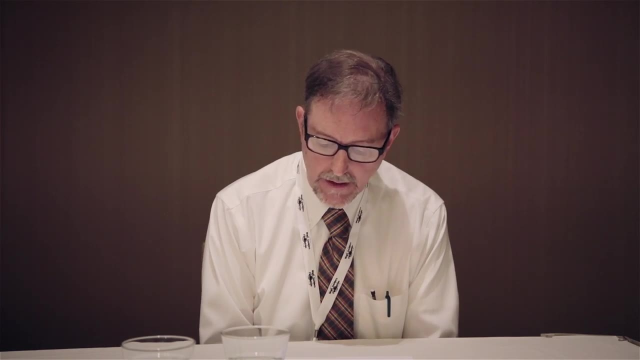 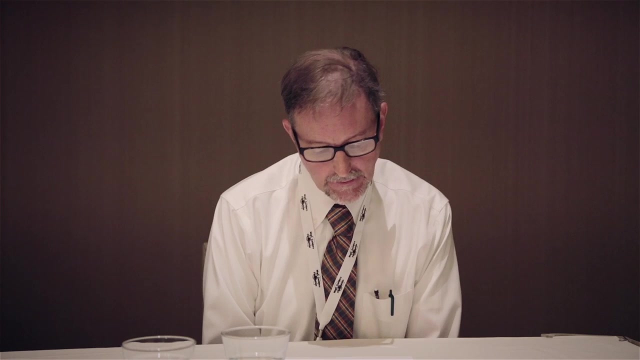 So you can consider again the musical case. Raising a genuinely musical child means bringing up someone who not only possesses technical skill but also has an abiding desire to make music and an enduring disposition to derive enjoyment from doing so. In like manner, a philosophical child is one who has come. 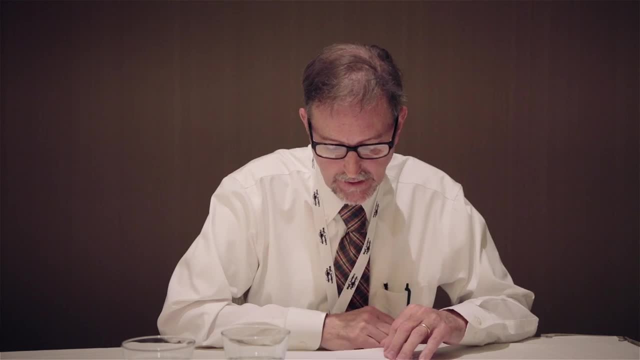 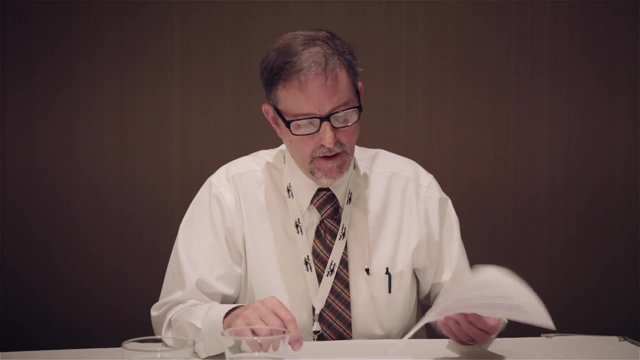 to take delight in philosophizing as a distinctive way of dealing with his or her innocent puzzlement and steadily growing demand for reasons- And of course we've had lots of examples of that from my other co-analysts- The claim that doing philosophy with children 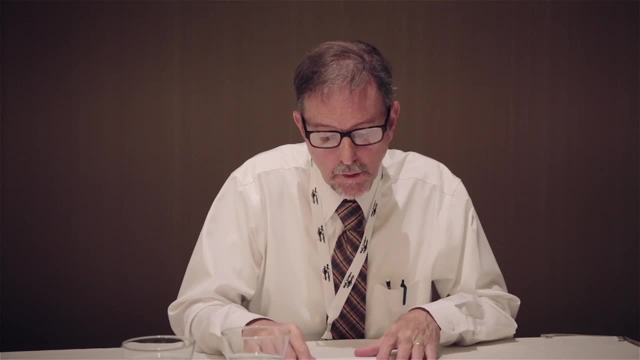 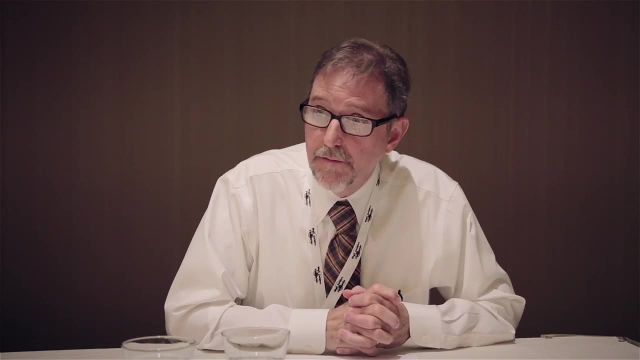 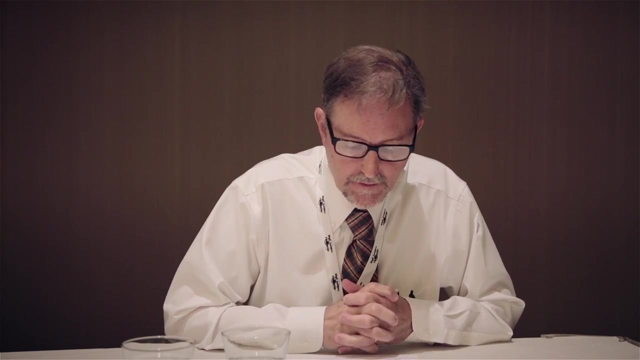 goes beyond supplying the tools with which kids can better reason about their ends is perhaps best appreciated when juxtaposed with a very different way of dealing with a child's spontaneous and forthright questions about life. Again, we've heard lots of examples of this. 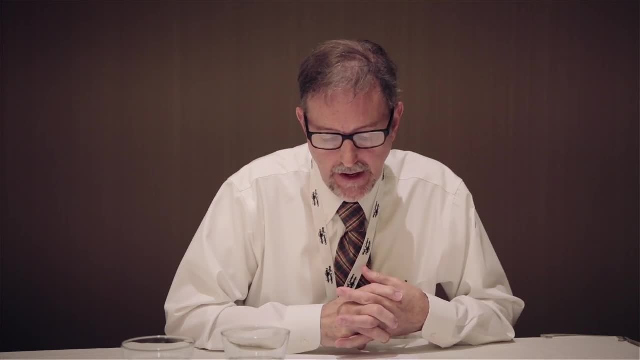 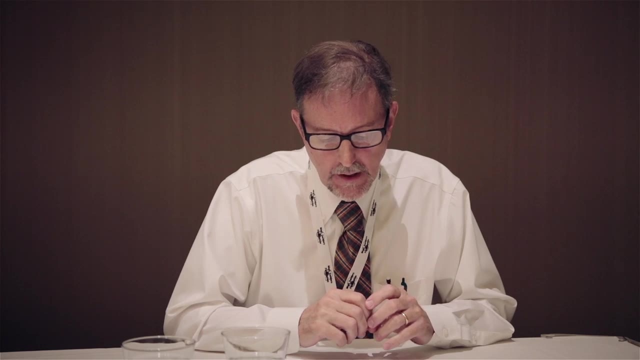 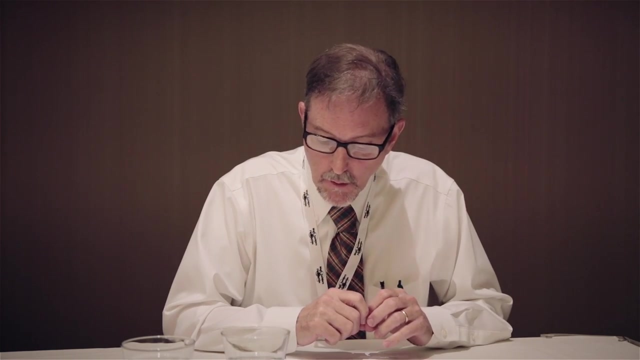 So consider a parent, when he confronts a child asking frank questions about the beginning of the universe or the nature of death or the purpose of life, responds with answers reflecting the parent's own deepest commitments and ends. Those are very good questions, such a parent might say. 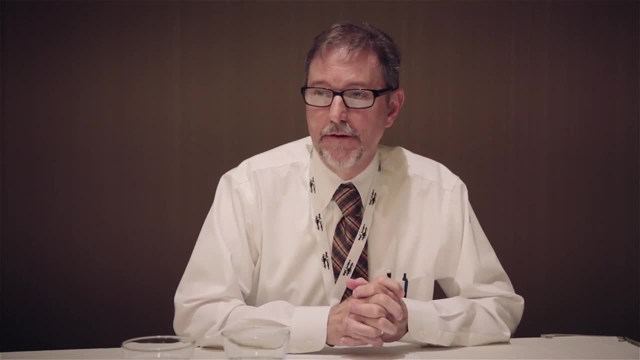 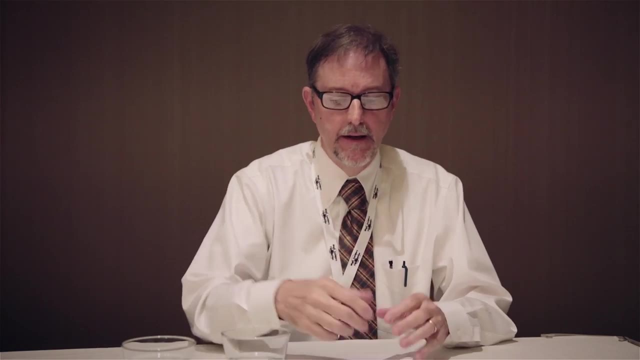 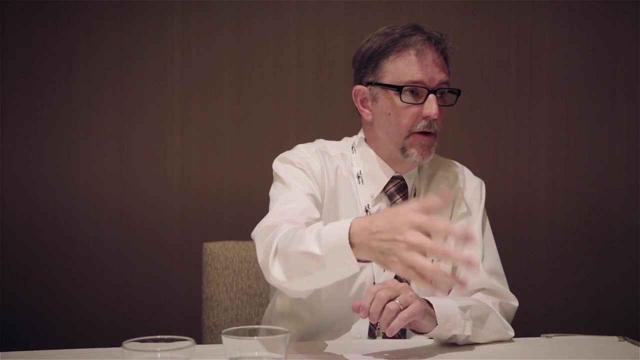 That's why it's important for you to know the answers. Here they are, And the parent then proceeds to instruct the child in accordance with, say, his deeply held religious doctrines, And then the details of those are shared with the child as the child grows up. 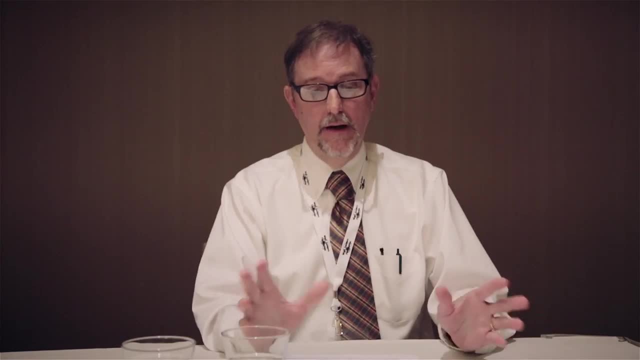 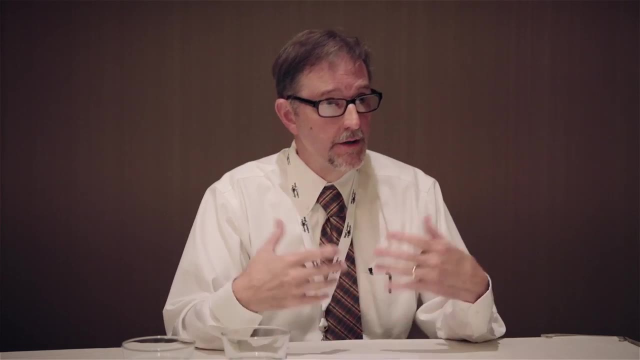 It's important to see that. well, I mean, it's an interesting question, I think- and it's actually one that we might wanna talk about later- to the degree to which this parent is failing to respect the agency of his child or is not engaging the child. 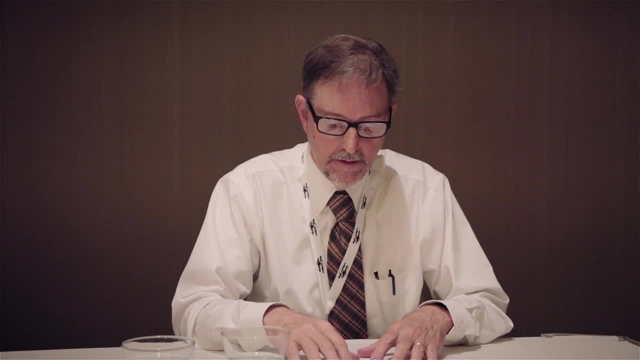 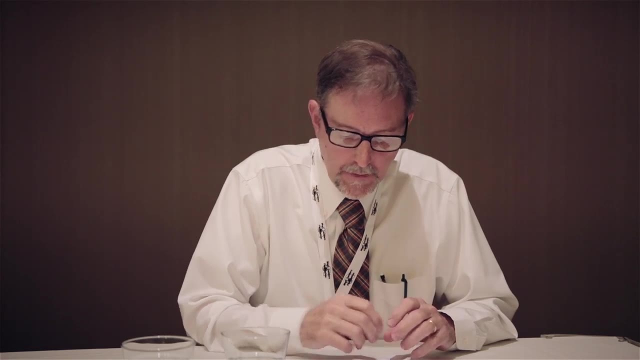 as an equal, as a partner, as a friend. I mean, that's an interesting problem. He appears to take the question seriously and to take his child seriously, But his response to those questions consists in introducing the child to and nurturing her within. 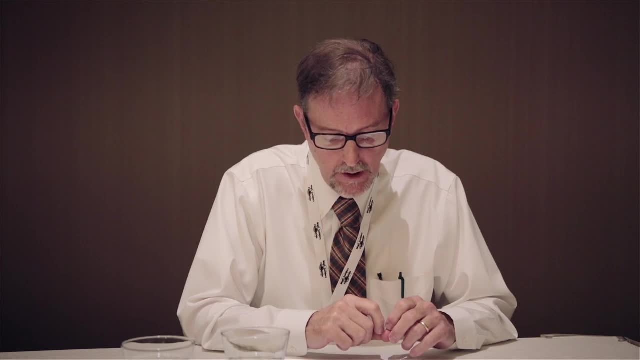 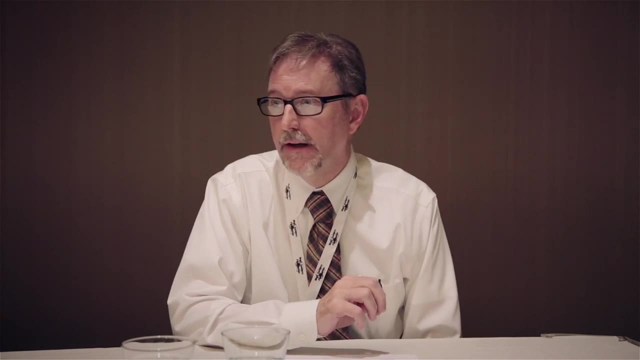 a network of traditional beliefs or a set of comprehensive doctrines aimed at putting the child's question to rest. This parent does not have the ability to do that. He does not model how to interrogate accepted assumptions. He wants instead to transmit them. 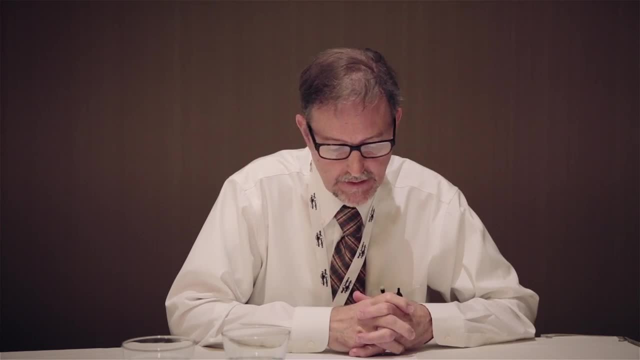 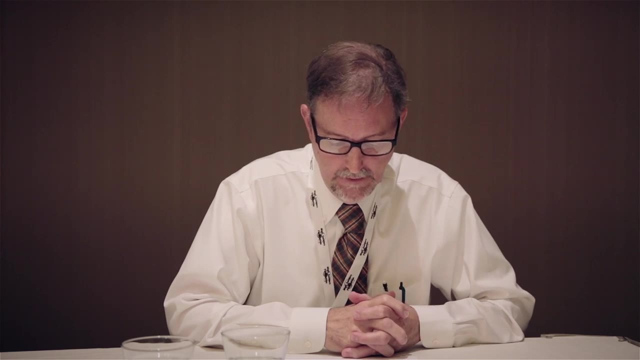 He does not delight in pondering the unanswerable, nor is he aiming to convey a sense of the strangeness and mysteriousness of the universe. He seeks instead to offer the reassuring comfort of the answers. The universe is not baffling or obscure. 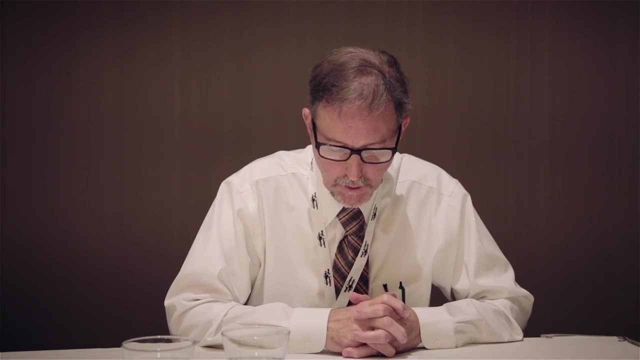 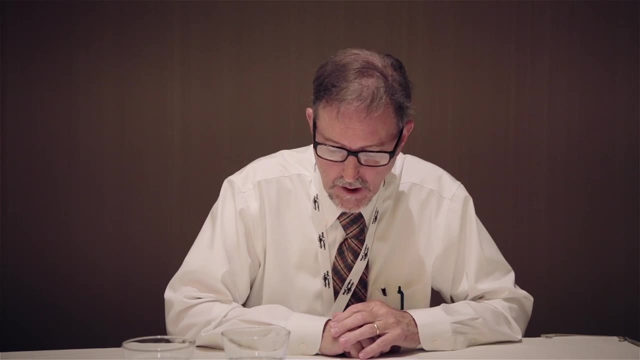 It is rather our home, a home with a meaning that is comprehensible and a purpose that is known. I don't want my child being encouraged to find her own answers to what death is or how to make decisions about what's right and wrong. 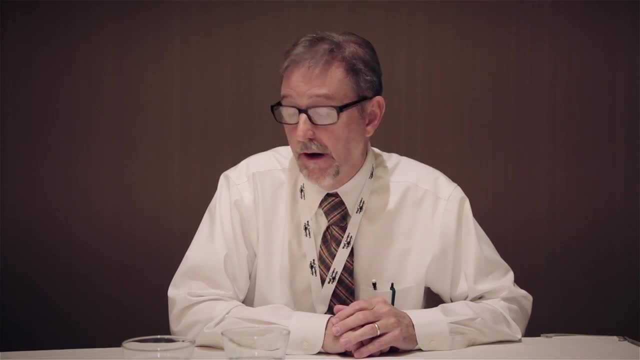 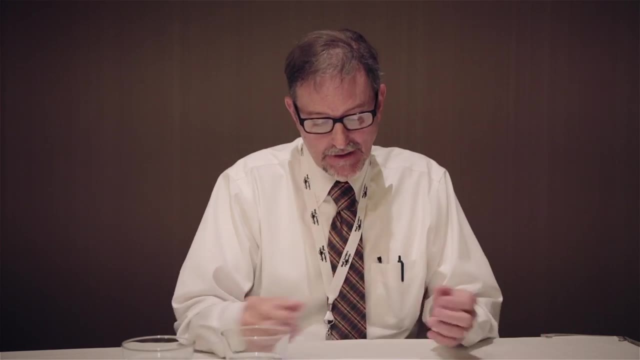 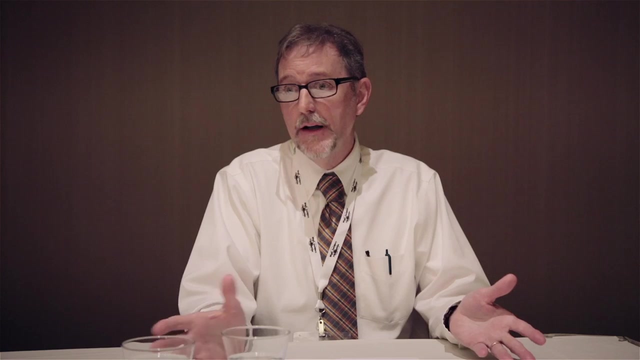 This parent might say: I want her to get that, as I did, from our tradition. So what do we think about that? I mean, it doesn't strike me that that's an obviously irrational parental response to a child's fundamental inquisitiveness, albeit however much at odds it is with 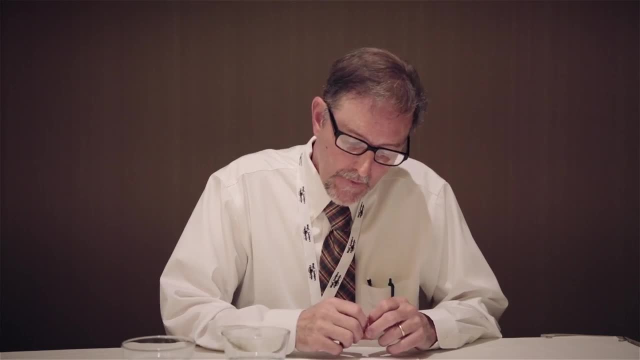 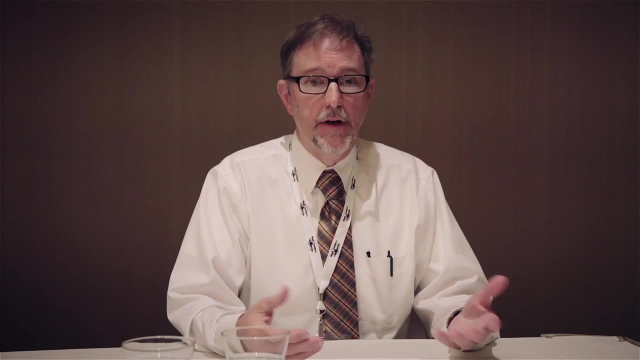 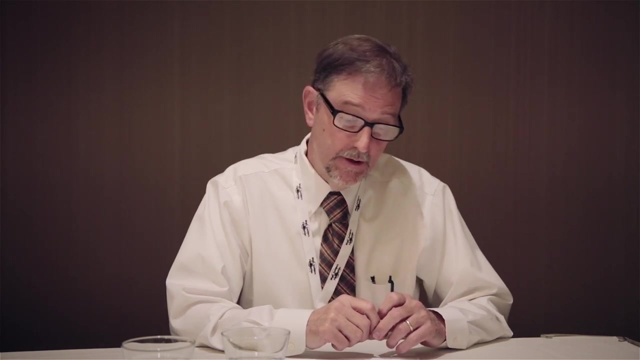 doing philosophy, or at least appears to be So. in that way, though, children raise questions that certainly can be taken up as philosophical, and we've had again lots of examples of this today. it's not obvious to me that Matthew Lippmann was right when he said years ago: 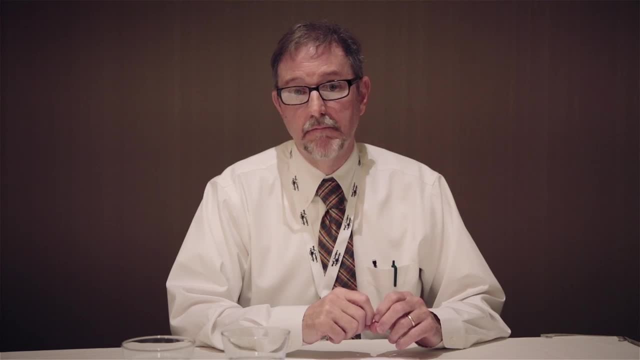 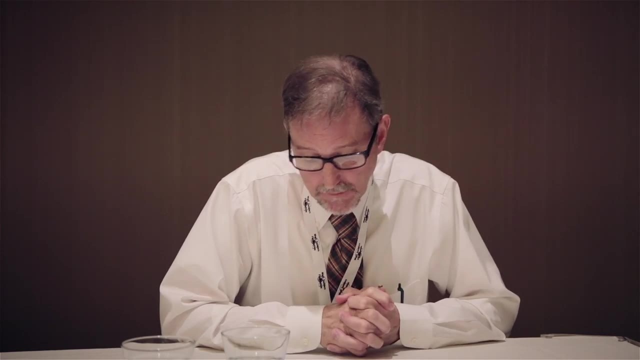 that these questions demand answers that are philosophical. So we might say then- and I think this is probably the right answer to my initial question, raising philosophical children just means doing philosophy with them, which, you know, Janet has lots of wonderful examples of in her book. 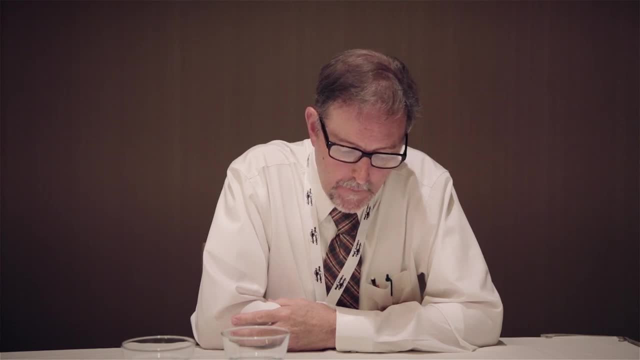 and Gareth Matthews, of course, years ago, did the same thing. But when we so engage our children, we're not merely helping them learn how to think, giving them critical tools with which to evaluate their lives, commitments and ends. We are also actively shaping those ends, and in a way that 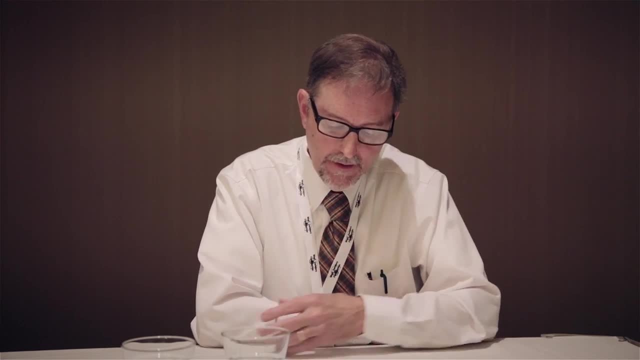 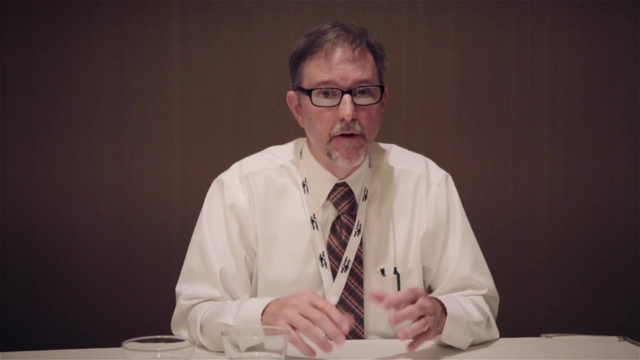 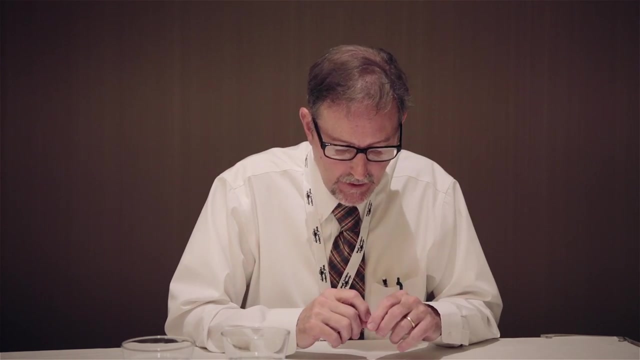 not all parents would accept. That, I think, further suggests perhaps a way in which we might think of children being naturally philosophical. That was an argument that Matthew Lippmann made in a number of books, Plainly curious And unencumbered by the crusty accretion of adult preoccupations. 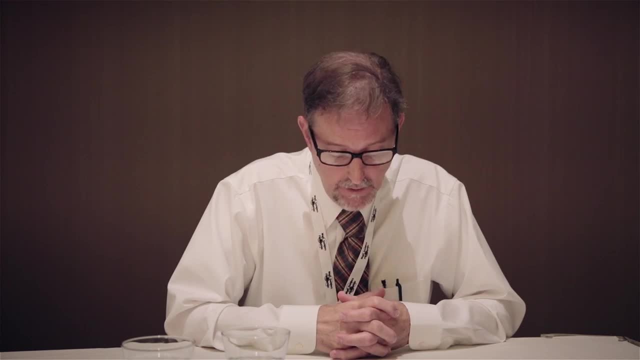 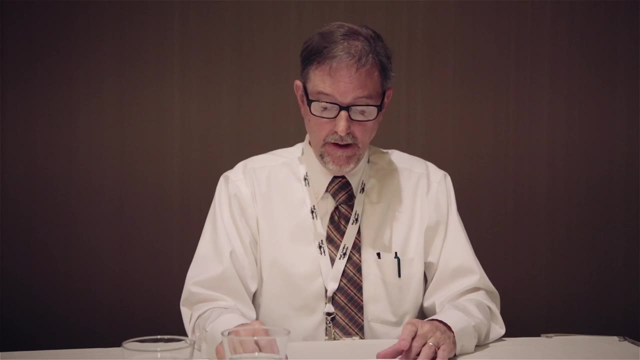 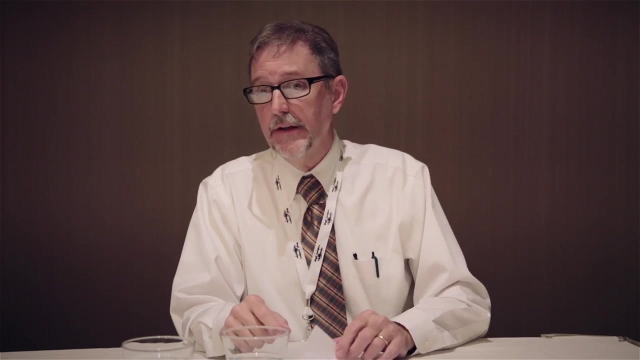 and time-worn habits of thinking. children do obviously display a playfulness with language and a desire to explore the boundaries of concepts. These predilections, which are in some sense precursors to philosophical reflection, merge and express themselves in the propensity to generate questions that often startle or embarrass parents. 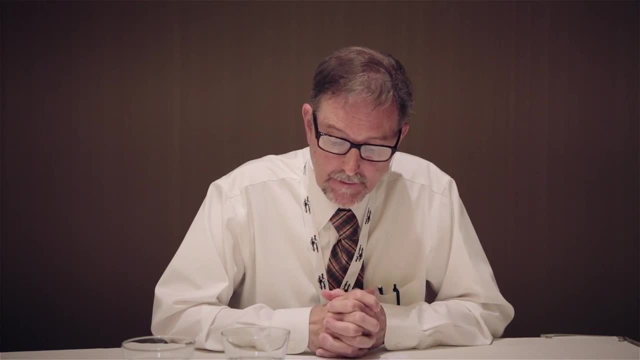 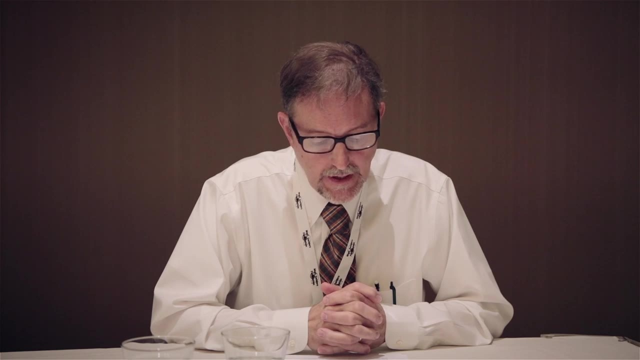 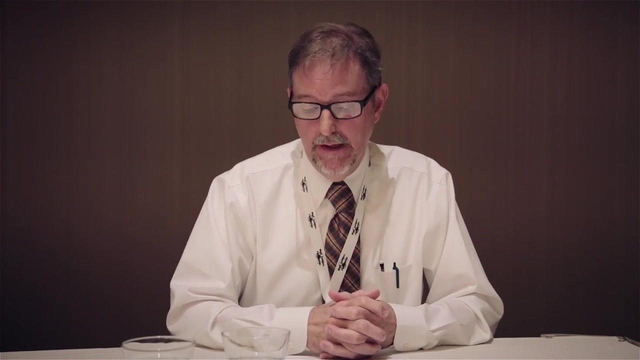 And we've had lots of good examples there too. This makes children, according to Gareth Matthews, ideal beginning philosophers, for whom philosophy is a natural activity, quite as natural as making music and playing games. Here Matthews could point out that musical understanding and an appreciation for musical 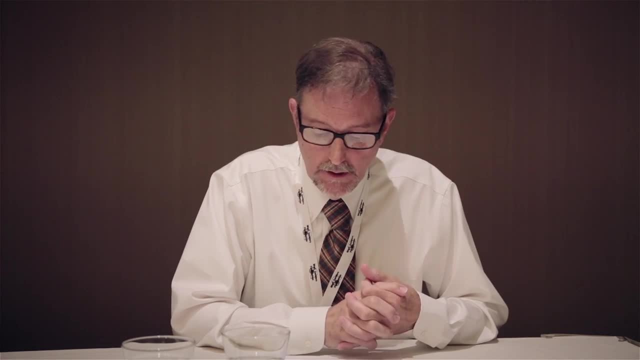 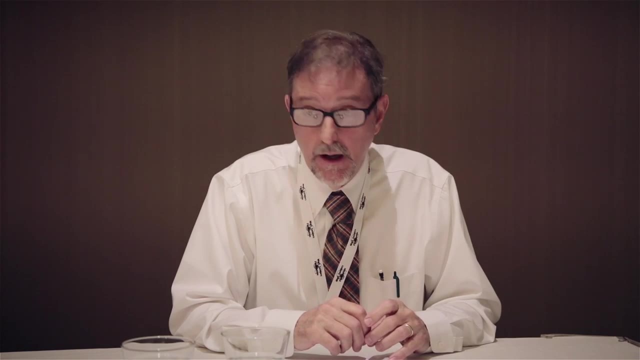 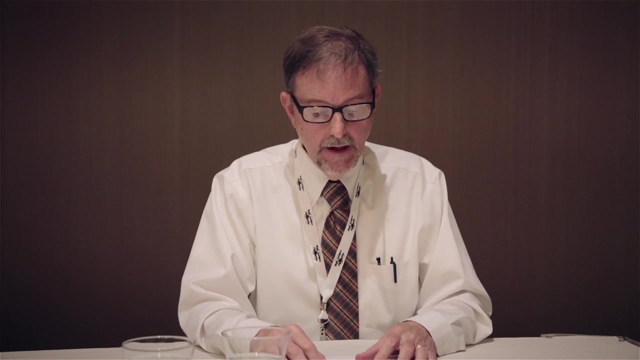 expression seem to come readily and unbidden to many young children, And music pedagogues argue that developing musical aptitude is most easily accomplished in childhood, in early childhood, as it appears more difficult to develop skillful musicality later in life. In like fashion, young children often are ready for encounters with philosophy, with 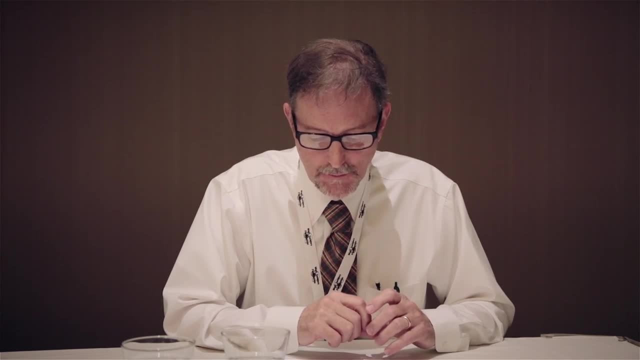 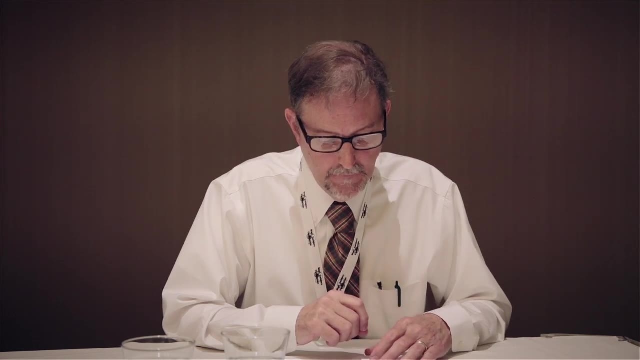 a receptivity that too often atrophies and withers in adults whose minds are no longer open to the imaginative and persistent questioning so central to the doing of philosophy. But Matthews' claim- and here's where I want to sort of raise a question about that, 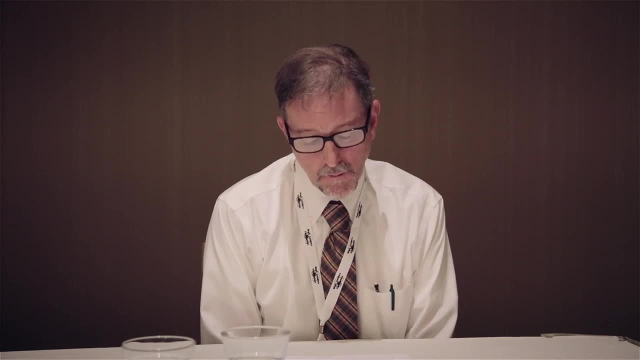 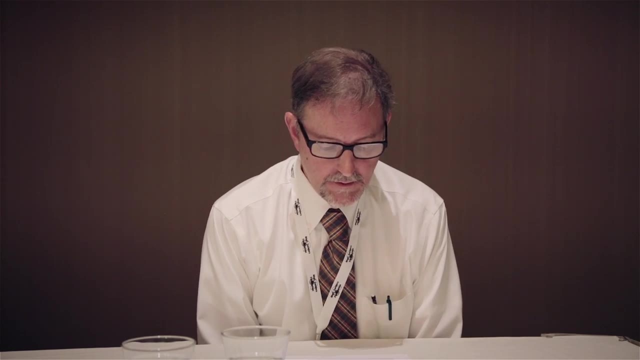 Matthews claimed that children are natural-born philosophers, seems to overstate the facts, at least in one way. Children aren't doing philosophy simply by virtue of plying their parents with questions, For the child who routinely asks why? can, as we've just seen, be answered in a manner 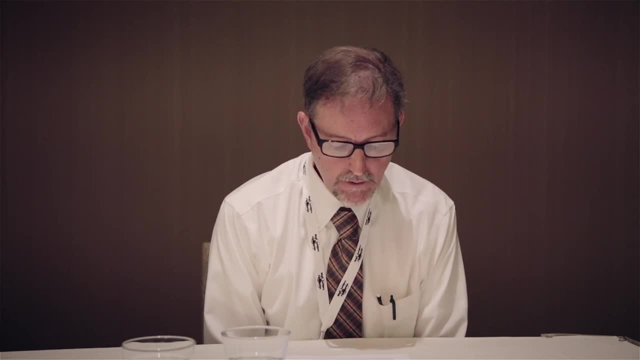 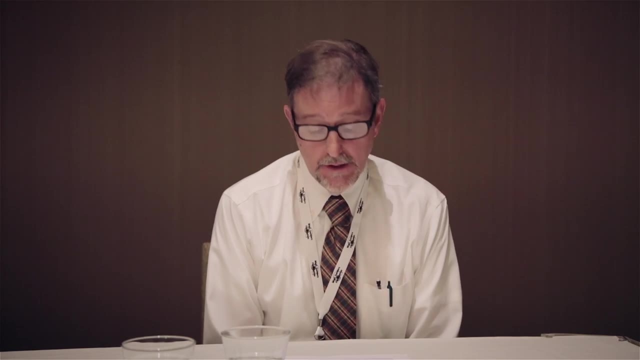 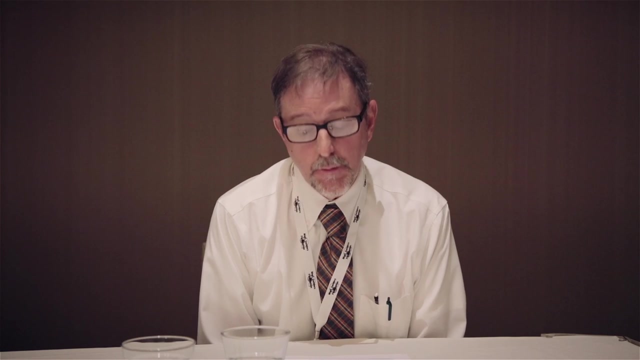 that neither aimed at nor succeeds in cultivating within her a way of addressing her questions that is distinctively philosophical. Young children, to be sure, ask questions at real depth and importance, questions inviting not only dialogue but probing analysis. But the conceptual playfulness and inquisitiveness evident in many a young child's questions. 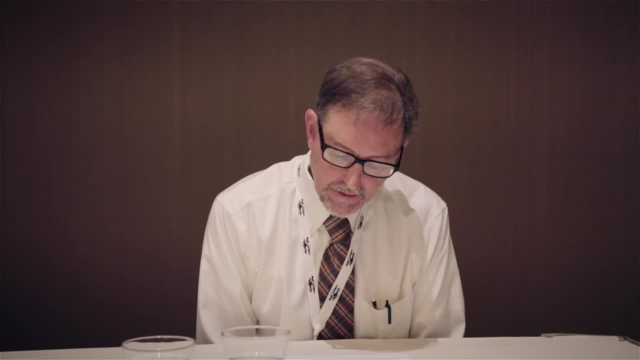 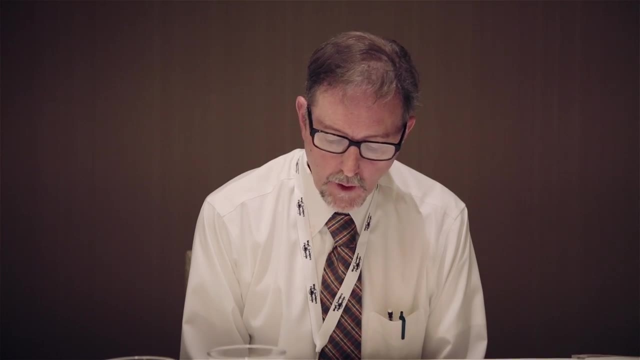 as we've just seen, can be answered in a manner that neither aims at nor succeeds in cultivating within her a way of addressing her questions that is distinctively philosophical, I think, only when she or his questions are taken up and responded to in a way that forms 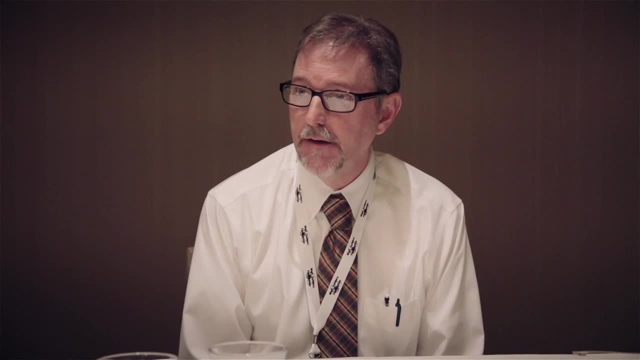 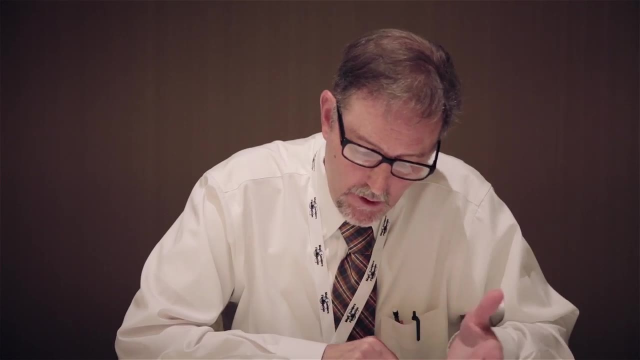 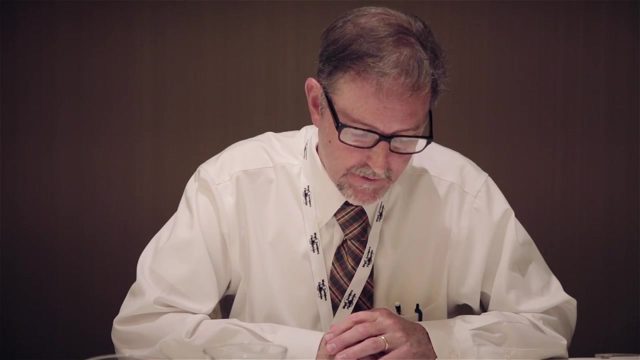 within her a particular set of desires and attitudes—a kind of philosophical orientation toward life—it becomes philosophical. Even young children can do philosophy, then, so long as their propensity to ask questions is directed by this kind of slowly forming set of preferences and attitudes and ends. Now some, I think, will object that this is not what they are about to do, but rather that it is. But young children have a great majority of friends who are either getting married or having family or living with their parents. 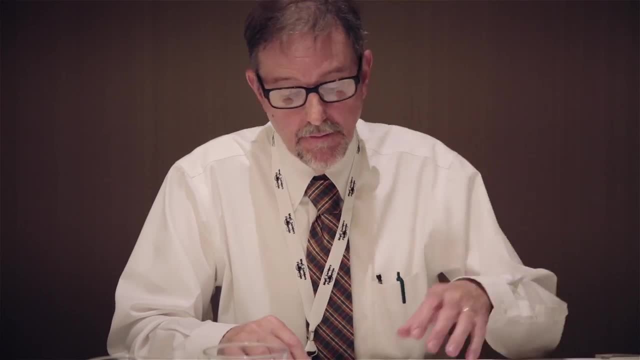 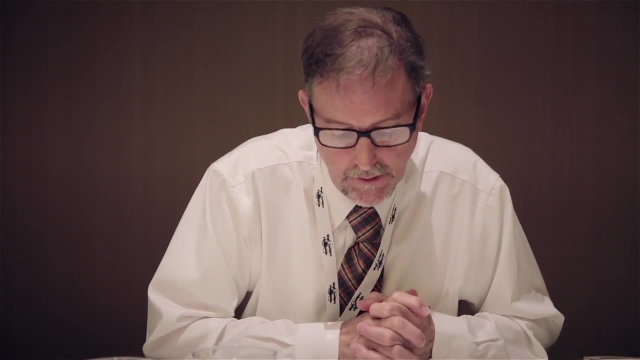 That's why they're involved with this kind of thing. This is insufficient to make a child's upbringing philosophical, assuming they lack as yet the conceptual resources and familiarity with a body of writing and thought that we normally associate with philosophical understanding. how a critic might ask, can children do philosophy? 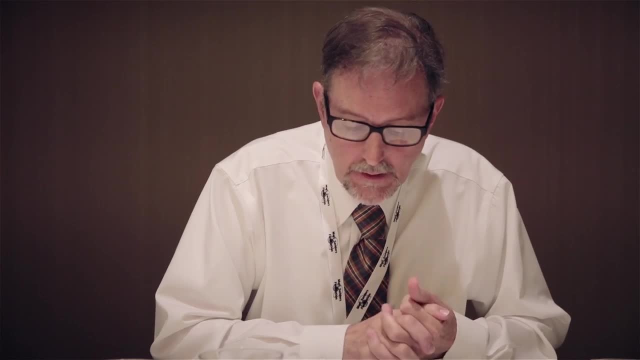 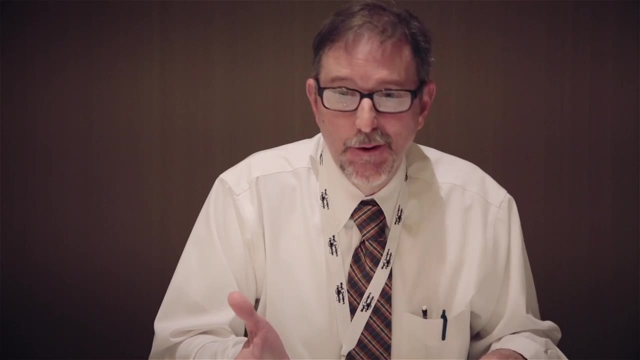 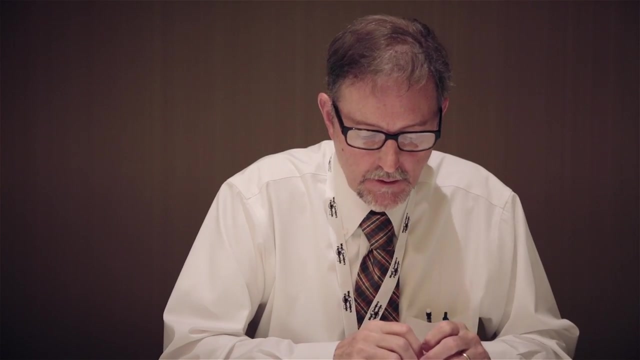 without knowing anything about it. After all, any child can manipulate a musical instrument so as to produce sounds, but doing so doesn't seem to be enough to conclude that the child is musical, Therefore being musical, and again, this is the argument that the critic, I think, is. 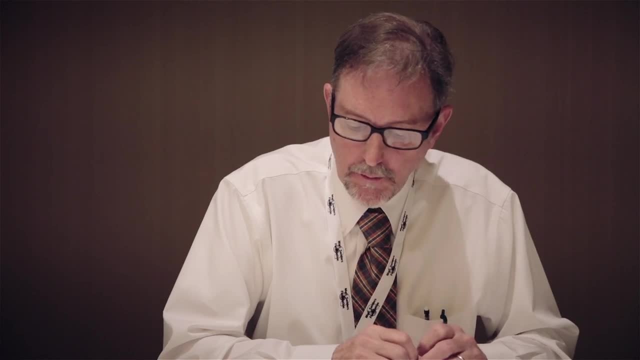 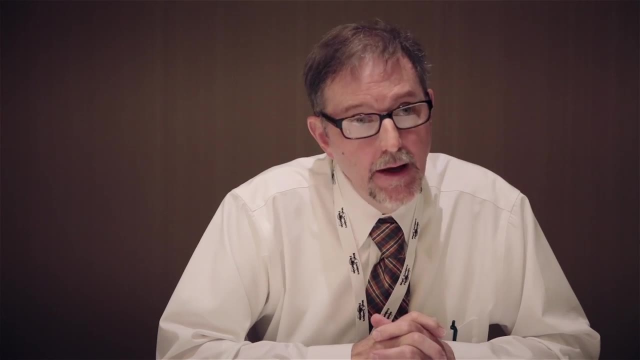 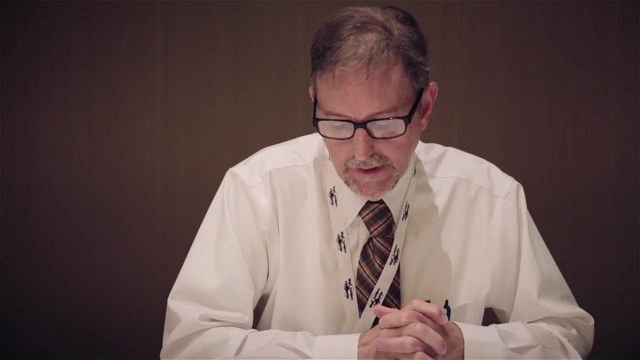 going to pursue requires much else besides an inclination to bang on a drum or pluck out some notes on a keyboard. A musical child is one who is being supplied with a language and a set of concepts within which to recognize and appreciate pitch collections and tonality, rhythmic and metrical forms. 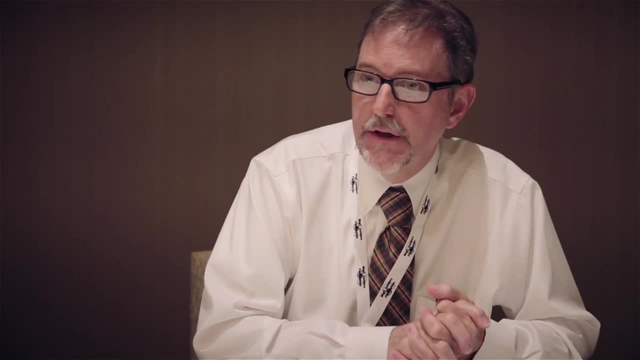 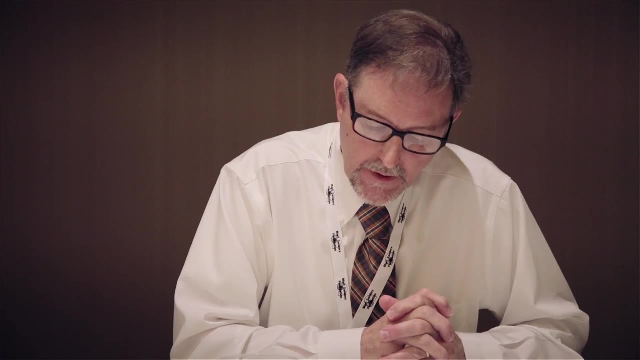 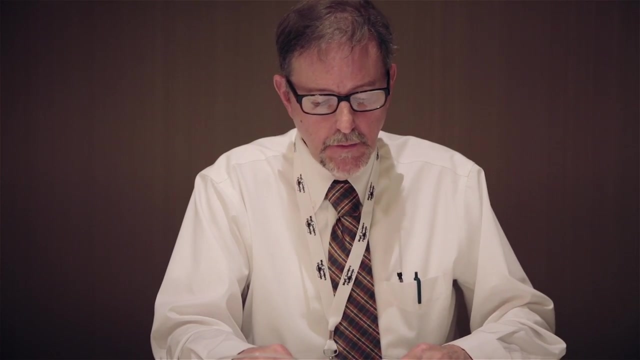 melodic and harmonic patterns, compositional types, instrumental timbre and so on. Musical children have been assisted to identify the right instrument with which to express themselves and how best to practice it Successfully. raising a musical child, therefore, invariably involves musical instruction and 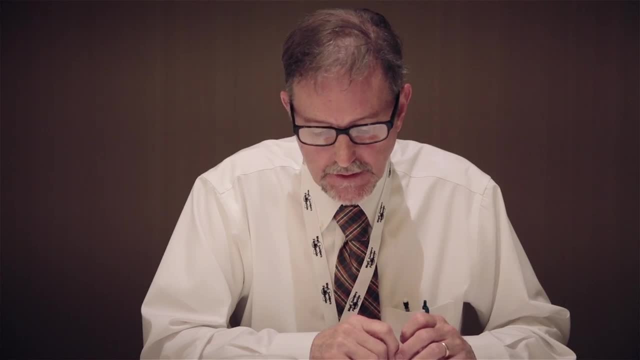 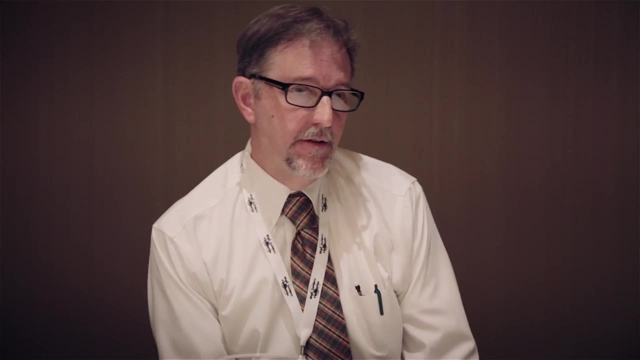 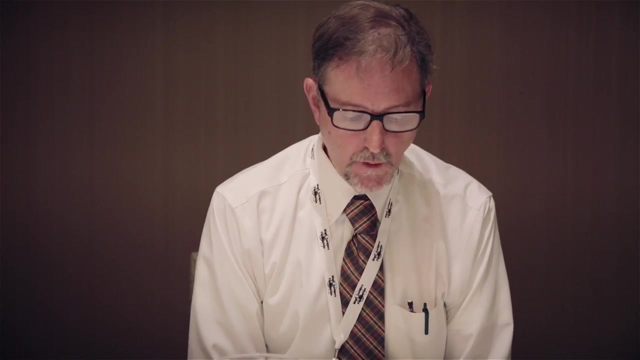 training, Long hours of practice to master an instrument must be coupled with instruction in theory and the acquisition of a specialized vocabulary. Why then- and this is kind of the challenge that the critic, I think, is going to pose to us- is you know why then doesn't raising a philosophical child require complement forms? 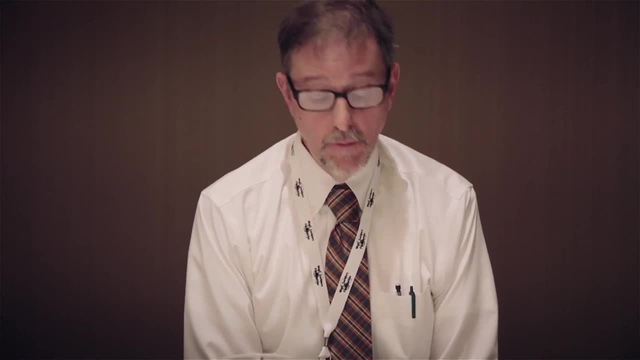 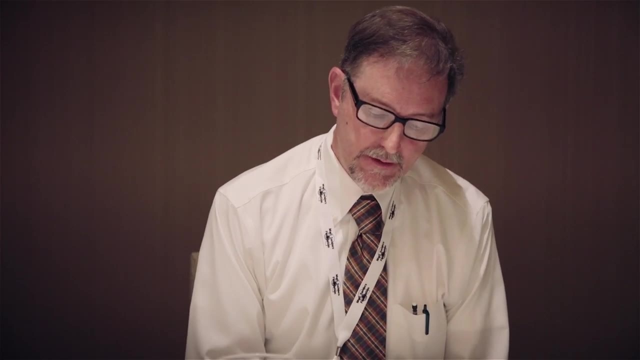 of instruction and training in philosophy before the child can really be said to be doing it. Well, the reply to that objection, I take it, is going to be something like this: that just as children can play a simple song, right, as opposed to just, you know, producing sounds. 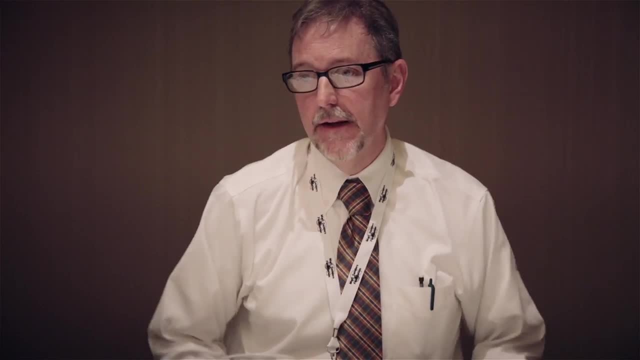 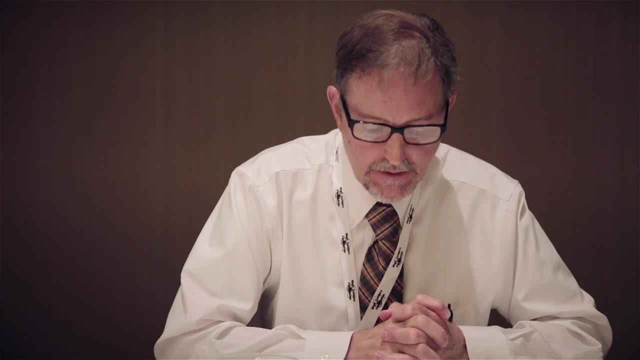 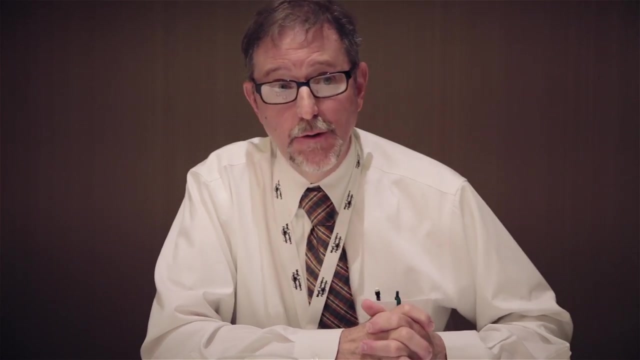 in time, even if they don't comprehend. you know music theory, so children can do philosophy once they enter into the kinds of conversations that we've been talking about today and you know, recounted in Jana's book, though they surely will be better at doing philosophy once they've 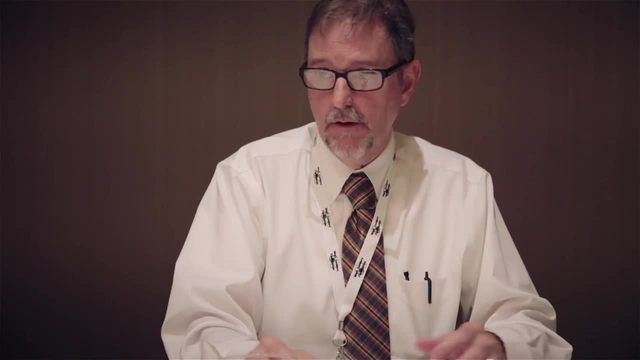 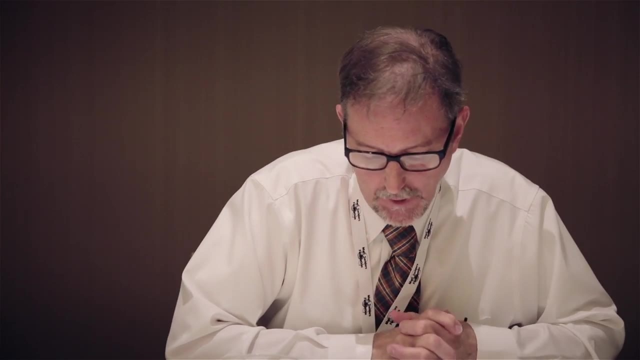 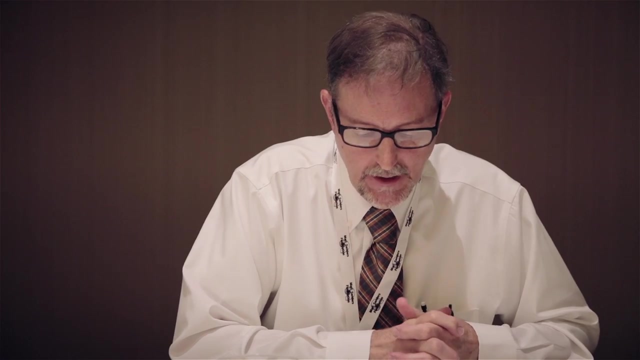 acquired, like their musical counterparts, a certain kind of technical vocabulary and body of knowledge. So the central question with which I began my remarks- did I raise philosophical children? can be reexamined in the light of these observations. On the one hand, my wife and I certainly did not set out to raise- you know, children who? 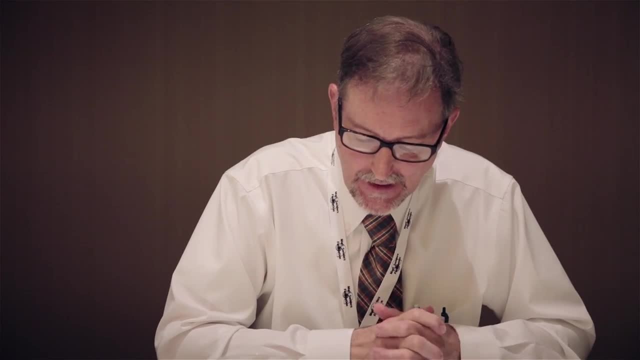 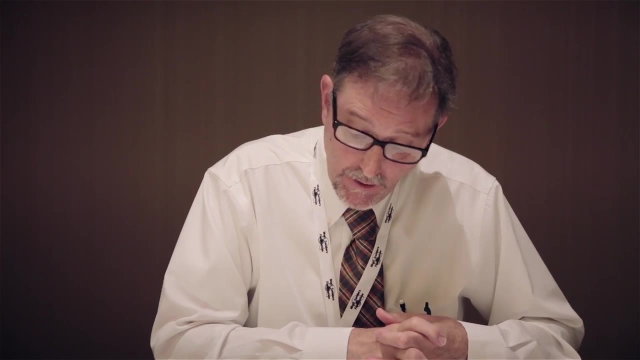 would adhere to certain rules. We didn't set out to do certain philosophical positions or something like that, Nor did I rear offspring so as to have junior versions of myself qua philosopher. On the other hand, we did, I think, largely succeed in nurturing individuals who turned 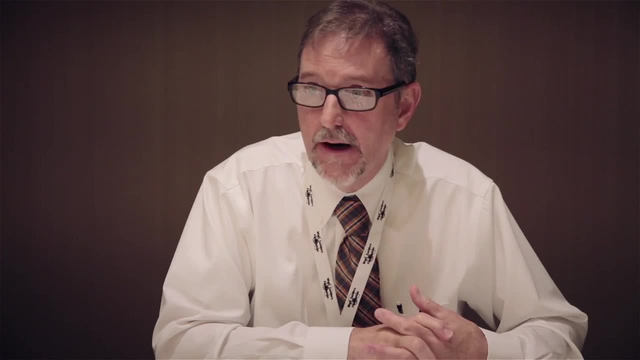 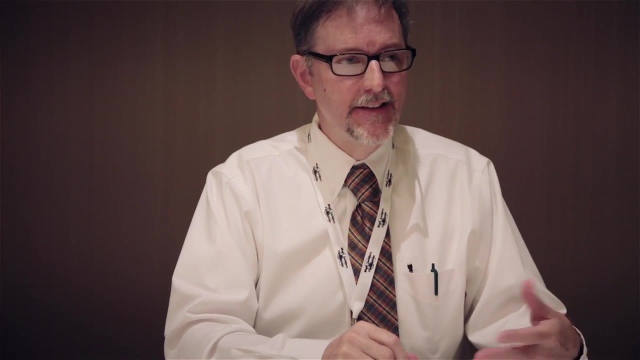 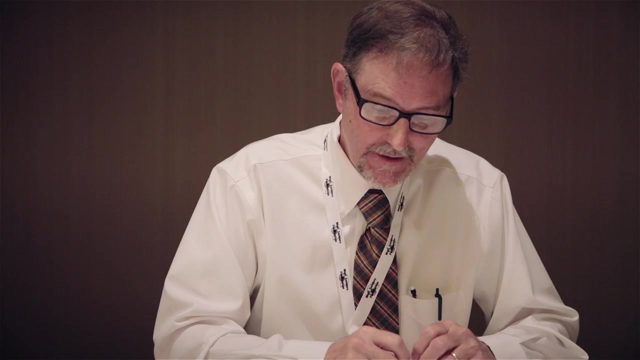 out to be inquisitive and critically reflective, proficient in careful reasoning and able to think for themselves. Nonetheless, I guess I want to say in the end, I disagree with my oldest daughter, Despite being, today, deeply pleased that my kids learned to argue so expertly, though 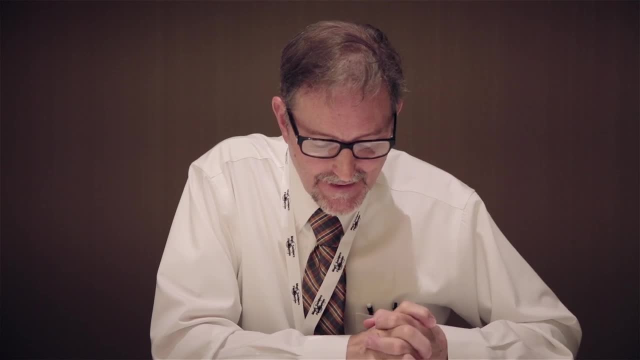 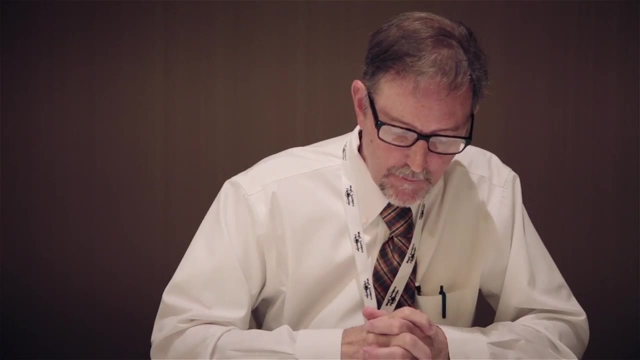 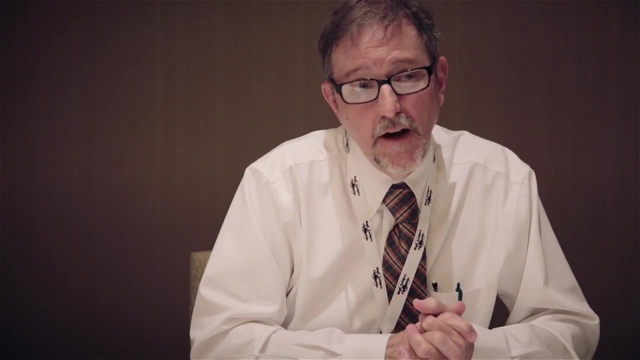 at the time I was not nearly so happy about it. I don't think that's enough to say that they were raised philosophically, For if what I've said to this point makes sense, then my initial question has to be reformulated: Did we raise our children in such a way that we formed in them a philosophical orientation? 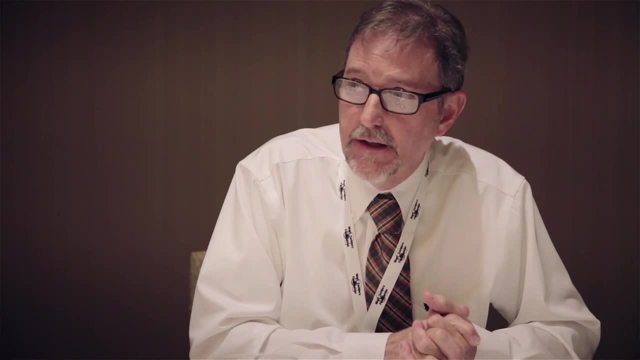 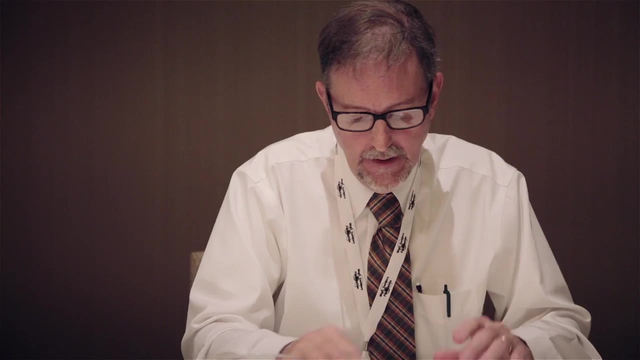 toward life? Did we bring up children who grew to possess a distinctively philosophical way of looking at and responding to their many questions about the world? Well, I think I could make a case, though I won't bother making it here- that we did. 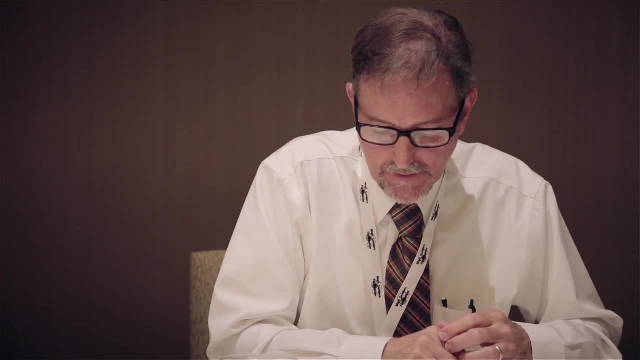 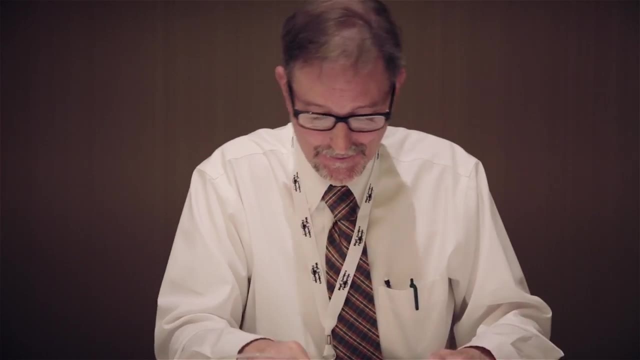 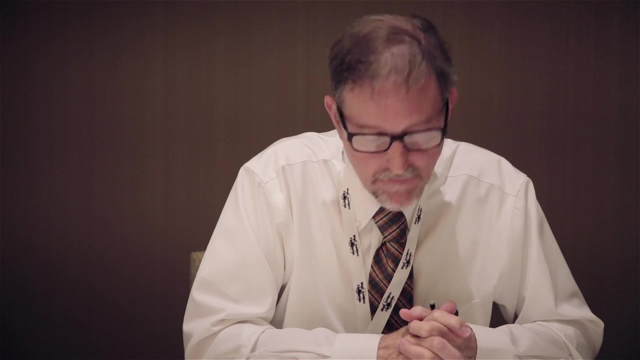 turn out, in that more exact sense, to raise a philosophical child in our son, who went on to go to law school. Maybe not any better a choice than going to grad school in philosophy, but we'll see. We did not do that, though I think as a result of having embarked upon a deliberate 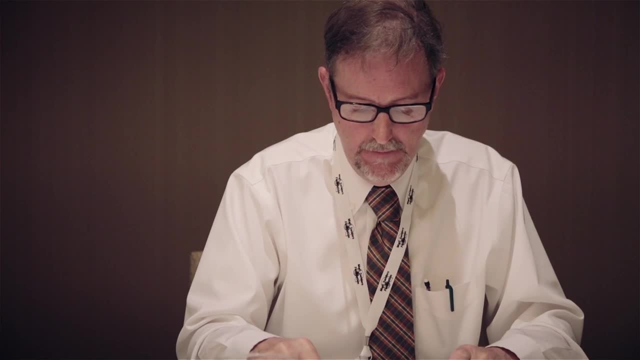 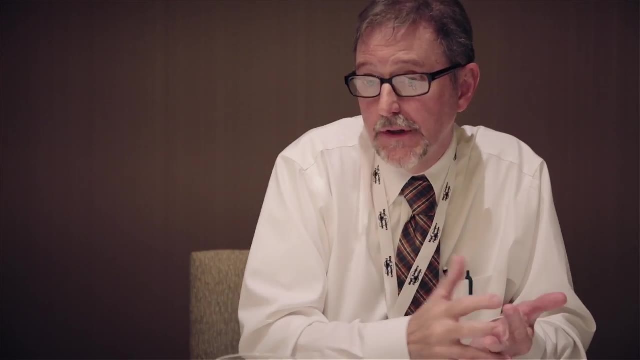 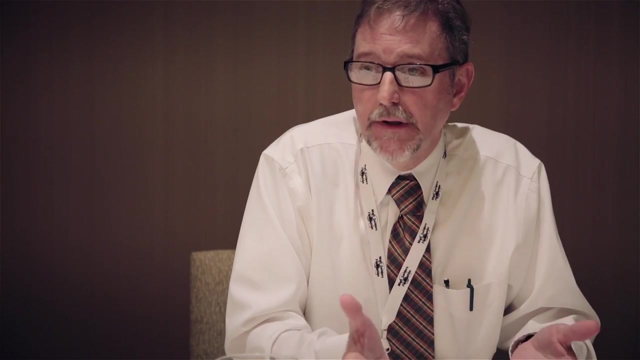 effort. I suspect, rather, that our son's philosophical orientation arose in much the same way that a set of musical dispositions and attitudes often arise in kids who grow up to be musical. Some parents believe that musical awareness and expression are intrinsically rewarding. 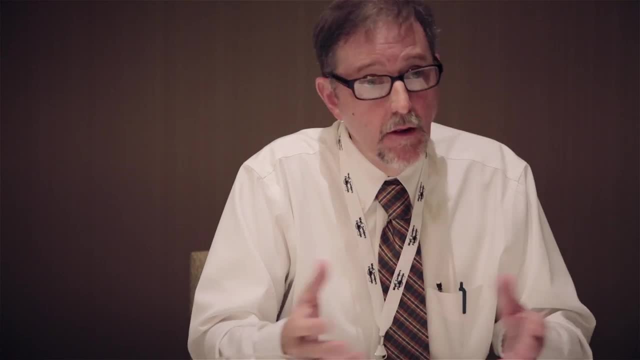 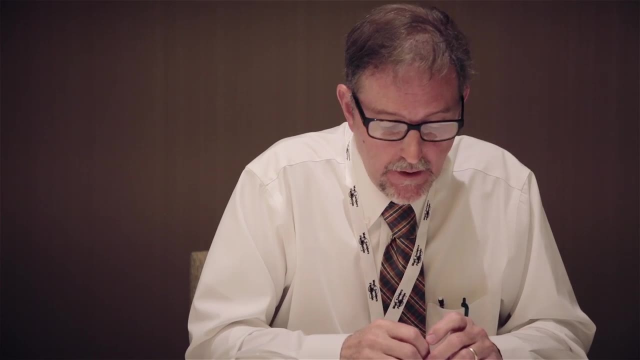 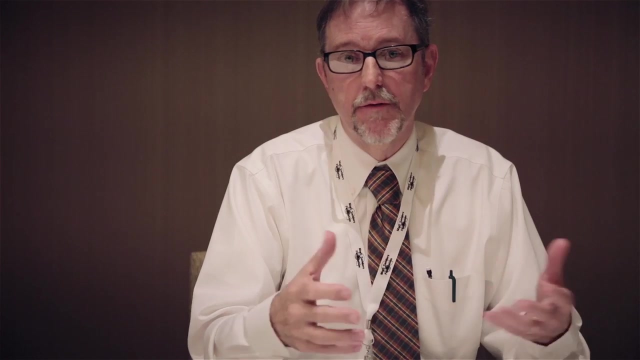 aspects of life, and that the lives of children raised musically are, in that respect at least, better lives. The world in which such parents nurture children abounds in music and, as a consequence, their offspring gravitate toward their parents' conception of the good, not as an upshot of 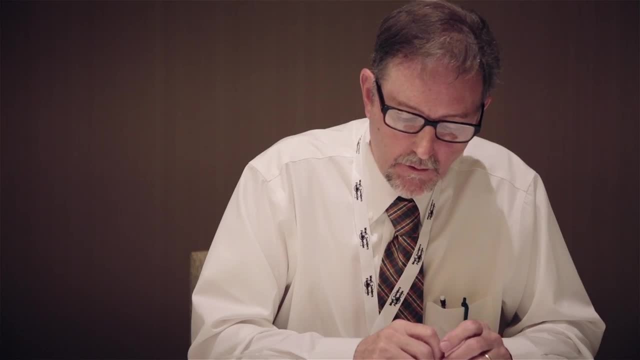 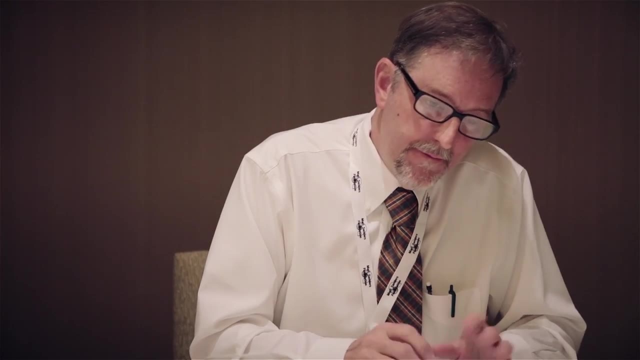 an undertaking aimed at instilling a musical orientation to life, but just as a result of a rich exposure to something that the parents value. So what I've just said there kind of suggests a distinction, maybe, between two ways in which we could think about life. 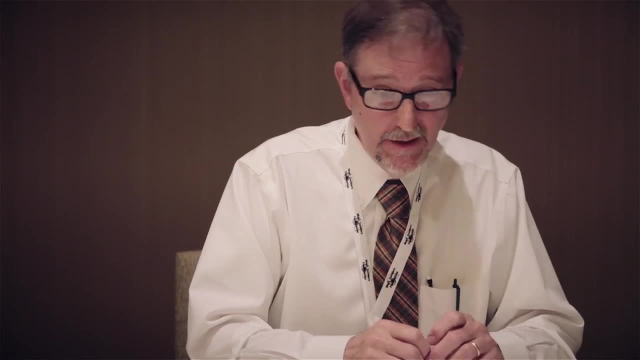 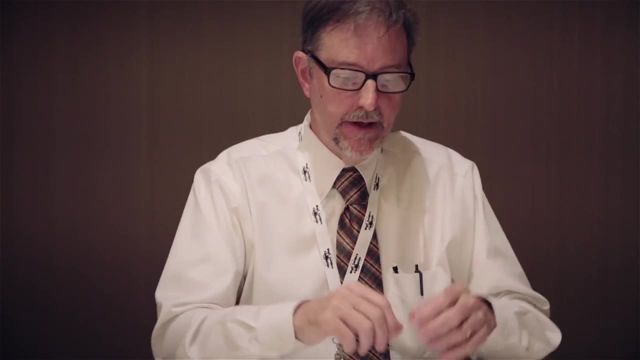 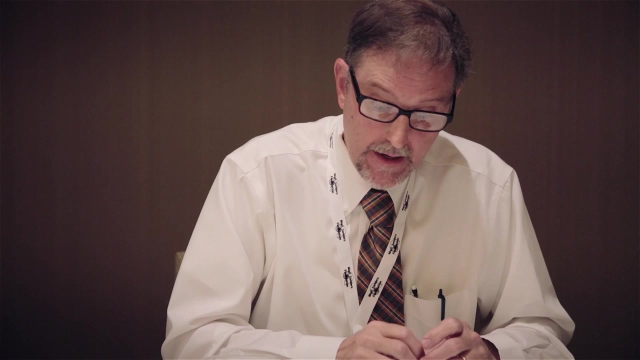 I mean, we could think about music, We could think about parents being said to raise children with a particular orientation, whether you know a sort of a distinctive set of attitudes and abilities and preferences, whether it's, you know, philosophical or musical, or athletic, mathematical, 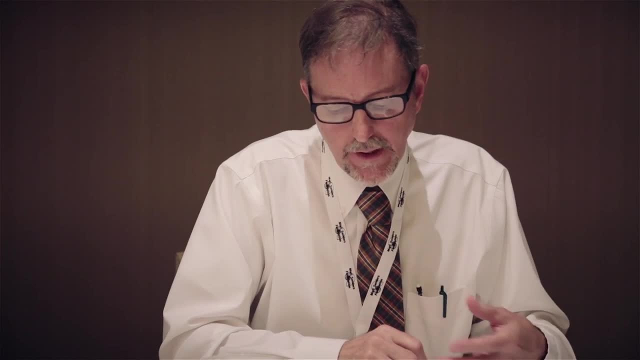 In a weaker sense. parents raise a child with a particular orientation when they expose the child to that dimension of life because they believe it to be intrinsically worthwhile, And the child comes as a result to share that set of convictions and practices. 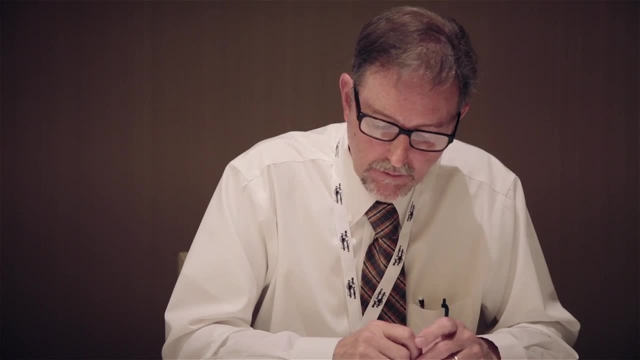 And that's what I'm trying to do here. I'm trying to make sure that I'm not just saying you know, I'm trying to make sure that I participate in that way of life. It's only in that weak sense that many parents, I think, turn out to have raised musical children. 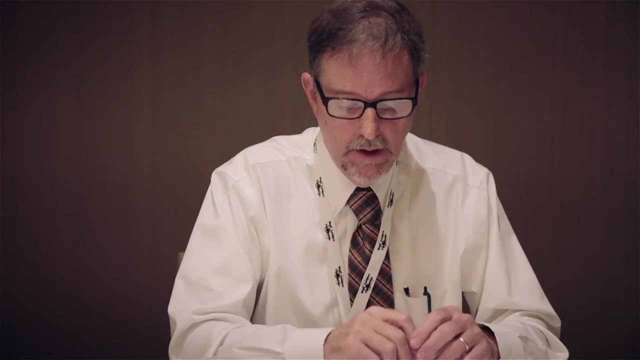 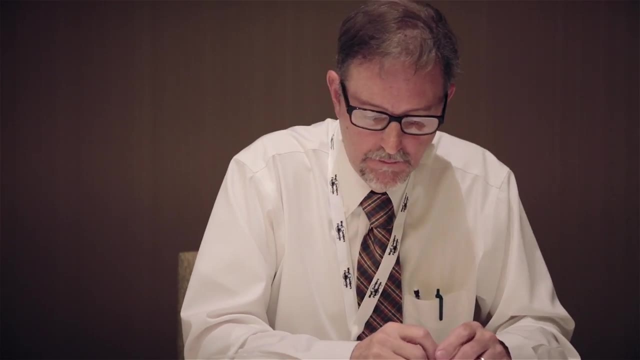 I mean, they model a love of music and they're putting out to love it as well. In a similar fashion, I think my son came to share my attitude that, you know, viewing the world or viewing life through a philosophical frame is a worthwhile activity. 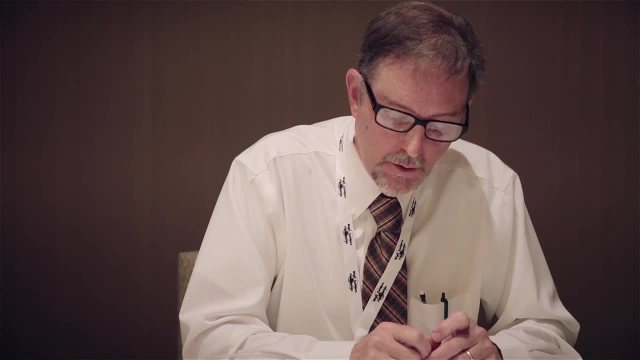 But we might think there's a stronger sense of raising children, according to which parents raise philosophical or musical or mathematical children, And that's not the case. That's not the case. It's the same thing with the math or mathematics or whatever. 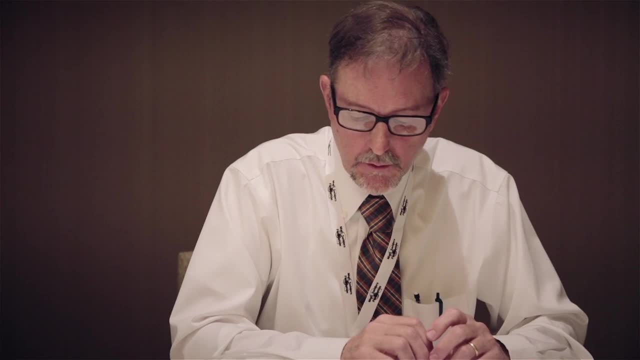 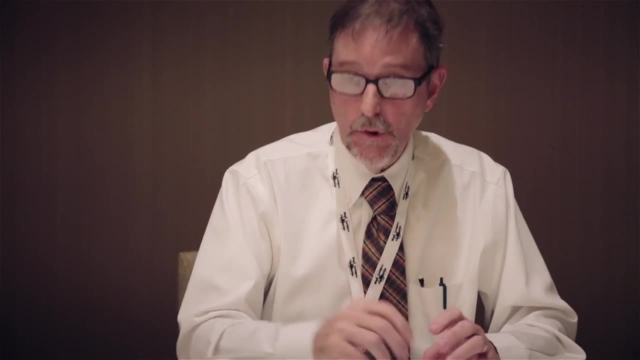 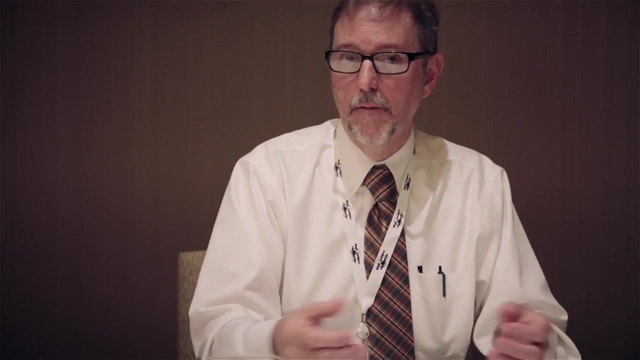 Children only when they, you know, sort of consciously pursue a deliberate plan aimed at producing children with, you know, that sort of orientation. So, on that stronger view, I mean a parent whose child turned out not to possess that orientation would have failed in some sense right in their parental lives. 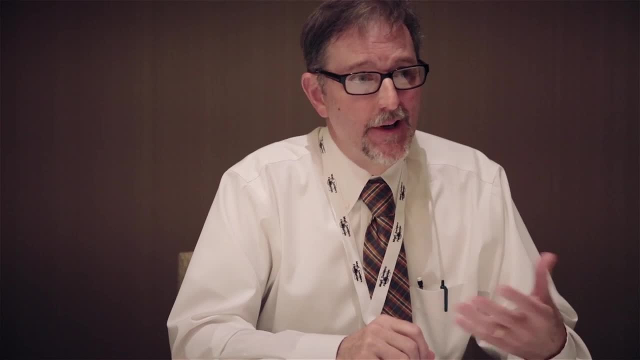 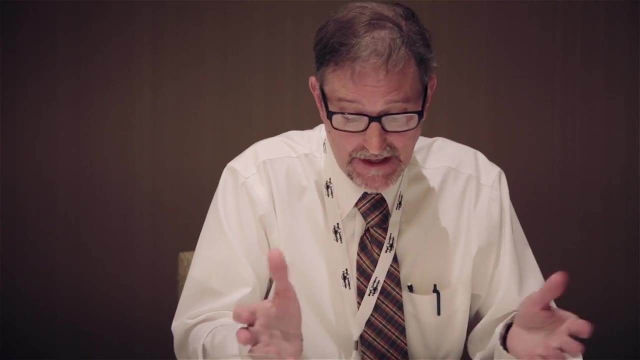 Well, so it is, as I say, only on, I think, the weaker interpretation that my partner and I turned out to have. I mean, I'm not saying that you have raised a philosophical child. I guess I'd say I'm, you know, one for three. 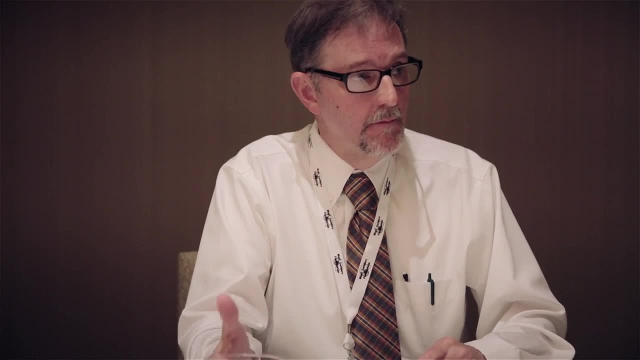 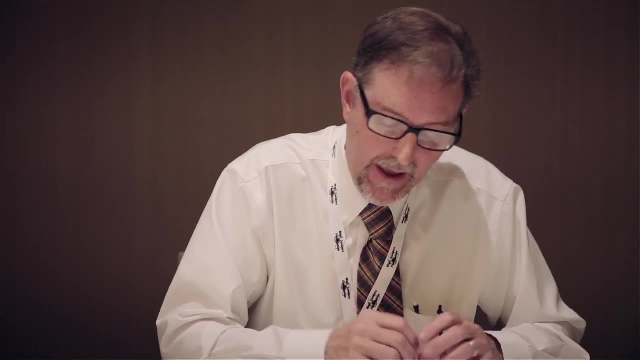 But you could imagine parents who adopt the stronger reading right. you're raising your kid, to be philosophical, only if you're kind of pursuing the aim of, you know, instilling this kind of frame of reference or worldview, whatever you want to call it. 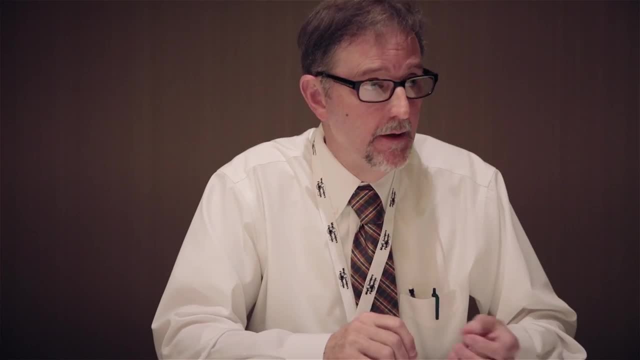 Might there be reasons for us to be concerned about that kind of undertaking? Well, maybe, But I think that question really came up. I think it's a good question And it can't be answered without tackling a much larger question, which I'm not going. 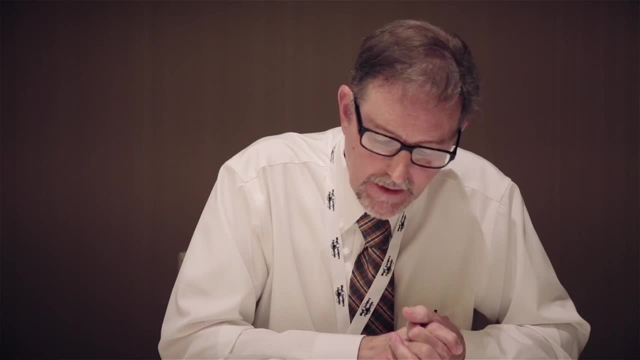 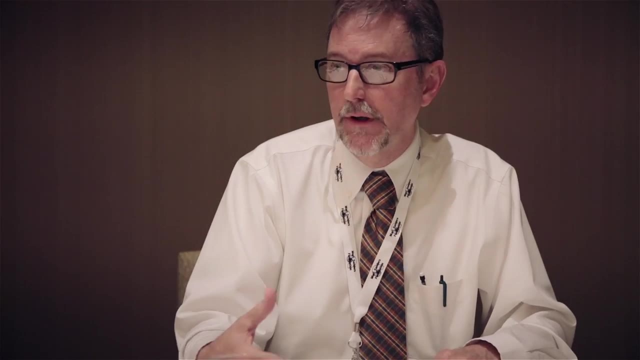 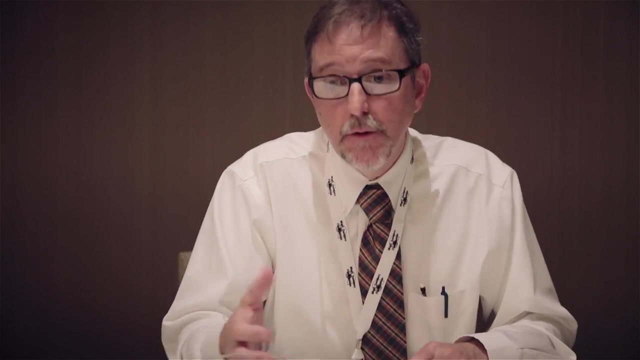 to obviously look at here, but that is how to identify the conditions under which efforts to mold children to shape their ends and preferences becomes morally problematic. But that's a much larger topic, obviously, than anything I can cover in these remarks, But I do think it merits further examination. 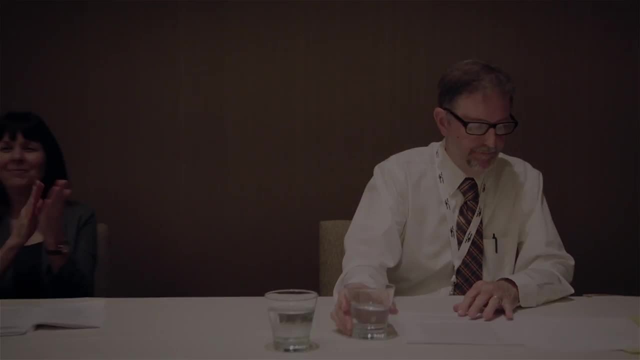 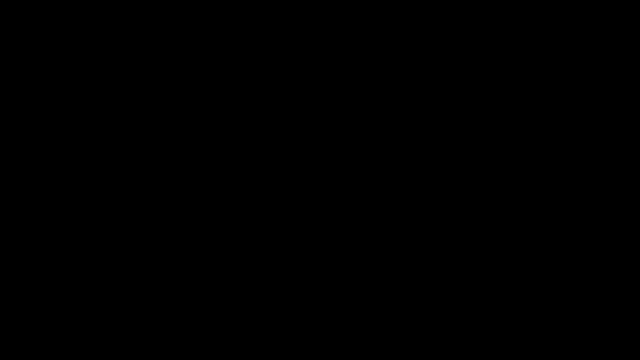